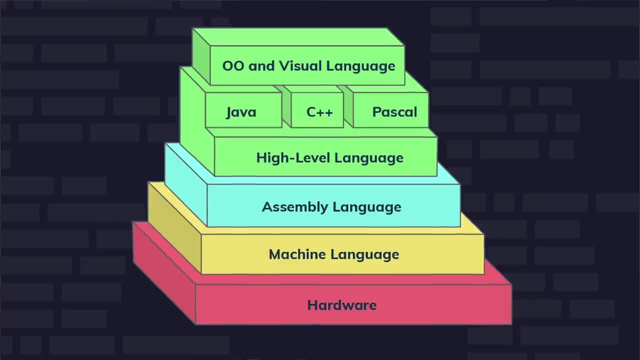 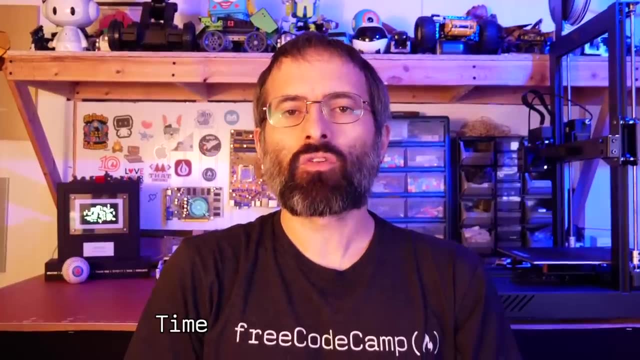 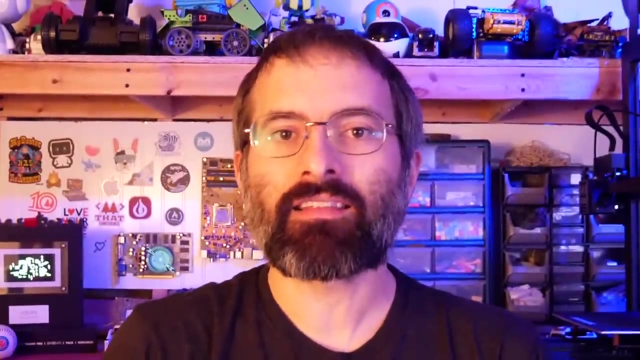 Assembly language is a low-level programming language for a computer or other programmable device that is closest to the machine language. It is often specific to a particular computer architecture, so there are multiple types of assembly languages. ARM is an increasingly popular assembly language. Scott Cosentino teaches this course about assembly programming. 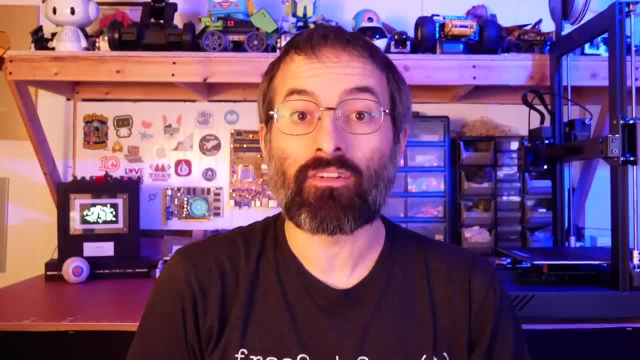 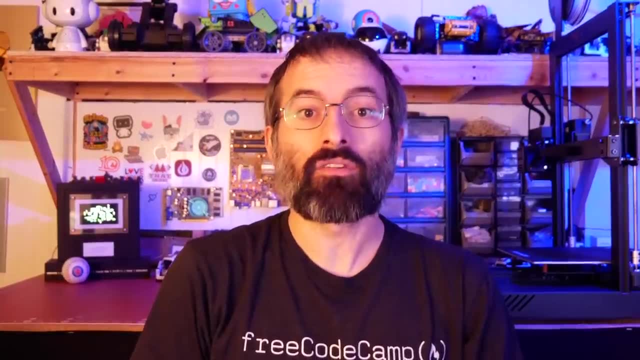 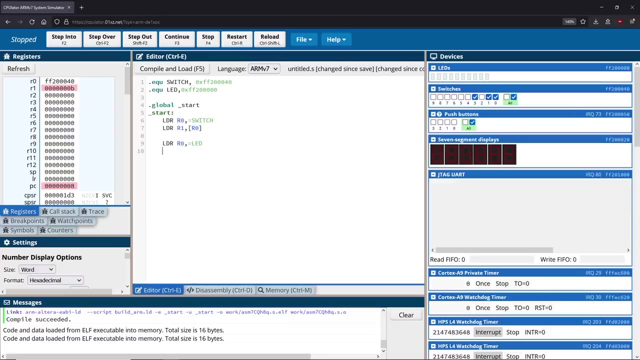 with ARM. Scott is a popular technical instructor and author. It is estimated that over 200 billion devices contain an ARM chip, making the ARM language valuable to understand. By understanding the ARM assembly language, programmers can work at a lower level, allowing them to. 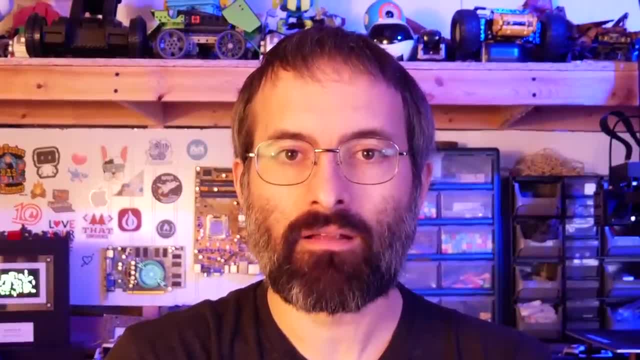 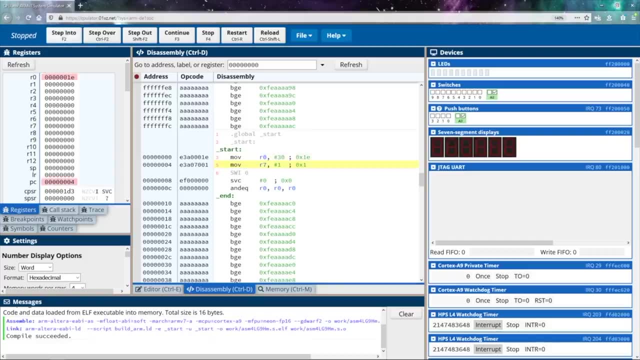 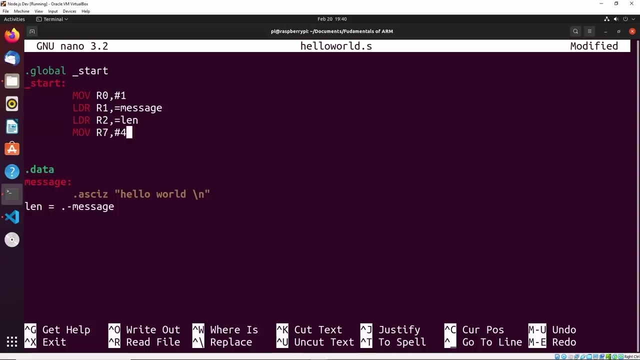 write code that interacts with hardware in an efficient manner. By the end of this course, you will have a fundamental understanding of the ARM processor, as well as the ability of assembly programming in general. You will be able to write basic ARM assembly programs using various instructions available in the processor. I encourage you to share the most. 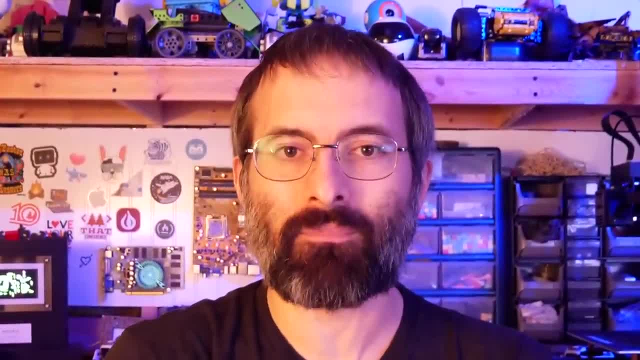 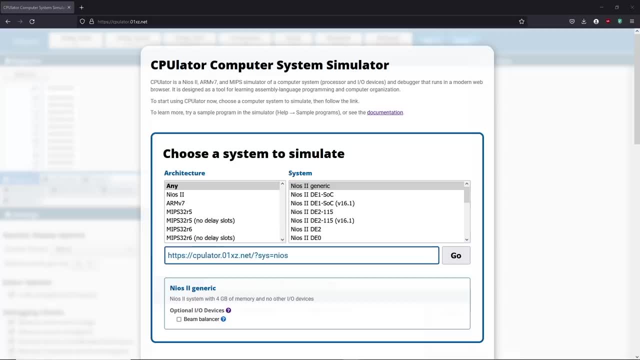 interesting thing you learn in the comments, for the benefit of other campers who are watching this course. Hello and welcome. I'm excited today to be presenting to you an introduction to the ARM assembly language. The main goal of this course is really to give you an introduction. 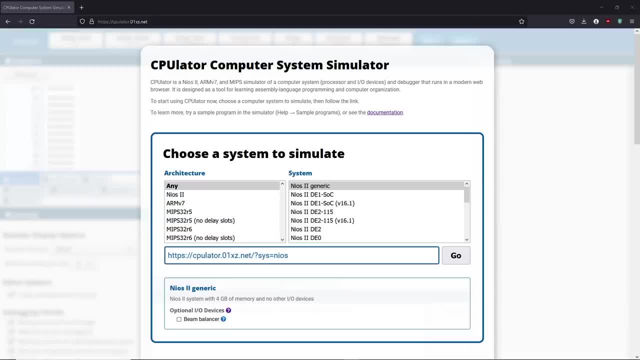 to the ideas of low-level programming through assembly languages and to help you understand the ARM programming language in general. ARM is a programming language that's used in a variety of different applications. You see it in a lot of different embedded devices and really popular devices such as different phones, A lot of Android devices and some. 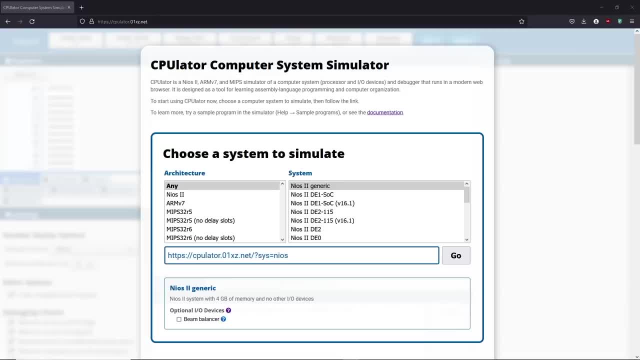 iPhone devices are running ARM-based chips and we're also starting to see them become a lot more used in. a lot of laptops, like the new MacBooks, are actually using ARM-based processors. Because of this, it's become a really important skill to actually understand. 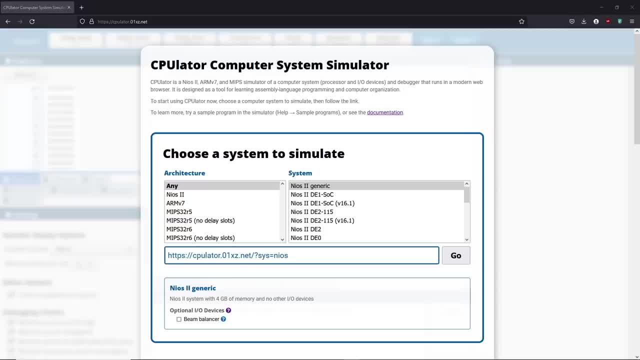 how ARM processors work and how you're actually able to program directly with them. This is because working at a lower level lets you be closer to the hardware, So let's see better interactions between the hardware and the software. It helps you more efficiently interact. 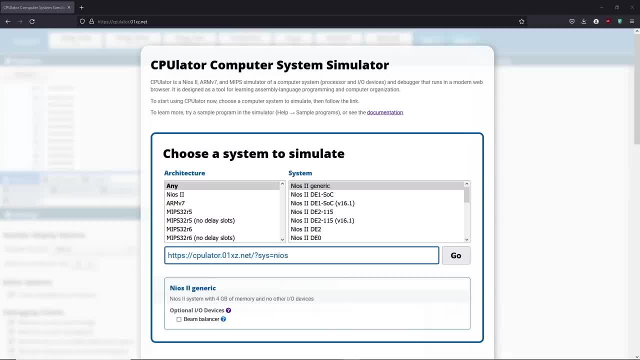 between hardware in any situations where you might need to do something like this. Generally, this course is going to give you a good familiarity with the ideas of ARM, including some of the basic instructions that ARM has, the different ways that arithmetic works and different 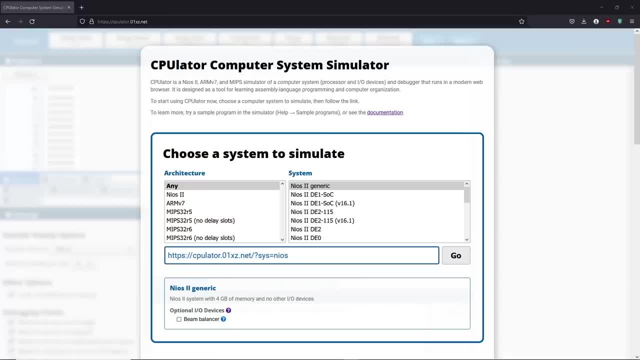 operations, such as logical operations and other things like that. This course is going to give you a good familiarity with the ideas of ARM, including some of the basic instructions like numbering operators and shift operators that are commonly used in the local assembly languages. We'll take a look at different ways that we can branch as well as loop inside. 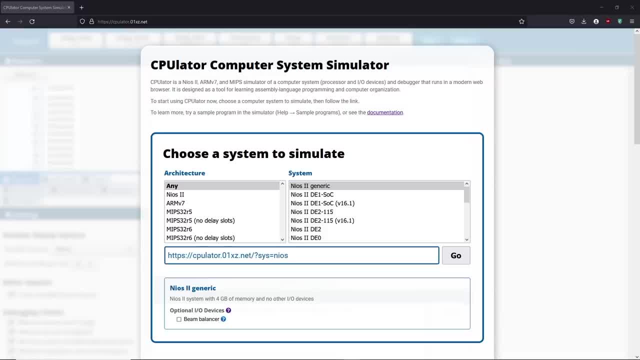 of assembly languages, And then, finally, we'll finish off by taking a look at some hardware interactions and as well as the different ways that we can use and troubleshoot ARM assembly in a Linux based system. Now, I'm going to primarily be using an emulator known as CPU-later, as it's very easy for you to follow along with this. 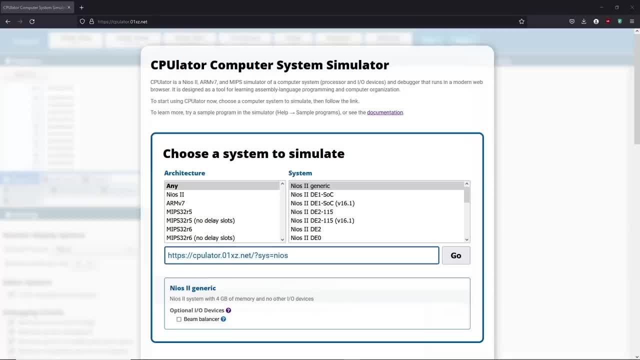 on the actual web browser that you have, So for the most part, you want to install a any sort of special equipment in order to make this work. The main approach here is to make sure that you can be able to interact with this course and follow along easily. 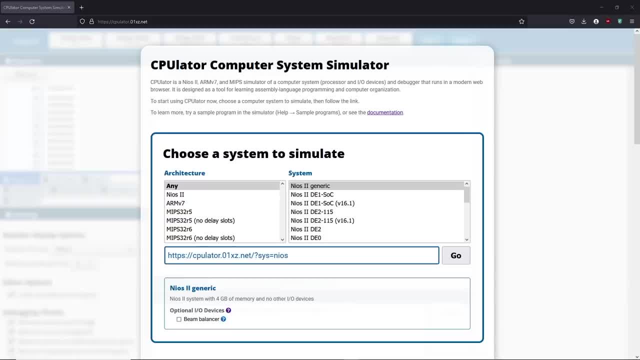 without any sort of special prerequisites. Now, the last few videos here are going to be Linux-based, so you will need some Linux-based machine or virtual device to be able to follow along with those. But overall, even if you just follow along with the emulator ones, you'll come away from this course. 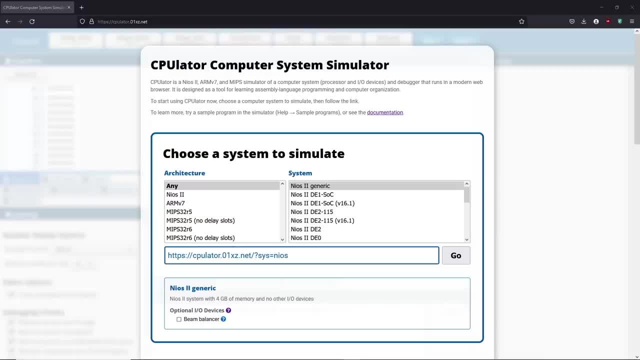 with a very strong understanding of ARM as well as assembly languages. So I hope that this course is valuable for you and I hope that you enjoy it. If you enjoy it, please feel free to leave a comment and let me know, And if you have any sort of questions, also let me know. 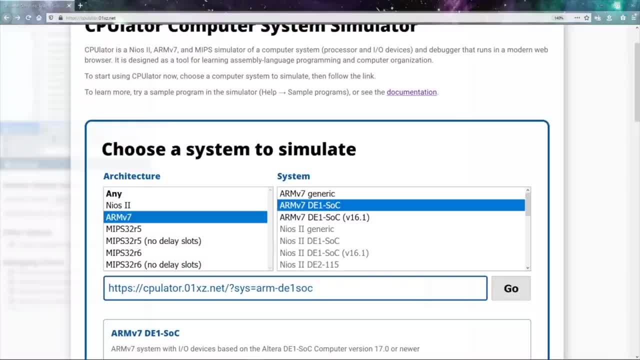 and I'm happy to answer anything that may come up. So in this video I'm going to spend some time just discussing the general idea of our architecture, of our ARM processor, as well as getting familiarized a little bit with the development environment that I'm going to be using in this set of videos. 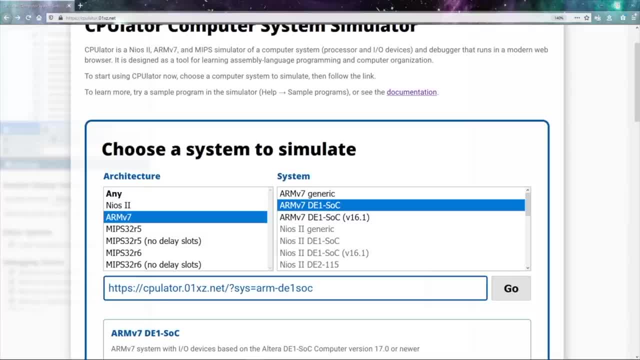 which is actually the CPU Leader Emulator. This emulator is available online for free, so you can access it from pretty much any computer, And inside of this emulator we have a lot of different architectures that exist. for us, The one that we're mainly interested in is ARMv7.. 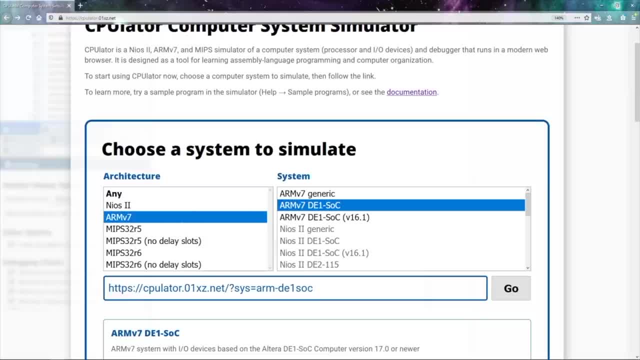 If you're familiar with MIPS or any other assembly language like that, you'll see that those emulators are also available for you. But generally we're going to be working in an ARMv7 architecture And specifically in this set of videos. 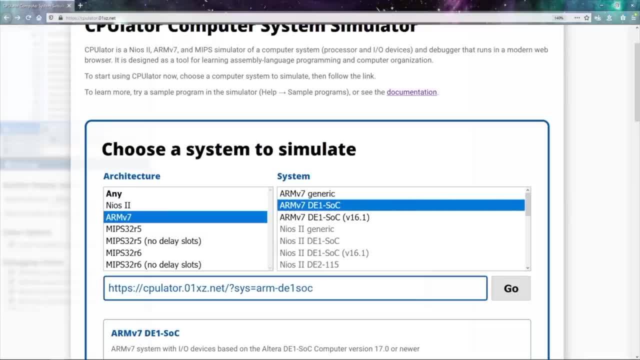 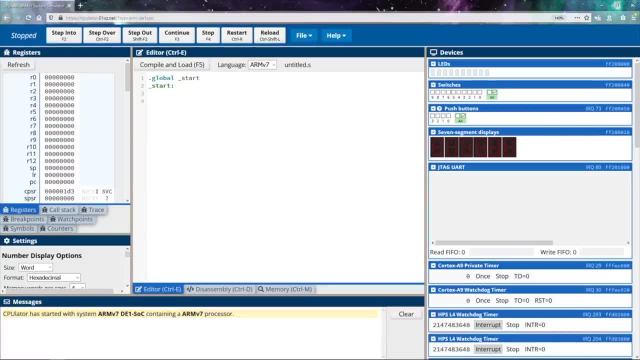 I'm going to demonstrate the ARMv7-de1-soc, So this will be the one that we'll utilize throughout this series of videos. So I'll press Go and we'll head into the emulator. Just a note if you're following along. 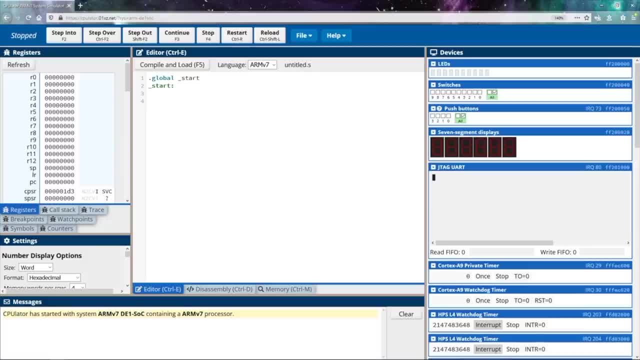 you can follow along through the emulator here or you can follow along on your own computer. if you have an ARM processor of some sort- Any v7 processor- you'll be able to follow along. fine, with Even earlier ones you'll probably be able to follow along relatively well. 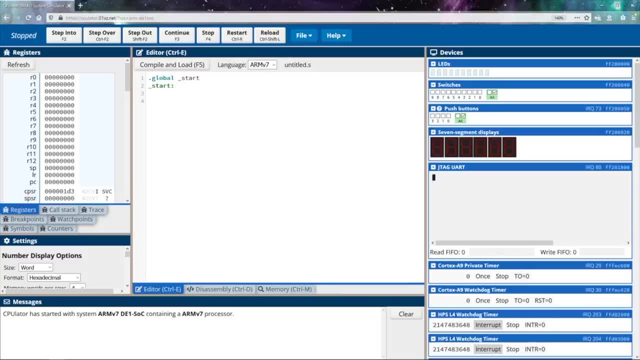 The main goal of this video is not just to teach you ARM-based assembly, but also to teach you the general principles of assembly so that you can easily adapt to any of these Any other assembly language things like x86, other versions of ARM and so on like that. 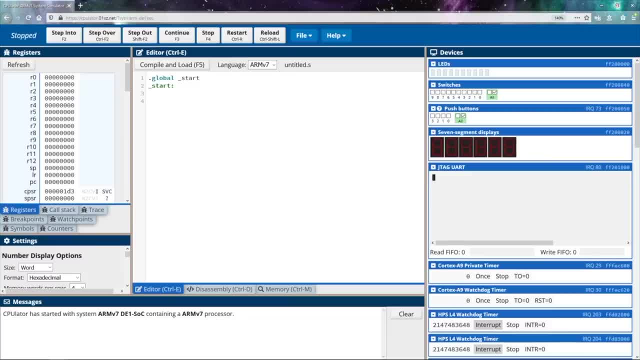 So, in general, the principles that you learn throughout this series of videos are going to apply to really any assembly language, with the syntax specifically being targeted towards ARM processors. So when we get into our emulator, there are a few things that we have available to us. 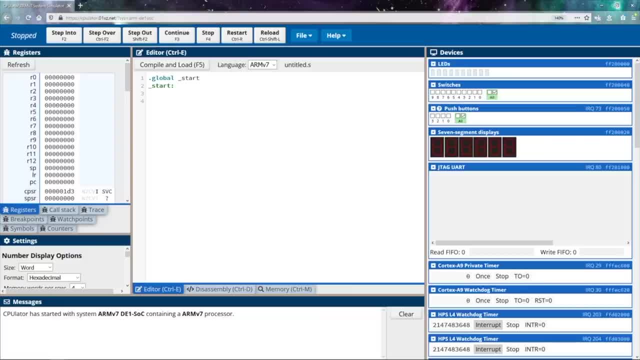 Well, there's actually a lot of things on the screen that we have available to us, And I'm going to walk you through some of the essential pieces that we need, just to get started. So the first idea that I'm going to introduce to you: 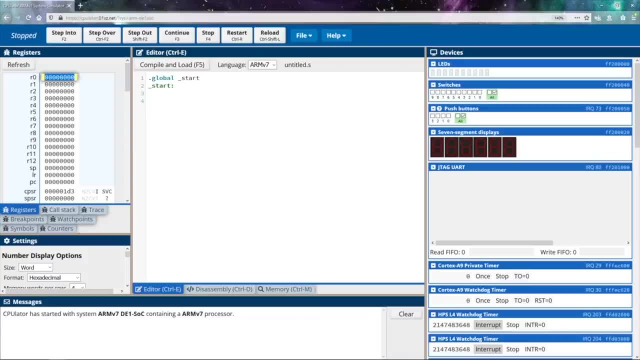 is the idea of registers, which we see over here on the left-hand side. Registers are areas in memory that are very close to the CPO, So they can be accessed quickly and they can be written to quickly, So the general storage is going to be relatively fast. 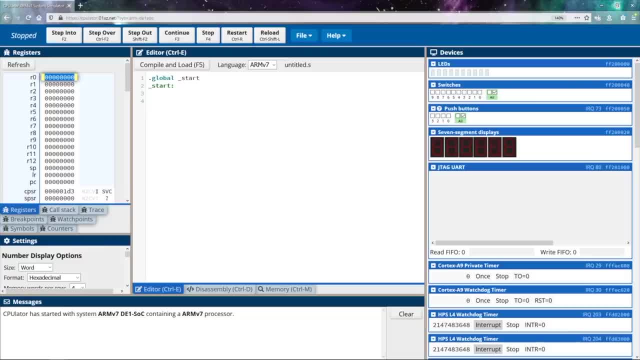 However, we have a limited amount of things that we can store inside of these registers. You'll notice that there's eight zeros inside of this register. Each zero represents a single hexadecimal value. Now, if you know about hexadecimal, you'll know that hexadecimal is going to represent four bits. 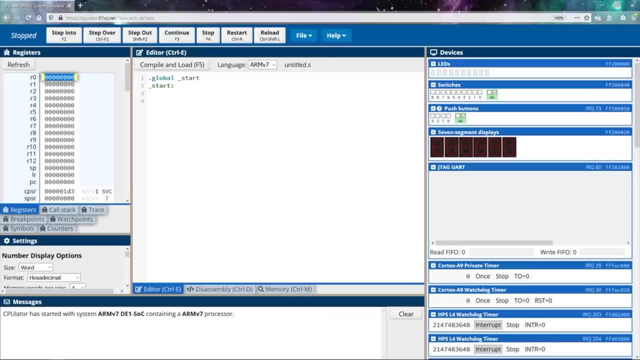 So each hex value represents four bits of data. Since there's eight hex values, each one represents four bits. We have a total of 32 bits that we can work with. This is because this general processor is a 32-bit processor, So we're going to be working in 32 bits. 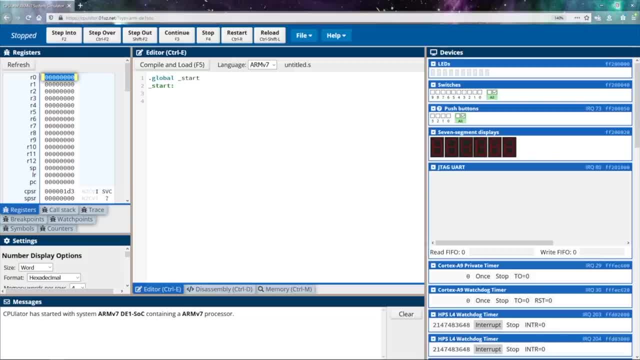 And that's the constraint of how much we can store in a single register. is 32 bits worth of data? We'll often refer to 32 bits as a word in terms of the size, So if you ever hear me refer to as changing a word's worth, 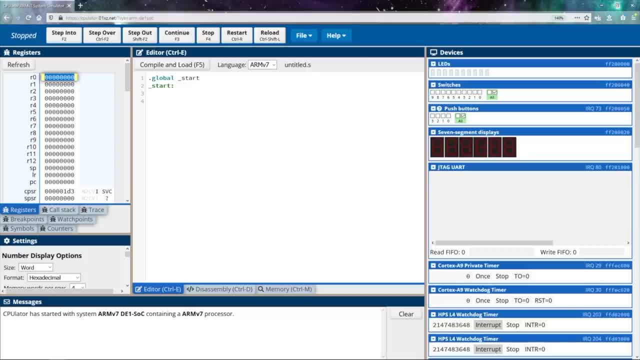 of data. I'm referring to 32 bits of data. The idea of a word transitions to other assembly languages as well, And it generally represents the total max size of data that could be stored in a register. So, for instance, if you were in a 64-bit processor. 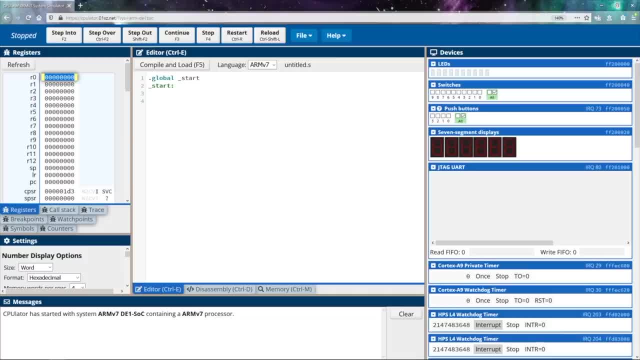 a word would be 64 bits in size, And then we have a little bit of a difference And then we have the concept of a half word, which is half the size of a word. So in 32 bits a half word is 16 bits because it's half of 32.. 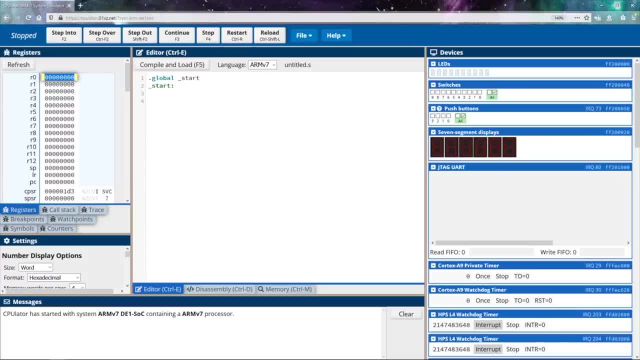 In 64 bits, a half word is 32 bits, because it's half of 64. And then, of course, we have a byte which is always 8 bits, And then we have a single bit of data. So those are the different sizes that we have available to us. 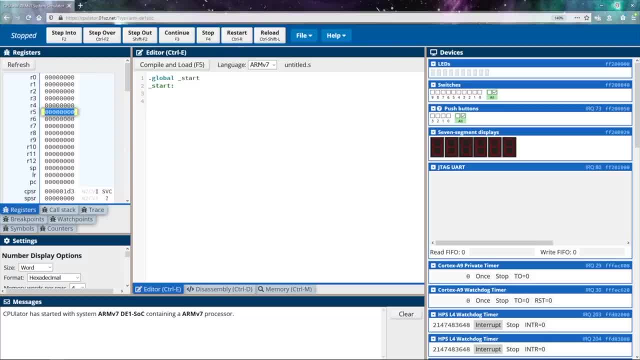 So in general, when we're working in assembly, we want to try to use these registers as much as possible. So all of these registers are going to be available to us, Exception that some of them are going to have special purposes associated with them. 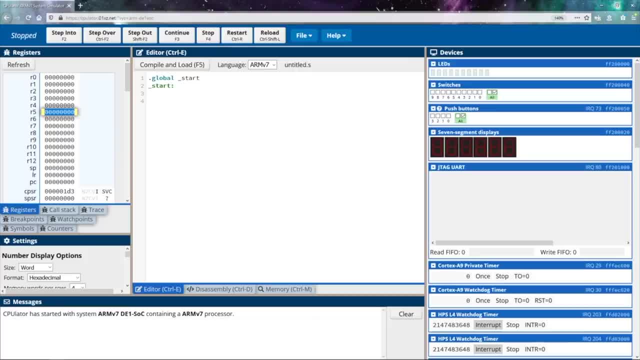 that we'll discuss as we start to see those special purposes later on. In general, I can say that registers R0 to R6 are general purpose. We can use them for whatever storage we'd like to use them for. R7 is going to have a special functionality to us related. 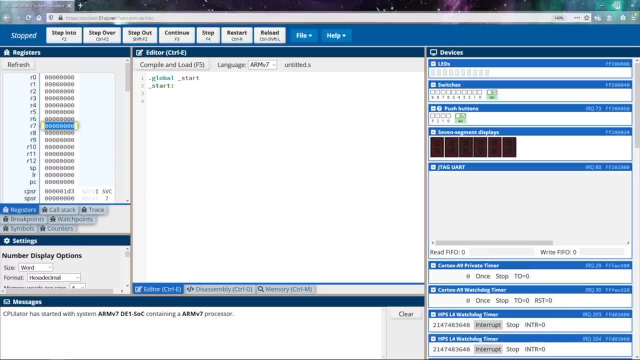 to system calls. Essentially, when we are working with assembly, sometimes we need to talk to the operating system And we need to ask it for, maybe, a resource or we need to ask it to terminate our program. When we call to the operating system, 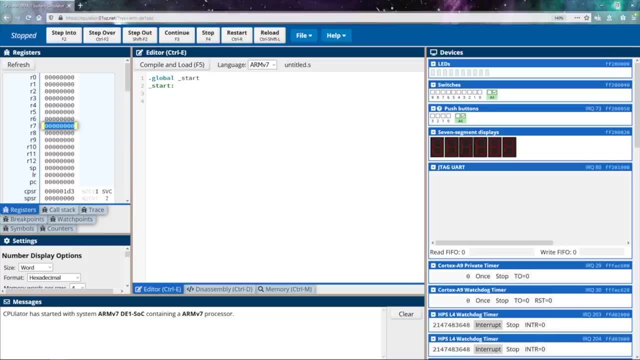 to ask it to do something for us, it needs to know what we're asking it to do And the way that we communicate, that is, by storing a value in R7. And that value will be some numeric value that it will map in a table to some specific action. 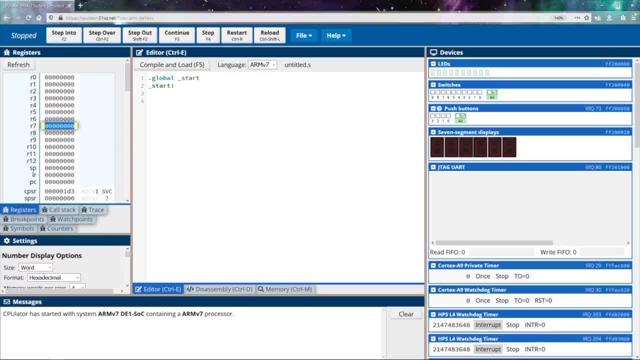 So, for instance, if I store the value 1 in R7, and then I interrupt the program, the operating system will read that and interpret it as end the program. So that's an example of how we might use that. So that's one example of a special purpose register. 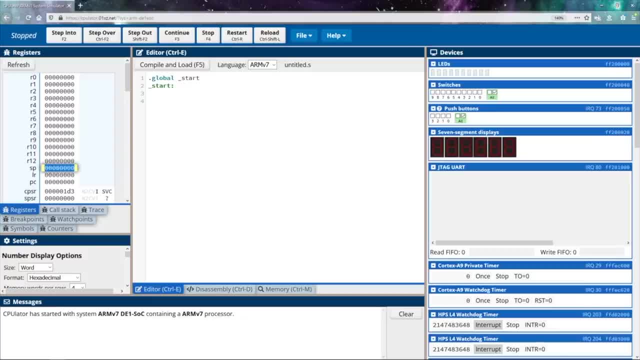 that we have. Now. there are other special purpose registers that are actually labeled in this emulator: SP, LR and PC. SP is a really interesting one, which is related to the stack pointer, And that actually introduces us to our next important concept. 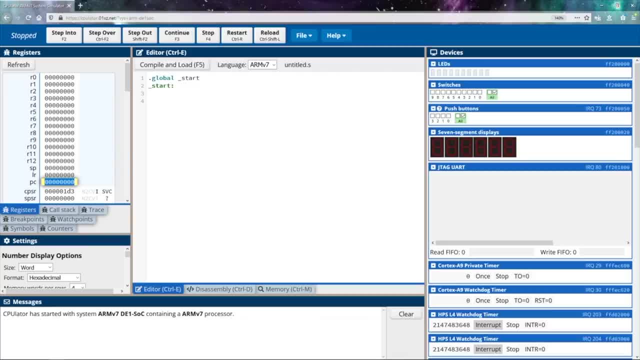 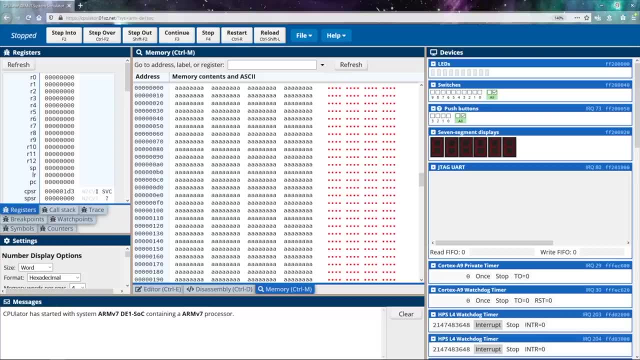 which is the concept of stack memory. If you head over to the memory section here, you'll see that you have a whole bunch of memory available to us, And this is referred to as stack, And this is referred to as stack memory. Stack memory is typically stored in the RAM of the computer. 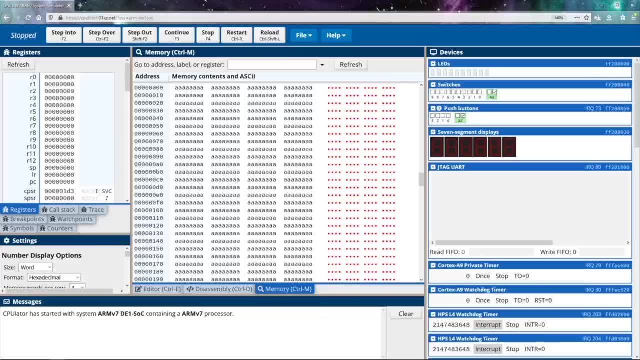 And essentially it's slower to access and slower to write to. However, we can store a lot more data in RAM comparative to data in registers. You'll typically see stack memory used when we want to represent more complex sets of data. Think of something like a list of numbers, for instance. 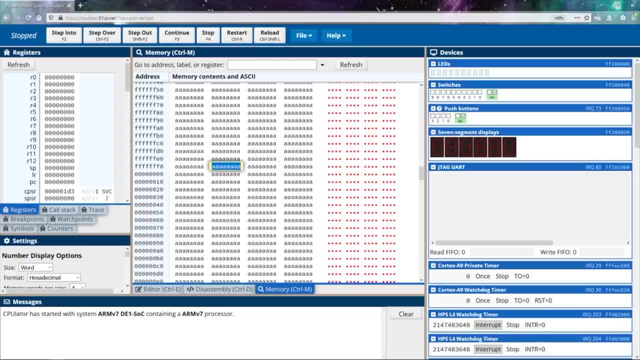 If I were representing a list of numbers, I could give each location in memory a specific number. If I were representing a list of numbers, I could give each location in memory a specific number, And that would be a list of the number of memory locations. 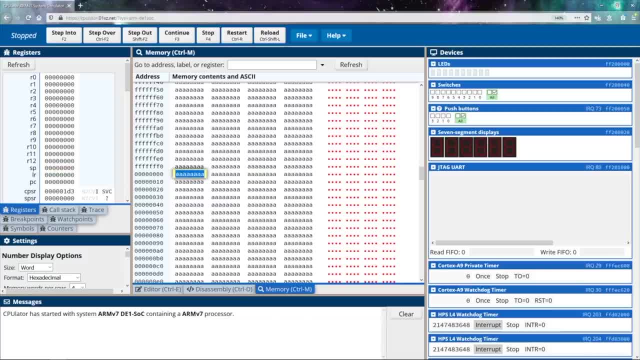 to get those numbers. That would be an example of when we might use stack memory. So the SP register is always going to be telling us the address of the next available piece of memory on the stack. So in this case, you see, it's pointing to all zeros, which. 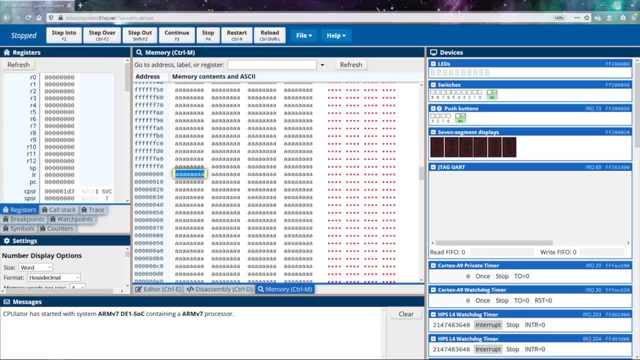 means that we are sitting at this location here. Now, in order to determine the actual locations, we can think of the address next to this. It's always going to be 4 larger than the previous, So this is at address 0.. 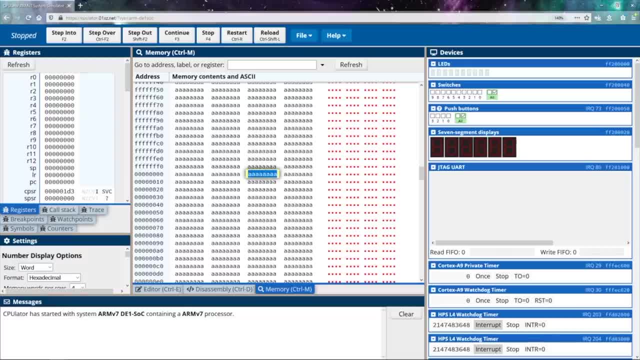 This would be at address 4.. This would be at address 8.. This would be at address 12.. And then we land here at address 16.. Now you might look at this and say, well, it says 1, 0.. 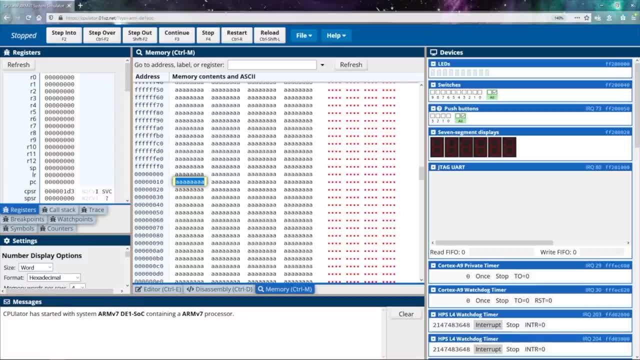 Isn't that 10?? Remember that we're working in hex. 1, 0 in hex is 16 in decimal, So just keep that in mind, that you're always working in hexadecimal. So that's just something to keep in mind there. 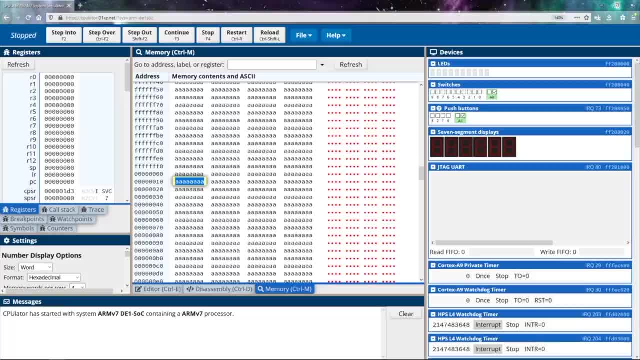 And that's the way that our stack memory grows, And you'll get really familiar with stack memory. We're going to work with it a lot throughout this series of videos, So you'll get a really good understanding of this as you continue to work with it. 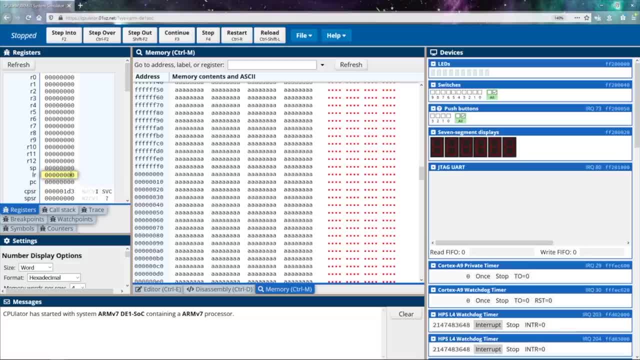 The LR register is another interesting one. It's known as our link register, And the best way to describe this is: if you've ever worked in a higher level language before, you'll know that when you have a function, a function has a return. 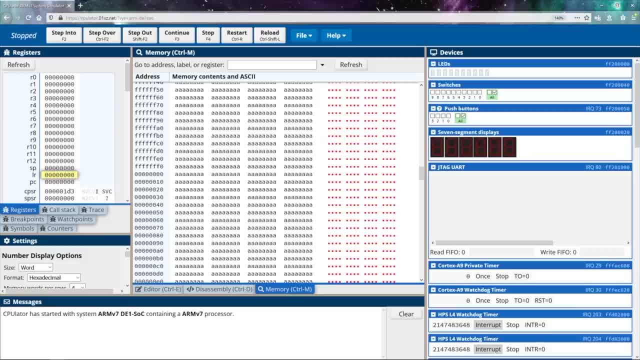 And that return allows us to move back to the location of what called the function. That's what the link register stores. It stores the location that a function should return back to, So we'll see that when we talk about functions in future videos. 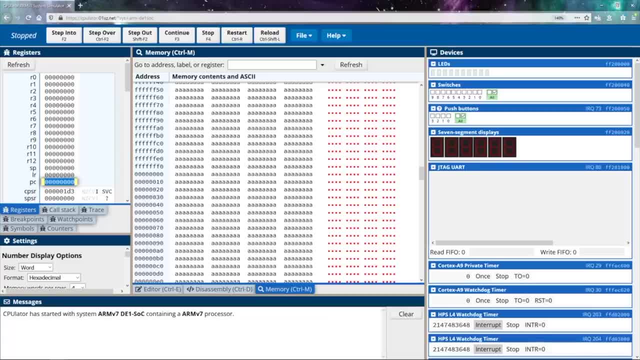 And then, finally, the PC is our program counter. What this does is it keeps track of the location of the next instruction to execute. So all of our instructions are stored in memory, like all the different things that we're asking the program to do. 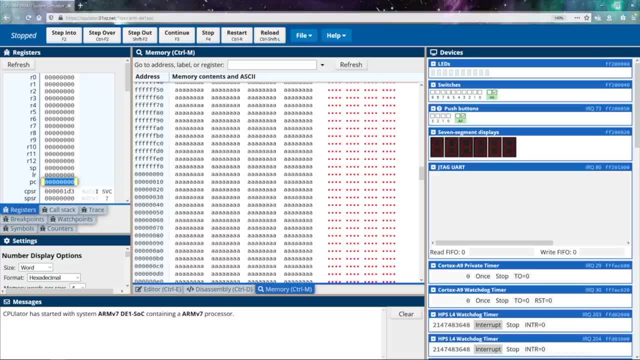 And the program counter allows us to move through piece by piece and determine where the next instruction is going to be located. So those are three really important registers to keep in mind And, like I said, some of these other registers have special purposes as well. 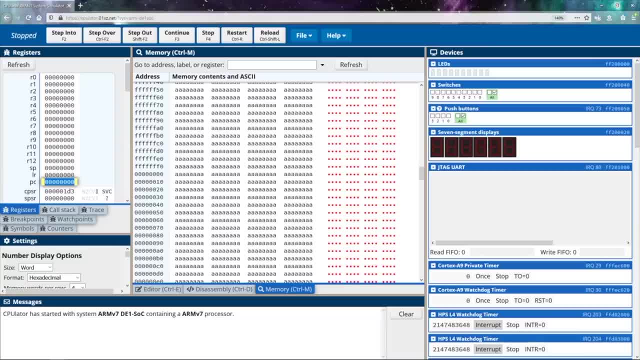 And we'll discuss those as they become relevant to us as we continue on through this. The one final thing that I'll discuss here is our CPSR register and our SPSR register. Our CPSR register is a special type of register that is used to store information. 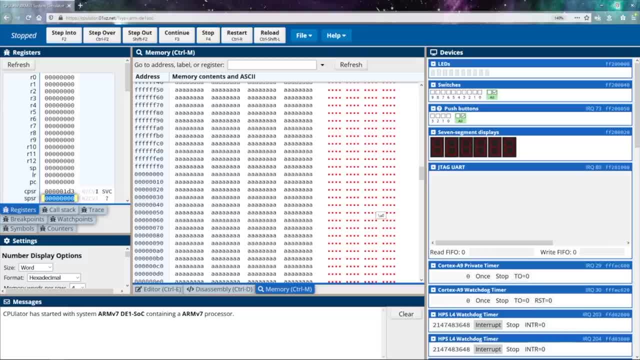 about our program. So an example of some of the information that it might store. if you subtract two numbers from each other, you might end up with a negative number. Now, if you remember in binary when we want to represent negative numbers, 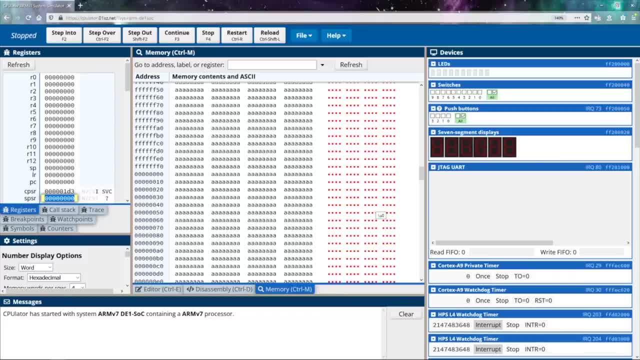 we need to use what's known as two's complement. Two's complement, essentially, it goes through some conversion mechanism in order to convert us into that format. We have to do the one's complement and then we do the two's complement and we end up with some number that 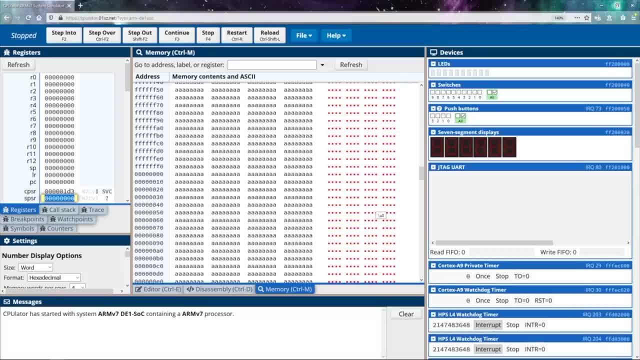 represents a negative number. The issue is that that number could also be a positive number, So it's both positive and negative, but we need to know whether or not it's representing a negative number or just a really large positive number. That's where our CPSR register comes in. 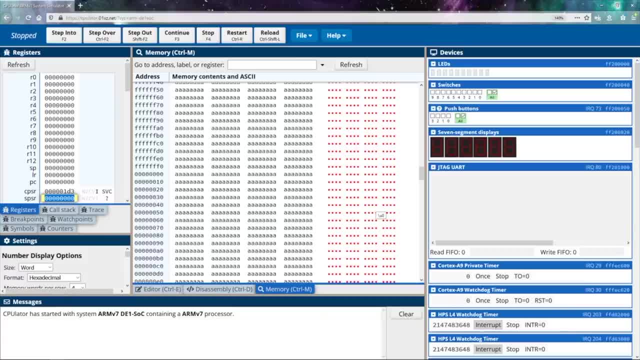 What it will do is it will set a flag in memory to say the result of the previous operation was negative. We can then take a look at that register and say: if the result was negative, interpret this as a negative number. Otherwise, interpret it as a positive number. 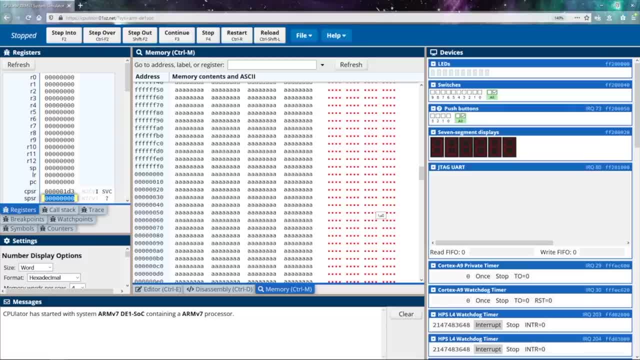 That's sort of the purpose of the CPSR register. It has a whole bunch of flags- It's sort of similar to that- that tell us special information about the operations: If a result was negative, if a result was zero, if a result had a carry or an overflow. 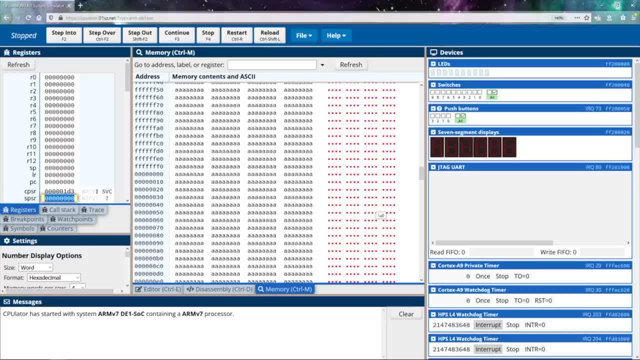 those are the sorts of ideas that we would typically see, So we'll see those again as we continue on learning about the different operations. So this gives you a general overview of some of the important components that we need to start programming in ARM assembly. 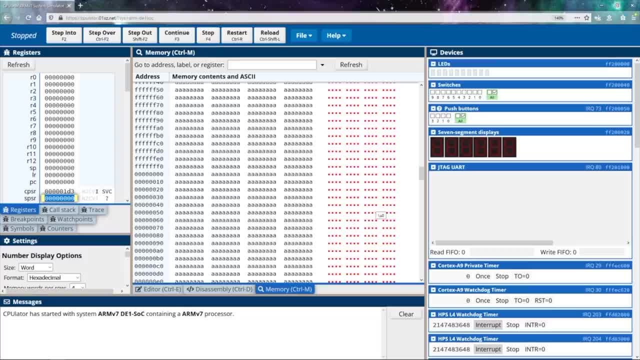 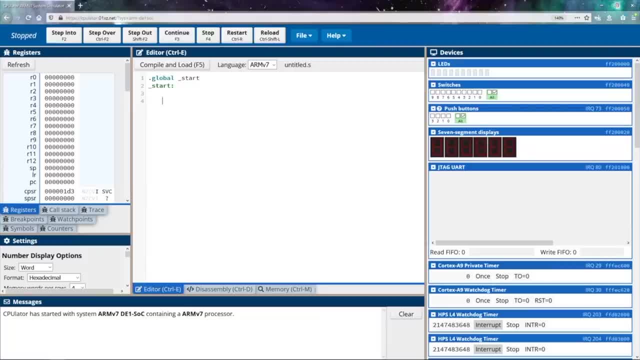 And in the next video we'll take a look at how to create a really basic assembly program. So that's it. That's what we'll take a look at next. So in this video we're just going to take a look at a really basic ARM application- just. 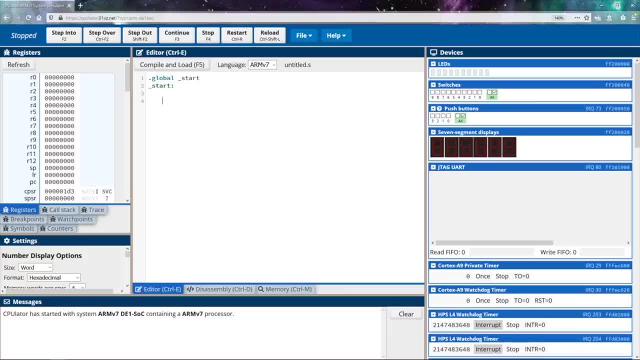 to get a really good fundamental feel of the structure of our programs as well as the way that they actually run. So we're going to go over a lot of the important concepts of where the starting point of our application is, where the ending point of our application is. 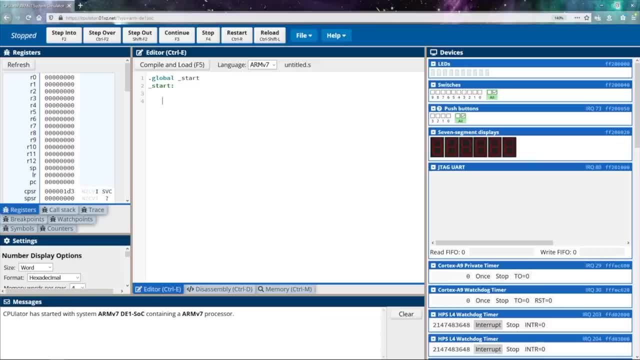 and how can we do all of the things in between. So, starting off with this idea, let's discuss the starting point of our program. You'll see that our emulator automatically puts in two lines for us. Now, if you're programming outside of the emulator, 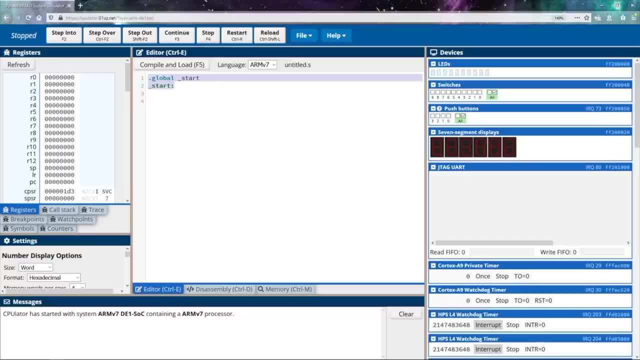 you won't have these two lines added by default. You'll have to add them yourself. But they are essential because they tell us the starting point of our application. So let me break down the lines one by one here. I'm going to start backwards with this underscore start. 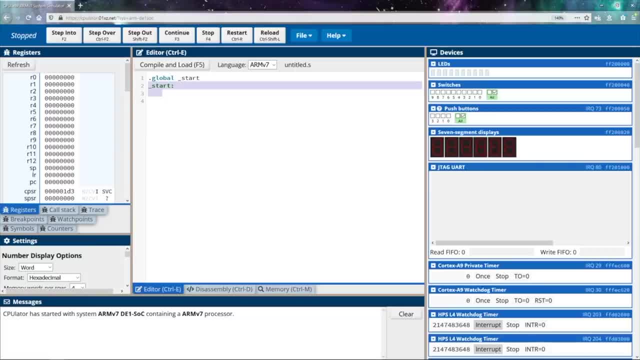 portion. here This is known as a label. A label is sort of synonymous with a function in higher level languages. It's a way of being able to divide out segments of code such that if you go to the label, you start to execute the code that is underneath that label. 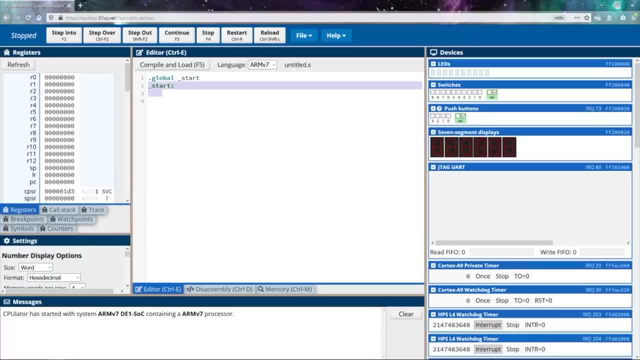 The idea of this is that we set up a start label which then we are able to say, OK, go to the start and start running the stuff that's there. That's the idea of what we're looking to do, So that's why we define our start label. 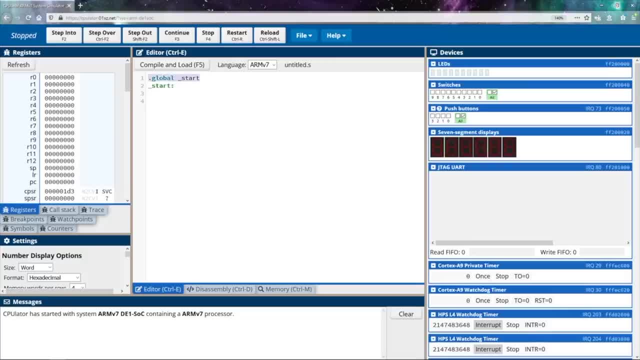 And then our global underscore start. here is a way of being able to tell people what is the starting point about the start label. So someone is going to be running our program, So at some point something is going to be running our program. 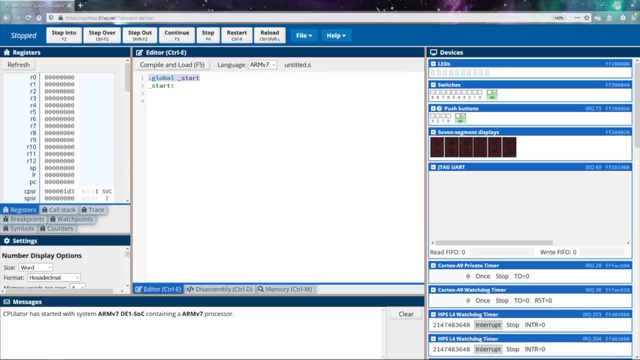 It needs to know where the starting point is as well. When we define labels, by default they aren't available to anything external to our program. The dot global is telling everyone else about our start label, So if anyone ever approaches our program and says I want to run you, where is the start? 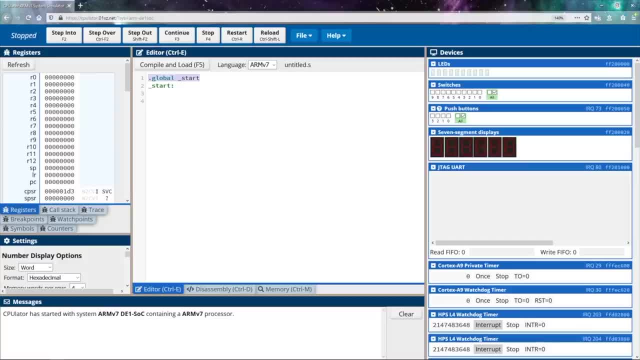 The start is exported via this global, which means that everything is able to see where the starting point is. Therefore, things are going to be running and things are able to go to the starting point to start executing our program. So this is the general idea of our main starting point. 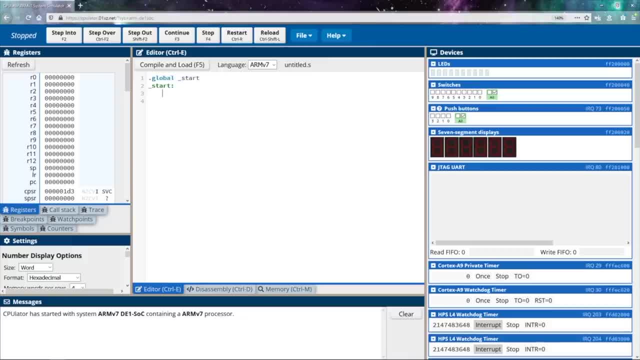 of our application. So everything that we write is going to be underneath this start label. So that's where we're going to start writing our code, And the code that I'm going to write is going to be very, very simple. All it's going to do is it's going to move some data. 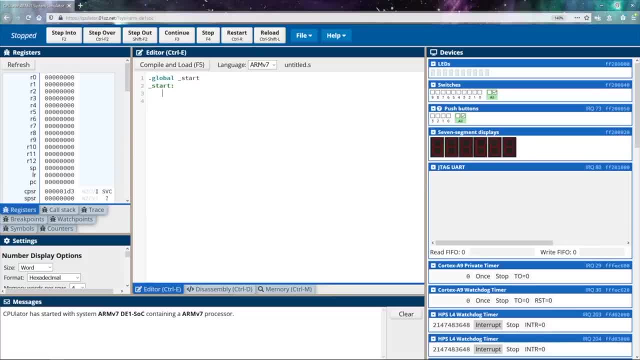 into register 0. That way you can see how we move data into registers. And then I'm going to move some data into register 7.. It might seem a little bit weird- Weird- that I'm jumping straight to register 7.. 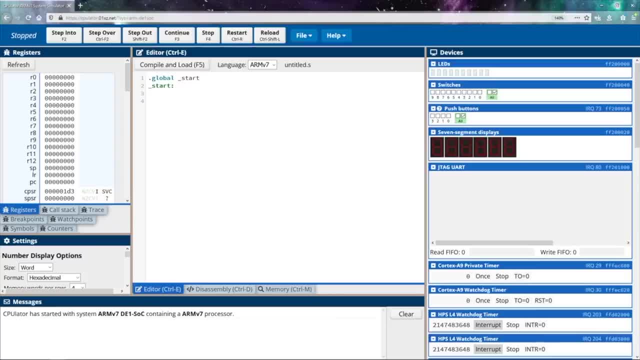 The reason being is because register 7 is a special purpose register. What it does is it stores information about system calls. When we go to the operating system, we often want to ask it to do specific things for us. The operating system manages input. 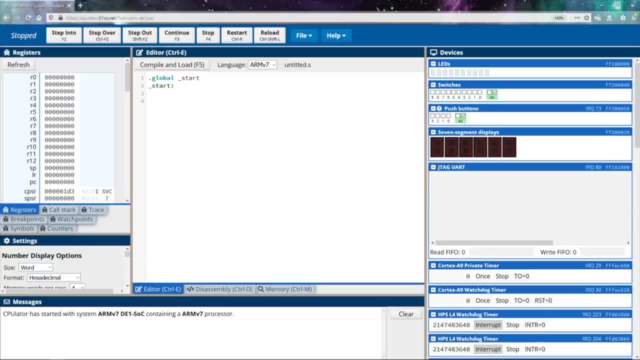 It manages output. It manages the execution of programs. So if we need the operating system to do something for us, we need some method of communicating with it. This method of communication comes in two pieces: The first is in system interrupts And the second is in system call numbers. 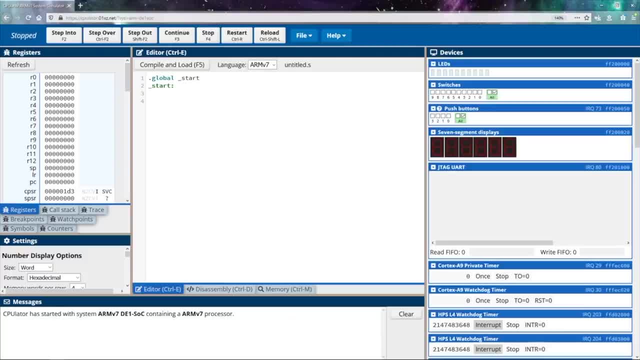 So we place a special number into register 7. And that tells the operating system what we would like it to do. So basically we place the number to R7. And then we call an interrupt. That interrupt goes to the operating system. 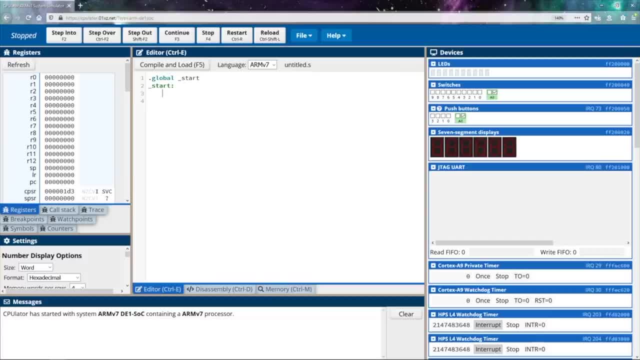 And it says: hey, we need something done. The operating system comes in and it reads: register 7. Which has some number inside of it. It takes that number and it compares it to a lookup table And it says: OK, well, that number. 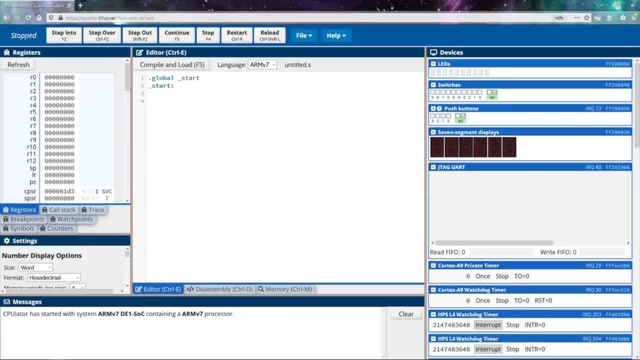 corresponds with this task And then it completes that task for us. In our case, our task is very simple: We want our program to end. So if I want to terminate the execution of my program, what I do is I move the number 1 into R7.. 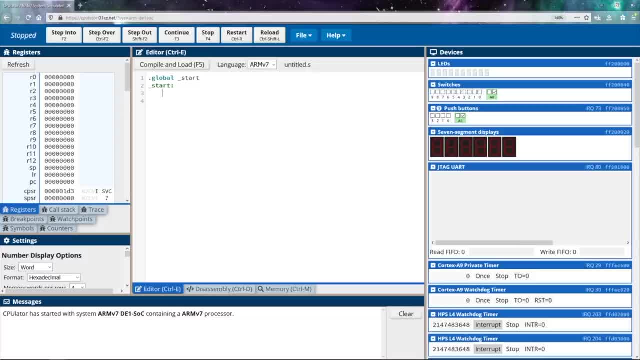 And then I call an interrupt. The operating system then goes to register 7.. It says, oh, I see the number 1 here. It goes to its little table And its table says 1 corresponds to exit the program. And then it terminates the program for us. 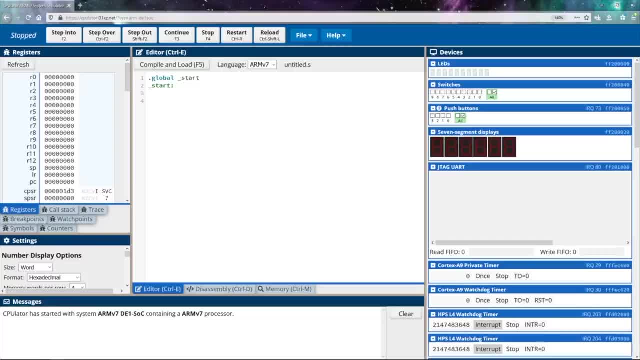 So that shows us how we end our program. So let's take a look at how that's actually written. So the first thing I want to do is move some data into R0.. That way we can see just generally how we can move data into registers. 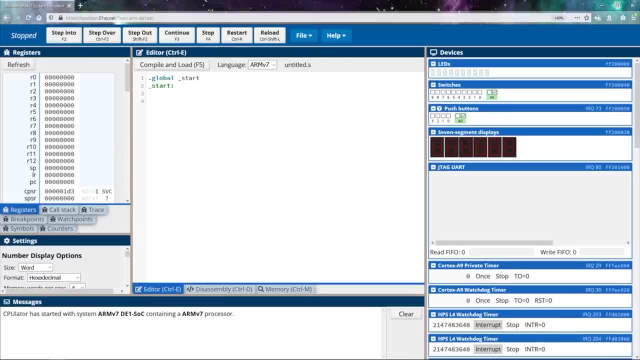 and what that looks like during execution. So the way that we do this is as follows. We're going to start by writing in what's called an opcode. Well, you'll see it set in a number of different ways either. opcode operation. 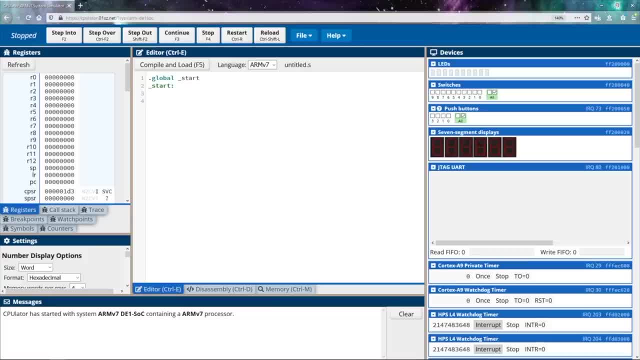 Mnemonic is also used. I'm going to refer to them as operations or opcodes. So we're going to start by writing in the operation that corresponds to moving data And that is MOV. Now I use capital letters for mine, You don't have to do that. 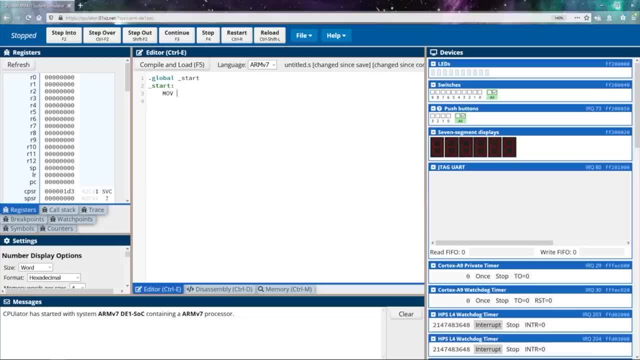 You can write it in lowercase as well. I just prefer this convention, And this is the one that I'm most comfortable with, So this is the way that I usually end up writing it. So the way that our move operation actually works is we're going to move data into locations. 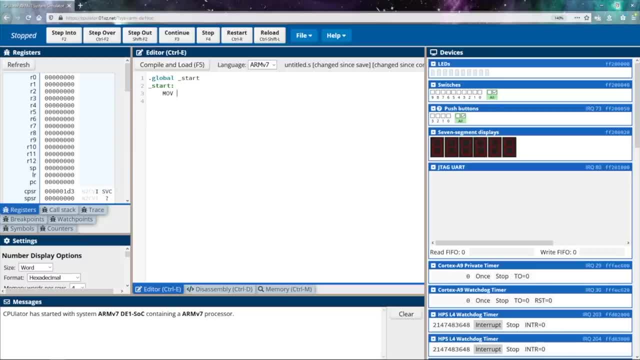 Specifically, we're going to move data into registers. So what we need to do is we need to provide it with two things: We need to give it a destination for our data as well as a source for our data. So the source is where we're getting the data from. 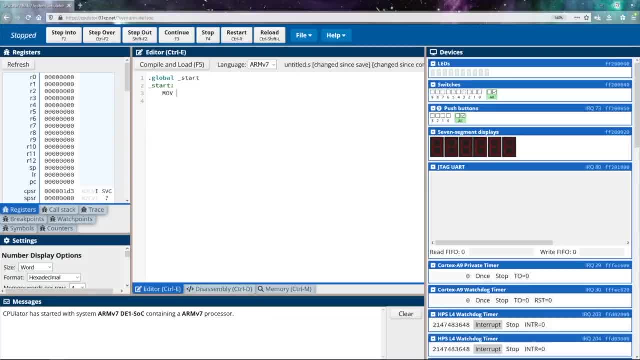 The destination is where the data is ending up. The destination is the first argument given to this operation And then the source is the second argument. So my destination in this case, where I want to store the data, OK, So my destination in this case is R0.. 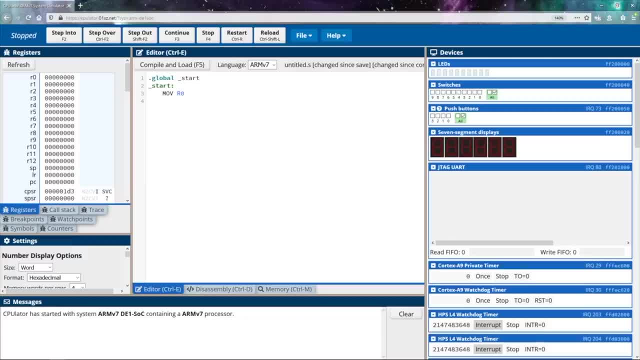 Again, I put a capital R. You don't have to. You can use a lowercase R. It's not actually case sensitive. I just prefer the convention for capital letters, So that's what you'll see me use. So I'm going to move into R0, the value. 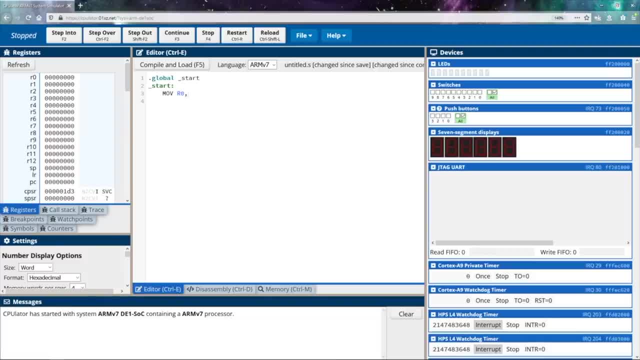 So I put a comma And now I'm going to specify the source. So my source could be a number of different things, And we're going to go through these different things as we continue learning about assembly, Because we can move data from registers. 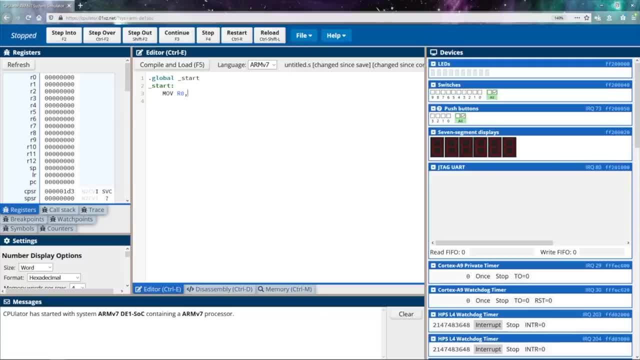 We can move data from memory, Things like that. In this case, I'm going to be moving a constant value into this register. So the way that we do this is we put in a hashtag And then we put in the value that we want to move in. 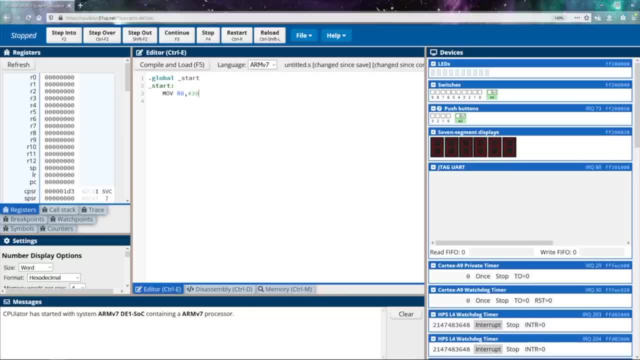 I want to move in the number 30 in decimal, So I just put hashtag 30. All this does is it takes the number 30. It places it into register 0. And that's it. That's how we move the data into the register. 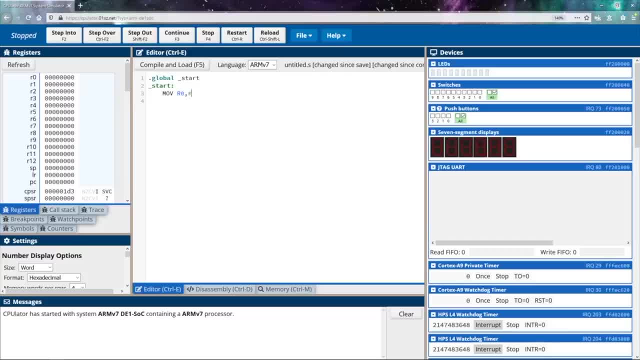 Now, one thing I want to point out to you is that you can put hex into these registers as well. The way that you do that is you put 0x and then the hex value that you want to put in, So, for instance, 0x, 0a. 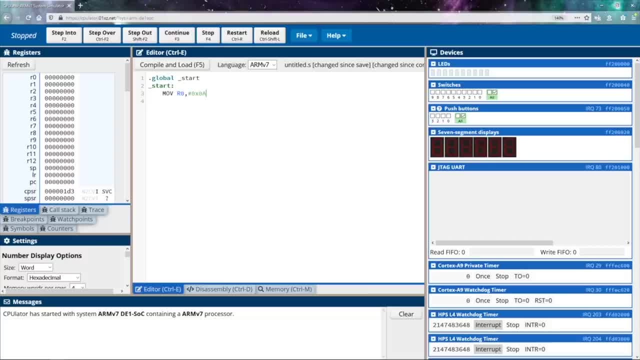 We write the value 0a into register 0.. So I just want to point out that that's the way that you do hex. In this case, I'm working in decimal And I'm pretty much always going to be working in decimal. 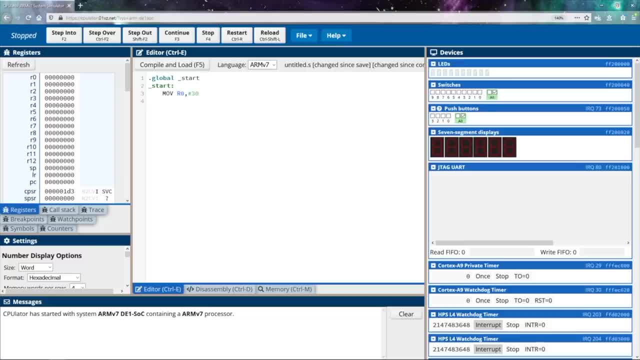 unless I have a very specific reason to be using hex, Just because I'm most comfortable with decimals. So that's what you'll see me using throughout this. So I move 30 into register 0.. And now we're going to do. 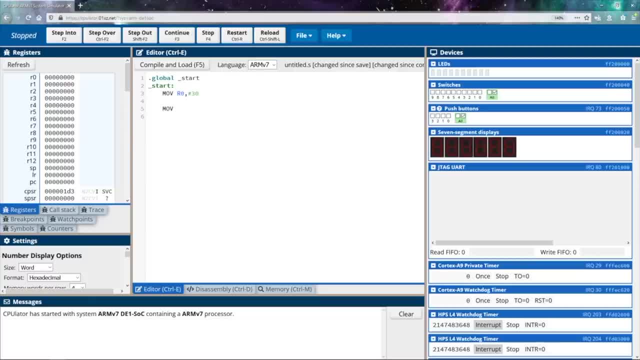 A portion that ends the program. So remember, I said that I wanted to move into register 7 the value 1.. Because 1 indicates that we're going to exit our program. And then I want to do an interrupt. The way I do this is as follows. 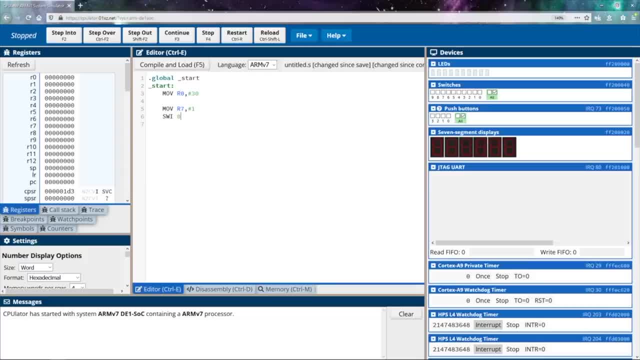 I say swi 0. Swi is a software interrupt. What it does is it interrupts the program And it lets the operating system take over. Like I said before, the operating system then reads the value in R7. That value is 1.. 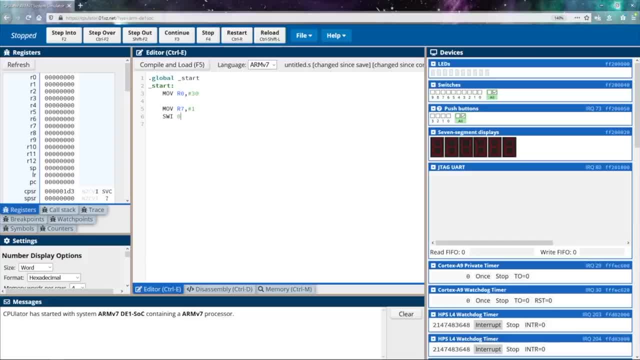 It takes the 1.. It checks the lookup table. It says: OK, well, 1 says that we should terminate the program, And so we're done. So that's really all there is to that. So nice, straightforward, simple. 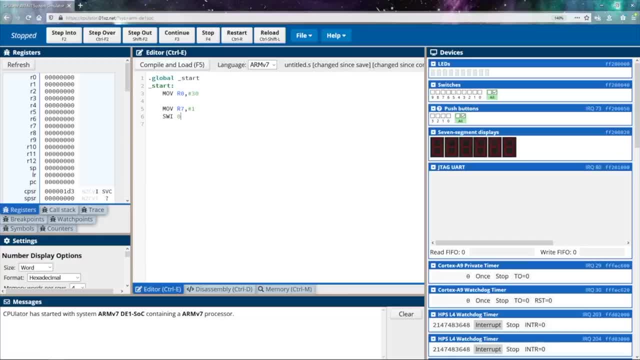 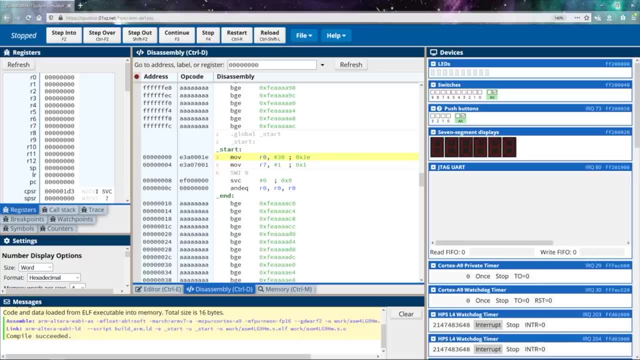 Let's go ahead and compile and run this. So I'm going to click on Compile and Load And, as you can see, it compiles our program together And we are now in our disassembly tab And we could see each of the instructions. 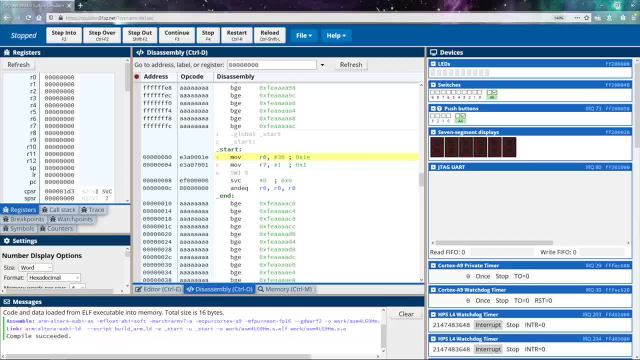 as it interprets them. Now. I will note to you that this emulator doesn't really do well with swi. It doesn't really understand software interrupts all too well. I'm writing this as if you were writing it for an actual ARM processor. 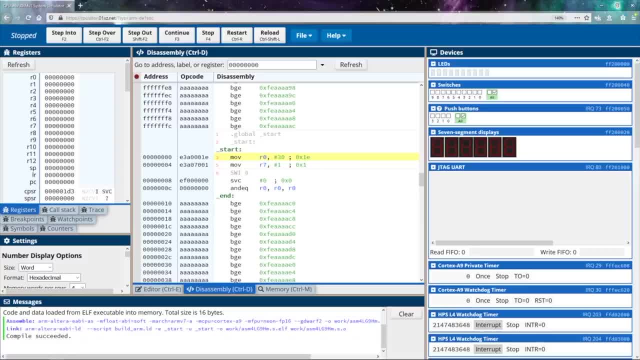 If you're running this on, say, like a Raspberry Pi that runs on ARM, swi is going to be what you're going to use, But our emulator won't end up executing it properly. So that's just a note, just a little quirk of the emulator. 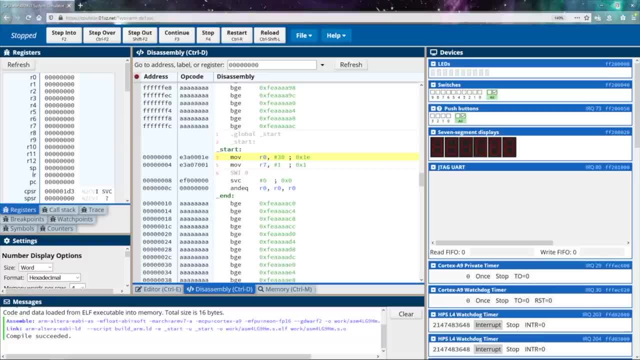 unfortunately, But if you're running on an actual ARM processor, this is what you would end up using, So that's why I'm teaching that instead of something more specific to this emulator. So, So, So, So, So So. 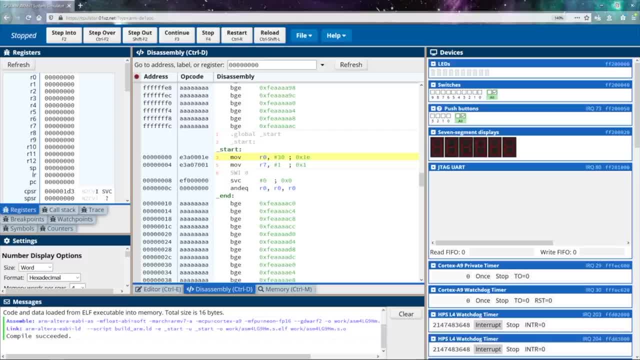 Let's walk through these operations. So remember: the first thing is moving 30 into R0.. If I press Step Into, it will execute that instruction. Now I want to point out a few important things. The first important thing is: you can see that R0 now. 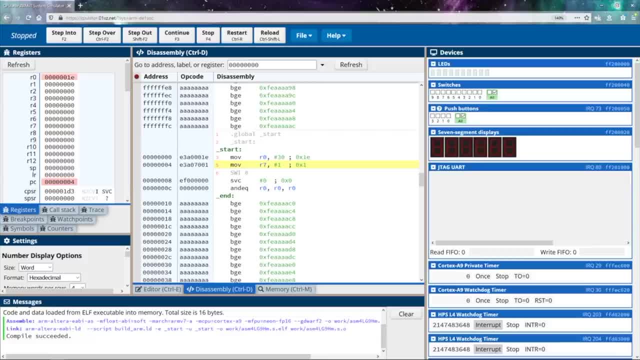 has the value 1E inside of it, which I will tell you is the same as 30 in decimal. If you wanted to verify that, you can actually come down to the settings here. Under Format, you can go to Decimal Unsigned or Decimal Assigned. 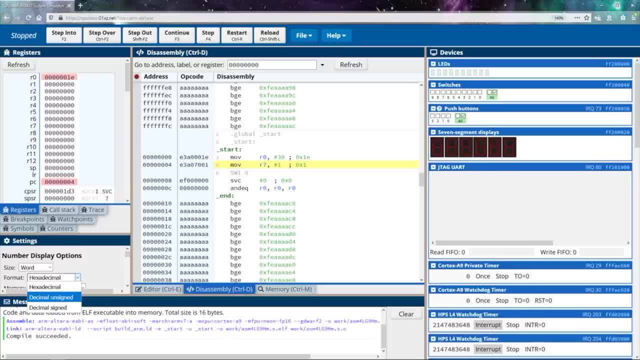 Decimal Assigned assumes that there's negative numbers. Decimal unsigned assumes that everything is positive. So we can go decimal unsigned, since everything is positive. You can see that that gives us a value of 30. So you can see. that's how we convert between, like the hex and the actual decimal value. 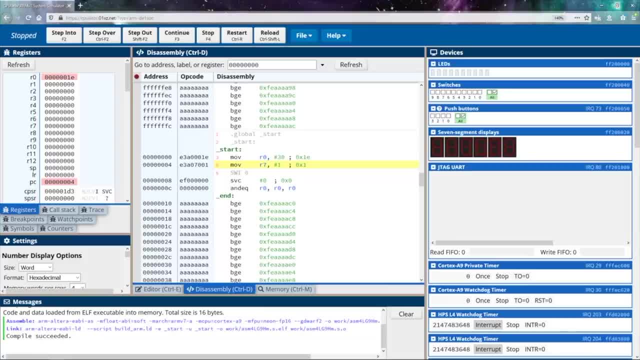 So that's something that we're able to do Now. one additional thing that I want to mention is you can see that we stored one e inside of here. If you're familiar with converting hex to binary, you'll know how to read the binary for this, And you can see that, in general, the most significant. 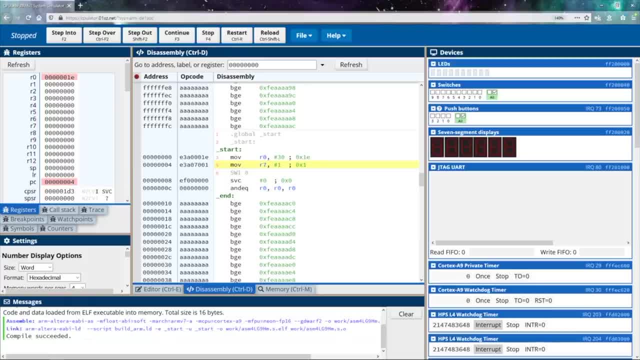 bit is on the left most side. We actually refer to this as a specific type of storage known as a little Indian. So little Indian refers to the most significant bit being on the left hand side. That's the way that arm functions as well as many other processors. But an interesting thing about. 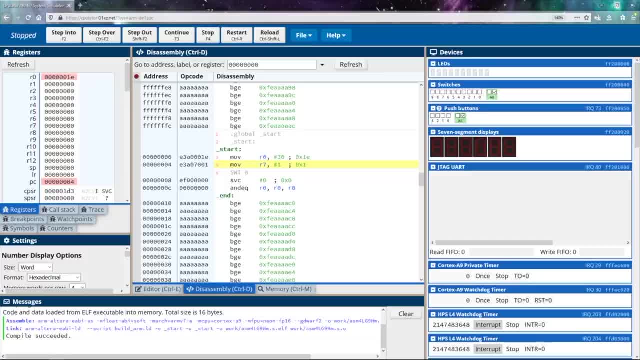 arm is that actually can be used on the opposite way as well. So the most significant bit on the right hand side, which is known as big Indian, we would say that arm is actually a by Indian processor, because we can change where the most significant bit is. 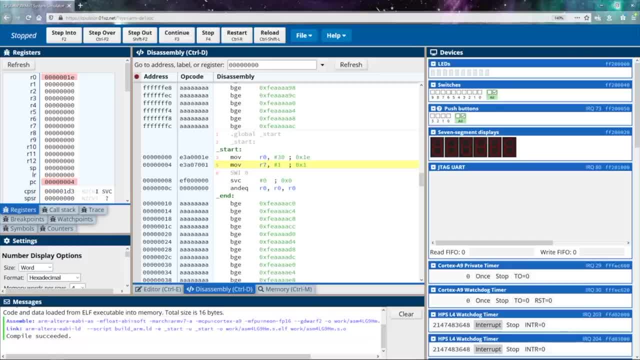 depending on what we're doing. So that's just something that I wanted to note about, like how things are actually being stored in those registers. Then the last thing that I want to point out here is the idea of the program counter. So the program counter is telling us where we're. 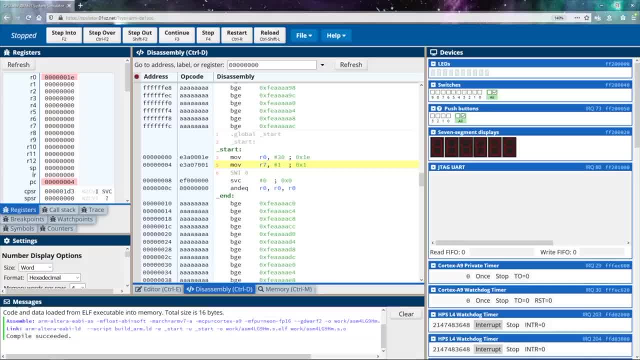 currently located. in terms of instructions, you can see, right now it's equal to four And at address four we have our move for one into our seven. So I just wanted to, you know, pull some attention towards how the program counter was using. That way you can get. 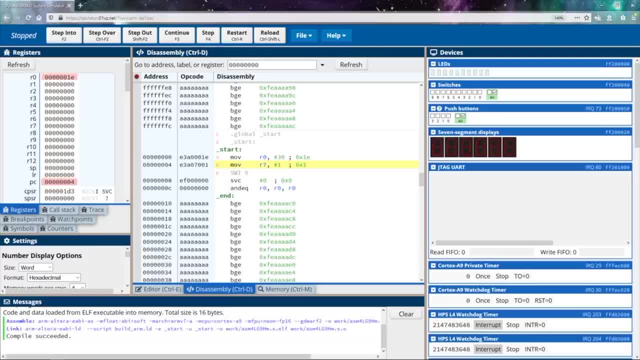 a bit more context compared to the last video where I just told you what it was doing. Now you can actually see it in action. So you can see in our next instruction we step into our seven gets a value of one, and then we would end up doing a system interrupt And that would end our program. 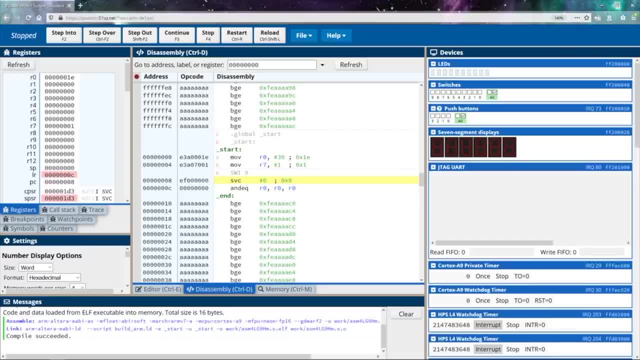 That's really all there is to it. This is a really basic assembly program that we've now written. So you've now gotten the basic fundamentals of writing a program And what the actual architecture is looking like. In the next few videos that I that I put up, I'm going to discuss a little bit about. 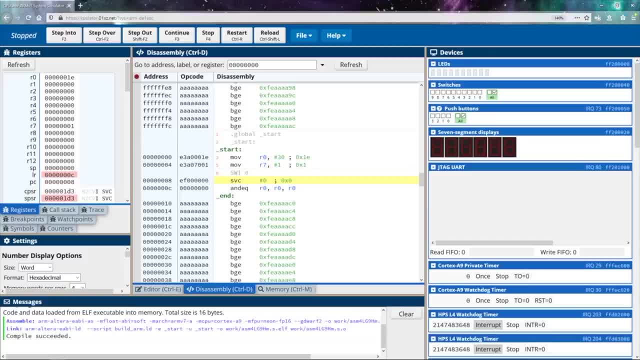 some of the different addressing modes that we have available to us, the different ways that we can move data to and from registers, as well as storing in the stack memory. So we'll discuss a lot more about memory storage And then from there, we can start to take a look at some some more. 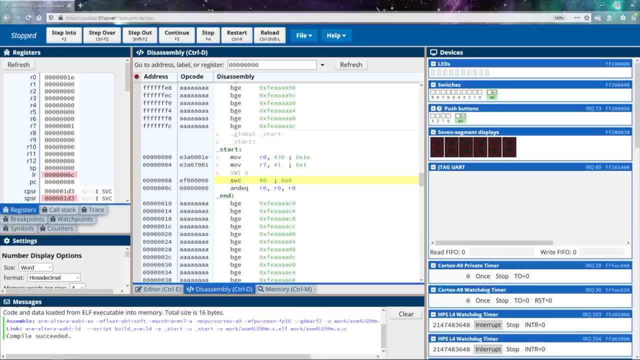 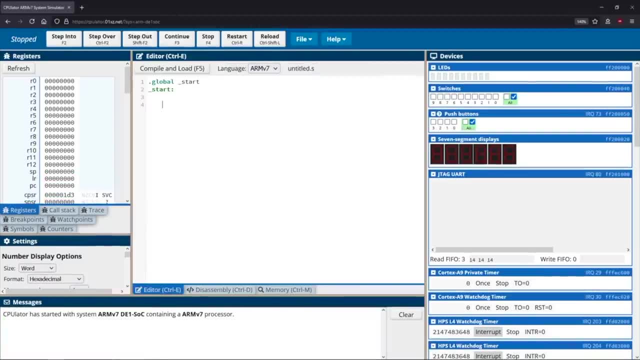 advanced operations and then some actual like algorithms and building some interesting stuff with our processor. So in this video we're going to take a look at the different addressing types that exist inside of arm, as well as other assembly languages, And the general idea of addressing types is that there 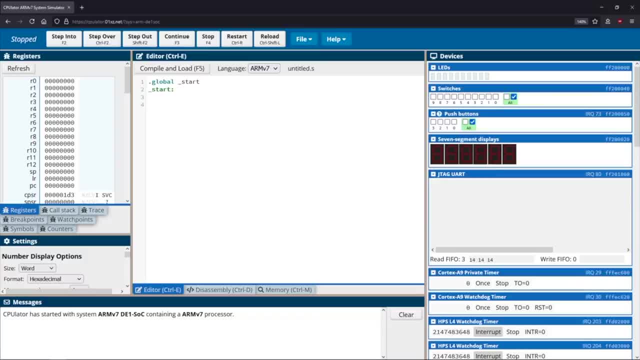 are ways that we're able to store and retrieve data from the various memory locations that we have. So, for example, in the previous video we use the type of addressing that is known as immediate addressing, And that's when we want to move into a register a specific value that is constant. So 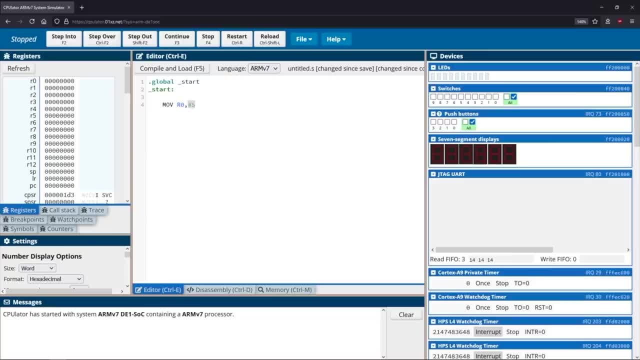 we have like a constant value like this- five on this side- being moved into a register r zero. we call this immediate addressing because we're taking an immediate value and replacing it into a register. A similar type of register type movement that we have is moving between two different 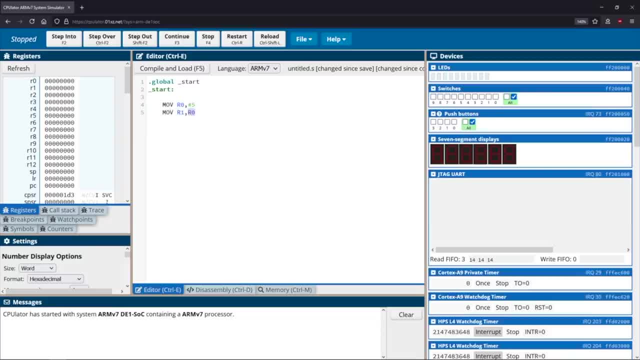 registers. So if I want to move now what's in our zero into our one, this would be called register direct addressing, So we're directly moving a value from one register into another. So those are two types of addressing that we have that work with the register memory, And they're the most common ones. 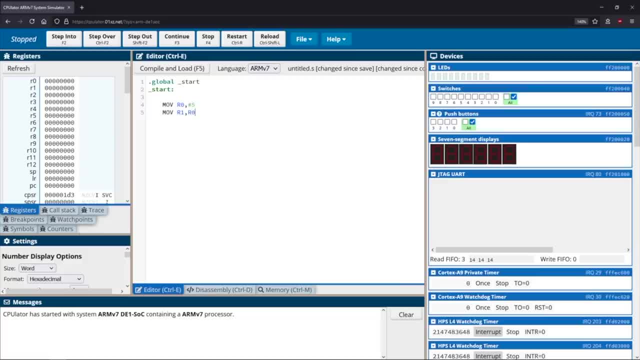 that we'll typically see when we're working with registers. Now, the more interesting type of addressing that we have has to deal with data that's stored in the stack. So to demonstrate this, I'm going to go ahead and show you how to get data onto the stack first, And then we'll take a look. 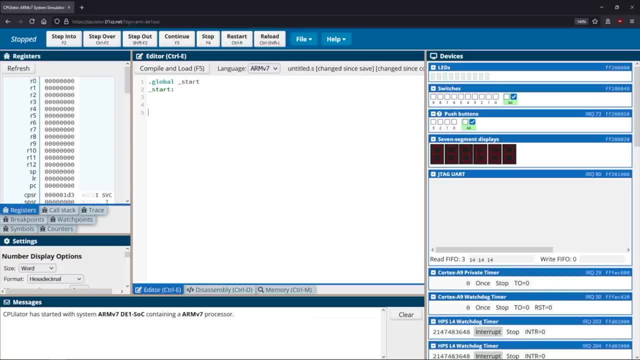 at how we can work with the data that's on the stack. So, first off, how do we get data onto the stack? To do this, we have to use a data section in our application, And the way that we do that is we just type in dot data. this is going to come below all of our like. 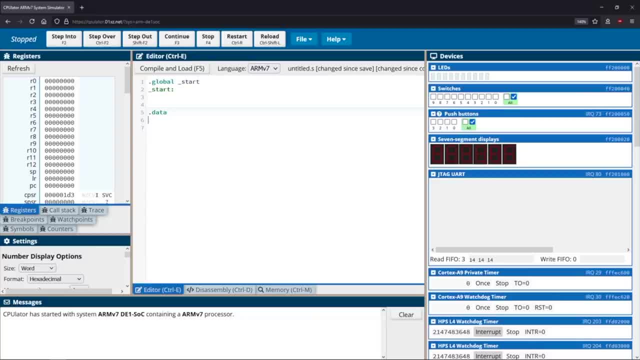 global start portion here. so you say I put it just right down here And what we're going to do is we're going to declare any data that we want to put in our stack memory And we do this in the way of giving it a label which basically functions like a variable name. 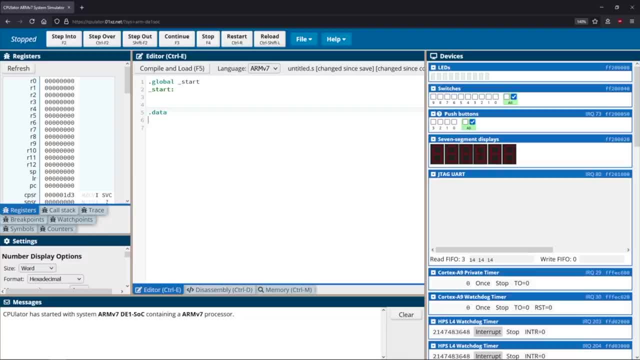 that we then declare the type of the variable and then the data that's actually stored inside of it. So, for example, I'm going to declare some data, I'm going to name the data list, and then you want to name it Azimoth or something, since this is where it is coming from. 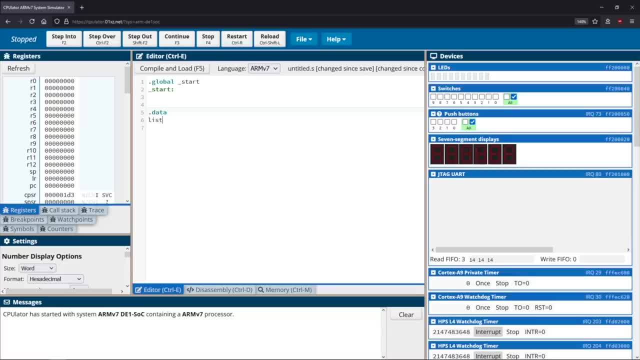 implying to the expected target. So if I wasn't available here, let's say infORMB, there's anOfVariableMuras and if data, I'm going to name the data list. So I'm going to put list colon And then I'm going to 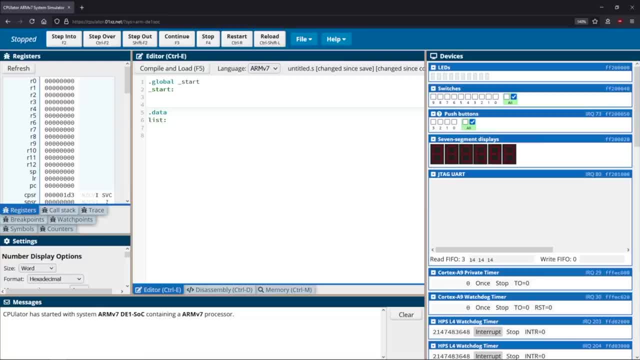 go to the next line And I usually like to indent to put the next portion here, just to organize it nicely, And in this case I want to store a list of numbers. So in this case, when we're dealing with numbers, numbers are going to be a specific size. In this case I want to work with 32 bit. 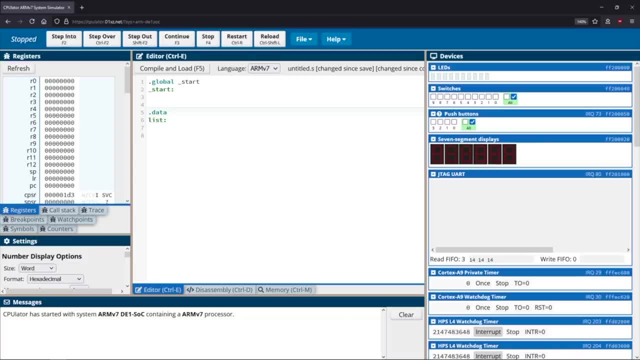 numbers And, as we've discussed, 32 bits is considered to be a word. So I'm going to type in dot word. This tells it that every single one of the values that follows should be treated as a word type, which means that they are 32 bits in size. Notice that we don't say like it's an. 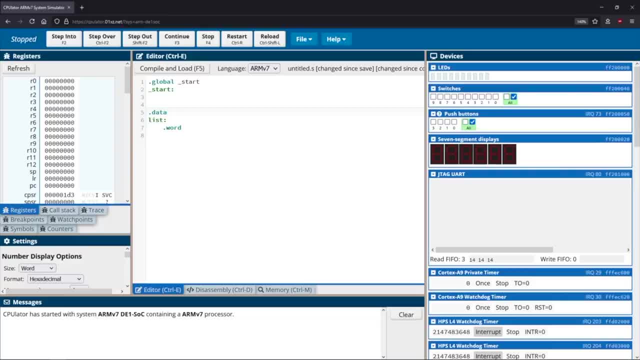 integer or it's a float or anything like that. Assembly is very basic. It's basically just got those, those basic sorts of data types. usually you're going to see things like ask- key or you're going to see things like the actual size, like word or half word or byte or something like that. 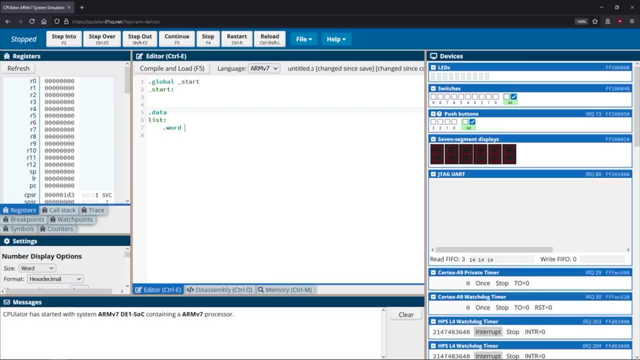 So in this case now we can just start listing off the numbers we want to put inside of our list. So I'll just put some, some random numbers in. it doesn't really matter what numbers you use. I'm putting in some, some positives and some negatives, So you can see the different types that exist. 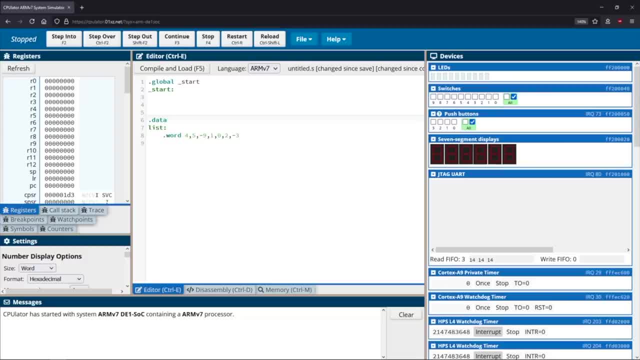 Now the very first thing that I need to do is I need to be able to retrieve where this list is located in memory, And what we do is we typically look for the first entry in the list, And then everything is going to follow sequentially from there, And basically what's going to happen is 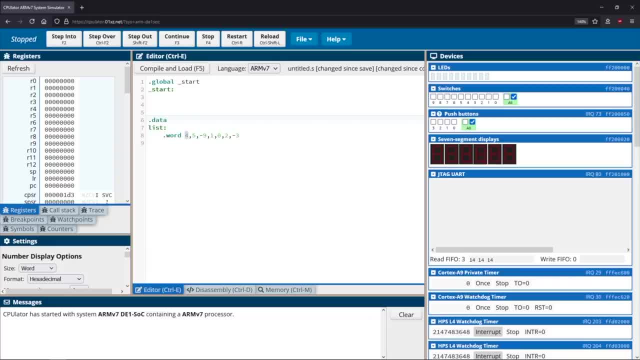 that they're going to appear in every single like slot in memory sequentially. So the first entry is going to be the initial from the first one. So you'll see that when we actually load up this program. So in order to get the first memory location into a register, we want to enter: 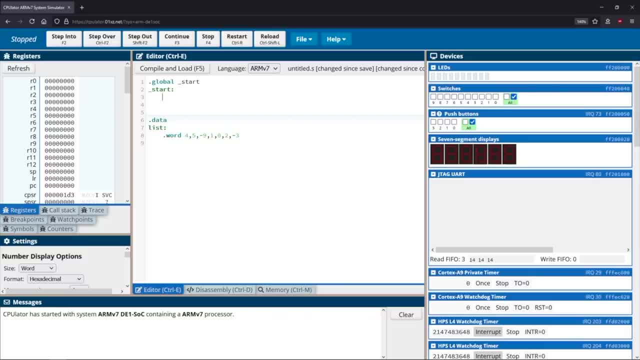 registers that we can actually work with it and manipulate it. it's easier to work in the registers than it is to work in the stack, So we want to get it into the register first, And to do this we're going to use an instruction known as LDR. And what LDR lets us do is it lets us load data from stack. 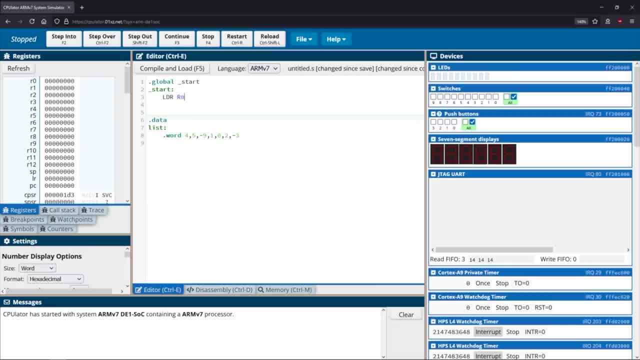 into registers. That's the main purpose of it. So I'm going to load into register r0, the location of the first value in our list variable. So this equals list indicates that I'm dealing with this list in my data section And what it's going to do. 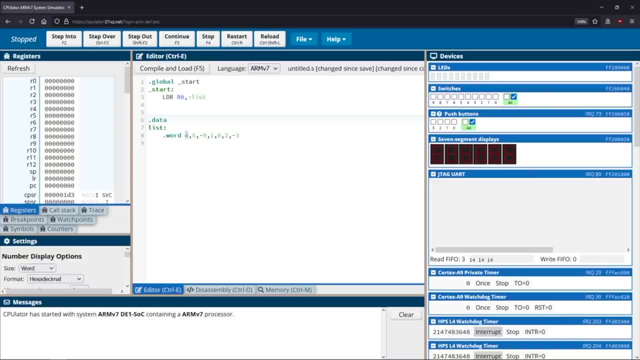 is. it's going to find out where this first value is located And it's going to place it into register zero. This is known as direct addressing, And this is how we essentially initialize the location of our list. So let's compile and load and see what happens. 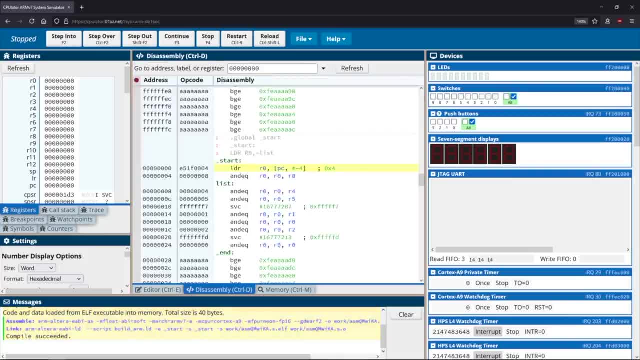 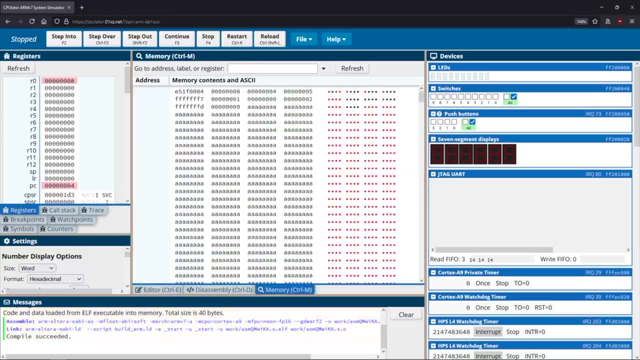 I'm going to go ahead and step into this LDR instruction And we're going to see that it's going to store the value eight into the register r0.. So what does that mean? It means that if I come into memory and I go, 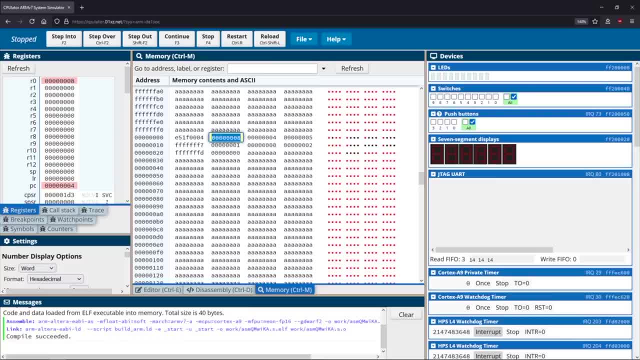 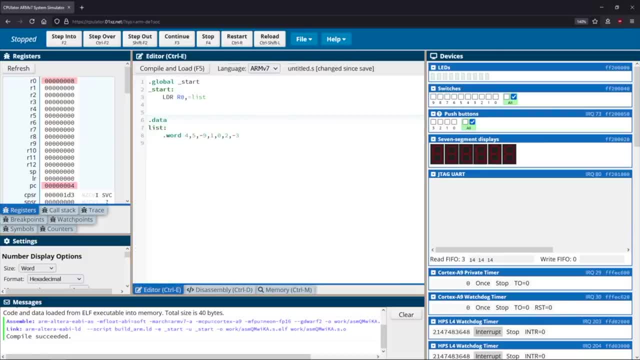 over to memory location eight. so this is zero. this is four, this is eight. right here you can see that this looks like the start of my list. So if we look, we have four or five negative 9102, negative three. 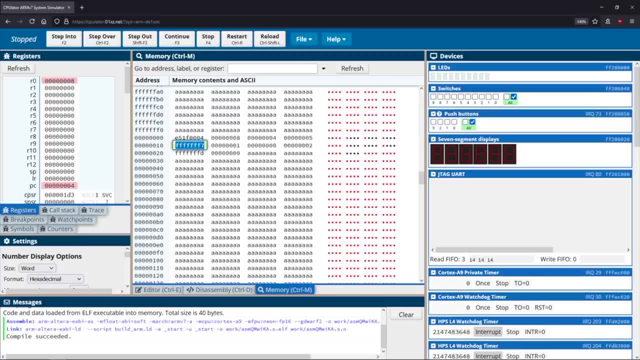 So I've got four or five. this might look a little bit weird. it helps to switch over our list. So if we go to our view here in our settings to decimal signed to see it a bit more clear, you can see that that's. 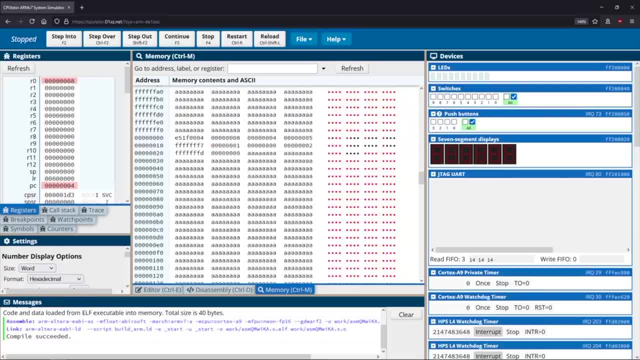 negative nine. Just as a little reminder. the reason why we see it like this is because it's stored in two's complement, right? So we have all the F's, which is all the ones, and then the actual number there, right? 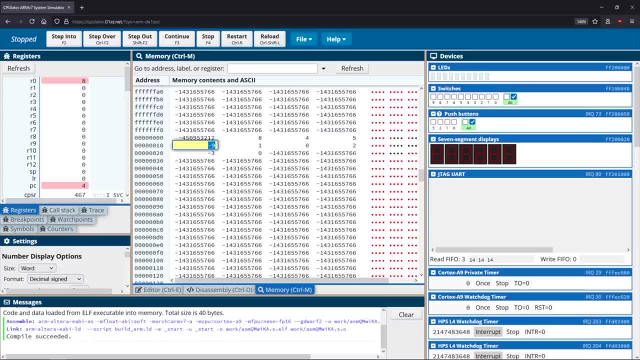 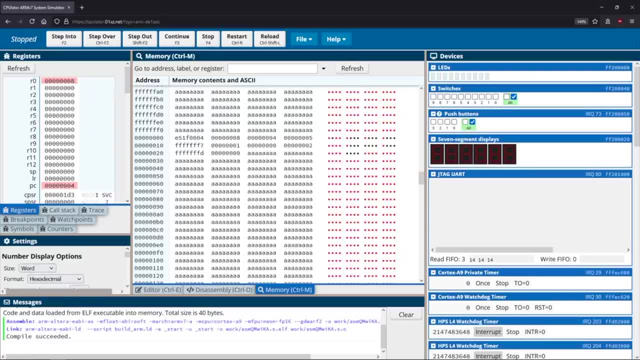 So you can see that that's generally how that's stored, But this helps us see it a little bit more clear, So you can see that these are all the entries inside of our list. So that's. that's nice and easy to look at And 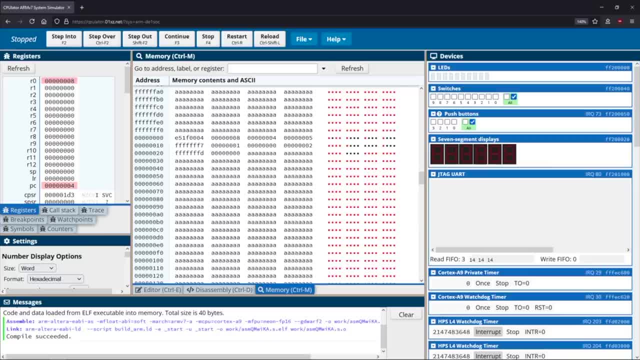 now we actually have the location Of the first value in our list, So that's nice that we have that location. The next question is: well, how do we actually retrieve the value from that location? And the answer is that we have to use another type of addressing. 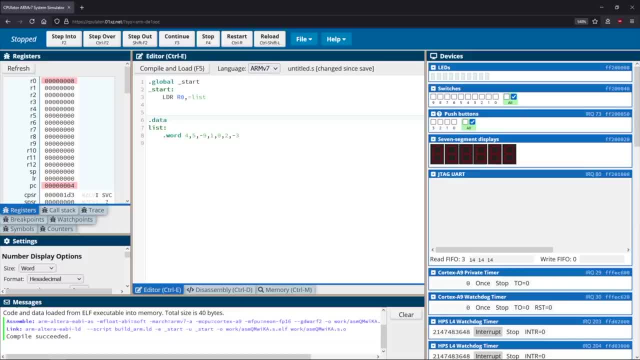 mode, And this one is known as register indirect addressing, And the way that that works is that we still use LDR, because we're moving from the stack into the register, And what I'm going to do in this case is I'm going to load into 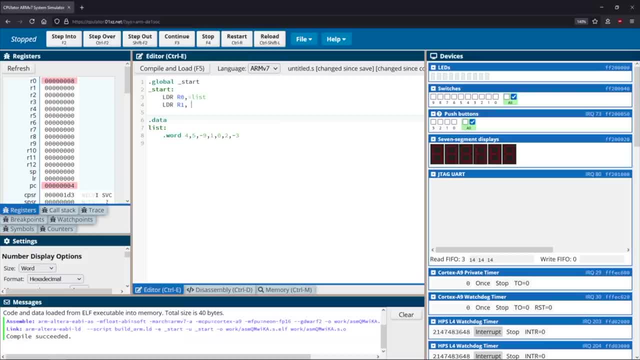 register R one the value that exists at the address of R zero. So these square brackets tell our assembler that we're really looking to find the value associated with the address in R zero. So when we compile and load this, what's going to happen is, in this case, we get 10. 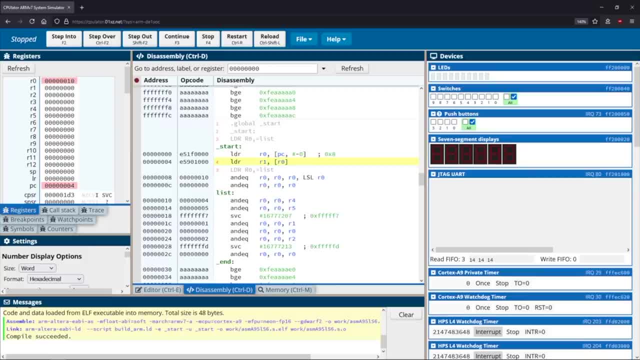 as our value in R zero or one zero. So you can see that it changes every time that I compile and run it. that's totally normal. Every single time that you run it, the memory structure will be slightly different, which is why we sort of have to. 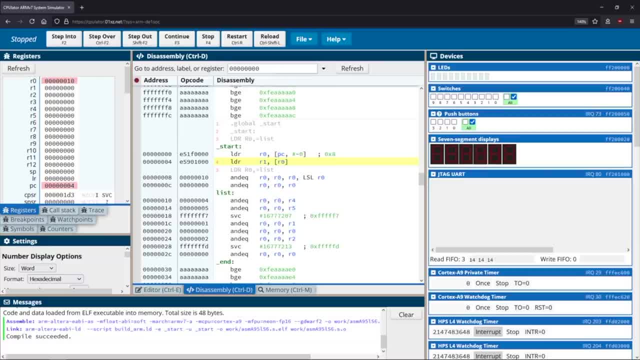 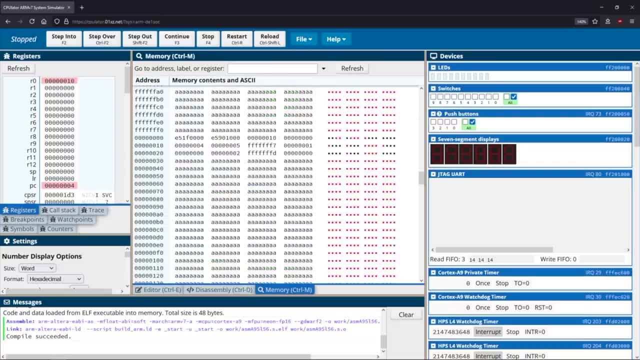 do more dynamic coding, like we're doing, rather than hard coding numbers in such as something to note as well. So you can see that our zero is equal to 10.. We come into memory. we can see that, indeed, 10 does look to be the location of the first element When we do our next. 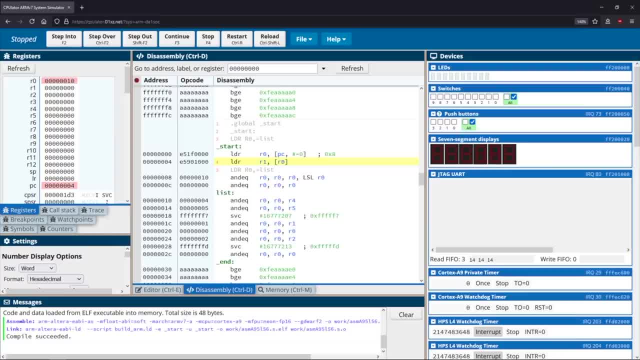 instruction: this LDR R one, and then the square brackets are zero. what it does is it takes a look and it says, Okay, well, in our zero we have this value here. And then what it will say is: they'll say: Okay, let's go to that memory. address what's stored in that memory. 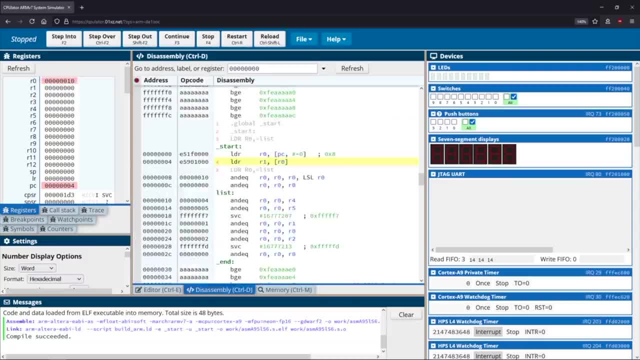 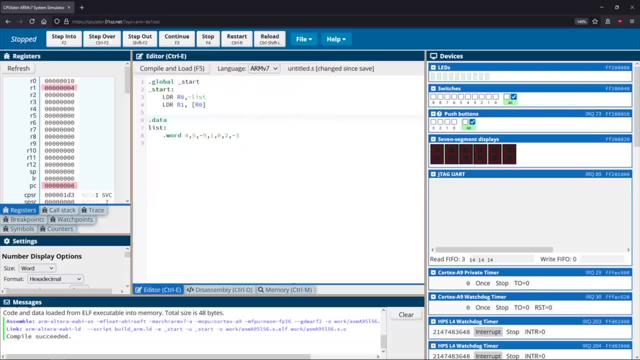 address. okay, four is stored in that memory address, So we'll return that back as our results And you can see that's exactly what we get is four. So just to give you a little bit of an analogy. if you're thinking about, like other programming languages, it always helps to think. 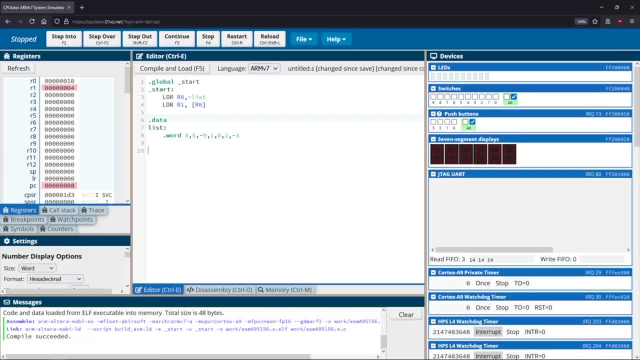 about this sort of like a high level world as well. In a lot of programming languages you might have like a list- you know, I could do like a Python, like list, for instance- and we can have like our different values, like this And what we're doing with this, with this. 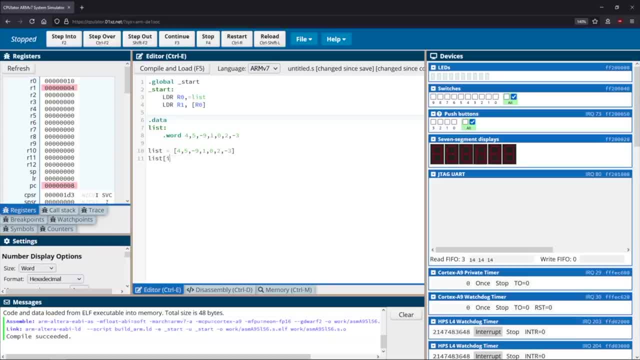 is, we're basically just trying to find the lists value at i where i is r zero, So it's really like the list value at r zero. That's basically what we're looking to do with this. So that's just something to note. Now there are other ways that we can access values off of. 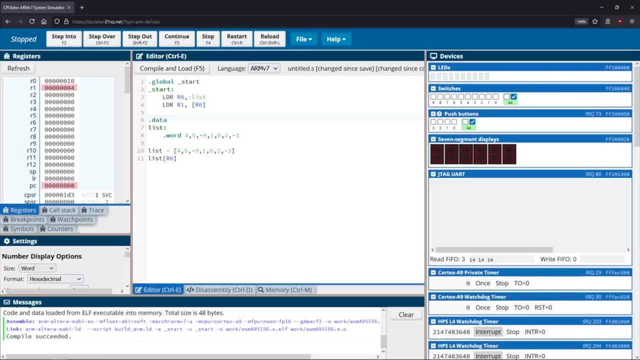 this list. One such way would be to use register indirect with an offset. What an offset does is it starts with the value in r zero, So, for example, in this case it's currently 10.. And then it's going to add some offset to it and then retrieves the value. So, for instance, what I could do is I could add four to it. 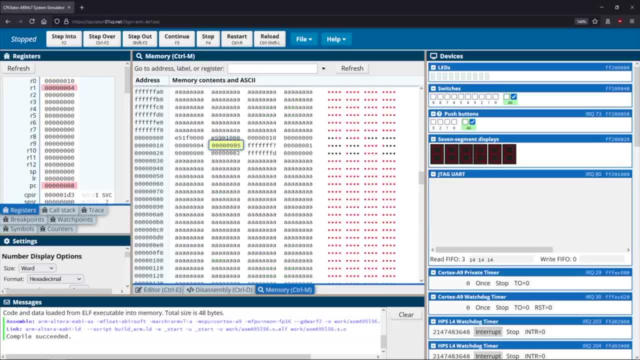 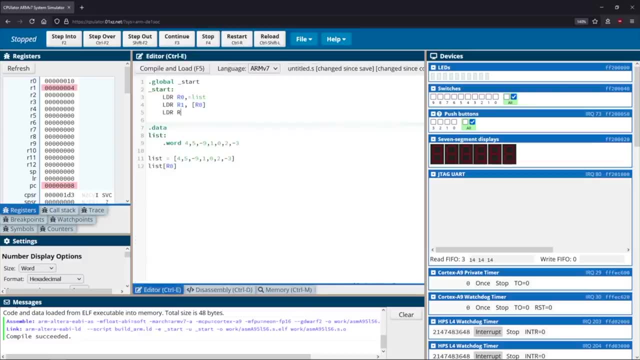 because if I add four to it that would take me to the next location in memory. Remember, this is 10.. This is 14 here, So I can add four to it to get to the next location in memory and retrieve that value. So that would be an example of something that we could do. So let's see how we actually do that. We would do LDR In this case, I'll put it into r two in this case, And we're going to do r zero. 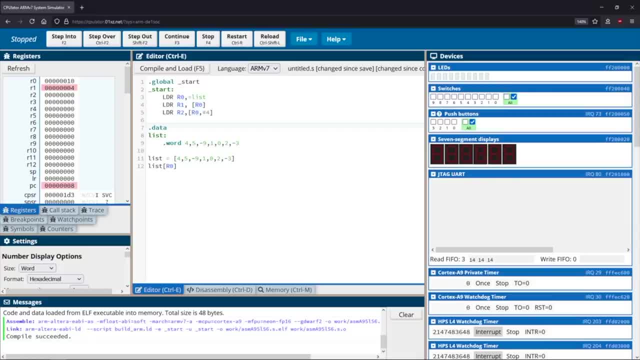 Hashtag four. So what this does is it takes the value in r zero, it adds the form to it and then it retrieves that value. it'd be sort of like doing r zero plus one In the high level context. I do plus one here because we're just moving one index over in the list. 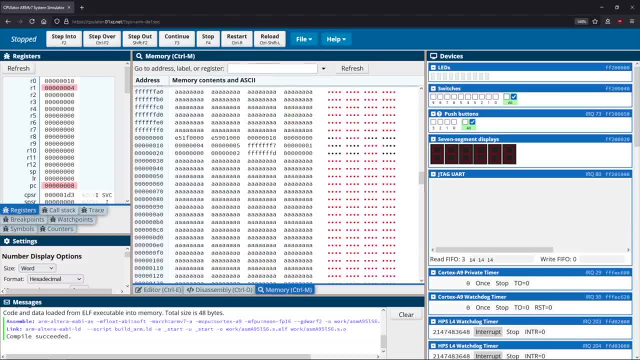 Remember, we're doing four here because we need to add four to this address here in order to end up at this location, which is the location of the next value in memory, so we could add this value to this address here. So this is our next location in memory. 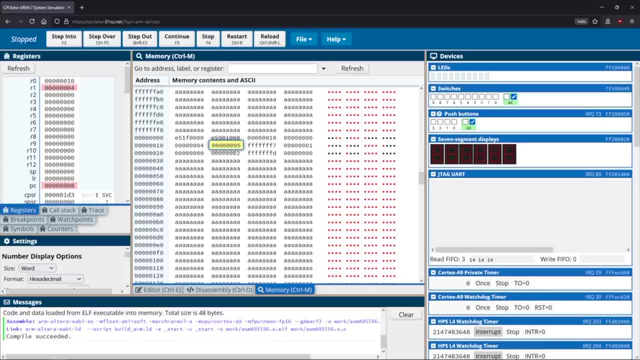 memory. So that's just generally how that ends up working. right, It's foreign hacks for each stock location And of course, we could do other things right, Like we could add eight to get to this, we can add 12 to get to this, and we can keep going like that. 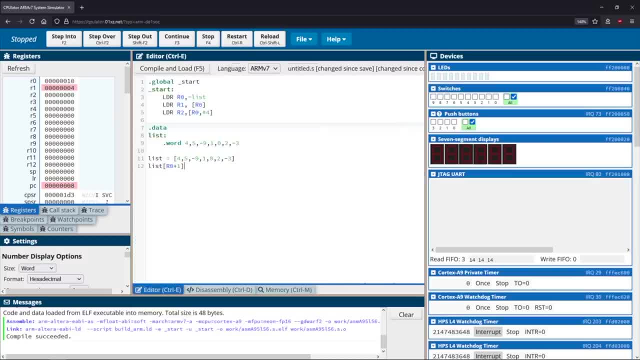 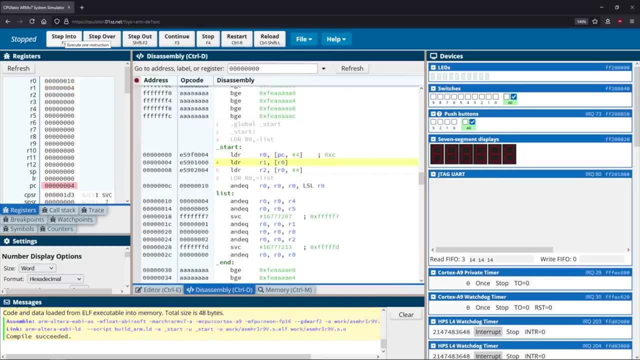 as well. So that's just something to keep in mind with this too, And just to demonstrate to you that this really does work. let's compile and load it And let's step into it. we can see we get 10.. In this case, four is the location of the first memory, And then five is what 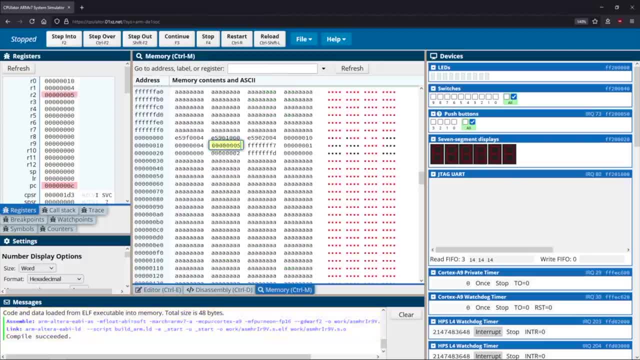 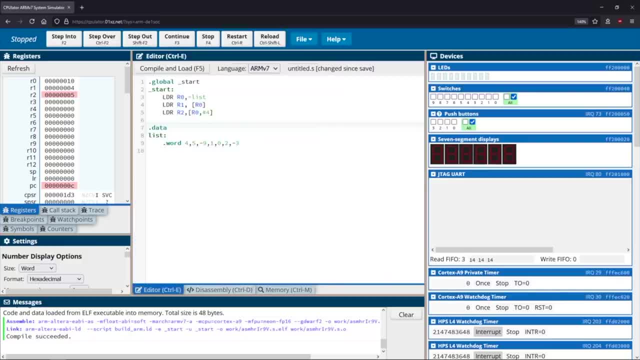 started the second location, And we can confirm that that actually is true. we can see five follows from four, So we can see that that does work the way that I have explained it, which is great. So the last two types of addressing methods that we'll talk about here are known. 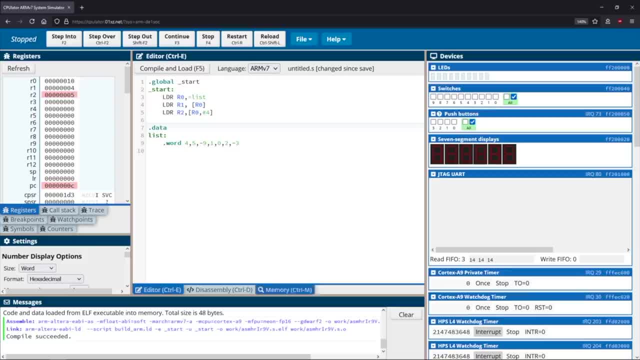 as a pre increment and a post increment. So I said previously that the first one that we have here is the same as doing like list, that are zero plus one With a pre increment. what we would be doing is we would be incrementing our zero. 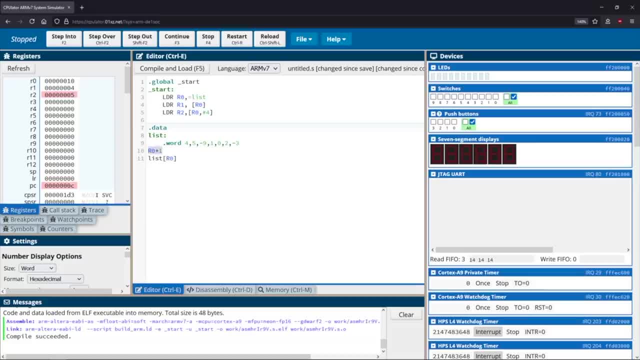 And then we would be accessing the value at r zero. So we essentially increment it and then we check it. So that's the way that a pre increment work: So it increments before it actually gets the value. And the way that this works is we just put an exclamation mark. 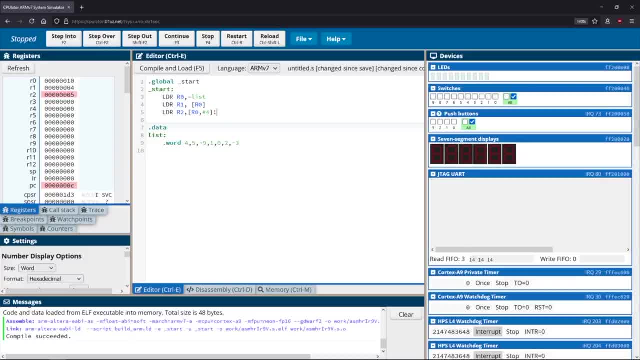 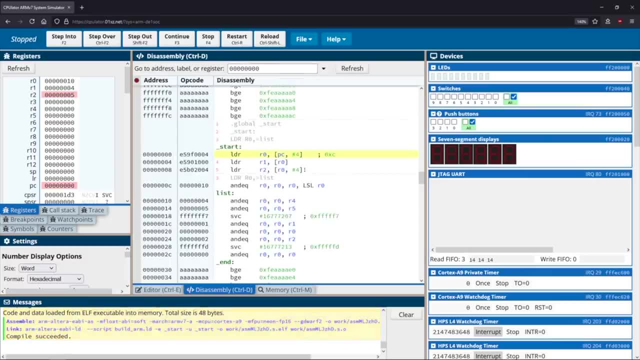 after this. So it's the same sort of syntax. we just put an exclamation mark that indicates that this is a pre increment now. So let's see what ends up happening. When I compile and run this, you can see that I get 10.. Still, four is still in this. 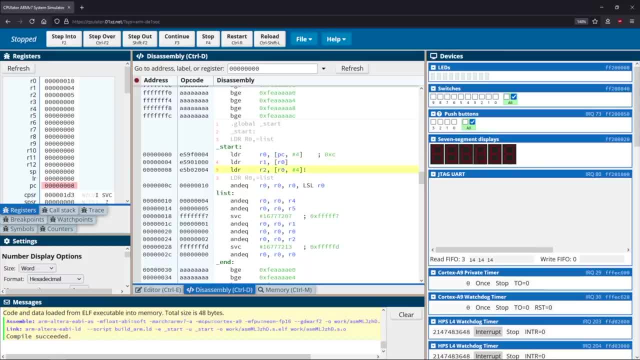 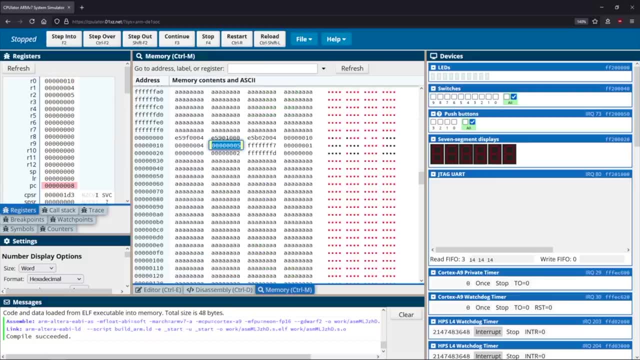 And you can see what's going to happen. is the results going to be the same? we're still going to get five, because it's going to increment this by four, which would take us to location 14.. In location 14, we have the value five. However, something very interesting happens. 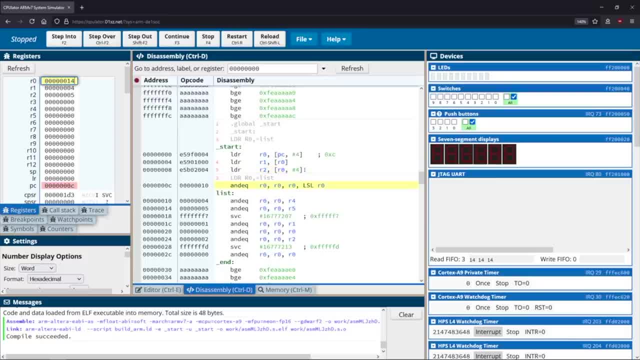 that's different from the previous example And that's that our zero changes to 14 afterwards. In the first example, where we're doing just an offset, our zero didn't change. When we do a pre increment, which has the exclamation mark at the end, it increments our zero and 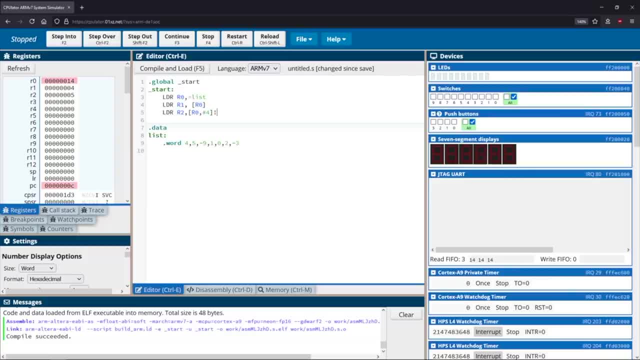 then accesses at that specific location. So that's the way this differs from our offset. And now, finally, we'll talk about our post increment. our post increment is very similar to our pre increment, just difference in when we actually increment the value, right It'd. 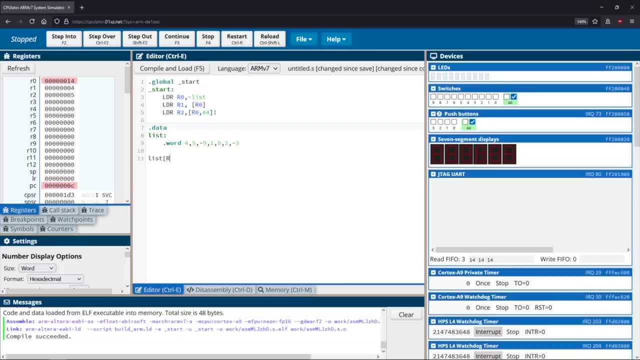 be the same as doing an access to our list- our zero- and then incrementing our zero value when index further, And the way that this is typically written is just like this: we're going to be R zero and then hashtag four like this, So that's generally the way that. 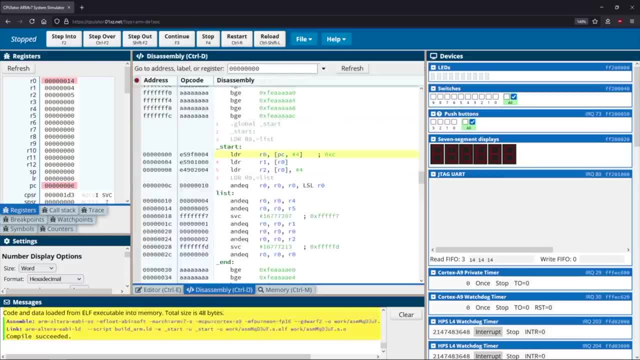 this will end up looking. So let's compile and load that and see what happens, So you can see again. we're at 10 as our starting location. four ends up being our value for R one And then for our two, we end up with the value four and then this increments to: 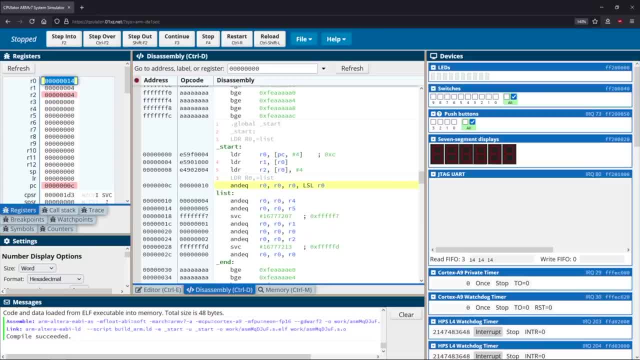 14.. The reason why we got the value four is because, remember, our zero started at the beginning, which is 10. And then, And we ended up accessing at that location, giving us four, and then we incremented afterwards. So, remember, the increment comes afterwards rather than before. 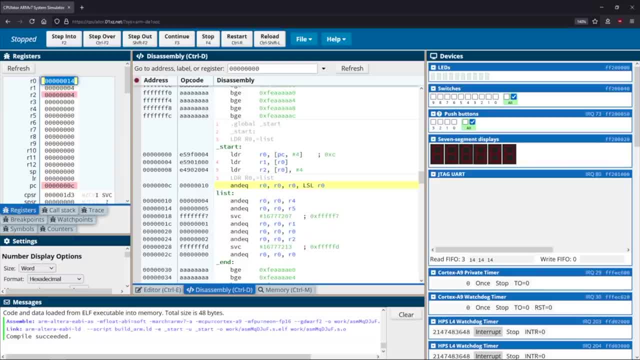 So that's the main thing to keep in mind with that, And that covers all of the different address loading types that we have available to us. So now you should be able to comfortably manipulate data and be able to retrieve from registers and retrieve from stack memory. 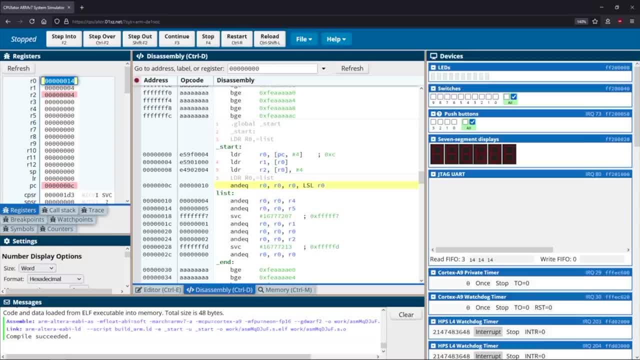 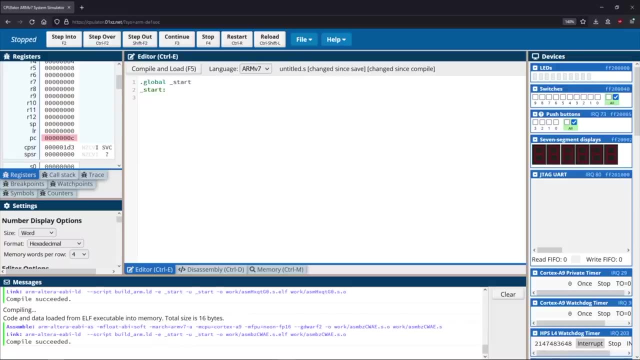 And we'll use this throughout various other videos as we continue on learning arms. So you'll get very familiar with these different addressing types as we work with them, and you'll see a lot of good applications of them as well. In this video, we're going to discuss some of the basic arithmetic operations that exist. 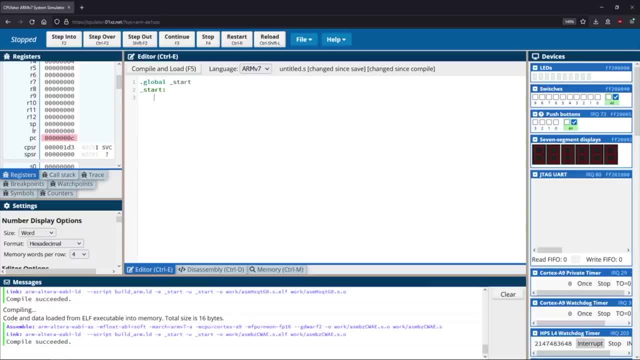 in arm assembly. In addition to discussing these, we're also going to discuss a few different modifications to these instructions that tend to be present in a lot of the instructions in arm assembly, And they allow us to do very interesting things Like setting the CPSR register after the instruction is run. 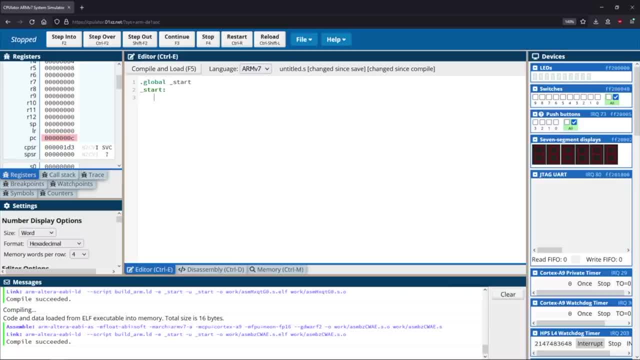 And the reason why we're going to discuss these first with arithmetic instructions is because arithmetic is easy. Everyone sort of knows about adding and subtracting and multiplying, so it's a very easy sort of place for us to work with these instructions. Once we get a basic understanding of these instructions, we'll take on some of the more. 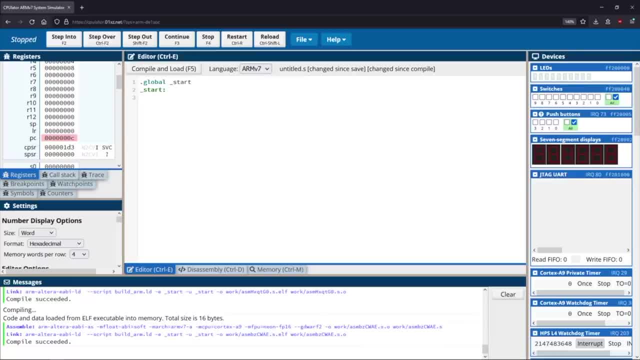 interesting and complex constructions allowing us to be able to discuss these ideas with a solid understanding and foundation already in place. So, to start off with the very basics, we can add, subtract and multiply numbers in arm using a set of instructions. 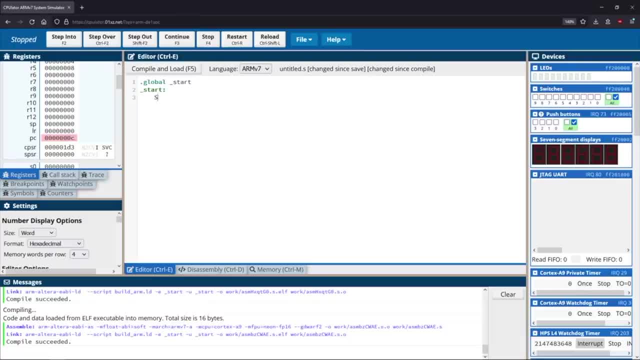 The first is add, the second is subtract and the third is multiply. Now you'll notice that division isn't included in this. Division turns out to be a fair bit more complicated than the other three instructions, so it requires a little bit more finesse to get it working. 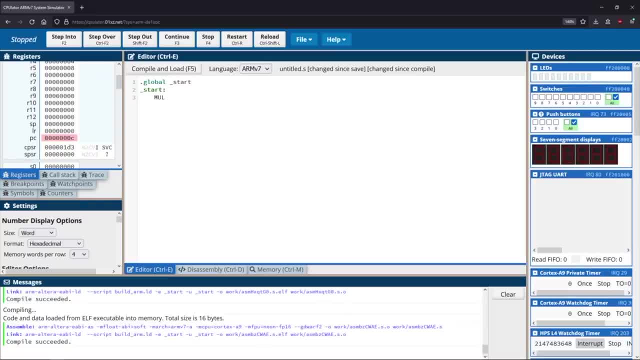 So we aren't going to discuss any division. We'll discuss addition, subtraction and multiplication. So let's get started. So when we want to add two numbers together, for instance, it's fairly straightforward to do. What I'm going to do is I'm going to move some data into some registers. 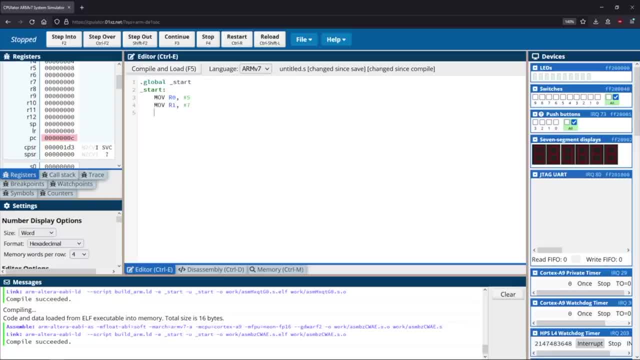 So we'll put some numbers into these registers and then we can use our add operation. Our add operation is going to take in a destination and two sources. So the destination for this is going to be R2, and then I'm going to add together two. 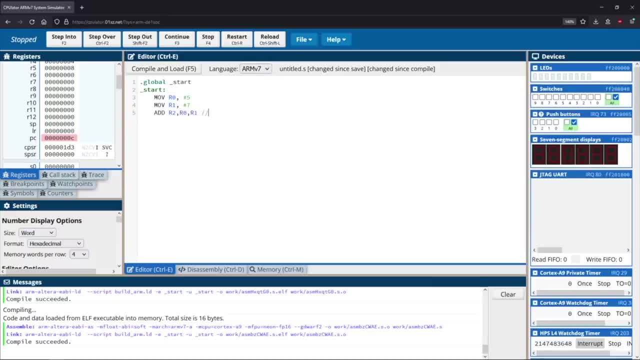 numbers. So I'm going to add together R0 and R1.. And what this is going to do is it's basically going to do this: It's going to put into R2 the result of R0 plus R1.. So that's all this is really going to do for us. 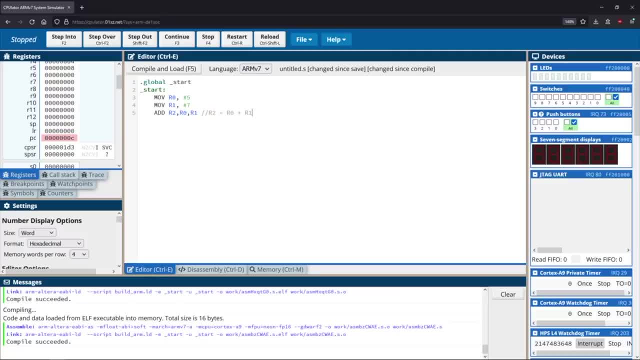 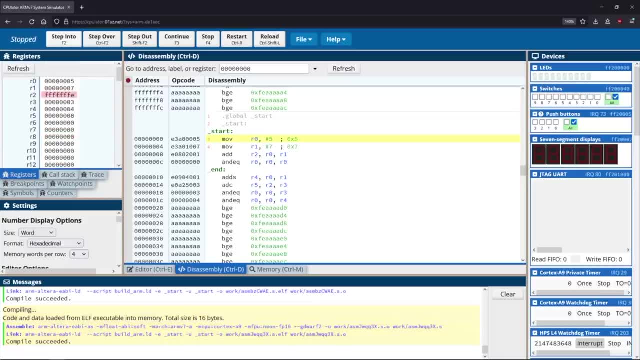 So it's just going to add the two numbers together and store the results in R2.. So that's nice and easy. Let's just take a look at how this works, just to get comfortable with it. So I compile and load. You see, I can load 5 into register 0,, 7 into register 1.. 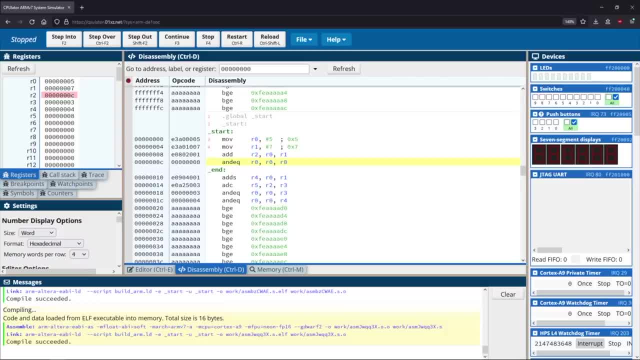 I add those two together and I get C, which is equal to R0.. So that's all this is going to do for us. So I compile and load. You see, I can load 5 into register 0,, 7 into register 1.. 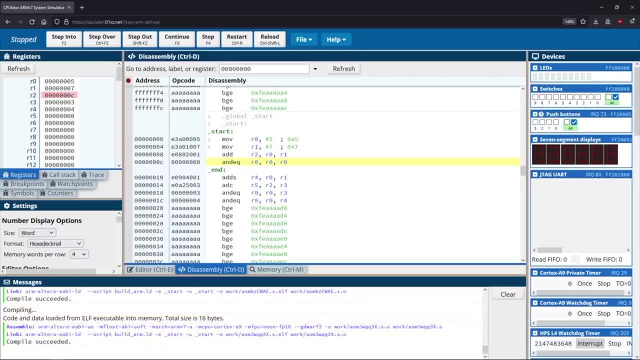 I add those two together and I get C, which is equal to 12.. So 5 plus 7 equals 12.. So we could see that the addition instruction works successfully. So that's the way that addition works for us, And the other instructions work very similarly. 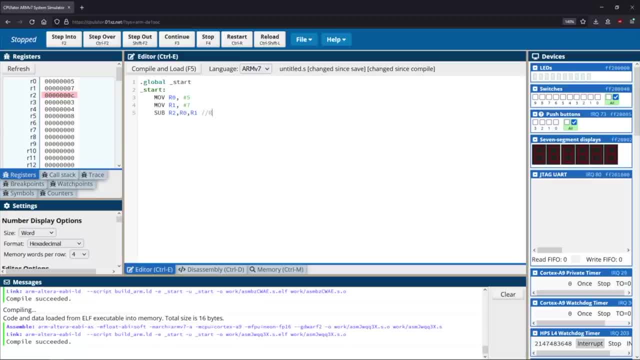 I can change this to sub, And what that will do is it will do the result: R2 equals R0 minus R1. And then we can also do multiply, And what that will do is it will do R0 times R1.. The main thing to keep in mind here is that R0 is always the first operand. 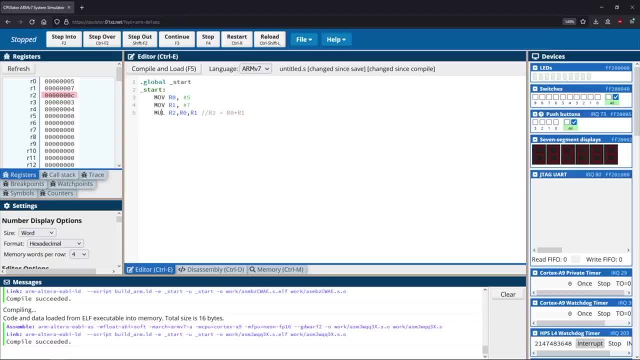 And R1 is always the second operand which only really matters in subtraction In addition to multiplication. the order doesn't really matter, But in subtraction it does, And you can see that when we take 5 and subtract it from 7 in this example here, we would clearly 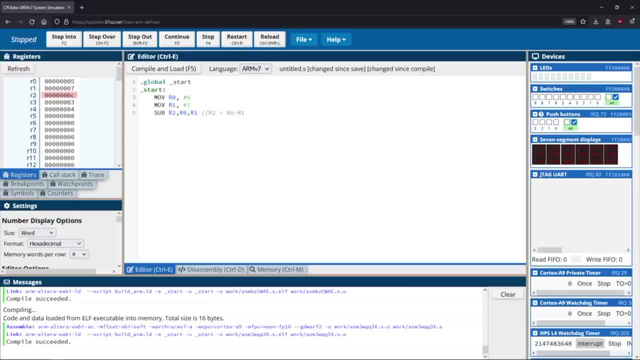 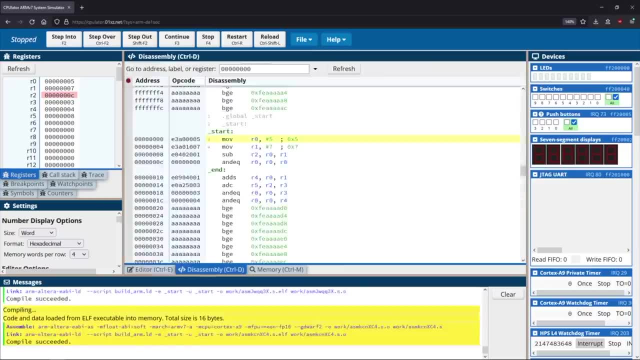 get a negative number. We'd get negative 2 as our result, And that's where the interesting ideas start to come in with our arithmetic operations. So if I were to do this right now, we can see that I get 5 and 7.. 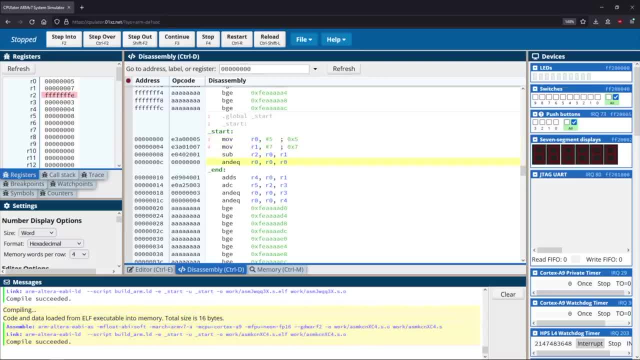 And when I subtract them I get this big number here or this big looking number here. And when I convert this to decimal signed, you can see I get negative 2, right, But if we're looking at it in hexadecimal it isn't really necessarily clear. 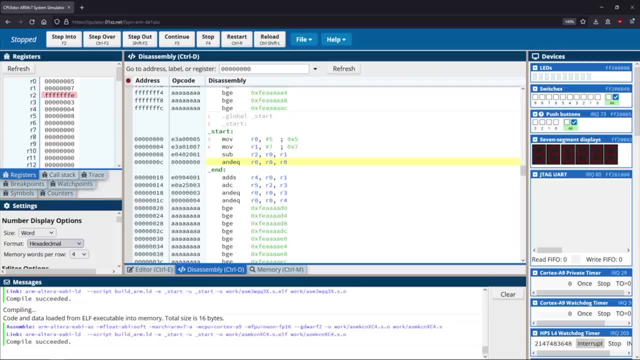 Because the reason why it's not necessarily clear is because we could have had a very large number in R0 and maybe a small number in R1. And when I subtract them, I would get potentially this very large number here. So the question is: is this a very large number or is it a negative number? 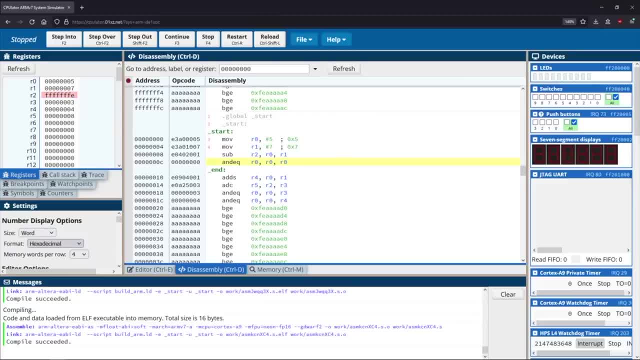 There's some overlap there, right? Because of the way that we store negative numbers in assembly, we don't necessarily know right off the bat if this is a negative number. I mean, I clearly know now because I put in 5 and 7 and I know that subtracting those 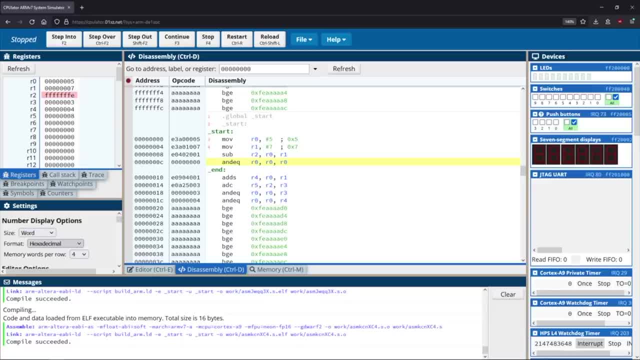 two gives me a negative number. But think for a minute: if we had, say, a user input and we subtracted two numbers that the user gave us, How do we know if they gave us a very large number or a negative number? right, 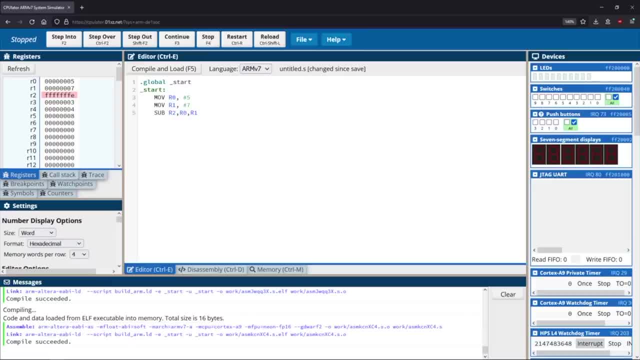 How do we know the difference between those? And just to sort of maybe drive this point home, I'll just show you what I mean by. it could have been a very large number If I were to put this as a hex right. so I can say, let's say, 1,, 2,, 3,, 4,, 5,, 6,, 7,, 8.. 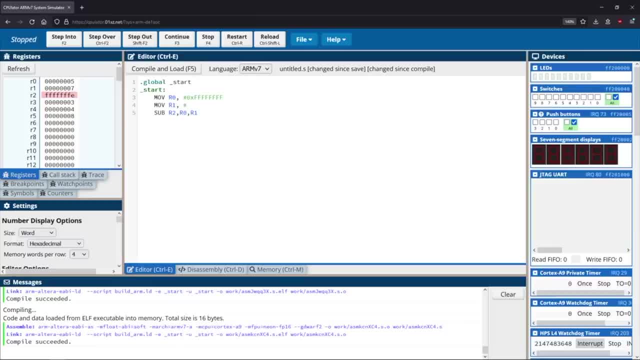 So we'll do all Fs like that, And then I would have to subtract 1 from that right And we'll just change around this ordering so that it's the first one. Well, actually, no, we can keep it like that, because we want to do R0 minus R1.. 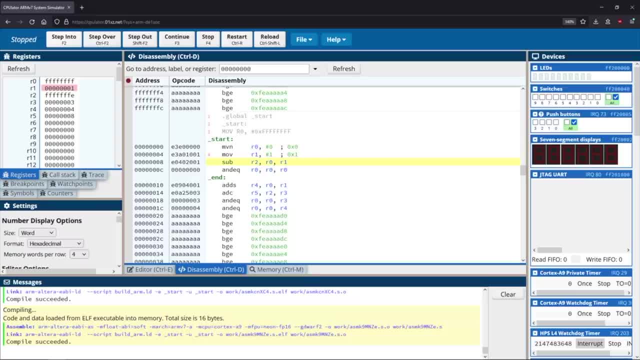 So what I mean by it could have been a large number is when I have this result here and I subtract it from this number here, you see the result is the exact same. right, We get this all Fs and then the E at the end. 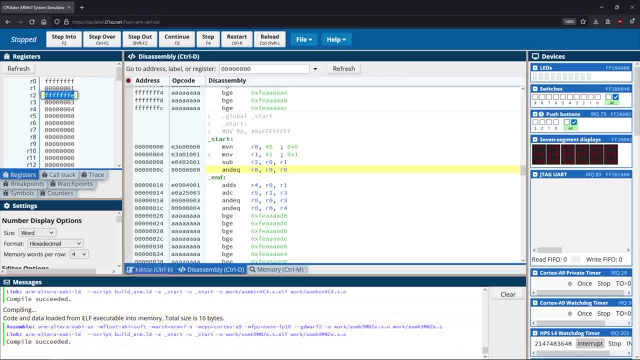 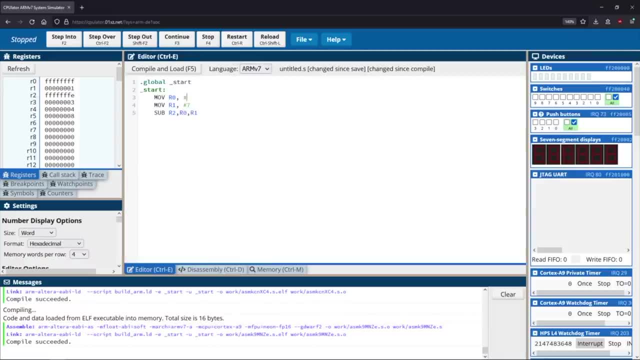 So you can see, if I take this big number and subtract 1 from it, I get this. But also if I take 5 and I subtract it from 7, like we did before, we get the same results. So this is why there's the question of: well, is it a negative number or is it a very large? 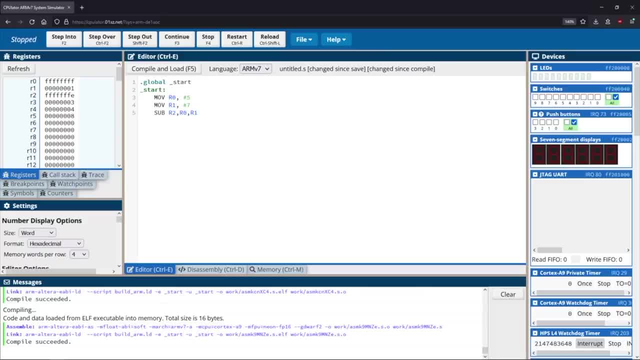 number subtracted from a very small number, And the way that we solve this problem is using the CPSR register, Which is this register right here. You'll notice some of these letters along here: the N, the Z, the C, V, I, all these. 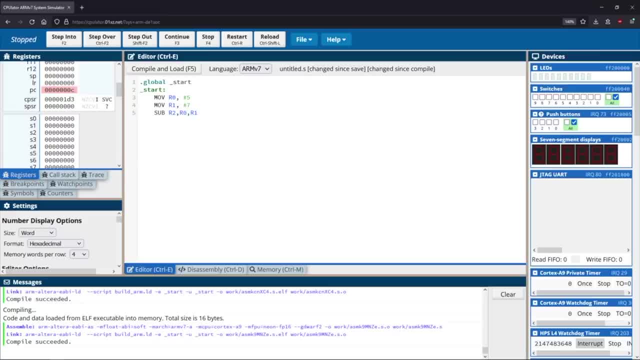 sort of letters. Each of these indicate a specific flag that is set in this register. The N, for instance, stands for negative, So it will tell you if the result of the last operation was a negative number. And that's exactly what we want, right. 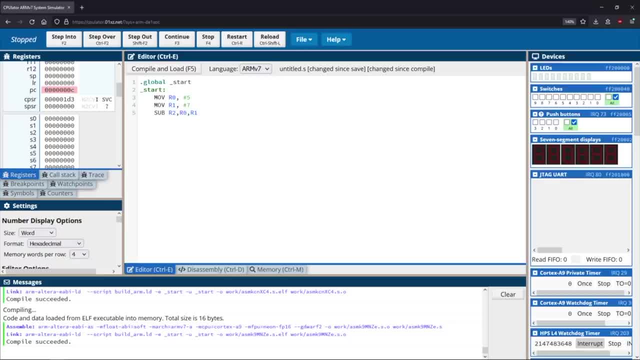 We want to set that flag so that we can understand that this result is negative. And I could do other things It can take care of if there was a carry in the operation, if there was an overflow, if the result was zero and that sort of idea there. 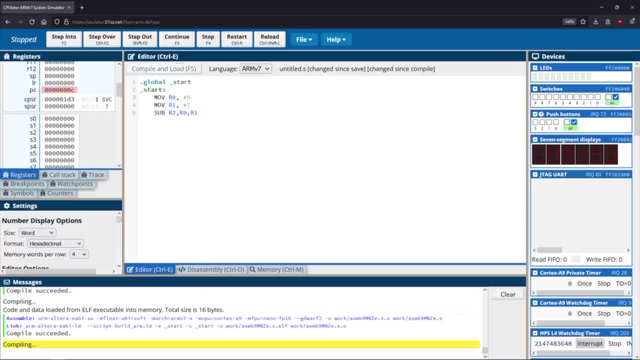 So how do we get that to actually set? Because, if you notice, when I compile and load this and I step through these instructions, nothing happens to the CPSR register. The answer is that we have to use a special type of instruction, called a in this case. 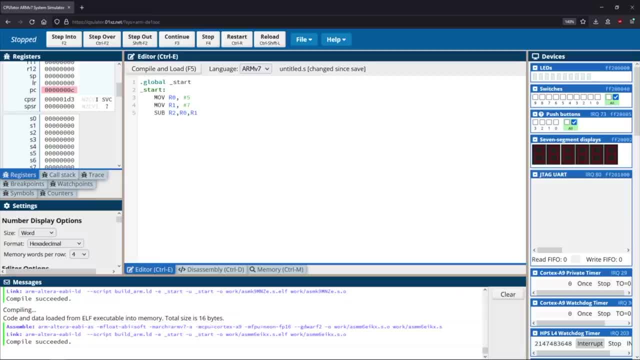 I'll call it an arithmetic with flags, And the way that it's represented is: we just add an S to the end of the register. So we're going to add an S to the end of our instructions. so sub S in this case. 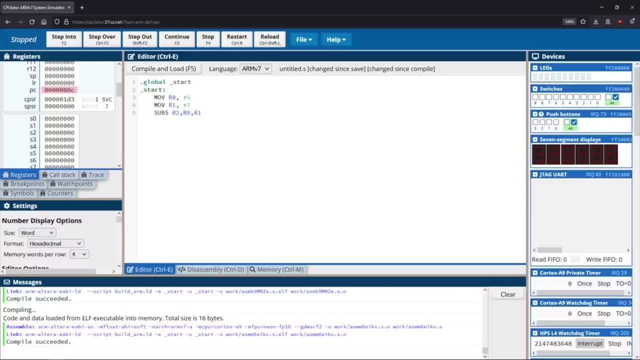 So sub S is going to set the flags in the CPSR register. And you might be thinking: well, why doesn't it just always do this? Why doesn't the subtraction operation just always set the CPSR register? And the answer is because to set the CPSR register requires at least one additional. 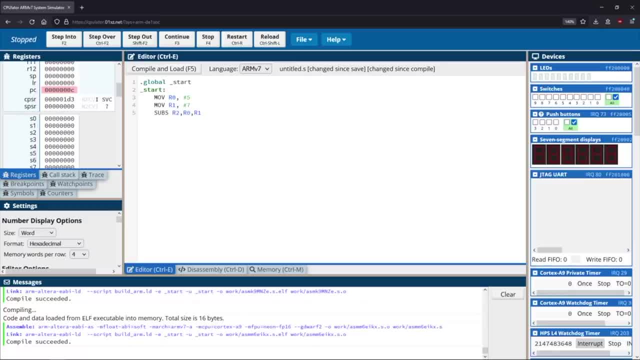 operation right, It requires us to actually load data into that register And that, you know, adds a little bit of overhead to the operation. If we don't need to do that, then we shouldn't, So that's why there's two separate instructions for this, because one of them is slightly 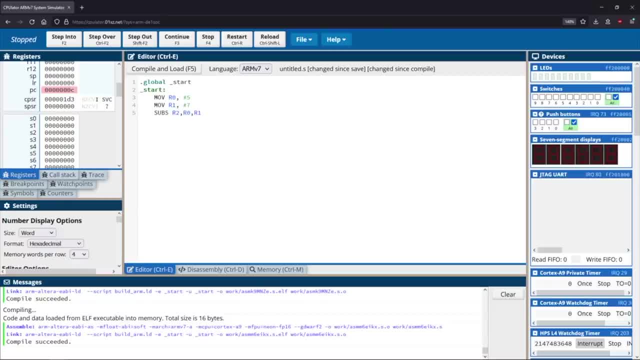 more efficient than the other, And slight efficiencies do matter when you're programming at such a low level. So then, the second question that you might ask is: well, when should I use sub S over sub? And the answer is: you should use sub S if one. you know that there's going to be negative. 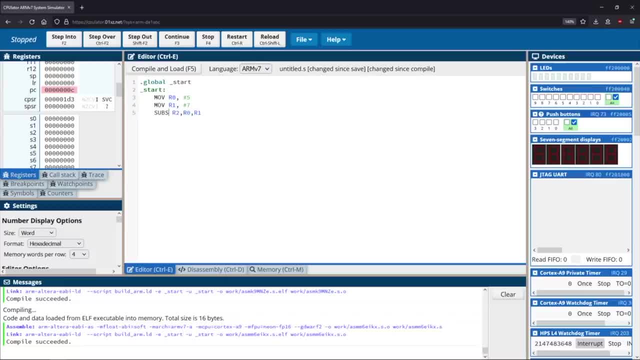 numbers or two. you don't know what the values that are going to be subtracted are. That means you're loading them from some location that you don't have. You don't have control over If you're just taking two constant numbers and subtracting them from each other and 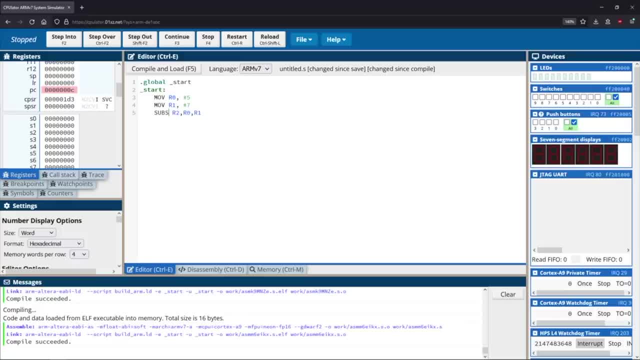 you know what the result is going to be, then you can use. you know whatever instruction is appropriate. If it's going to be positive, just use sub, that's okay. If you don't know, then you should use sub S So you can check to see if it's positive. 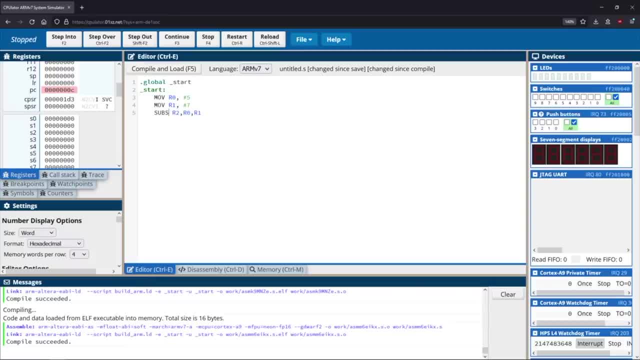 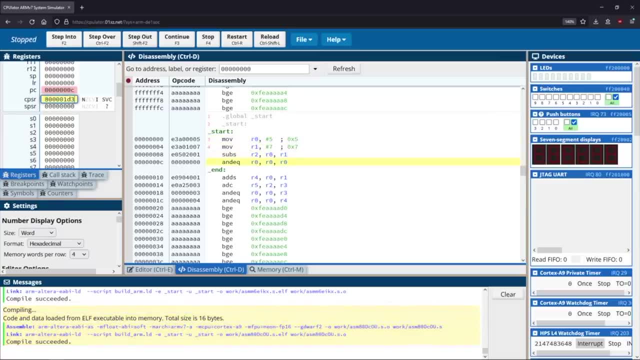 or negative. So just to demonstrate what this ends up doing when I compile and load this: like I said before, when we do this now, you see that this CPSR register has changed and you can see that It is now bolded. that means that it has identified that the result was a negative number, rather. 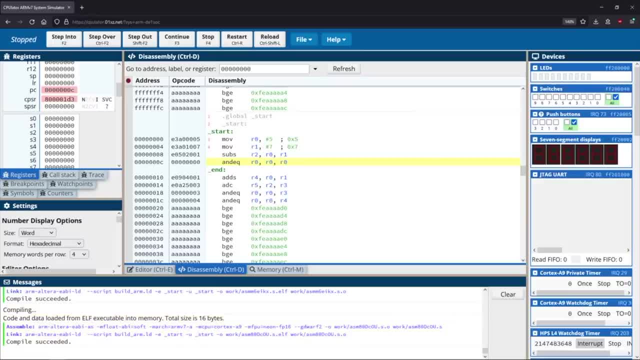 than a positive one, And that's exactly what we were looking for. Now, just to note, the reason why this bit is set to eight is because so each of the four bits at the beginning of the CPSR register stands for one of the flags. 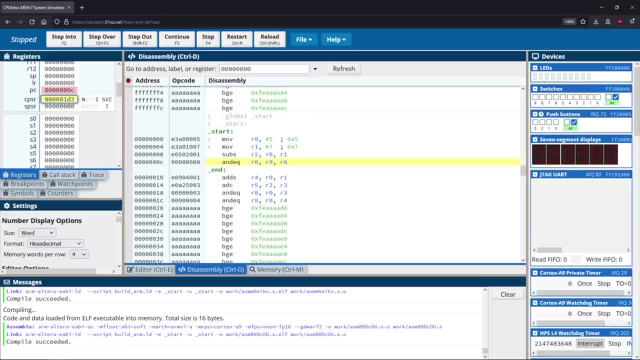 And that's the same with every bit. every single bit is one of the flags, So since it's set to 1000, that means the negative is set to one, which means that it was negative. And then I think that the other four, or the other three zeros are the zero the carry. 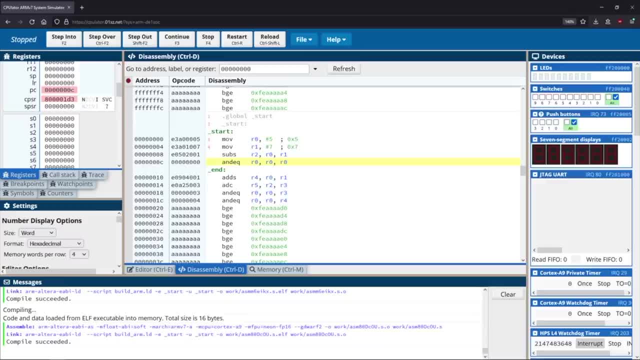 and the overflow, which are all set to zero, And that's why they're grayed out here. So that's the way that those flags are actually set. So if you're not working in an emulator, you'll just see that set as eight rather than seeing 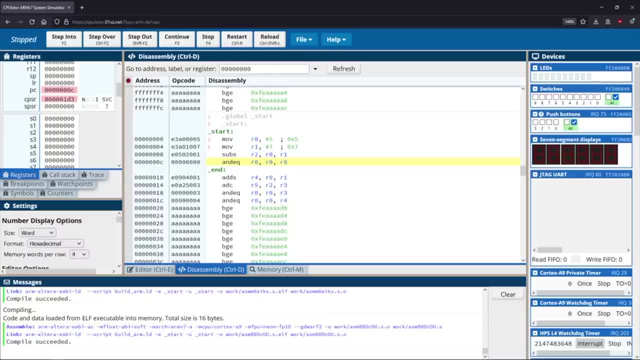 the end highlighted. The end being highlighted is nice for when you're learning, because obviously that tells you: hey, it's a negative number. But if you're doing this just like on, like a Linux system or something like that, you won't see that, you'll just see the eight instead. 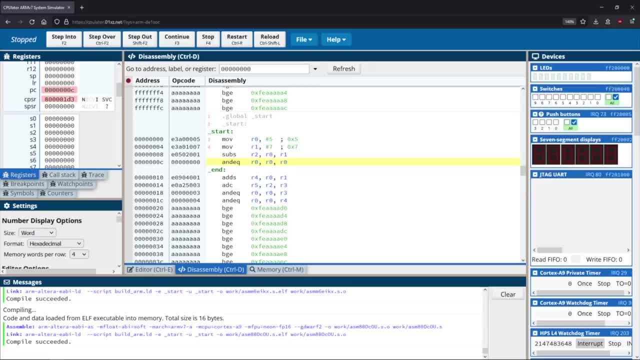 So it's it's good to understand Exactly what that's doing as well. So that would be the idea of our arithmetic operations. Now there's one other additional arithmetic operation that is quite helpful for us, And it's the fact that when we add two numbers together, in some instances you might end. 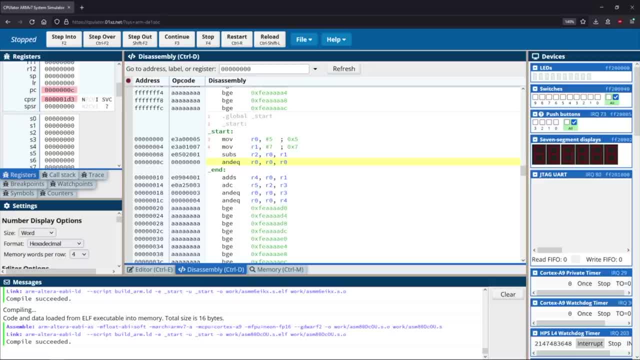 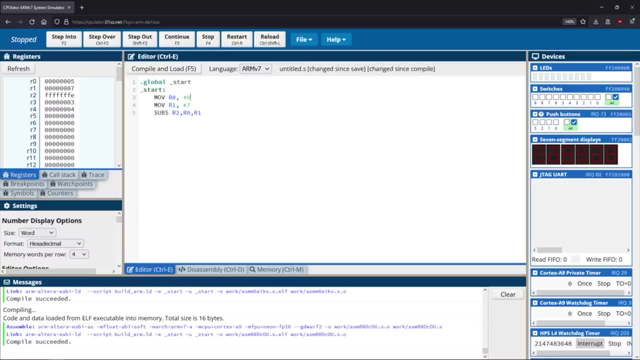 up with a carry And basically what that means is that the number was way too big to actually be stored inside of a single register. So, to give you an example, If you have, like you know, something like this and you want to add it to, maybe something like this, right? so 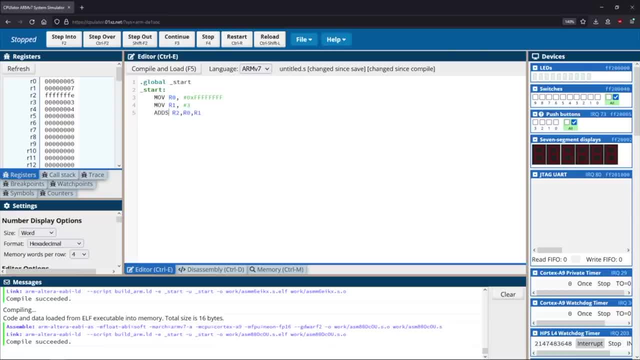 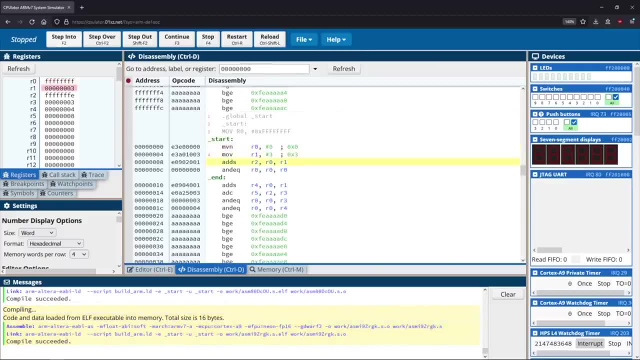 we'll just say: we'll add this. And this is another example where you would want to use something that actually sets the flags. And the reason being is because when you do this addition, you'll notice that when you add these numbers together it's far too big to actually be stored in one register, because 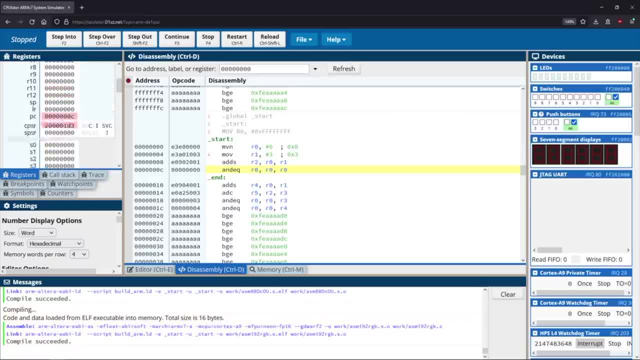 it overflows beyond 32 bits, right? So you'll see, when you do this, it actually sets the the carry flag in here. So you'll see, when you do this, it actually sets the flag in here to indicate that there was a carry that happened in this operation. 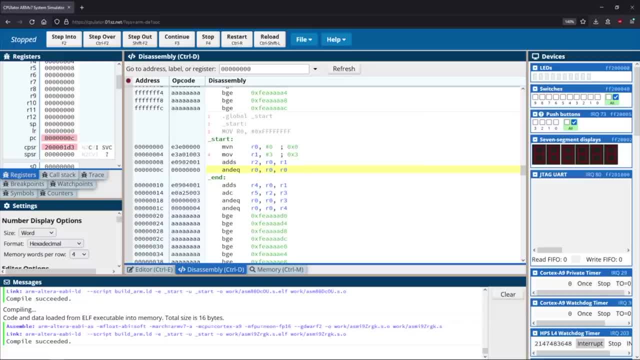 So these are the sorts of operations where you end up with, potentially, a carry right. So when these sorts of things happen, we want to be able to catch them, as we did here, But we may also want to use that carry at some point later on. 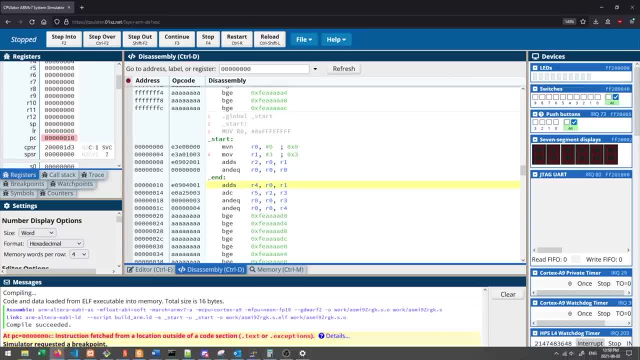 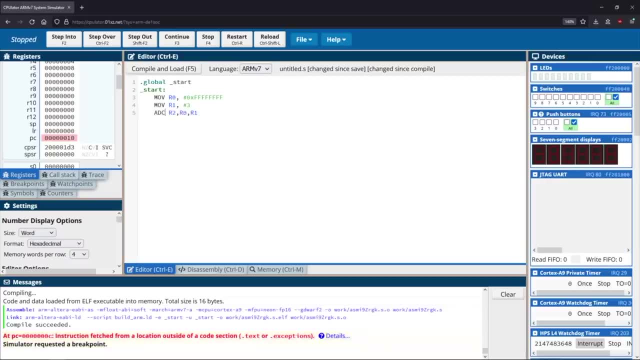 So if we want to add a carry operation, then what we need to do is we need to use the ADC operation. What this will do is it's going to give us the ADC operation. What this will do is it will add a carry to a result. 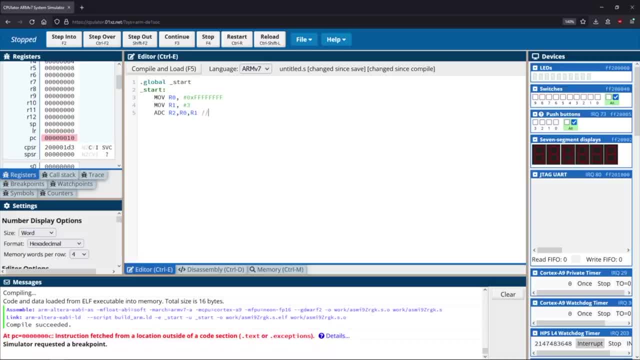 And what I mean by that is basically. so if we were doing this, this operation here, the result would be r2 equals r0 plus r1 plus the carry, So the carry will basically be a one if this flag is set equal to one, or it will be a. 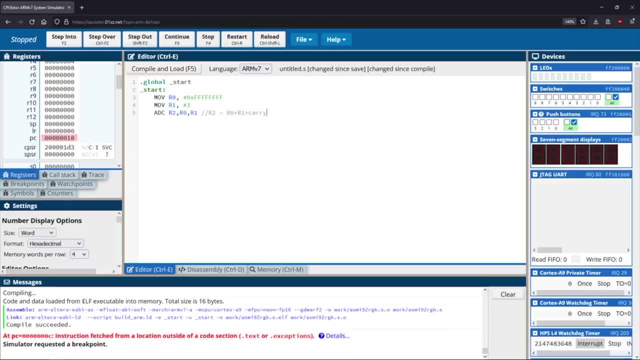 zero otherwise. So that's the way that this works. So it's either set to zero if the carry is not set, Or it's set to one if the carry flag is set. So that's the way this ADC operation works, And there are other ones as well. 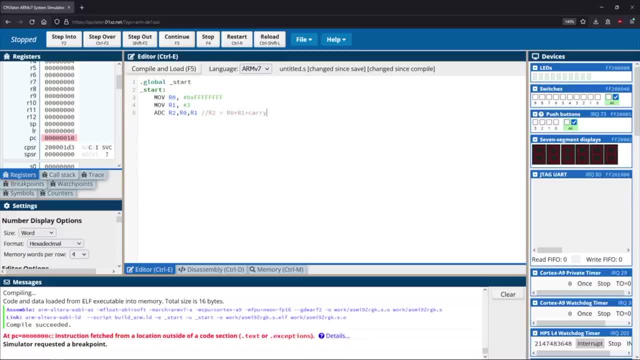 So we can subtract as well, Using the same sort of idea. we can also multiply with the carry, But the most common one would be the add, which would be ADC like this. So this gives you an idea of some of the fundamental arithmetic operations. 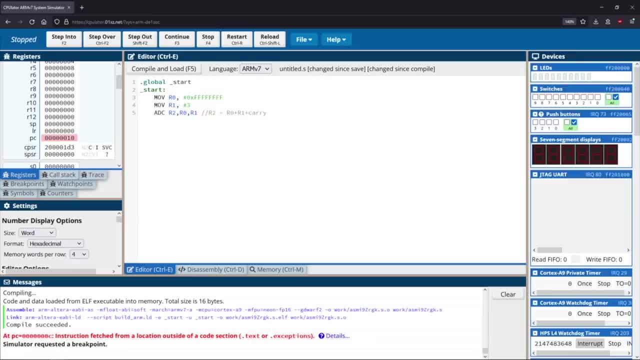 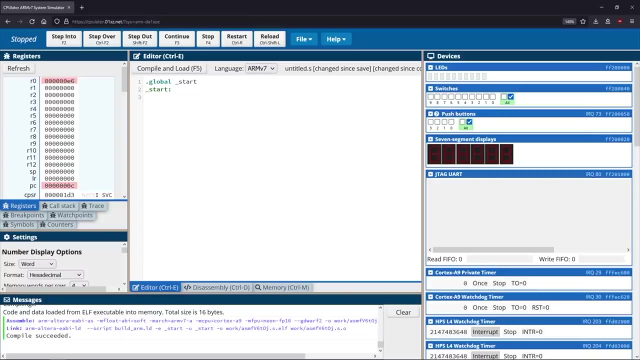 And we'll see these as we discuss other assembly programs. But this just gets you familiarized with how we add, subtract and multiply numbers and some of the little quirks of setting flags when we do these different types of operations. In this video we're going to take a look at basic logical operators in ARM. 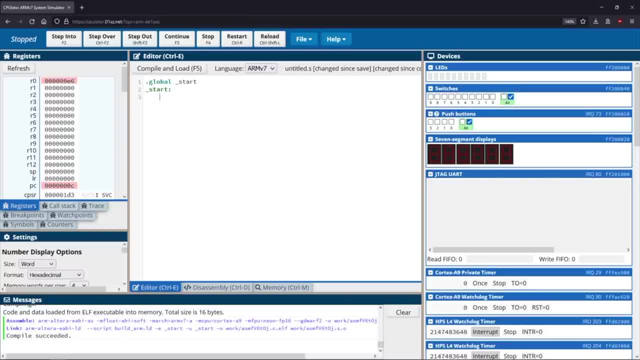 So these are operators such as AND, OR exclusive OR and negation that are used to complete bitwise operations on registers, And we're going to take a look at how these operators work. Let's take a look And in addition to that, I'll show you a few basic things that we can do with these operators. 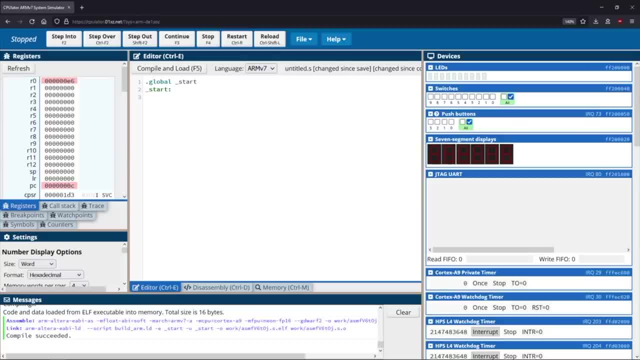 aside from the typical ideas of, you know, comparing if two inputs are the same or not, or those sorts of ideas. So, starting off with the instructions, the AND, OR, exclusive, OR, they all work very similarly to the arithmetic operators that we saw in the previous video. 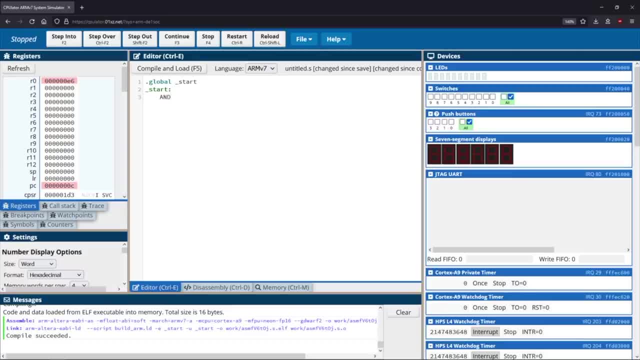 And by that I mean, for instance, if we were going to do an AND, we would have the destination for the results And then two things. So if I want to add an AND to the number of ANDs in R0, we're going to take the number. 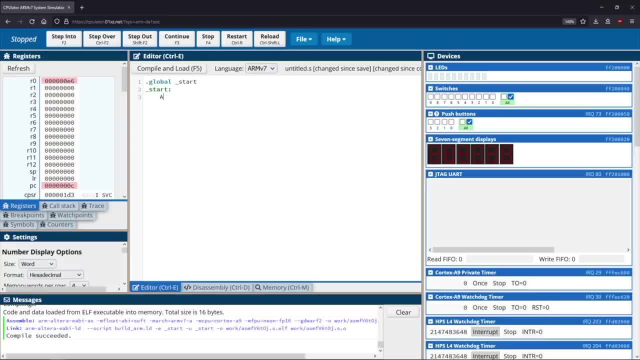 of ANDs that are being anded together. So that's the way that our AND operator will typically work. So, for example, if I were to do like a simple, let's move and let's move it to R0 with value FF. 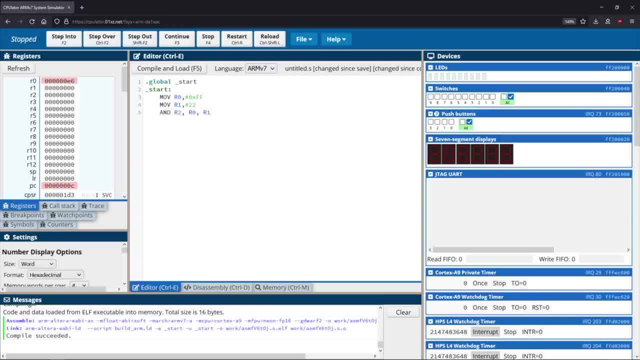 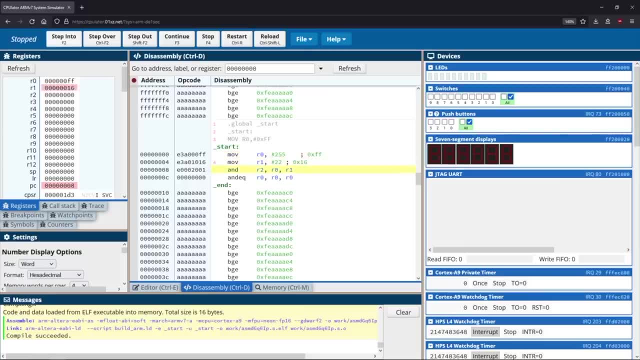 Let's move it to R1- the value I don't know, 22, for instance, And let's AND those two together and store the result inside of R2.. this one, we get 16. And then the result of ending those together is 16.. Of course, because all of 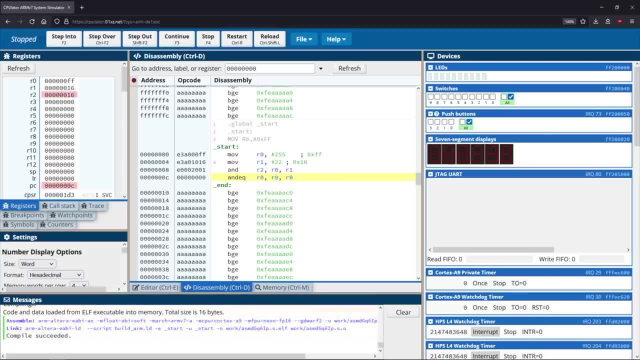 the inputs in the first one are all ones. So wherever the ones match up, we get one. wherever the zeros match up, we get zero, And that gives us the exact same result back. So you can see that that works the same way that we would expect any typical logical and to work. So this would be the 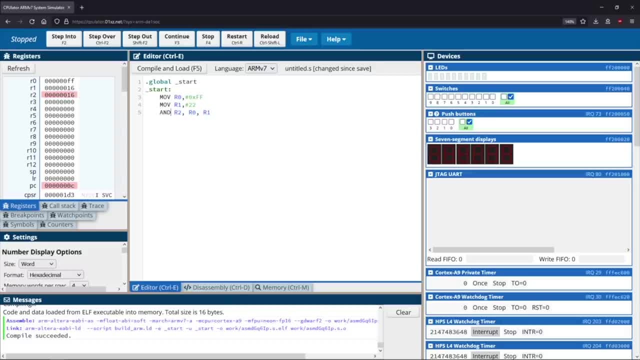 idea of our end. Now we can also do an end that sets flags using and s. So I just always want to note that with these instructions, typically there's always a complimentary version that will set flags as well. Most commonly, you're going to see just and being used, since we don't usually 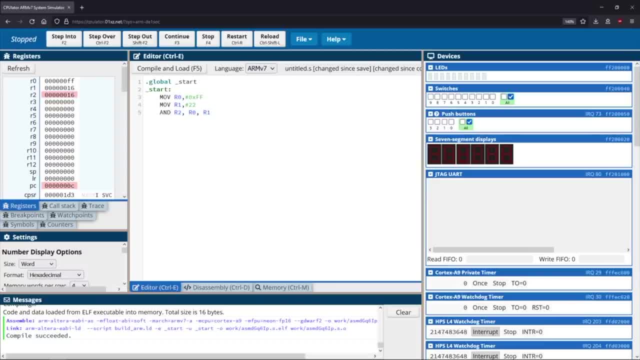 have flags getting set with the and operation. It's mostly just a matter of completing the logical operation and storing the results. So that gives us our and instruction or or instruction is similar. It's O R R for or. So just keep in mind it's not or, it's or with two Rs. 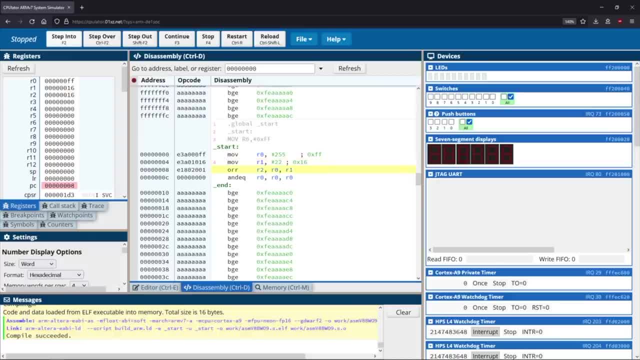 So, again, just to demonstrate how this works, you can see there are two inputs, are FF and 16.. And we are those together. we get FF because, of course, anywhere that there's a one, we end up with a one. And since F and F is all ones, 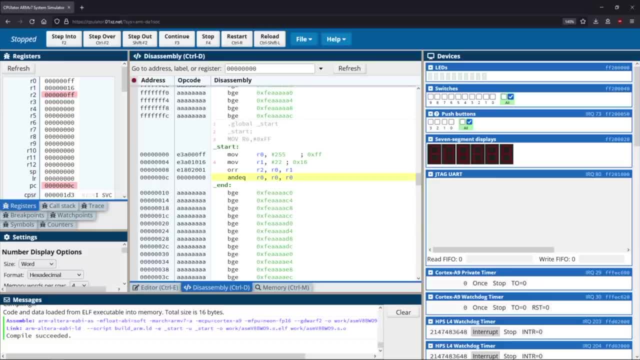 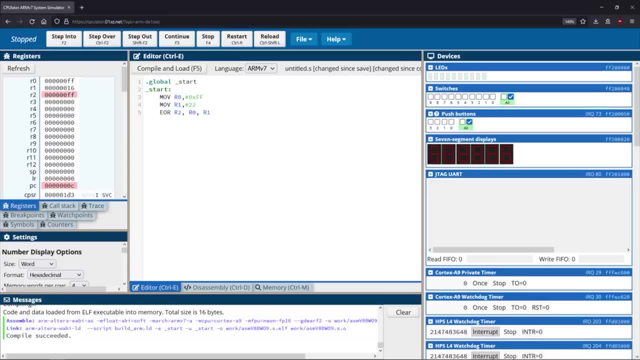 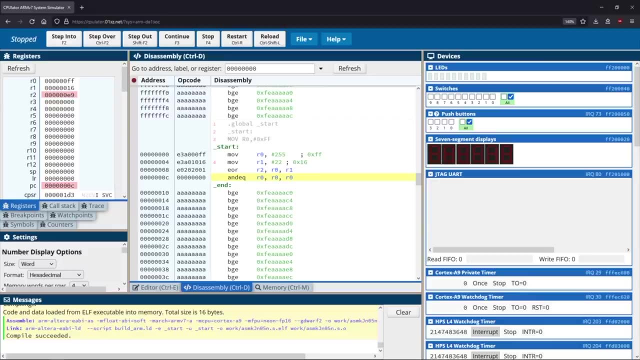 we always end up with ones which gives us the FF as our results. So that gives us our or operation, And then finally our exclusive or is E O R. So this is exclusive, or So just to show how this works, we have the FF, the 16. When we do those together, we get E nine. 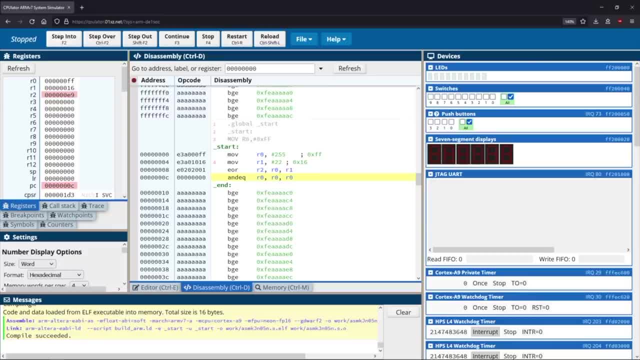 we get a one- Remember that an exclusive or is going to only give us a one if one of the inputs is a one, not both of them, right? If both of them are the same, we get a zero. Otherwise we get a one and that's our exclusive or? So you see that when we do this, we get exactly. 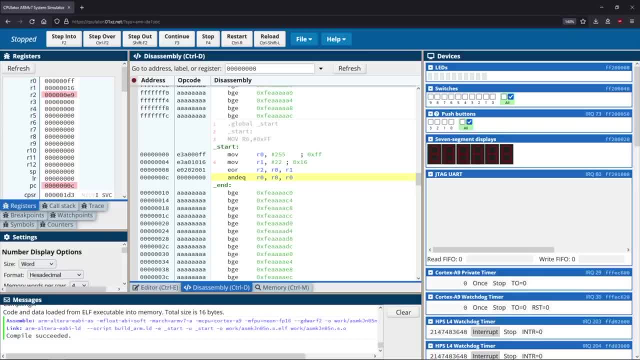 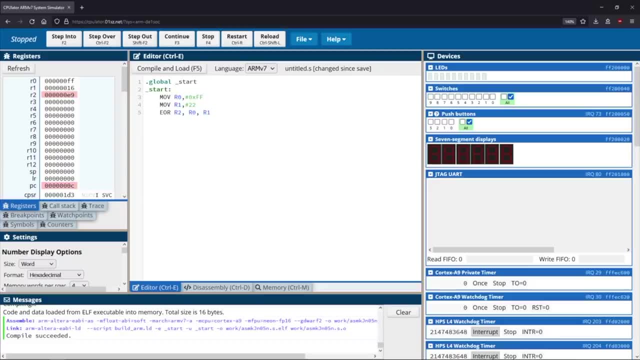 that result as expected. So those are the very basic logical operations. They're very simple and straightforward. There's nothing particularly special or interesting about them. The one that's a little bit different actually is negation. That's one that I want to talk about now. So with negation we do something slightly different. 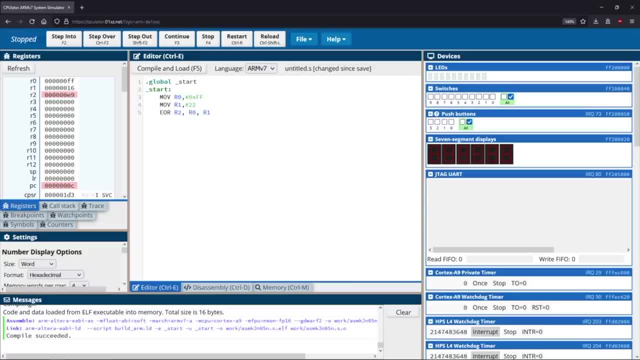 than just doing like a knot on the actual register itself. you might expect that you might have like a knot operation that does that negation. That's not the case in an arm. What we have instead is we have a special instruction called move negative- MVN. like this: What move negative does is it moves. 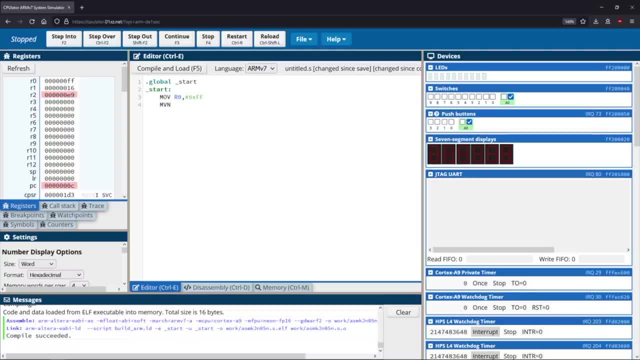 from the source, the negation of the source into the destination. So it negates the source and then puts that result into the destination. So it does a move and a negation at the same time. So to demonstrate that, let's just do this with r, zero and itself: what? 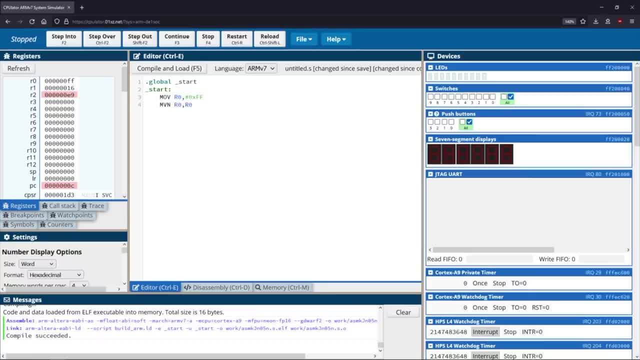 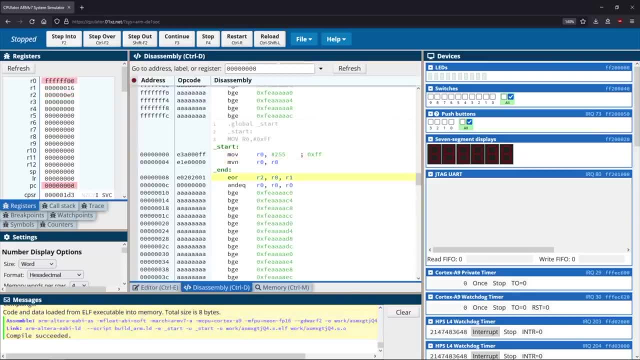 this will do is it will move r zero, it will negate it and put it back in the register that we started with. When we do this, you see that we start off with all Fs and we negate it. we get zeros in the. 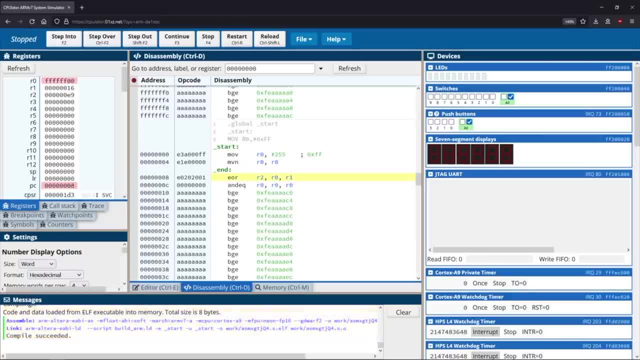 first two bits and Fs and all of the later bits. Now this might seem maybe a little bit strange, But if we do a negation, it negates the whole register, not just like the single bits or anything like that. it does it to the whole register. Now, when we have something like this: 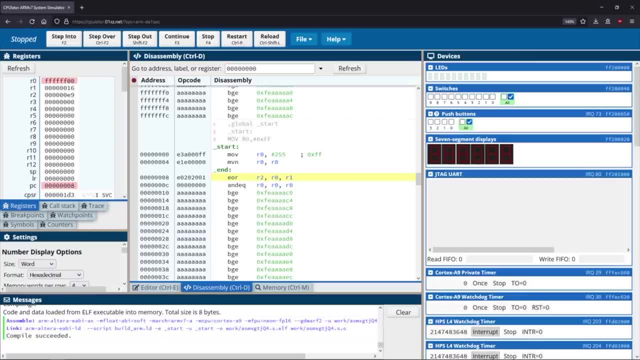 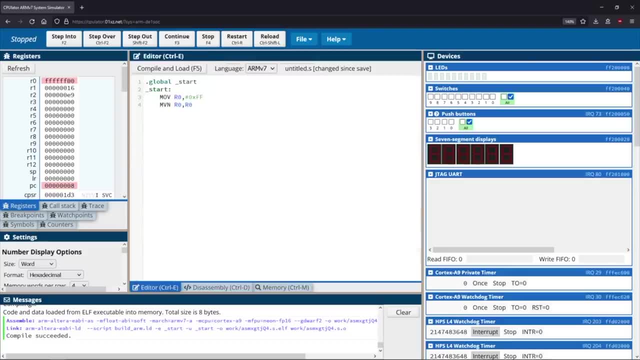 happen. we might want to make it so that the other registers are set back to zero, And the question is: how would we do something like that? And well, actually we can use our and operator to do something like that, right, What we could do is we could do an and storing the result in r zero. 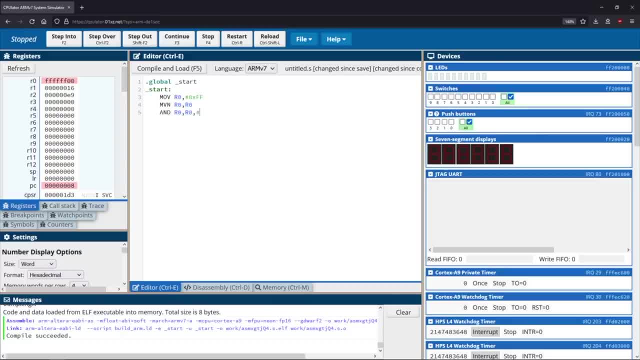 we could do an ANDing it with something that we know is going to give us zeros for this first six bits, or those first six hex values, right, Which would be zero x 123456.. And then the others would be FF, to keep whatever's inside of them. This will clear all of these bits, because anding 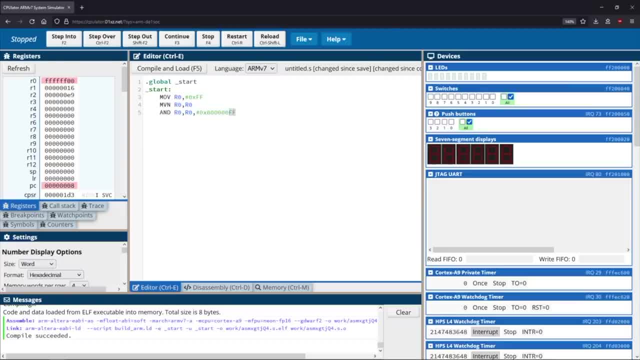 zero with anything gives us zero, And since these are always one, if we add anything with them, we'll get back what we started with right, either a zero or a one, depending on what the value actually is. And now the result of this is we start with the FF, we negate it and then you can see when we 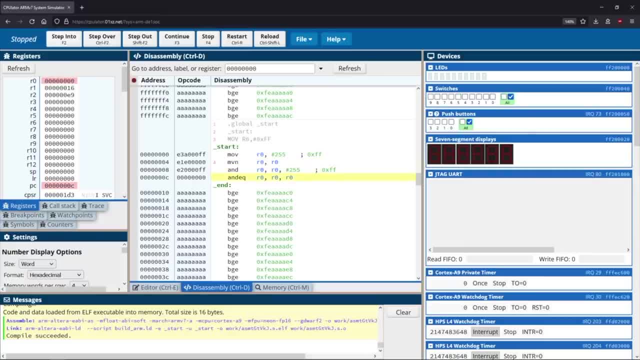 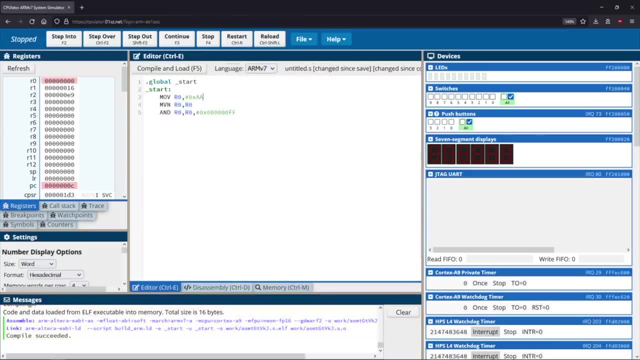 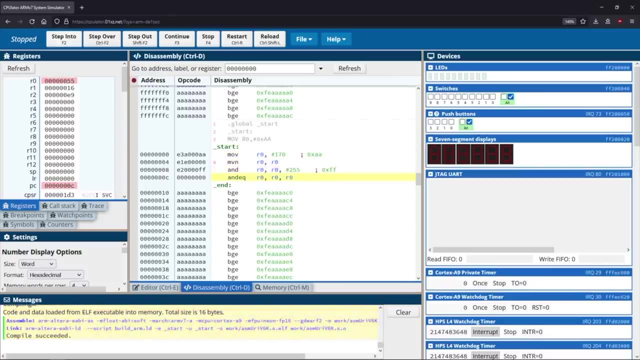 do the AND, it clears all the other bits, giving us this result back. And you know this might become a little bit more clear if I use like: let's do AA, for instance. When I do AA, for an example, you see that we get five. five here rather than zeros. You see that when we clear it, we keep. 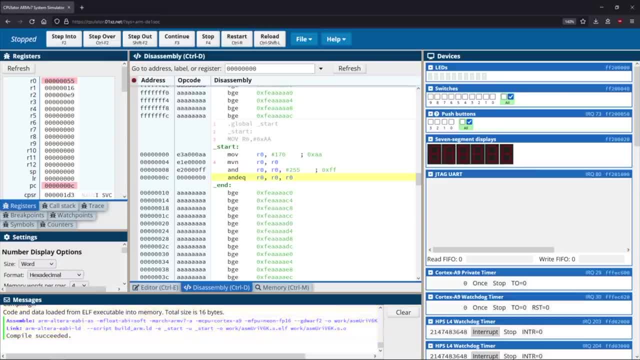 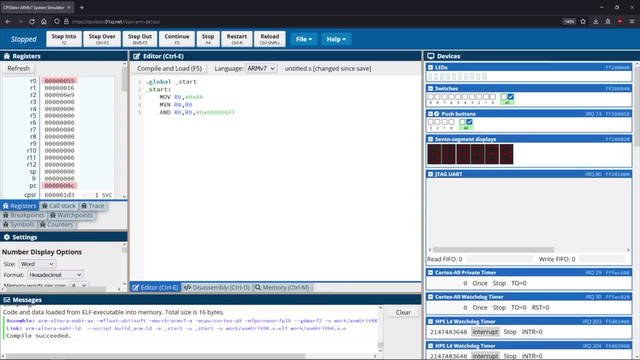 the five, five and get rid of everything else. That's something that we can use AND to be able to do is clear specific bits in a register. So that's one of the applications of AND. So this gives you a very basic overview of the different types of logical operators that exist. 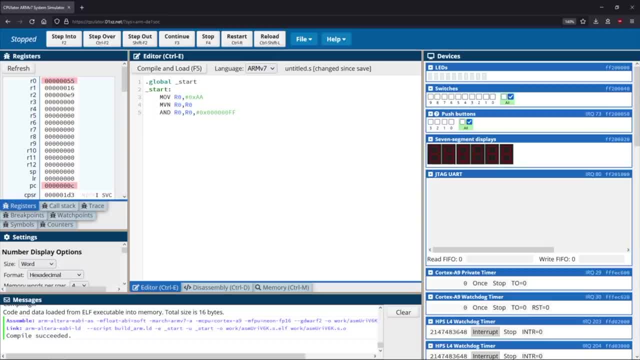 in ARM. This is, of course, very high level, and just like very simple examples, right? I just want to give you an idea of the instructions, an idea of what they might be useful for, And then from there we can continue to build on top of those concepts. So this gives you the very 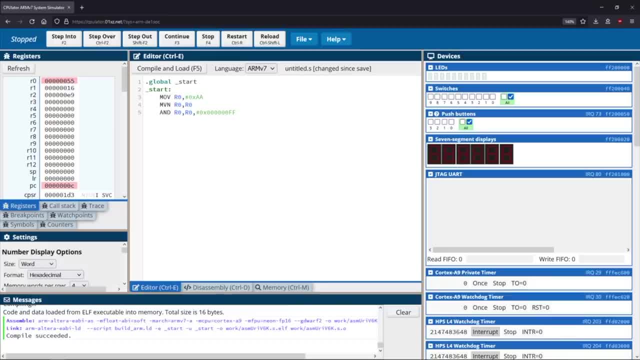 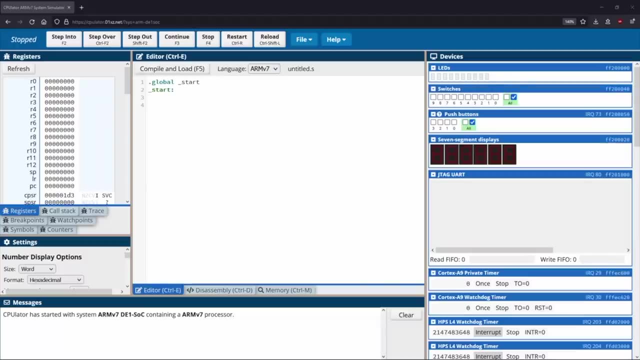 fundamentals of the logical operations, And then in future videos we'll see how they might be used in more practical sorts of applications. In this video, we're going to start to discuss logical shifts as well as logical rotations, And these two instructions are really useful in the sense that they allow us to manipulate. 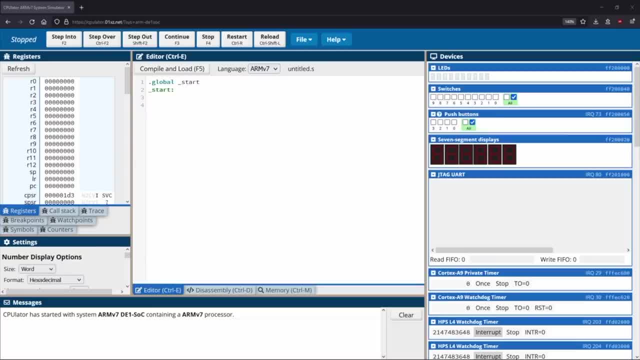 numbers at a bit level by way of shifting everything to the left or to the right. This has a lot of unique and interesting properties that are actually really useful to take advantage of. So what I'm going to do in this video is it's easier to look at this as a bit. 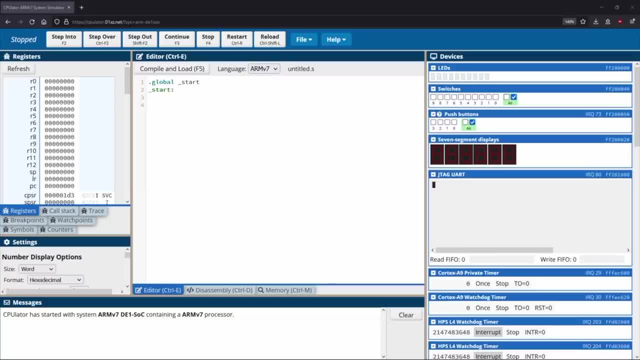 level operation rather than with hex or decimal. So I'm going to demonstrate to you what it looks like from a binary perspective And then in the next video we'll actually take a look at some examples with instructions in ARM. So this is just going to get you that basic foundation of 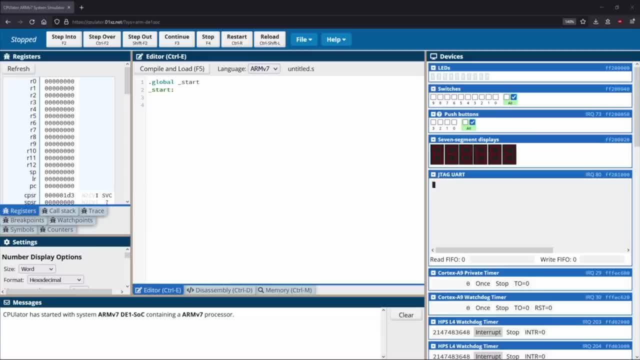 what is a shift? what is a rotation? What does it look like? What does it represent? Why do we use it? So that's going to be the main goal here. So we'll start off with shifts. With shifts, there's. 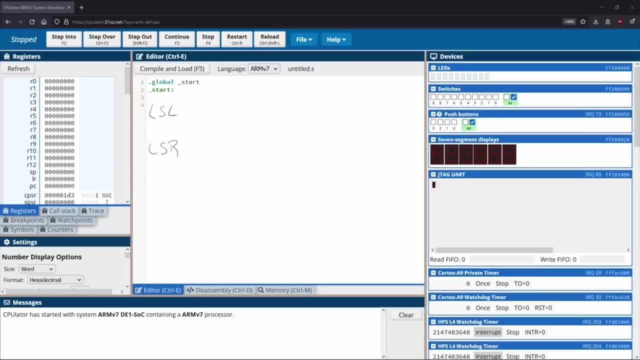 two different types of shifts that we see. there's a logical shift to the left and a logical shift to the right, And these two differ based on what direction the bits in the binary number shifting in. So to give you a basic example, let's just pick a binary number. let's say 1010.. This is 10. 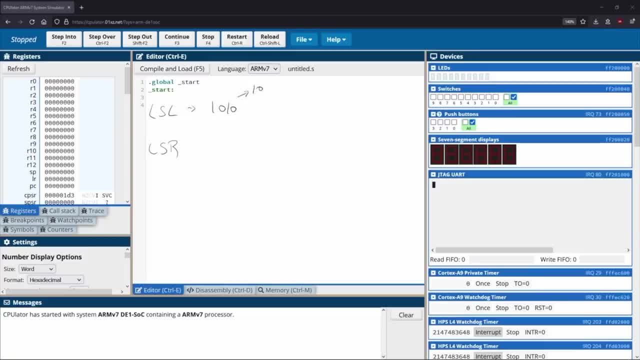 in decimal. So when we look at this number, when we're doing a logical shift to the left, what that means is that I'm going to move everything one position to the left of where it started. So this zero moves over here with this one used to be. this one moves over here with a zero used. 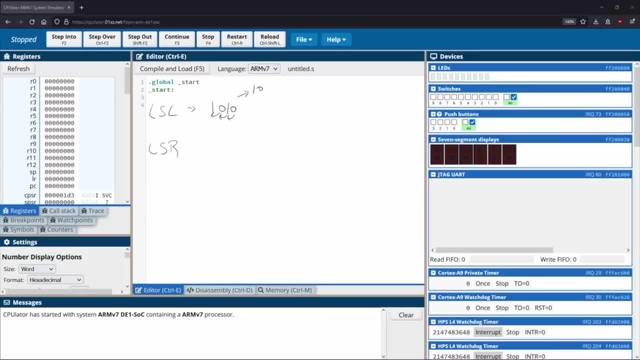 to be the zero moves to the one. And remember, since there's eight bits, I didn't write them in here, But there's, you know, eight bits of space here available. the one is going to move over here to this empty bit that didn't use to have anything in it. Now, the actual result of 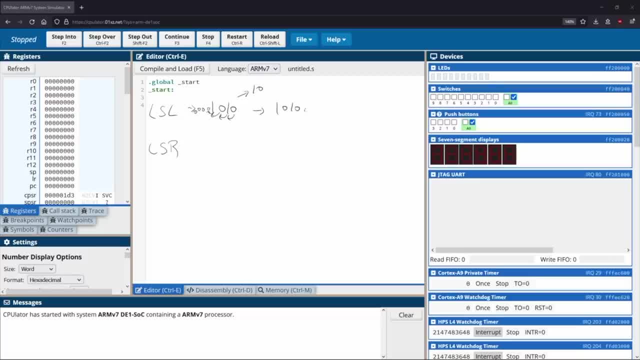 this is the following: we get 1010. And then there's an extra zero at the end. Now, when we take a look at this binary number, we actually see a really interesting property come up, And that's the fact that this is actually equal to 20 when you translate it to. 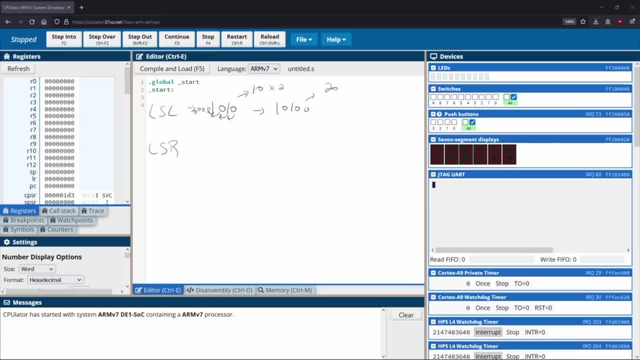 decimal And notice that this is exactly double what we started. it's like we multiplied the value by two And it turns out that isn't coincidental. that is true for every single instance of a logical shift to the left. It's the same as multiplying the value by two. As such a logical 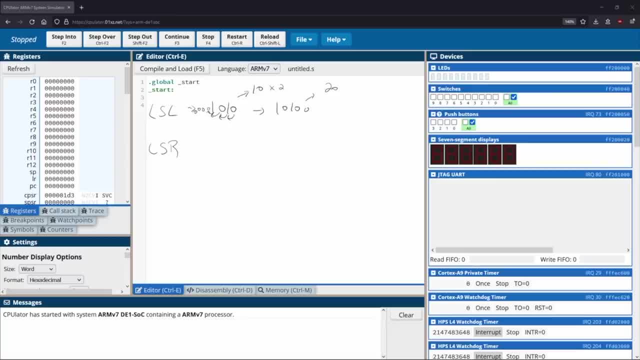 shift to the left actually represents a fast way to do multiplication by two, And that's the main value of doing this logical shift to two. So, as we looked at the answer, we're actually going to do it in the second latency. This is the first time in the last time we're actually using these two Now. 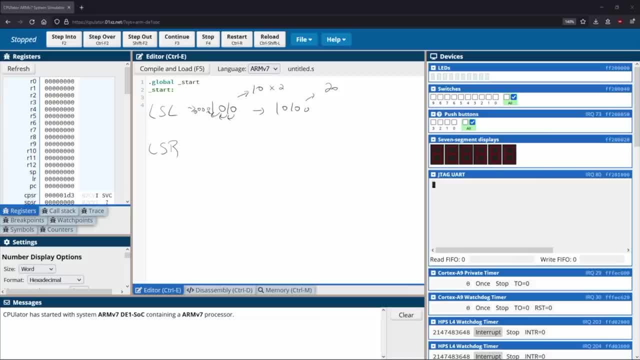 you can see the first time. you can see the first time and the second latency, And that's when you're actually just doing the first latency And then when you're actually doing the second latency, this logical shift. Now, there are other reasons why we might want to do it, But this is one that's. 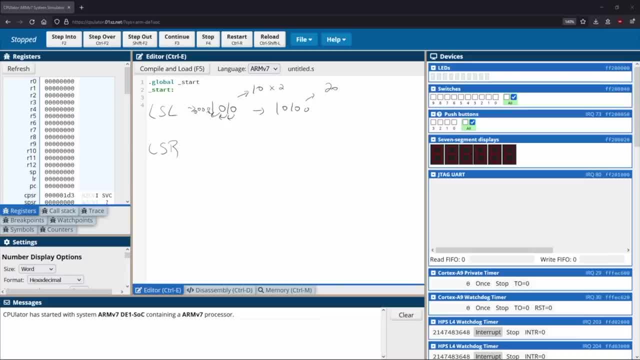 very obvious and prevalent, So this is something that we could take advantage of. So this would be the idea of your logical shift to the left. Now, when we take a look at a logical shift to the right, it does something very similar, but in the opposite direction, right. So we start off. 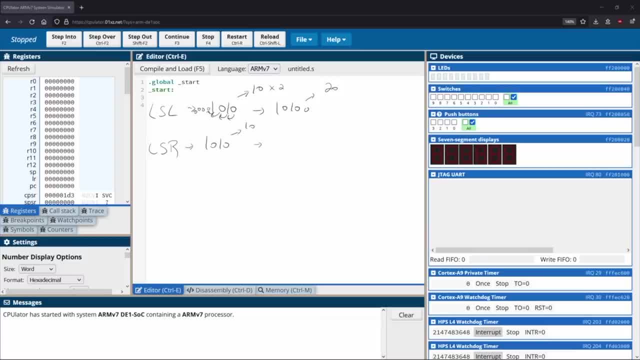 with 1010, which again is equal to 10.. If I shift everything to the right, it would mean that this one shifts over here with a zero used to be. the zero shifts over to the one, the one shifts over to the zero, and then we just get rid of the zero at the end, right? So this zero just gets it. 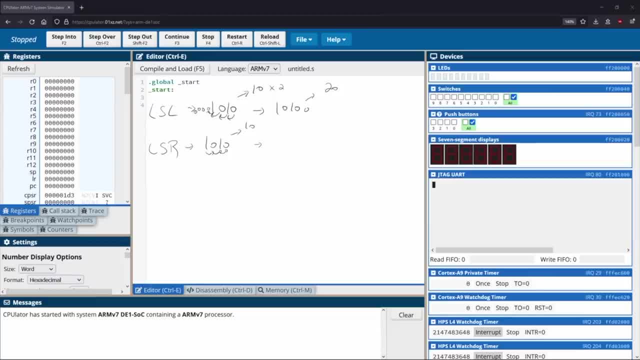 disappears right, So we don't really care about it anymore. Another thing that I'll just note here quickly: remember, there's technically zeros to the left of this right, So this zero here moves into the vision where this one used to be. The result of this is the following: we get 0101.. 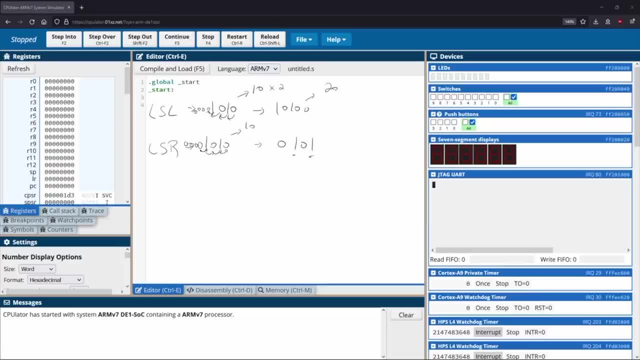 And what is this equal to? Well, this is equal to four and one, which makes five. Notice that this is exactly half of what we started with. So it turns out that when we shift to the right, it's the same as dividing by two. So 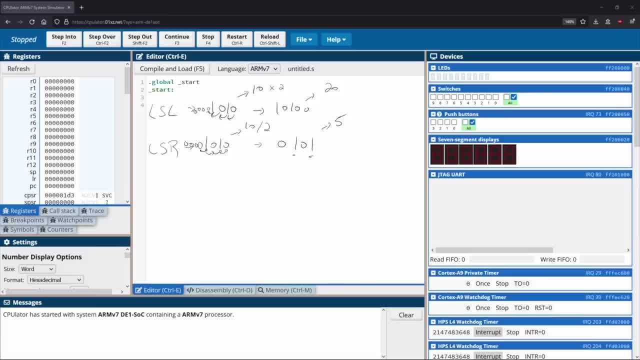 remember that we didn't really have a way to divide numbers before there wasn't really a division operation in arm. This is a way that we can implement division. we can do divisions by two, which allows us to be able to actually do full division operations. So this allows us to have 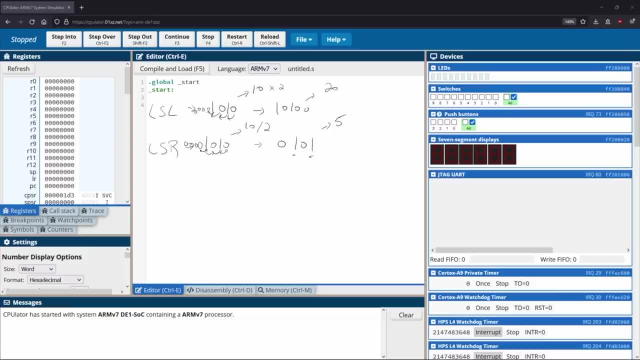 division. And again there's other reasons that we might want to do shifts to the right or shifts to the left, But these are the two most obvious ones that are really valuable to know about. And just in case you're really wondering like, why is this true? you can. you can intuitively figure out why this ends up multiplying by two. 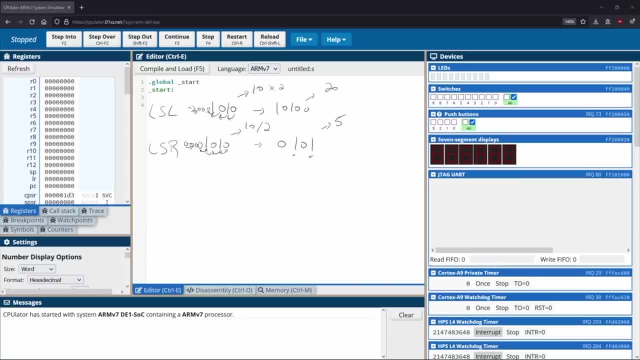 right. If you think about what shifting to the left really does, is it increases the power of all- the powers of two here by one, which is the same as multiplying by two, whereas this one decreases all of them by one, which is the same as dividing by two. 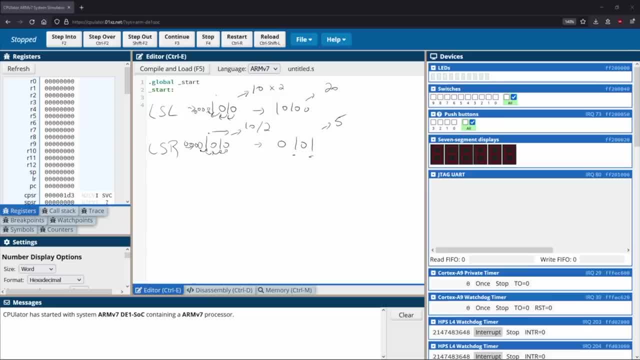 So there is actually an intuitive reason behind that. if you want to go through and actually sort of like derive why this is true. So that gives you an intuition behind logical shifts and hopefully gives you a bit of an understanding of why we care about them and what they are useful. 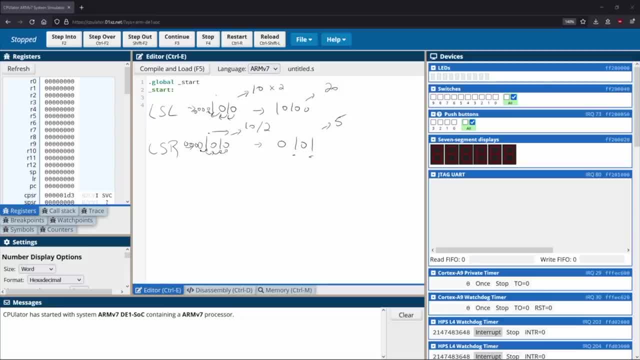 for The next thing that we'll talk about is a rotation, which is r o r, And a rotation only really differs from a shift in one single way, And that is that, when we talked about the shift to the right, I said: 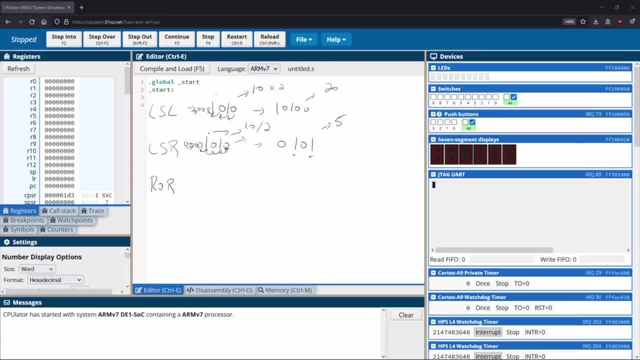 is zero, we just get rid of it, right. So the rightmost thing, we just get rid of it, we don't care about it anymore. With a rotation that doesn't happen, the rightmost thing actually loops back over to the leftmost position. So let me show you an example of that. Suppose that we have the 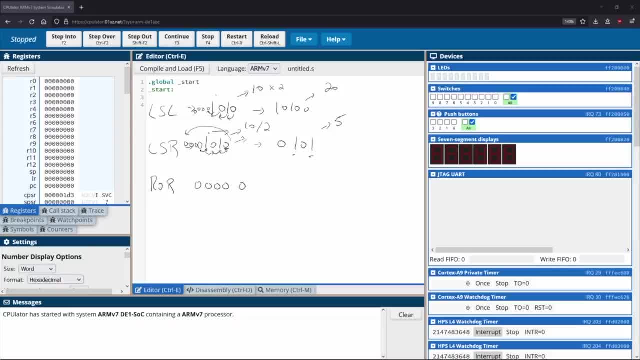 following. So I'll do all eight bits this time And suppose we have something like this. So, first off, if I did a logical shift to the right, what you would end up with is you would end up with: you know, we have all the zeros here. 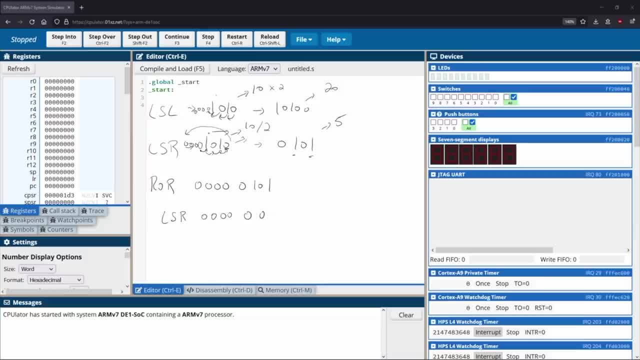 We have zero, remember- everything shifts over to the right one, So you'd get 0010.. This would be a logical shift to the right. in this case, right Now, if we were to do a rotation, what we end up. 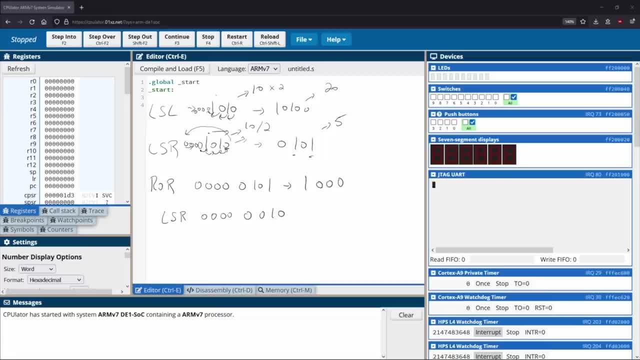 with. instead, as we end up with this, we end up with 10000010.. Notice that this one moved to the front rather than just getting eliminated. So this gives you the difference between the logical shift in the rotation. Now you might ask: why would we want to use a rotation? 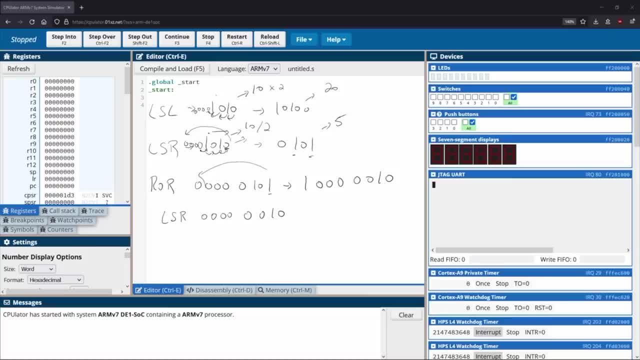 The uses of a rotation are actually a lot more abstract than a shift. When we're dealing with rotations, we're typically using it for things like hashing, we use it for crypto, we use it for graphics. it's not an entirely common operation to see. it's typically actually left in for 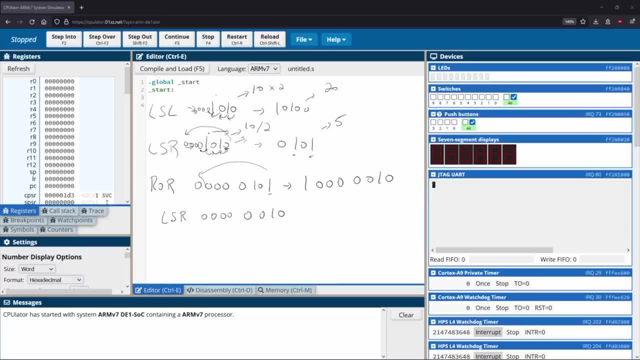 historical reasons, And one thing that you'll notice because of this is that arm doesn't actually have a rotation to the left like an ROL. this does not exist, So we can only rotate to the right. If you do a rotation to the left, you can technically do it with rotation to the right. So if you want to, 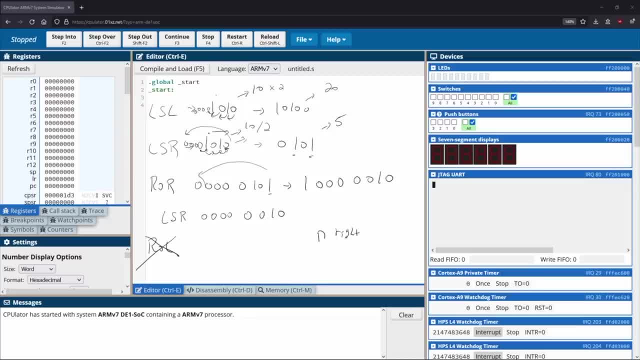 shift n bits to the right. what you would do is you would do- sorry, if you want to shift n bits to the left. rather, what you would do is you would do a rotation to the right 32 minus n times, And you know you could sort of play around with that and see that it actually is true, What that does. 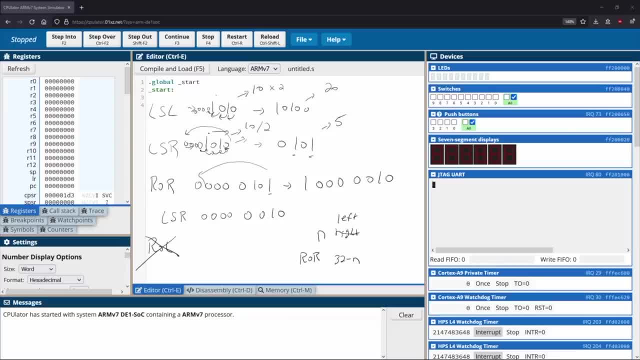 is, it rotates over to the left hand side rather than the right hand side. But again, these sorts of the rotations are not very commonly used, We don't see them all that much. so they're sort of just something that I'm adding in here to say, hey, these exist, There are some applications of them. 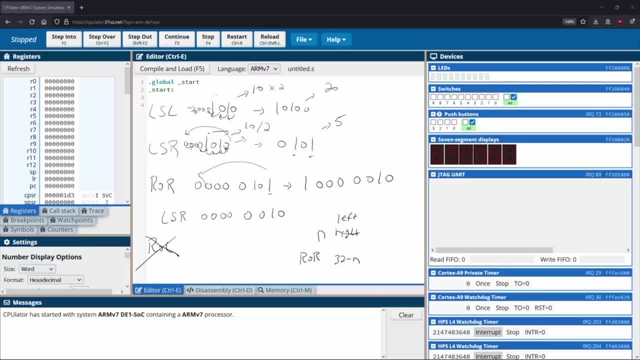 in hashing and crypto and graphics. You might see them at some point, but they aren't entirely common. But this is how they work, just in case you ever do see them. So this should give you a good groundwork foundation for logical shifts and logical rotations In the next video we're going 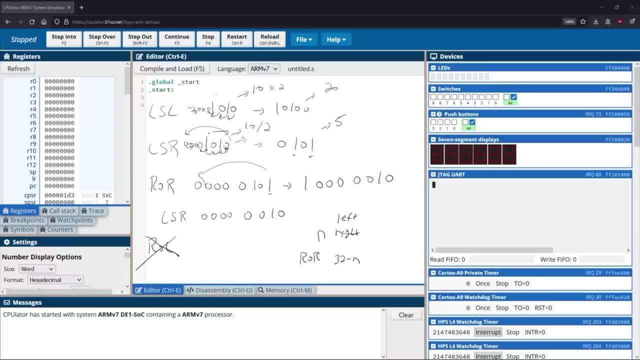 to actually go through and see how we can implement these things in our ARM assembly emulator. In this video, we're going to take a look at how logical shifts and rotations are actually used in ARM, So we're actually going to take a look at some practical examples and see how these 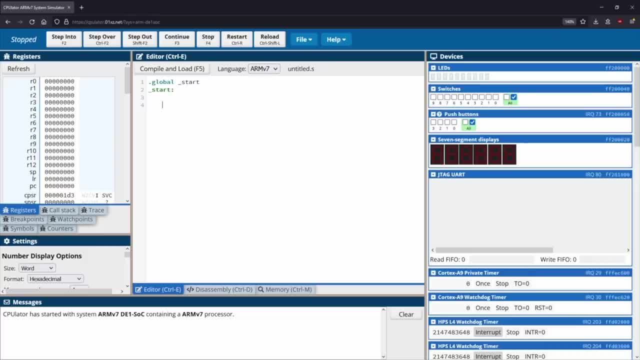 instructions actually work and be able to demonstrate that they do actually do, as I said, multiplying by two and dividing by two- and make sure that these results are actually truthful. So to start off with, let's look at a very simple example. We'll do something. 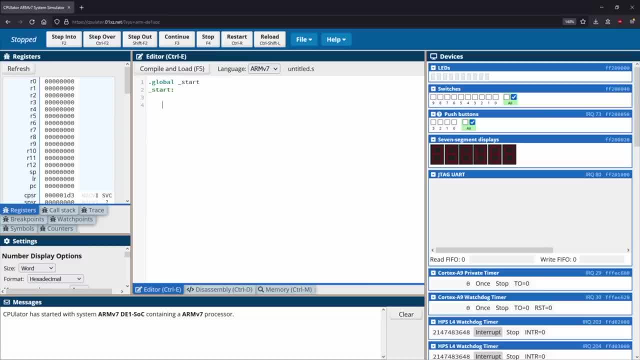 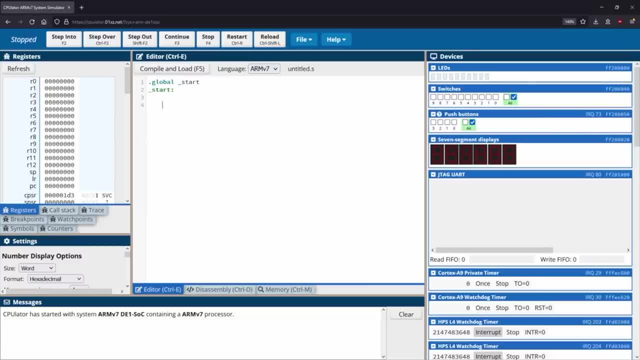 what we did was we had 10, and we did some shifts on it. So we did some shifts to the right, some shifts to the left, And we'll take a look at what those results end up being. So, to start off with, I'm going to go ahead and move the value 10 into register zero. 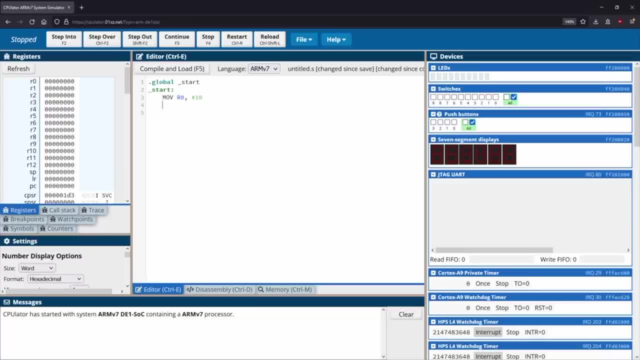 Once we have done this, what we're going to do is we're going to do: let's do a logical shift to the left to start off with. So the way that we do this is we're going to do lsl, We type in the register that we want to shift, And then we're going to indicate. 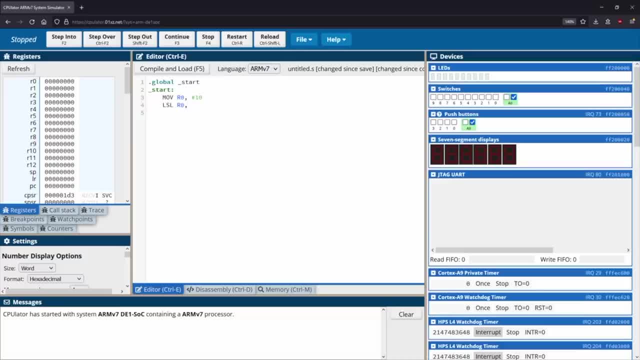 how many times we want to shift. So what I was demonstrating in the video previous was that we could shift one time to the left, And if we shift one time to the left it was the same as multiplying by two. With arm, we can actually specify to shift multiple times if we want to. And the way to think. 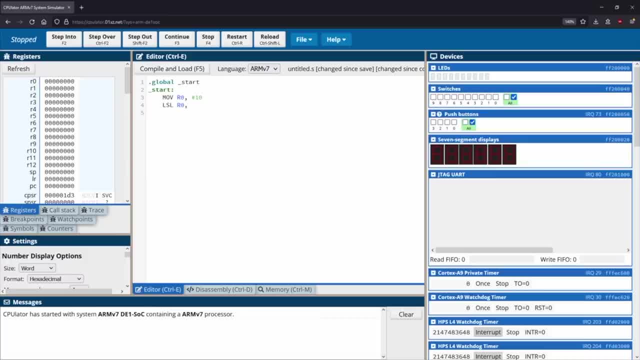 about that is that it's the same as just multiplying by two repeated amount of times. So if I shift to the left twice, what I'm doing is I'm multiplying by two twice or multiplying by four. right. If I shift three times, that I would be multiplying by two three times right. So that's. 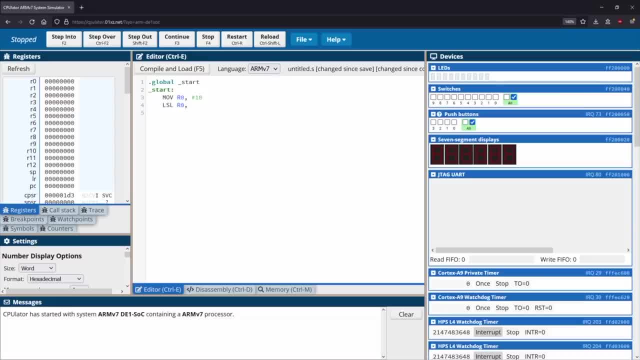 the idea of what we're looking at when we're saying how many times we would like to shift. So if I want to shift everything to the left one time, which would be the same as multiplying by two, I simply indicate that here Now. something that's interesting about this is that you can 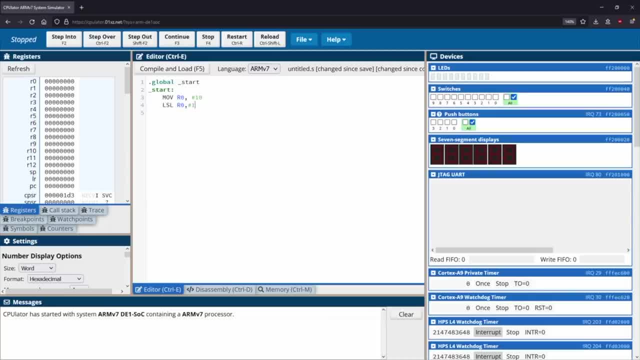 actually use this to shift by a variable amount, right? So I could put in like a register, like r1, and say shift by the number of times that's inside of the register r1, right? So there's ways of being able to combine this together to be able to utilize like a variable. 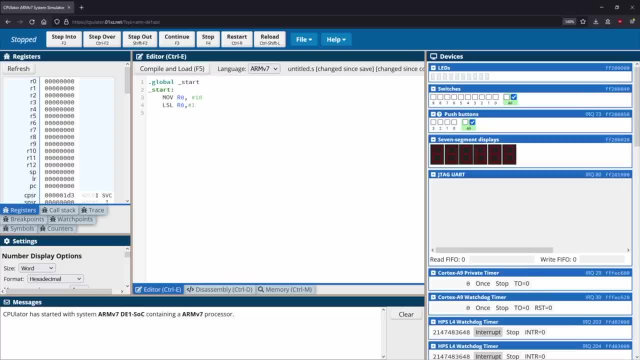 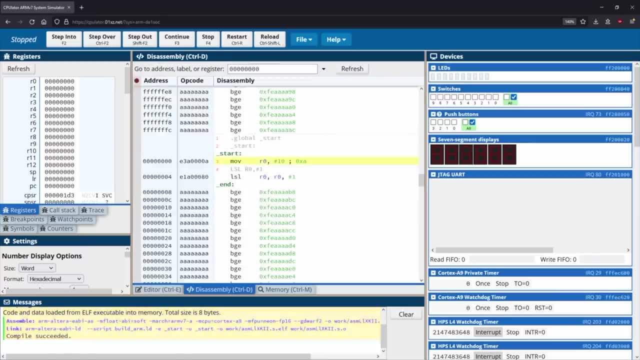 amount of shifting. So that's one thing that you're able to do. that I just want to note here. So, with that being said, let's take a look at what this actually does. So we compile and load. the first load is going to put 10 inside of this register, And we're just 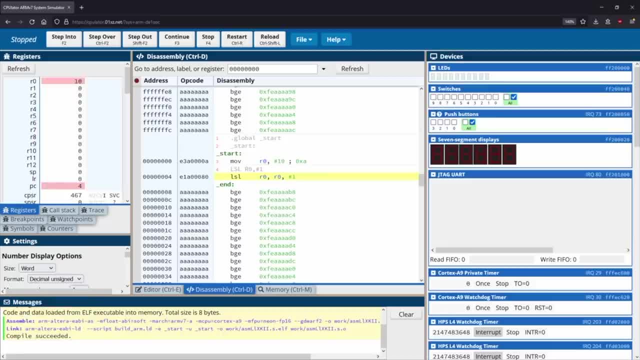 going to go ahead and change this to decimal, just that way we can see it a bit easier. So you can see that we have 10 here. The next time that we move through, we do our shift, which changes it to 20.. And, as you can see, it does as I said it would. it multiplies it by two. 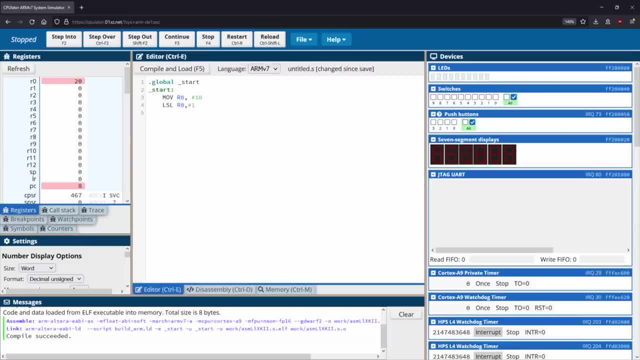 And just to continue on with this, we'll go ahead and do a rotation to the right and just we'll do a shift to the right, rather and see what that ends up doing. Now, what I'm anticipating this is going to do is it's going to shift to the right by one. 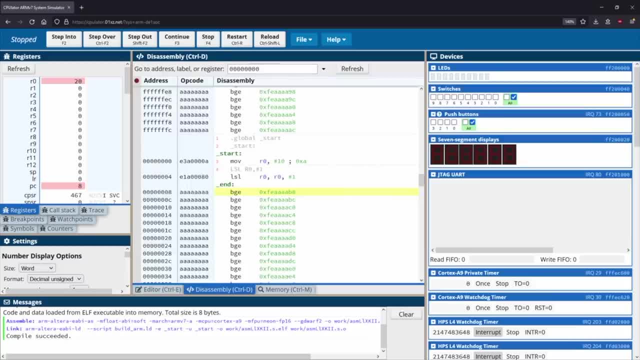 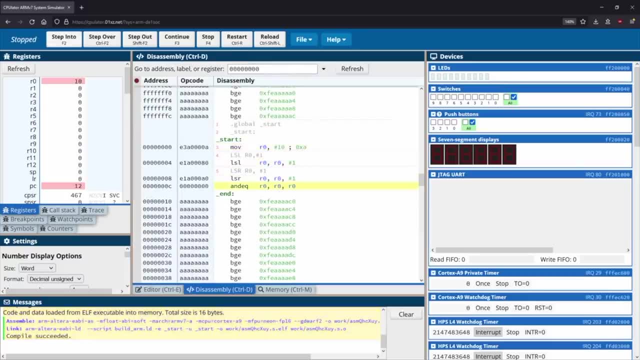 bringing us back to 10.. And let's just see if that actually does happen. So we'll go ahead and compile and load. We start at 10,, we end up at 20.. The next shift brings us back to 10.. So you can see that generally this is working the way that we expect. 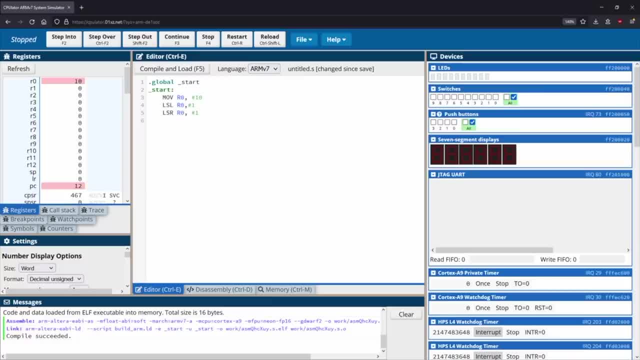 it to. So this is nice and simple, nothing too complicated here. Now, one thing that we can do is shifting. that's quite interesting and unique is that we can combine it with the move operator to do a move and a shift at the same time. This is a really useful sort of thing to be able to do. 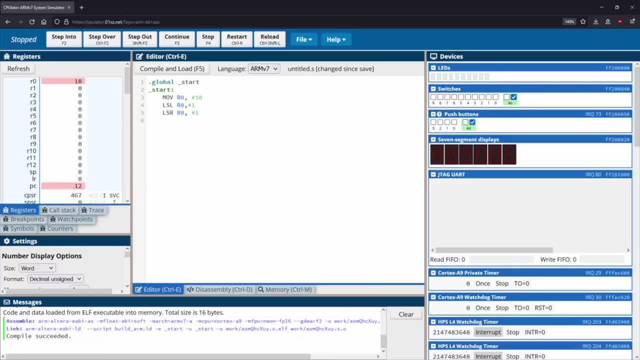 To give you an example, I don't want to shift our zero. maybe I want to store the result of multiplying our zero by two into register our one. So just to demonstrate what that would look like currently with our current instruction set, I'll just go ahead and get rid of this line. What I'm saying I want to do is I: 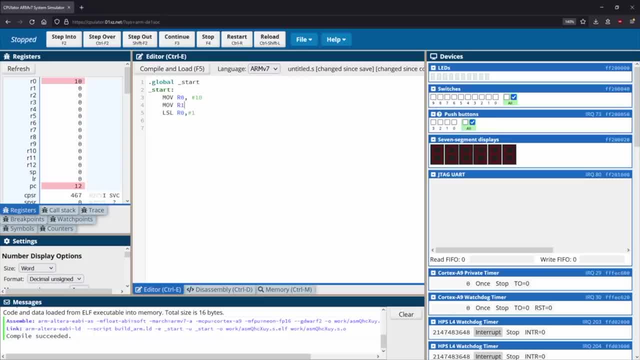 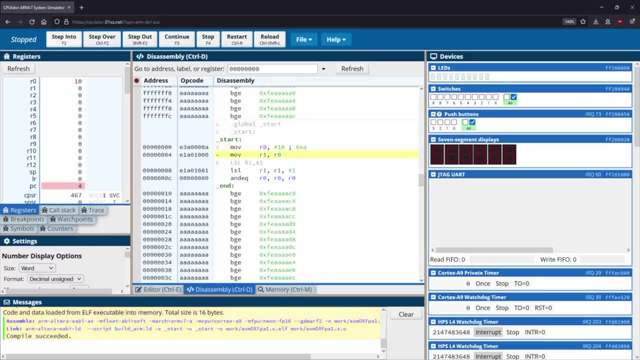 want to move, you know, our- into our one, the value our zero. And then what I want to do is I want to do a shift on our, one by one. So what I'm doing is I'm preserving the value of our zero. 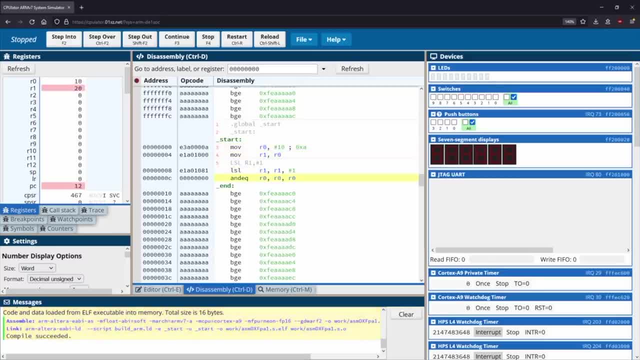 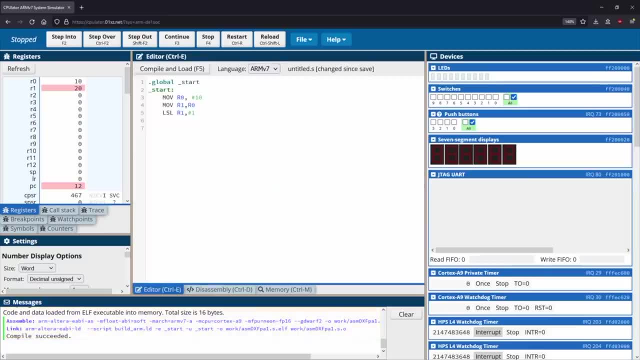 rates. that way, our zero doesn't actually change. our one stores that value instead. Now, rather than having to do the move and shift in separate instructions, we can actually do them together. So what I can do is I can add on a third piece here I can say LSL One, just like this. what this is going to do is: 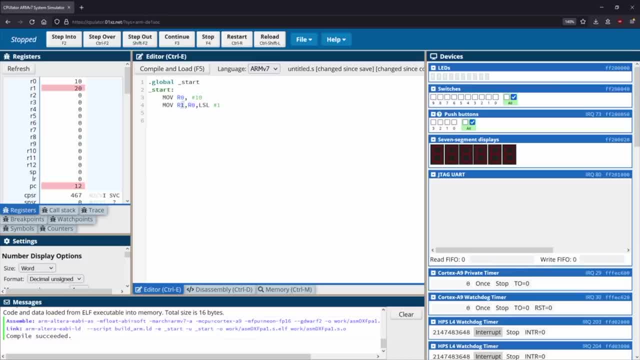 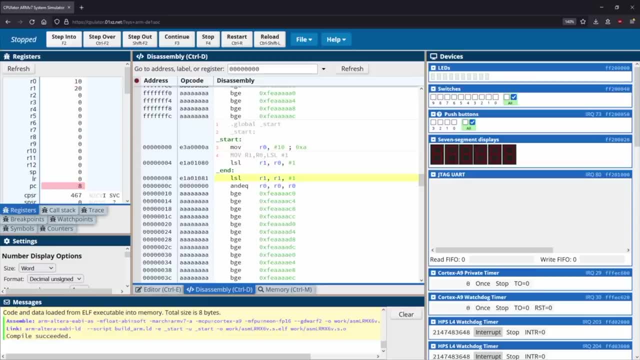 it's going to move the value stored in our zero into our one and then it's going to shift it by one. So let's take a look at what happens. So we get 10. And then you can see we get 20 directly. So you can see that it does that shift. 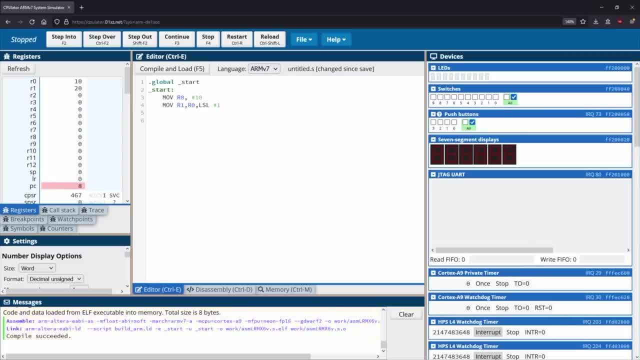 immediately, right, So we don't have to worry about it happening. you know, multiple times. right, we don't have to do it in multiple separate instructions. we could do it all in one instruction instead. So this is something sort of unique about the shifts that we haven't seen with. 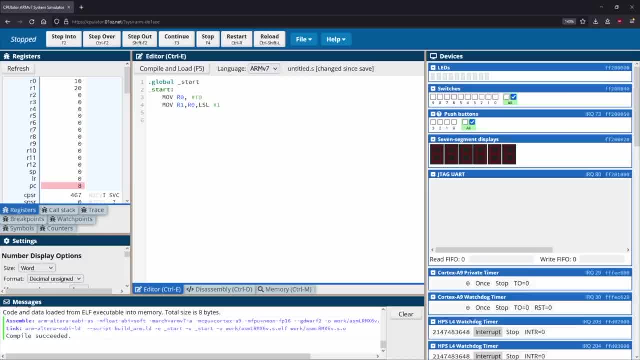 other sorts of instructions so far. So that shows you how the logical shifts work inside of arm. I'm going to end off here just by showing you a rotation, Just that way you're able to see what that ends up looking like. So the instruction for rotation is: 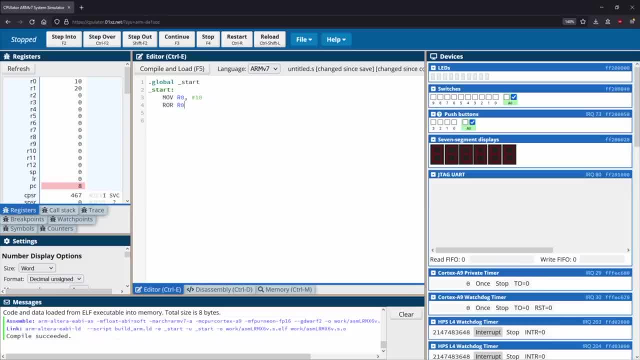 of course ROR, like we said, And of course we could do some examples of shifting by one, for instance, although we should pick a number that will actually flow over into the remaining, you know, and so that goes over to the left hand side. Let's see, I think our value perhaps like well. 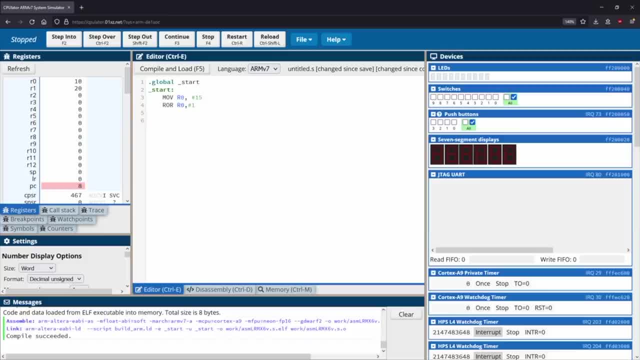 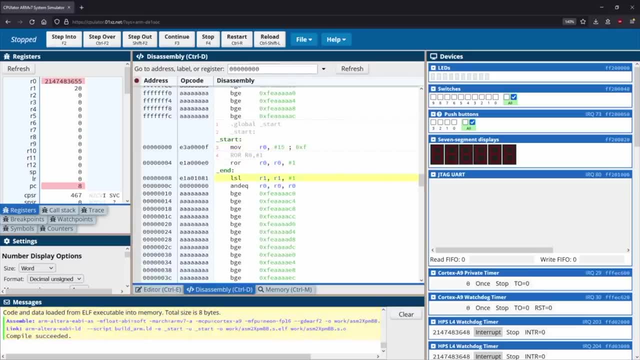 value like 15 should definitely do it right. We don't have all ones on the right hand side, So let's go ahead and give that a try and see what happens. We get 15. And you see, when we overflow over, we get this massive number. here, This one: 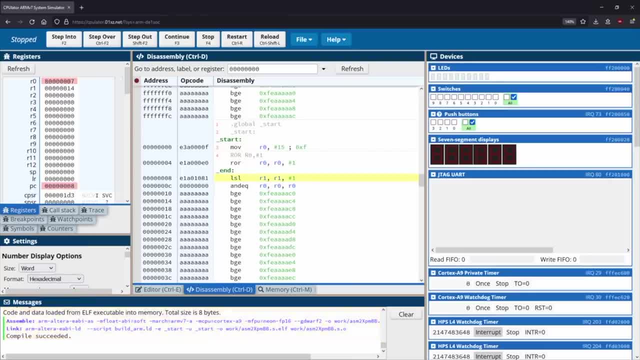 it actually helps to look at the hex to see what ends up happening, right? So you can see that we have eight as our first hex value, which is 1000.. So you can see that the one shifted over to the front, we still have seven on the right hand side, which implies that we have, you know, all of the. 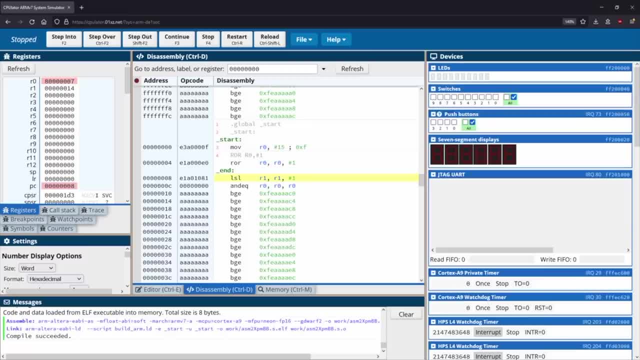 ones remaining, except for the one that was on the end. right we have 0111. And then, on the other hand, we have 1000 on the left hand side. So you can see how this rotation is generally working. it is doing sort of the idea of what I was saying would happen with it. 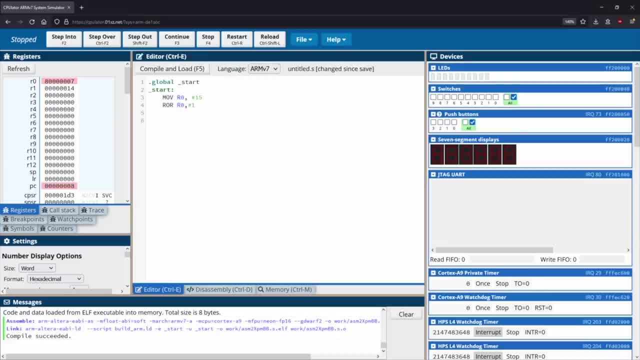 So this gives you an idea of how the rotations work, And I want to note as well that you could do the same thing with rotations that we did with with moving right. we can put it into the move instruction And we can rotate as loyal as the move right. So the same sort of idea is what we 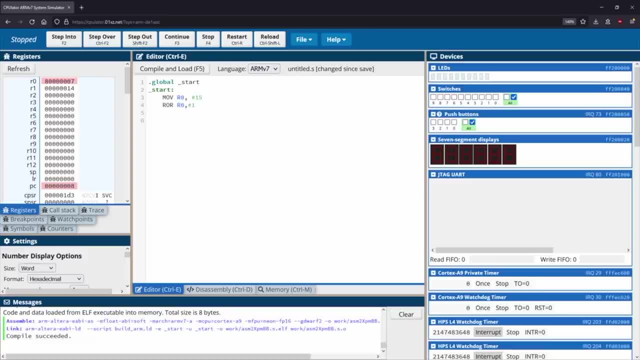 did with these shifts before. So this demonstrates you how rotations and shifts work in arm. So you now understand what these operations do, what their value is and how the instructions can be used in arm. Next video we'll take a look at some other instructions through arm and we can get a better understanding of some 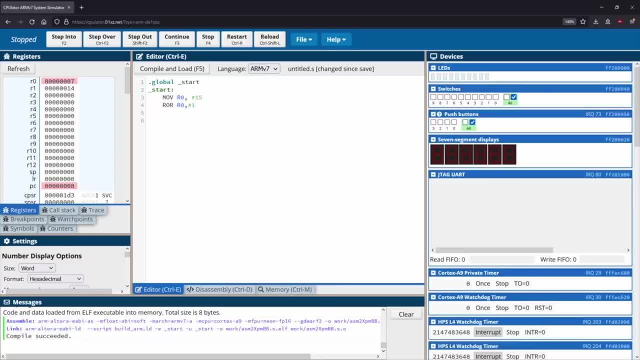 more advanced things that we can do with this programming language. Now that we understand some of the basic instructions in arm, we can start to take a look at some of the typical high level constructs that we would see and find out how they map generally into the 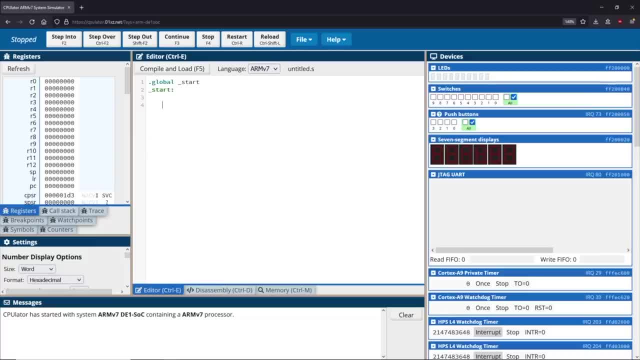 assembly language, And the way that we're going to start with this is by taking a look at statements related to conditionals. These would be statements sort of like if statements in higher level languages. we want to take instructions based on the results of something else that has happened. 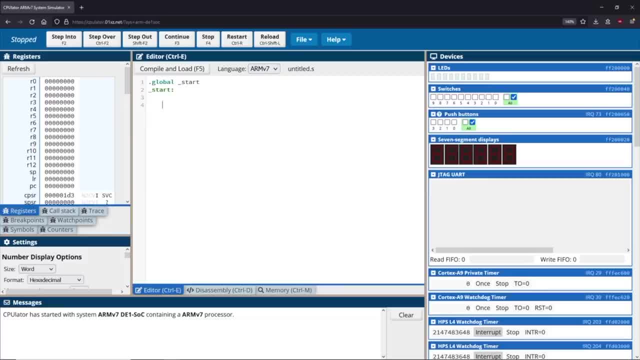 in the program already- perhaps something related to a user input or something of the sort- And we want to be able to take different paths based on the values that are provided. So in this video I'm going to give you some really basic examples of how this can be done. 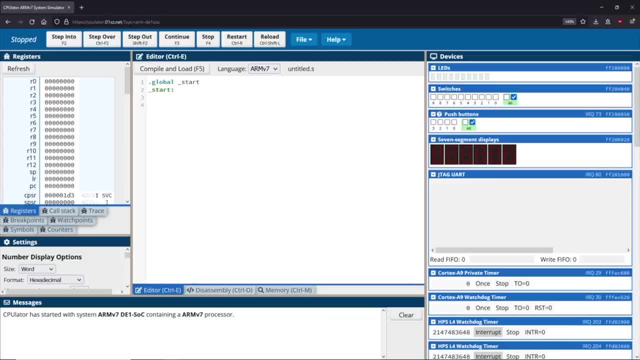 So the main way that we do these branching instructions is using comparators and branches. So a comparator is something that allows us to compare two values to determine whether or not they are greater than, less than or equal to each other. Branches, on the other hand. 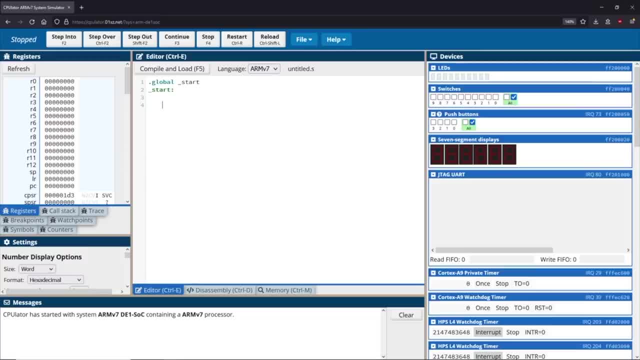 allow us to move around our program to different locations based on the result of comparisons. For example, we might want to move to a different part of the program if a result is greater than another, Or maybe if two results are equal, we move to a different location in the program. 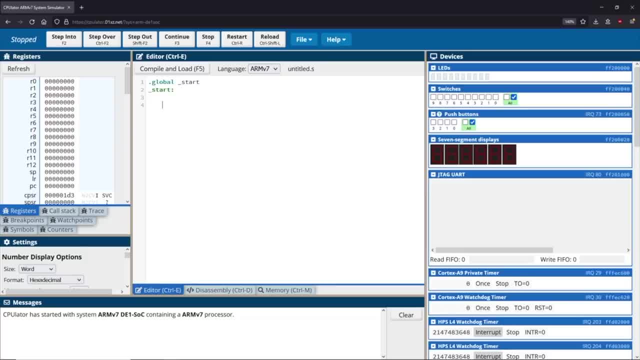 This is very similar to the way that if statements and else statements work in your typical programming languages. So let's take a look at a really simple example. I'm going to go ahead and move some values into some registers. We'll do some comparisons and see generally how these branches actually work. 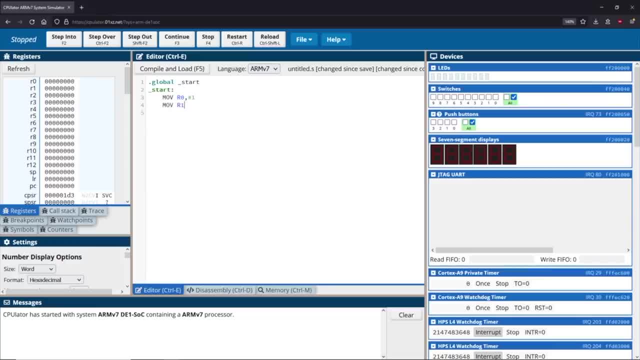 So let's move it to R0.. The value 1.. I'm going to move 2 into R1.. And now I'm going to do a comparison between these two values. The way that we do this is we use CMP. That's our comparison instruction, And then we give it. 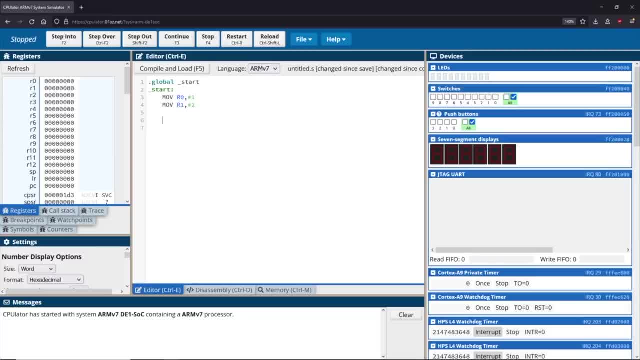 two arguments. I'll discuss how this generally works once we've got it written out here. So what a comparison is really doing is it's going to take a look at R0 and R1, and it's going to do the following computation: It's going to do R0 minus R1.. So it's going to subtract the two from each. 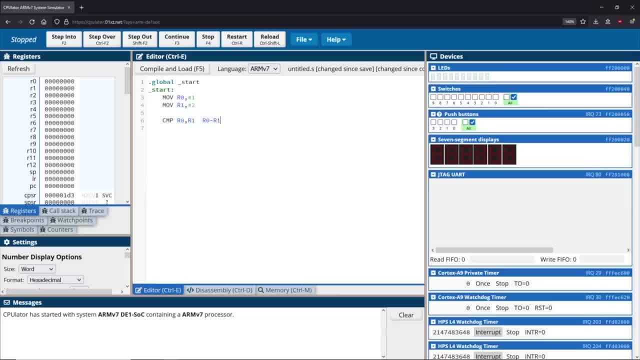 other. Why does it do this? Because this is a way of comparing two values. We know that if R0 is bigger than R1, then the result of this will be some positive number. If our R0 is smaller than our one, the result will be some negative number. And if they're the same as each other, 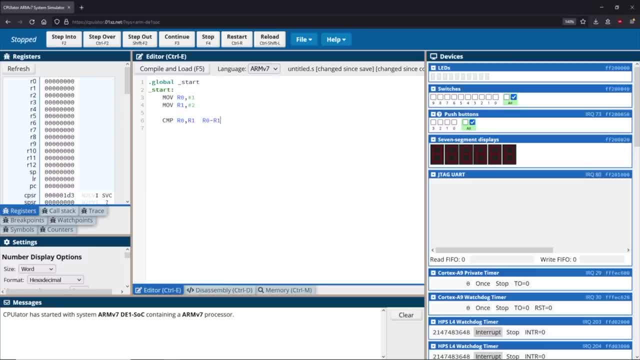 of course the result is going to end up being zero. we can know those three results based on the subtraction of the numbers. So what will happen is the computation for the compare will do this subtraction, And what will happen is the CPSR register- this one right here is going to get set based on the results of the subtraction. 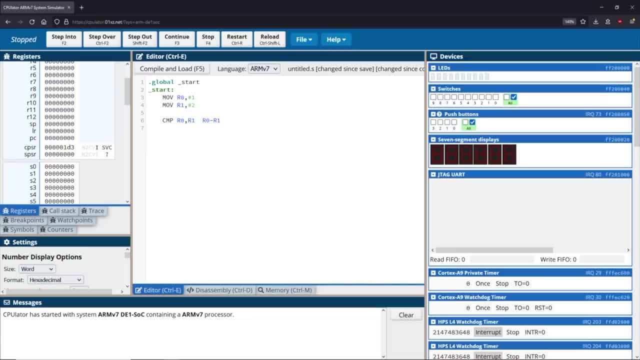 Now, as we've briefly discussed, in the CPSR register we can set different things like negative, zero, carry overflow and these sorts of flags. Well, it turns out that that's very useful for this situation, Because suppose, if we subtract these two numbers- and I want to see if 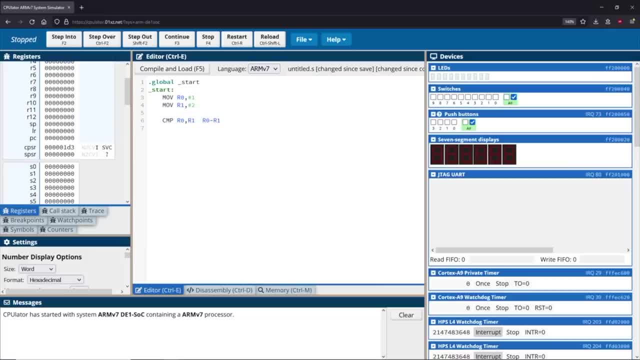 r0 is smaller than r1.. If r0 is smaller than r1, I expect to get some negative number And that would mean that the negative flag should get set in the CPSR register. So you see how all this sort of fits together. we've sort of put the puzzle together and we can see how we can use all of. 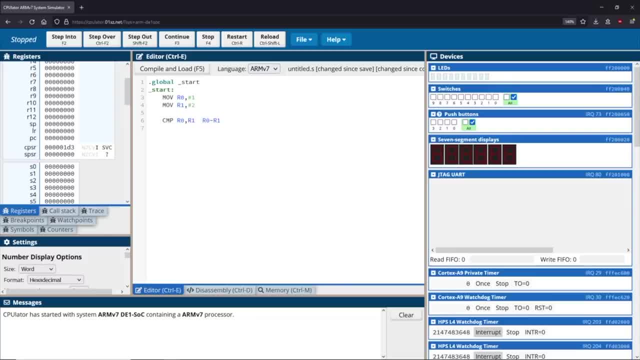 these different pieces to get our conditional statements. So this is a very high level construct that we're able to replicate in assembly. For that matter, we're able to replicate the. this is a very high level construct that we're able to replicate in assembly. For that matter. 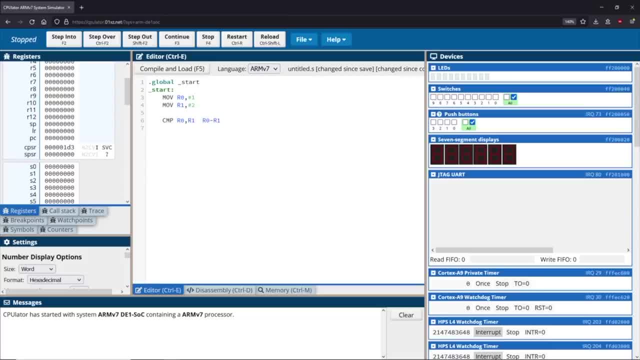 when you compile your high level languages, it's using this sort of idea in the background, maybe not exactly like this, but similar sorts of ideas to this. So, understanding that, what happens after we do this comparison? Well, in this case, maybe we want. 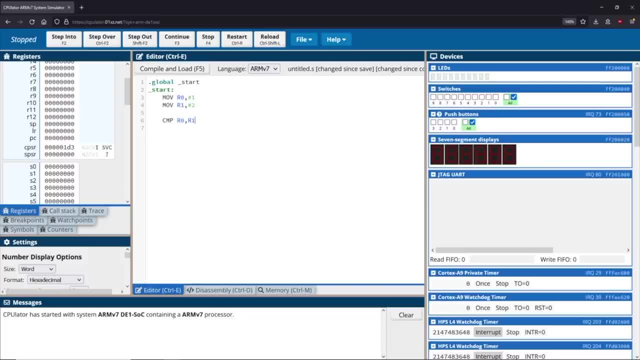 to check to see. if so. let's say, we want to check to see if r0 is bigger than r1. So we want to see if it's greater than r1, what we can do is we can use a branch greater than which is written as bg. 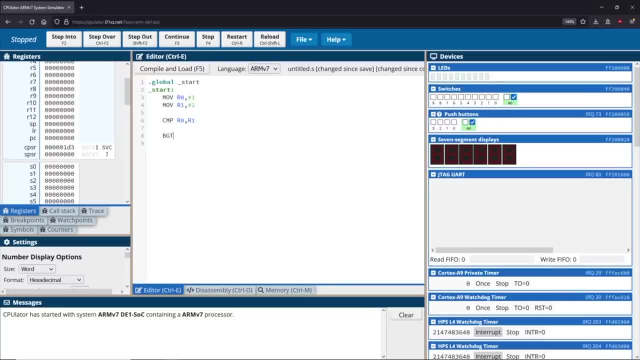 greater than, And then we can get a branch greater than, which is written as bg greater than r1.. t, So it's B is branch, and then GT is greater than, and what we do is we give this a location, and the location is going to be some label, And we did also discuss briefly the idea of 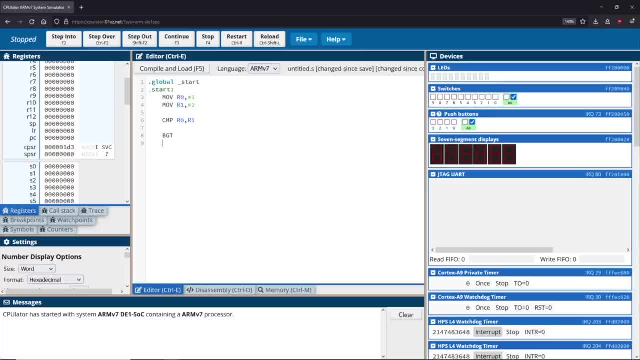 labels. So start is an example of a label, And we can actually add more labels if we would like. So I can add in a label like greater, for instance. this would be the label that will run when the branch greater than occurs. So what I can say is I could say BGT. then 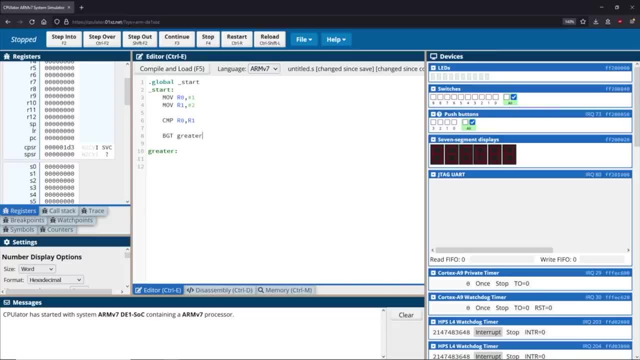 I can see greater. What will happen is, when it does this comparison, if it finds that our zero is bigger than our one, it will move to this greater label and it will start to execute whatever is provided here. So in this case, we'll just do something to see that. 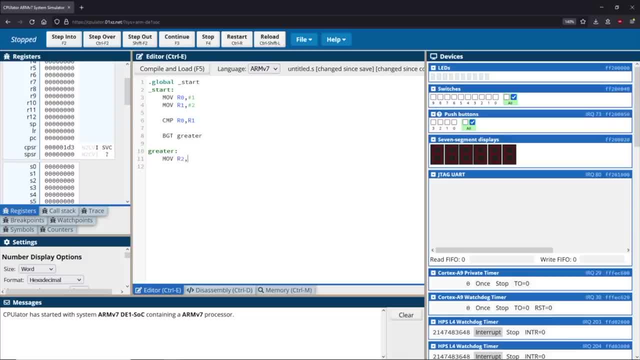 this is working. we'll move the value into our two. So that would be an example of this. Now let's go ahead and run this and just see what ends up happening, So you could see generally that these values actually aren't greater. 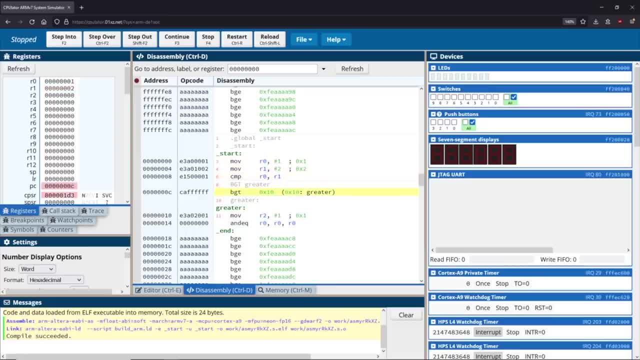 right, Our zero is not greater than our one, which means that we shouldn't actually take this branch here. Now the question is: what happens after if we don't take this branch? And the answer is: we just continue on as if we never actually executed this instruction. 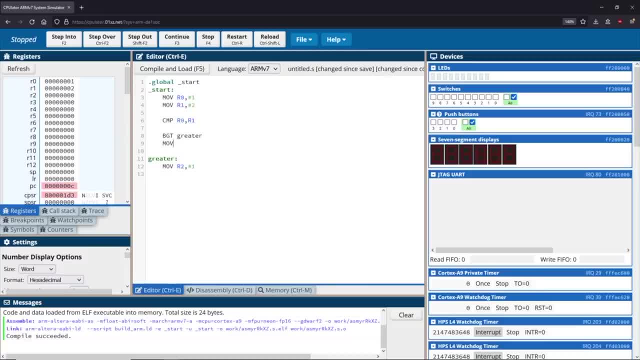 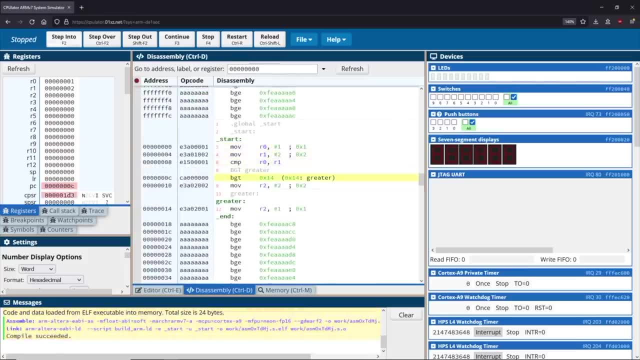 So maybe make this a little bit more clear, Let me add in a move instruction inside of here. So we're going to go ahead and add a move instruction inside of here And then, right, so we can add in this move instruction And we can see that when we do this, the comparison 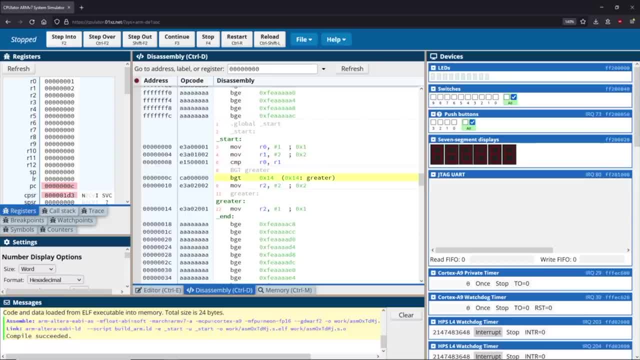 ends up not being a value that's greater. you can see the negative flag is set, indicating that the subtraction was a negative number. When we do this, you see that it skips over this branch and it just moves into the next instruction. So you can see how that generally. 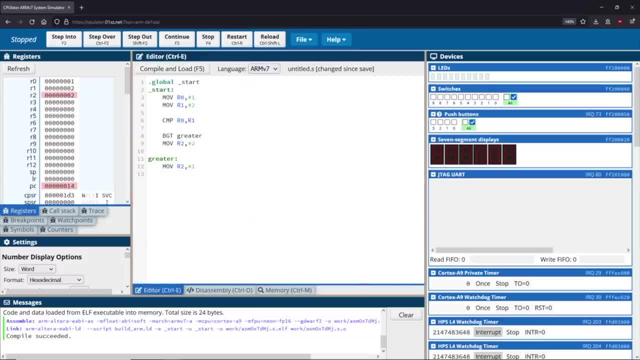 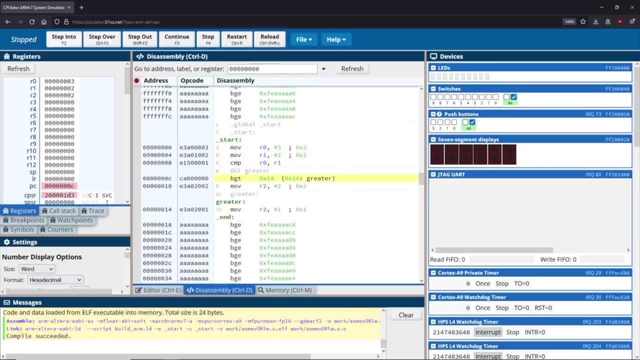 works. Now, if it were greater, right, if I said three, for instance, here and we ran this, what would end up happening is we do our comparison. you see that we don't get a negative number. instead, we actually get a carry And this indicates the value was. 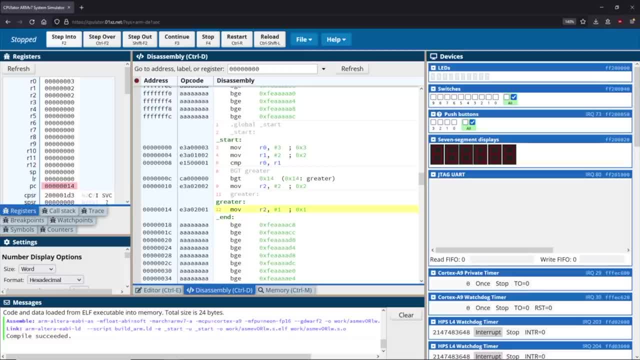 bigger rather than being smaller. you'll see that we can move into this branch for greater than you can see that, rather than moving into this instruction, it skips it and goes to this greater label. So this gives you an idea of what's actually happening with. 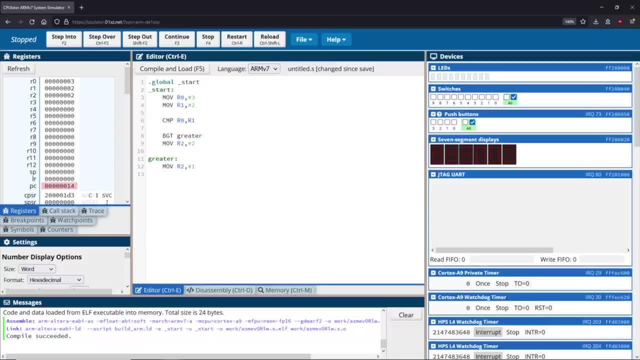 these branches. Now, generally, when we're doing these sorts of instructions, it's important to note the flow of assembly languages. if the value isn't greater than when we have this instruction here, we saw that it moved to this instruction. However, once this instruction 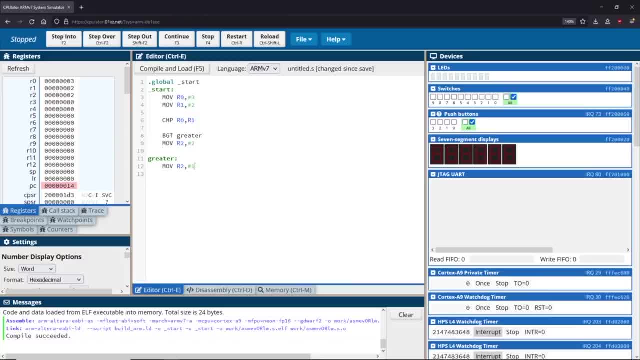 finishes, assembly will continue moving through until it reaches the next instruction, And you can see what ends up happening is we end up in this greater branch anyways, And that is, of course, a problem. We don't like that. What we want to do is we want to skip the 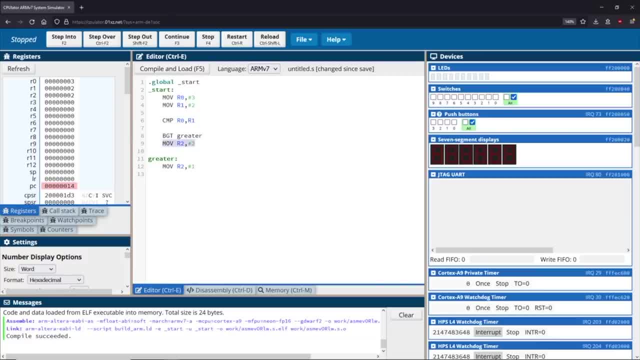 greater branch. we want to make sure that we don't actually reach it if we're not in a greater than that value. To do this, we can use branches as well. So there's a special type of branch called a branch. always be a L, So branch, and then always, And this will 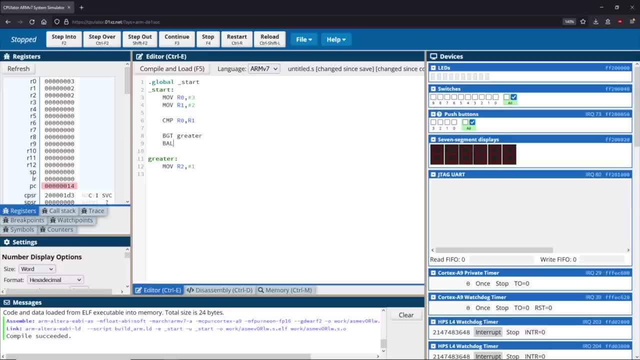 always execute, So we'll always branch this location regardless of what happens. So for B a L, what I could do is I could say, rather than going to greater, I can go to a different one. you know, maybe I'll call this one default, So in this case we can create a default. 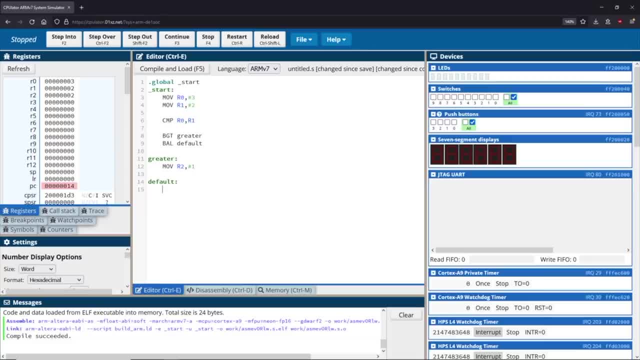 default label And then we could do something here. So I could do the same thing as before. Right, so we move to into our two, And we could see that in this case, if we don't reach this greater branch, we move here and we always branch to default, which skips over. 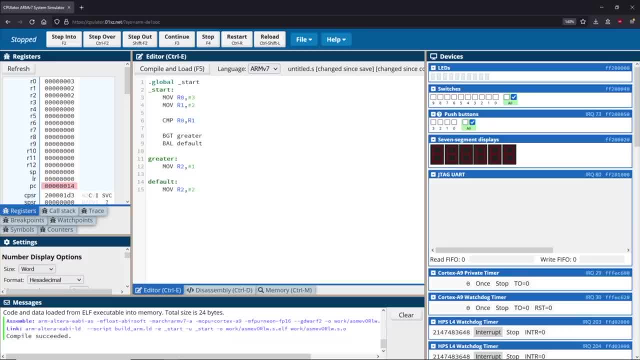 greater and ends up here Instead. this allows us to effectively bypass this greater instruction. Now, another thing that we need to keep in mind here is: once we finish the greater portion right, we would also fall into the default case, So it's just very important to note. 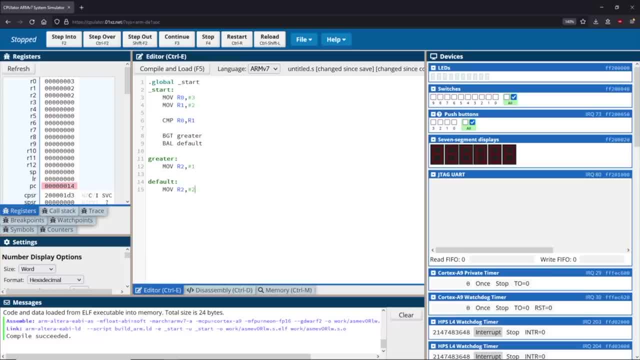 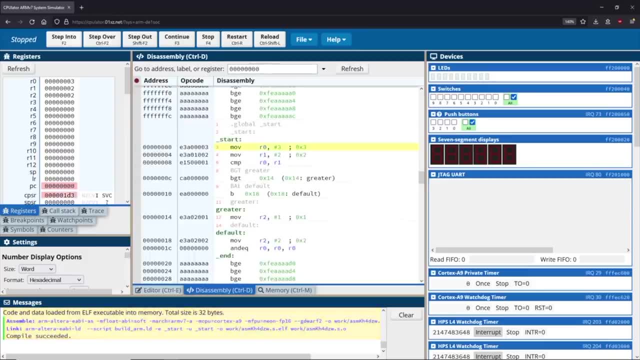 that the instructions are always going to run sequentially. I want you to understand that very clearly, that everything is going to run sequentially here, right, And I can show you this right. So if I compile and load this, we have three, we have two, we 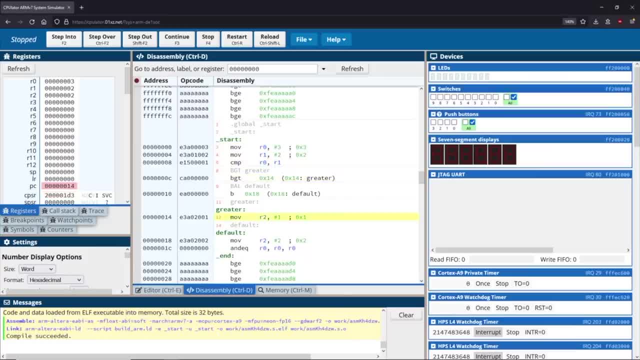 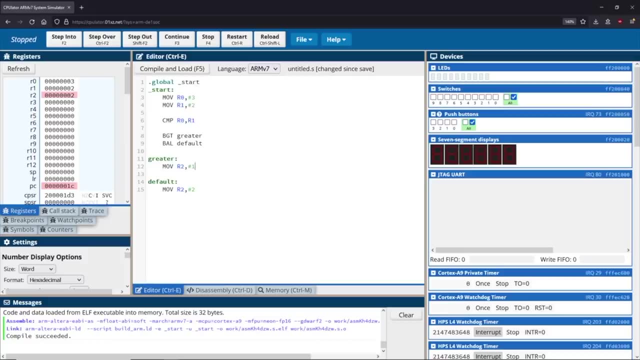 subtract them, we do the branch for greater than we end up in this move instruction, right? So we do this move instruction And you can see that we end up in default next, right, and then it runs that instruction. So it's very important to note that it's always going to move sequentially, right? So if we 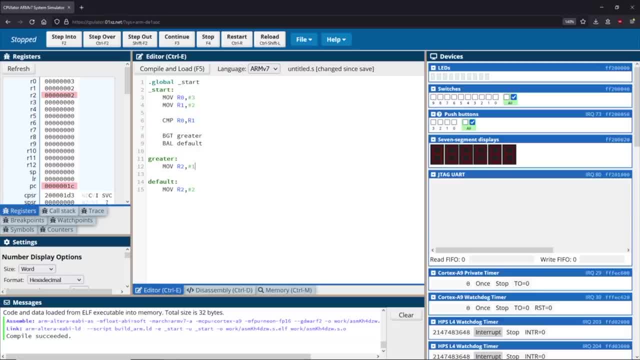 don't want to go into default after greater, I should add in another branch to move somewhere else. So this is just something to keep in mind when you're writing these branches. everything runs sequentially. that can be a little bit tricky, So just be very careful of that Stepping. 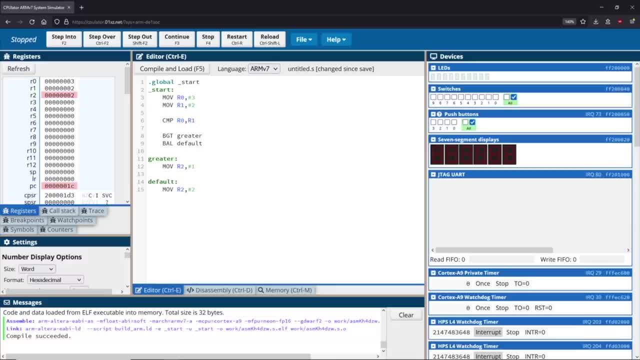 through the programs is going to make it very clear what is going on. you'll understand it completely once you step through a few programs, But just keep that in mind And keep thinking about that as you're writing your code And running it and practicing with it. So this gives you a general idea of the different 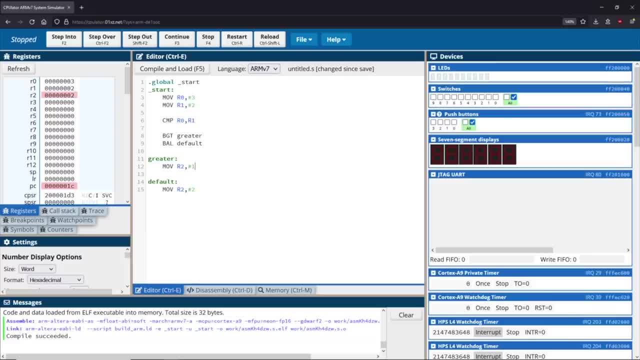 branches and how they generally work in our program. Now, there's, of course, a lot of different branches And I'm not going to like show off every single one of them. are going to have to give out a detail for them. I'll just sort of like lay out a few of them here. 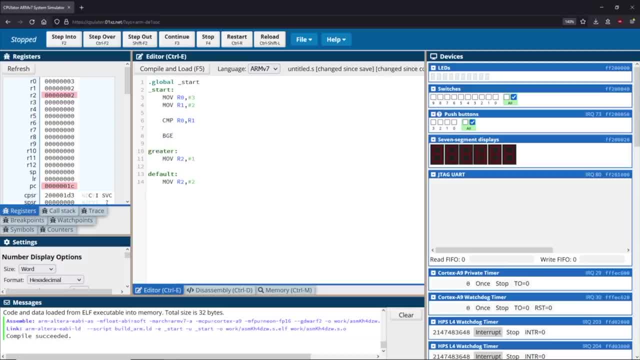 that are common. So if greater than and greater than or equal to, we have less than and less than or equal to, And then we have equals or does not equals. Those are the different branches that we have available to us, And they're fairly intuitive. 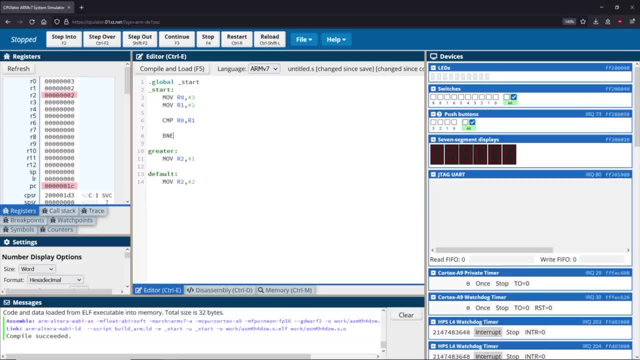 in naming right. EQ equals any, not equals, LT is less than, le is less than or equal to, so on like this. you can get a whole table of these through the arm documentation. there's actually a lot more than the ones that I'm showing here. I'm just showing you the most. 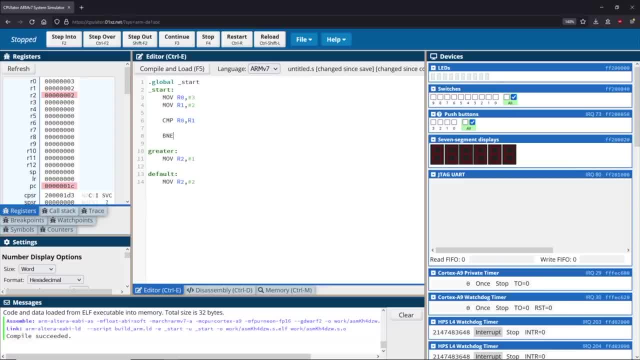 basic ones that will come up most frequently. If you ever find yourself needing a very special branch, it likely exists And you can find that branch in the actual documentation. But this gives you the main overall picture of what branches are commonly used. how do we? 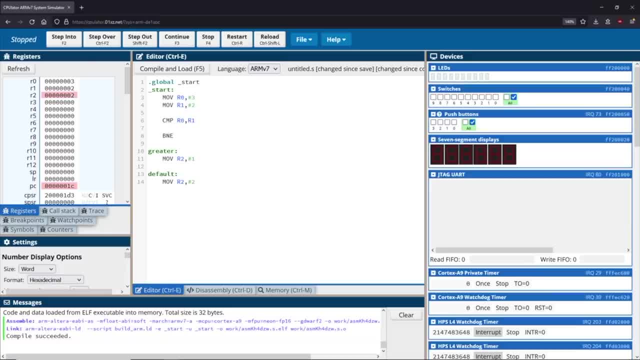 use branches and what is the effect of using the branches. So that's everything for this video. In the next video, we're going to see some applications of branching in the form of looping. So branches allow us to implement looping and repetition as well. So we're going. 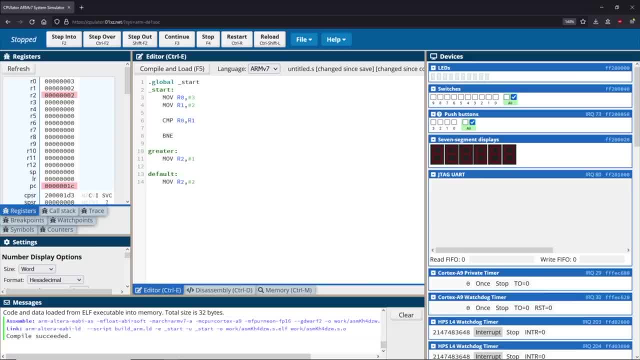 to take a look at this sort of concept and be able to build some interesting applications and hopefully help you understand this idea of conditionals and branching a little bit more. In this video we're going to take a look at some of the applications that we're going. 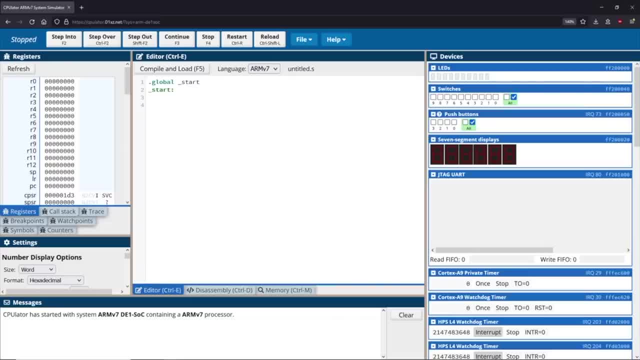 to talk a little bit about looping as a consequence of the conditional statements that we learned in the previous video. When we discuss the idea of conditional statements, one of the big benefits that we can get out of them is the ability to repeat instructions, Of course. 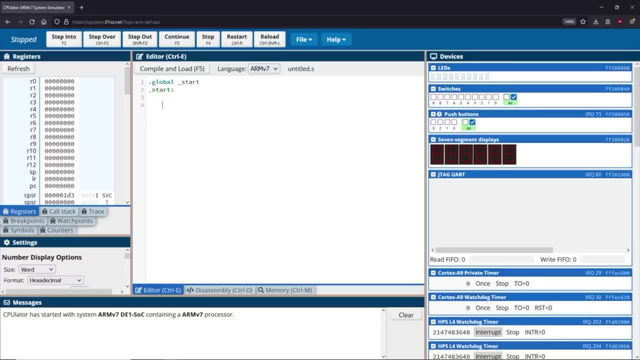 if we could branch to a specific label. we can always move back to a specific starting point and repeat instructions, And we can always exit that repetition using a comparison and some form of branching as you would with like a for loop or a while. 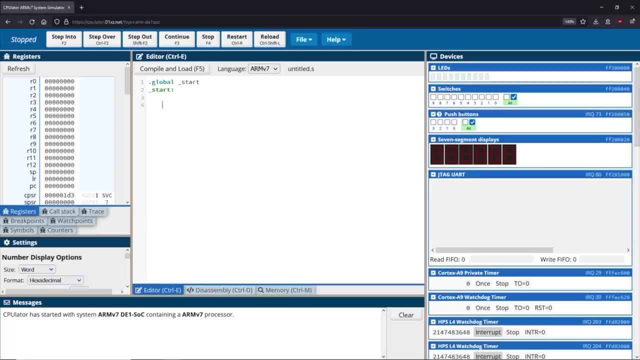 And, as Sy bastard mentioned, paradigms are arbitrary and floaties, Spring and loop don't refer to ourselves. so we have arguments that can get才ticed, For example lingio, and also in the case of Noble root linear mechanicsabadier. when I say linear linear, I'm talking the normal. sense of what I'm describing. There's number of terms, but I do want to explain what you're referring to here. First of all, let's briefly think about looping as employees of furniture, It can be anything which we like and receive orders from. like these times they call these. 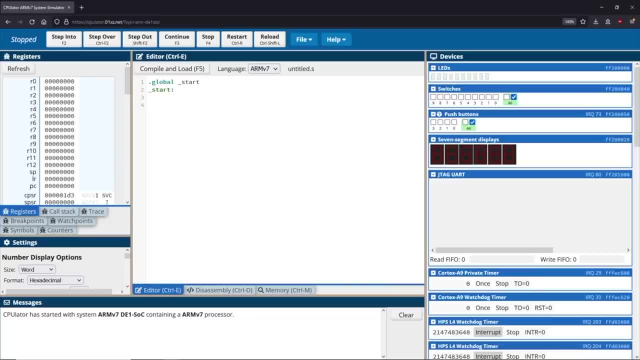 loops. We always do. This is important, boss, right? All right. first of all, there's structural. refresh your knowledge and apply some of these instructions in a more practical way. What I'm going to do is I'm going to start off by defining a list of numbers. 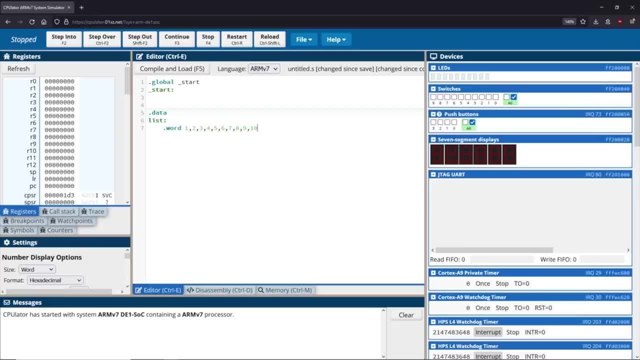 And this number list is just like all the numbers from one to 10.. So something very simple for us, And what we're going to do is we're going to load this list into memory And we're going to try to iterate the list. So the first few parts of that is fairly simple, right? We're going to load the. 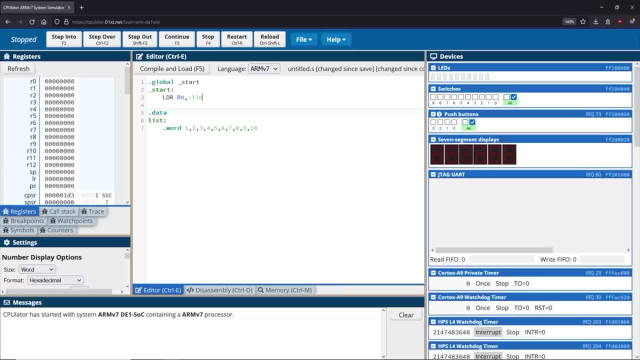 list into memory using LDR. So that part is it's no big deal. And then what I'm going to do is I'm going to start by loading the first element into my, into my memory. I'm going to use our one to store the elements of the list, And what I'm going to do is I'm going to add up all of the numbers. 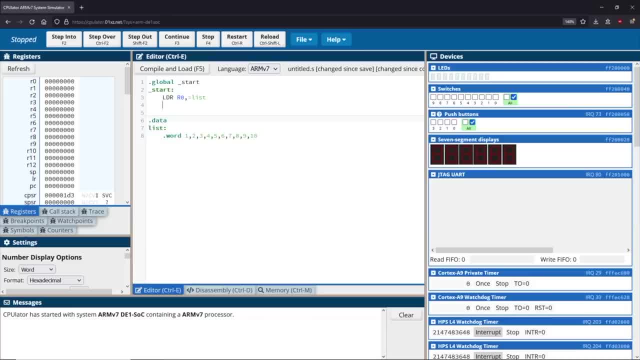 inside of the list And I'm going to store that result in our two sets- sort of the main idea of our program. So let's go ahead and do that. We'll start by loading the value of the first value of the list into our 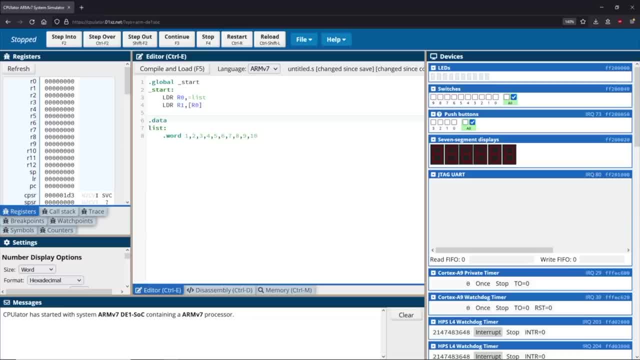 one. Of course we use that using addressing based on the address that was placed inside of our zero, And then we can do the addition to add that first value into our two to sort of like initialize everything right. So that gives us sort of like an initialization And then we can actually start to talk about the 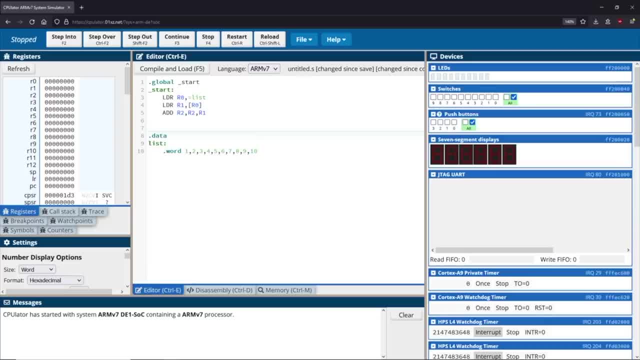 looping portion of this. So this starts up the list. So what we've done so far is we've sort of set to the the first value of our sum equal to the first value in the list, And then what we're going to do is we're going to iterate. 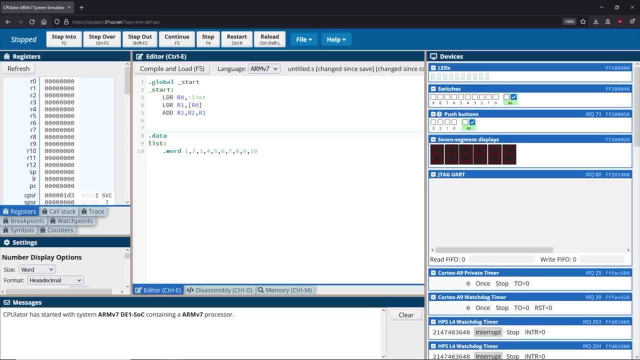 past that point and add those values onto that are to register till we've reached the end of the list. This creates an interesting concept, right? How do we find the end of the list? Well, let's take a look at what our list looks like in memory. going to go ahead and compile and just step into 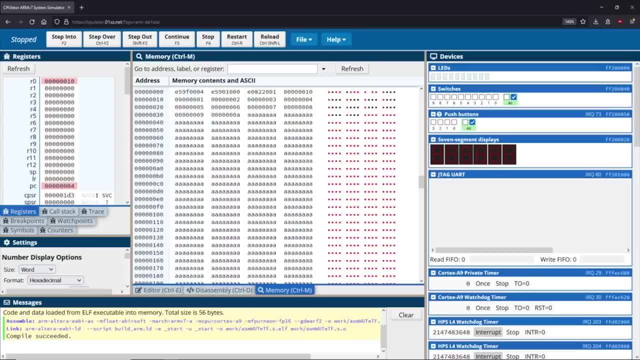 it to find the location on my list. It's at location 10. In memory and we could see it right here. You see all the numbers from one to 10. And then afterwards we get all of these A's repeated. 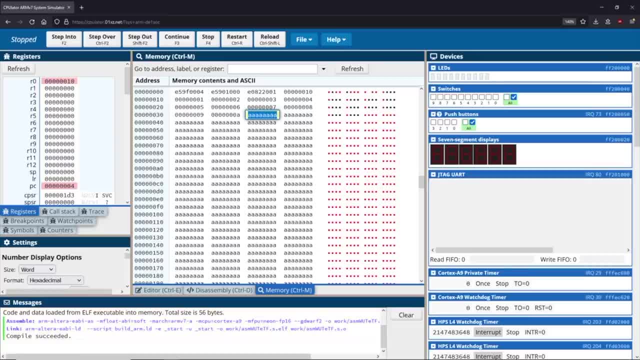 Now it turns out in the case of my memory I have all A's as a representation of an empty slot in memory. So it goes to serve that if we have this set of A's, we've reached the end of the list. So 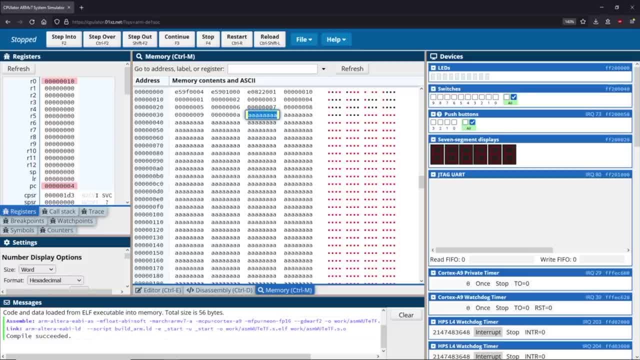 I'm going to continue to move through the list, iterating, until I reach something that is equal to this. Now, how we do that check is actually a little bit complicated. We actually have to do something sort of interesting here Now when we work with. 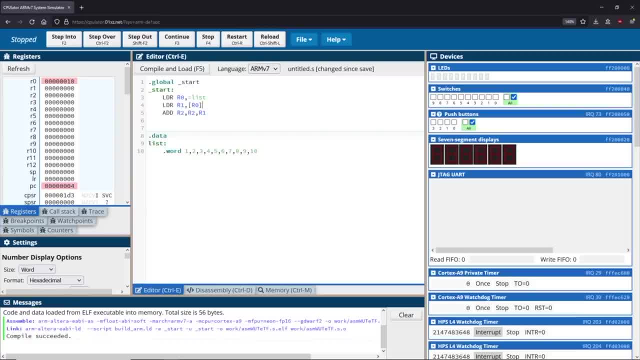 assembly. you might think, Okay, well, that's easy, I can just compare, you know that value and then we'll be done. But the way that assembly- specifically arm assembly- handles literals is a little bit weird. So when we have those immediate values or literals, they can only be a specific 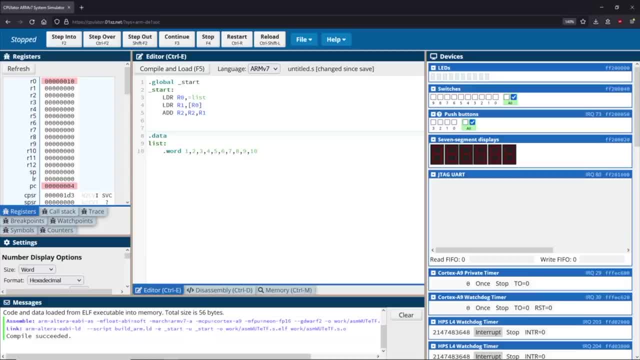 size And above that size is typically two hex values. So if we have something bigger than two hex values, we have to be a little bit more creative with how we deal with this, And the main way that we're going to deal with this is we're going to use constants, And constants isn't something that. 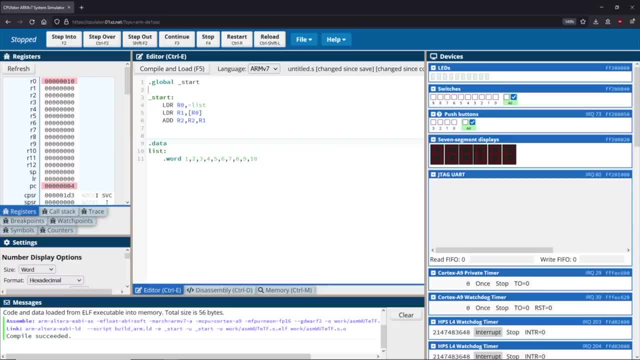 we've really talked about so far, but they're very simple. At the very top of our program, we're going to define our constant using a keyword that is dot, eq u, So eq u, like this, Similar to defining our list. we're going to give this a name and a value. 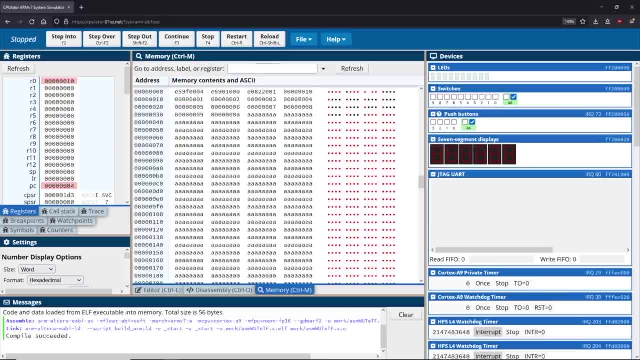 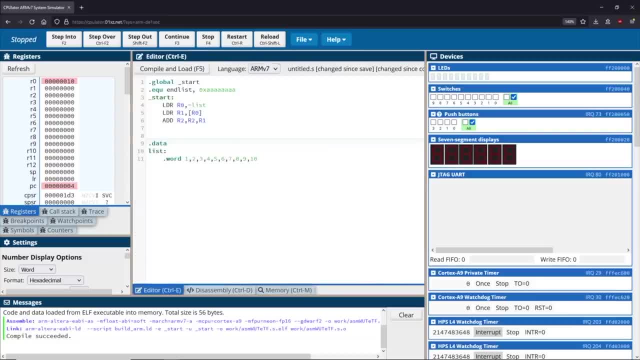 And I'm just going to go ahead and copy it because I don't want to mess it up here. So just copy this over, I'll place that there, And there you have it. that is our constant defined. So this defines a constant called endless, and it gives it a value, which is this: 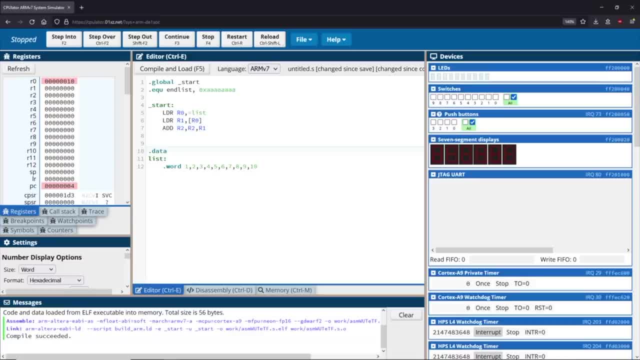 value here And then we can load this into memory using an LDR, like we've done with the, with the list loading it. it's going to load this into our three, just have it available to us. So there, we have this value now loaded into our three And now we can actually do our loop. So 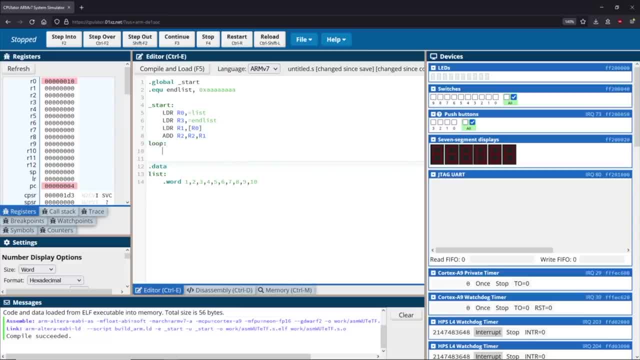 I'm gonna start by creating a label for our loop, And what our loop is going to do is it's going to load the next value in the list. So what this will do is it will increment by four and then it will load the value of that address into our one, And then it's going to take a look at the 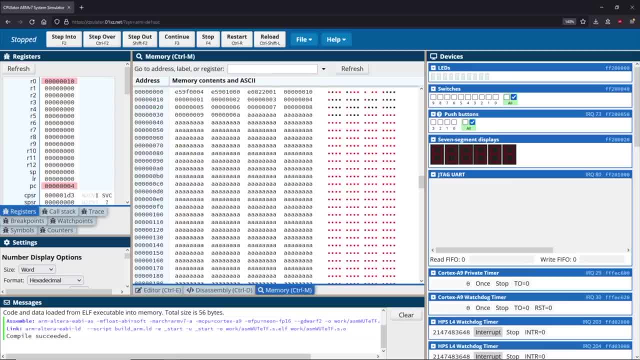 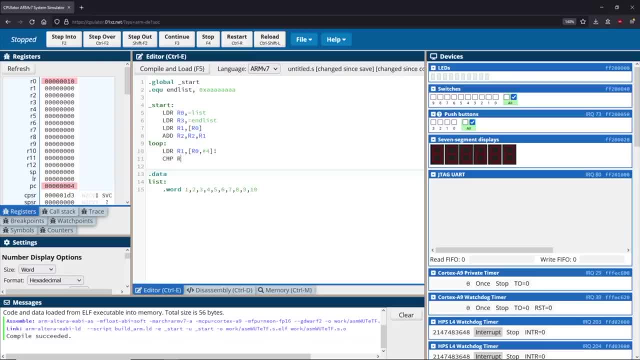 this value and see if it is equal to that location and memory that is empty. So this, all these A's here. So remember we start that at r3.. So we're going to compare r1 to r3.. If those are equal to, 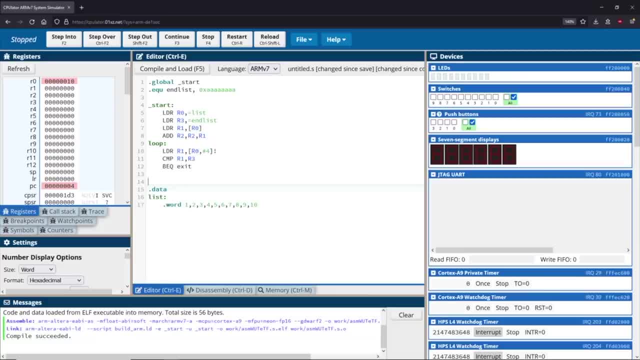 each other. we want to leave the loop. So I'm going to say bq exit. I'm going to put a label exit here. The label exit isn't going to do anything, it's just going to be the exit point of this loop. Alternatively, if we have not reached the end of the list, what I'm going to? 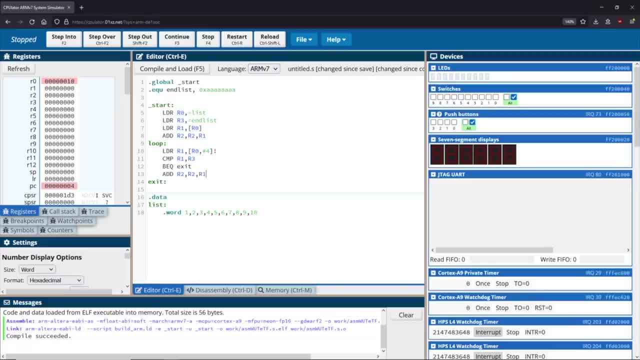 do is I'm going to add the value into r2.. And then I'm going to loop again, So I'm going to branch to the top of the loop. So, to understand this, what's going to happen is it's going to load the next. 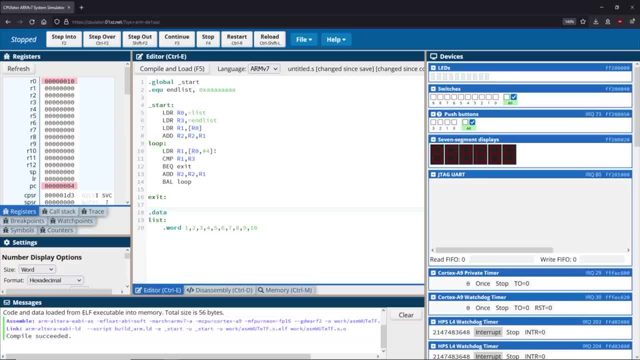 value in the list, If that value is equal to the end of the list- so this set of memory- that sort of- is uninitialized- then we're going to go to the exit. Otherwise we're going to add that value to the total And then we're going to loop again. Now, this isn't the only way that we. 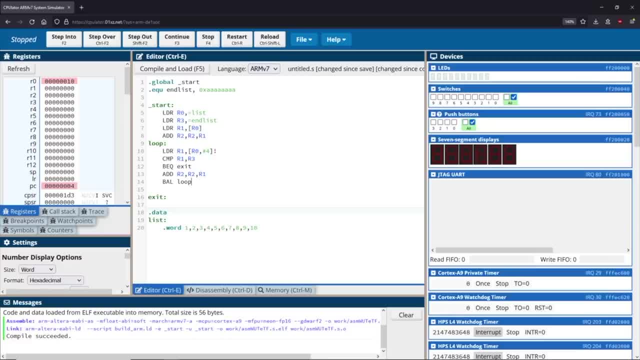 could find the end of the list. we could know the length of the list. that could be another way that we might be able to do this, And there are likely other tricks that work in assembly to be able to do this. However, mostly when we have the length of the list, it makes things a little bit easier. 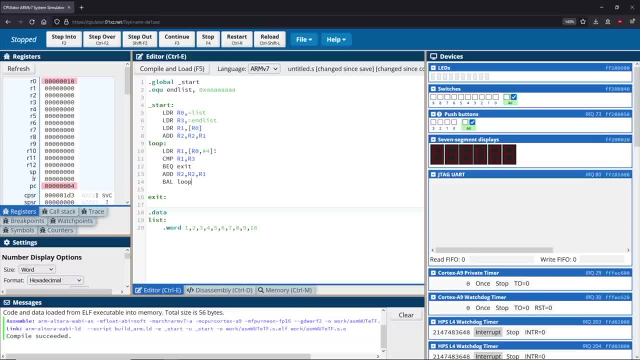 for us to be able to do. There's an interesting idea of uninitialized memory. it can be a little bit unpredictable, right? We don't necessarily know that these values are going to be stored this way, So we're going to add that value to the total and then we're going to loop again. 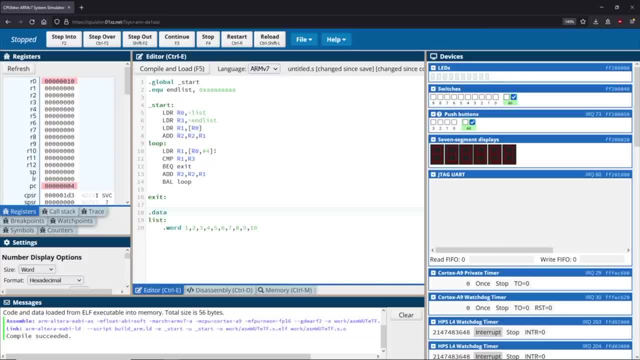 So the way that I'm doing it right now is a simple example that's going to demonstrate to you the idea of looping In the real world. when we're doing this, it's a little bit more complicated. what we would end up doing is we would end up putting a special value at the end. 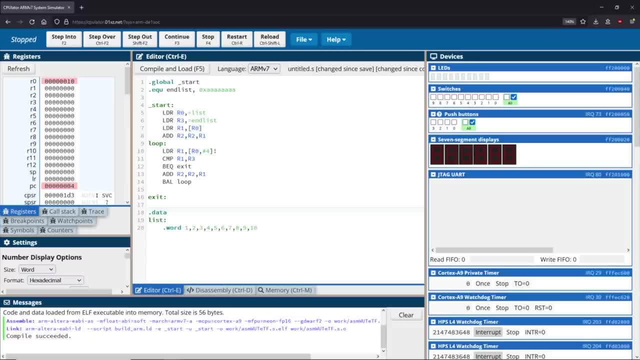 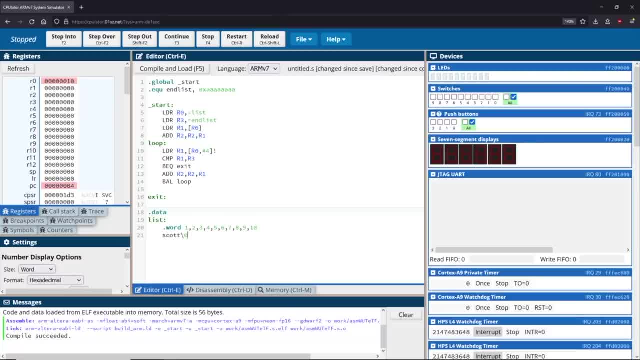 C programming, you'll know that characters and strings have a special value at the end of it, And it's this backslash zero character. it's called the null terminator. What this is doing is it's indicating the end of the list. So when we iterate, we know where to stop. So that's just to. 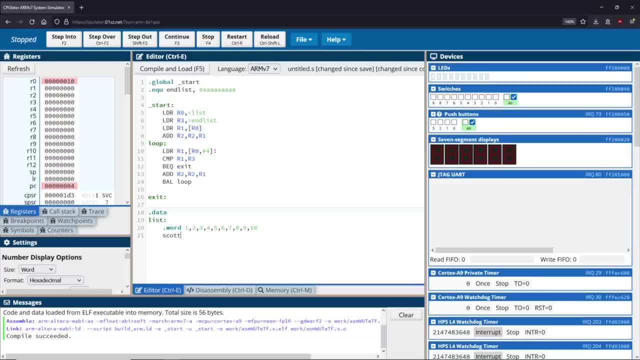 give you a bit more of a practical idea of how we do this. But for now we'll assume that we're in this perfect world where uninitialized memory stays put And we don't have to worry about that. But just in case you're curious about that, that would be the way that we would usually handle. 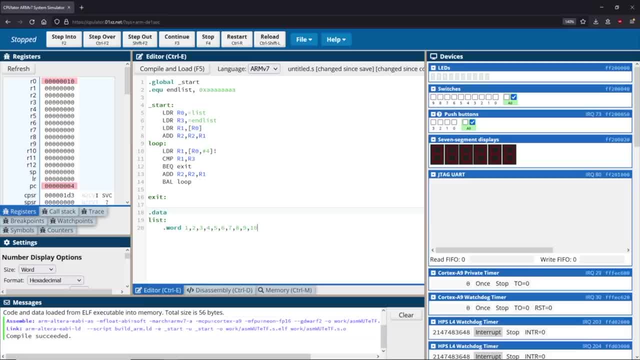 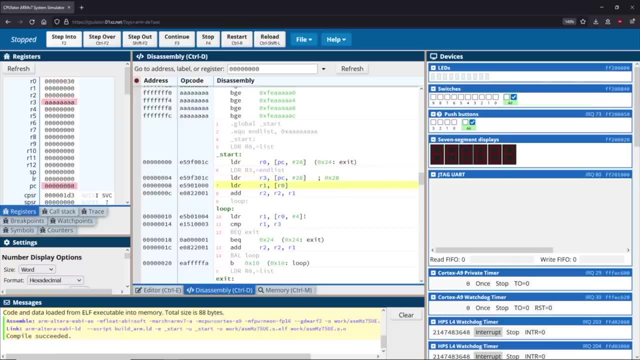 this sort of idea. So with that out of the way, let's just talk about what this program does. Let's go ahead and execute it So you can see that we get the location into memory. we then load in that end location so we can check for it. We then start by loading the first value, which is: 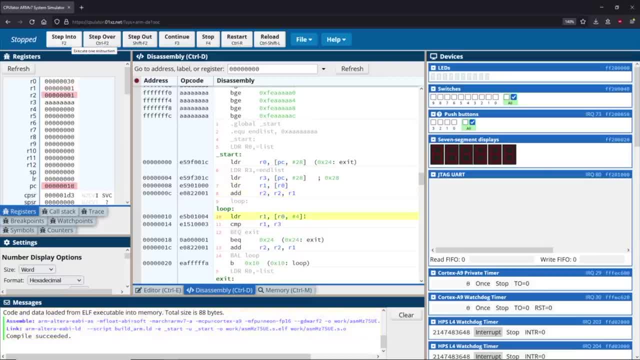 the value one and we add that onto the total. Now we get into the looping So you can see the next value is two. we check if that's the end of the list. it's not, So we add that value to the. 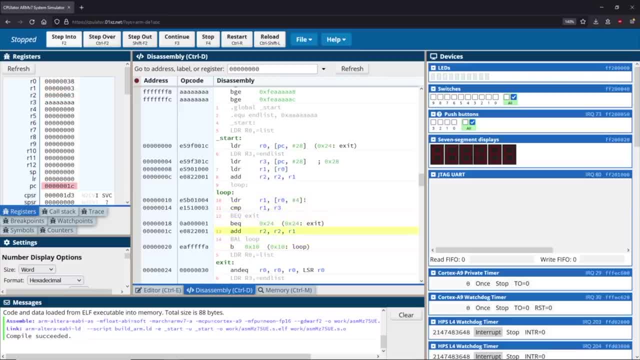 total, And then we go back to the top, And then we continue doing that, And you'll see that this continues on For a while, right? So we're gonna do this for every single value inside of the list. it will just keep looping through right, right, seven, eight, nine and 10.. And once you reach 10, you'll 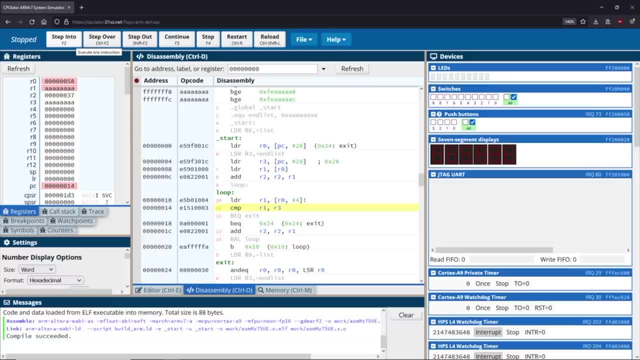 see that the next value is going to be that end of the list of the A's there. So at this point we compare them, we see that they are equal to each other And you see that it skips us out to the exit rather than adding it to the total and the looping again. So at this point we've exited the. 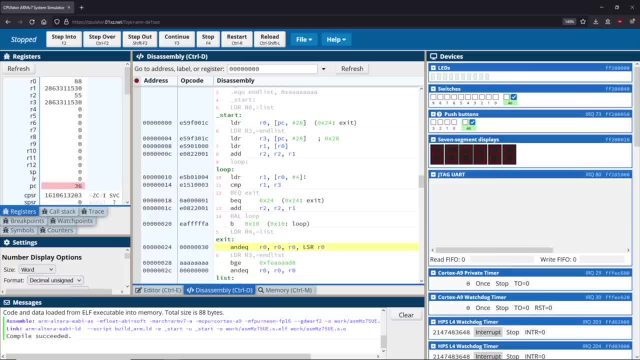 loop. everything is done. we've iterated the list And you can see that the value that we got at the end was 55, which is the value of adding one to 10 inclusive, And that's the way that we set up our loops. So, using this sort of concept, you could do. 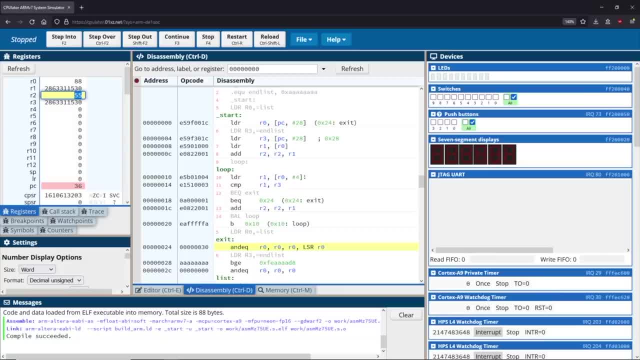 all sorts of different loops you could do for loops, you can do while loops, And you know you're able to sort of expand your knowledge from here. this gives you the basic fundamentals. it shows you how you can use the branching for the loops And from here you can apply this in many different 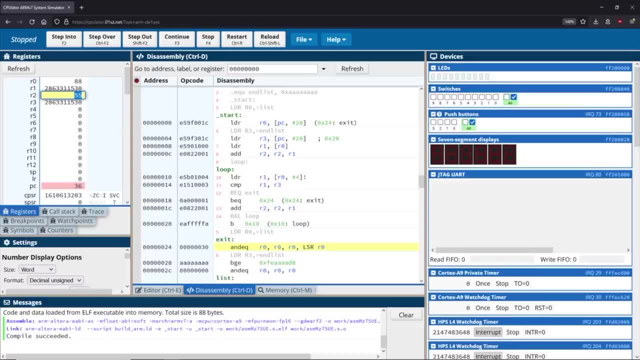 ways whenever looping is actually required. So that's everything for this video And the next few videos. we'll take a look at some other instructions that we're able to use related to this idea of sort of structuring our program through conditionals and looping, and see different ways. 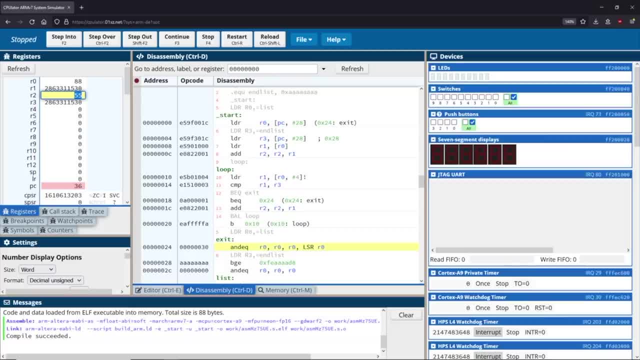 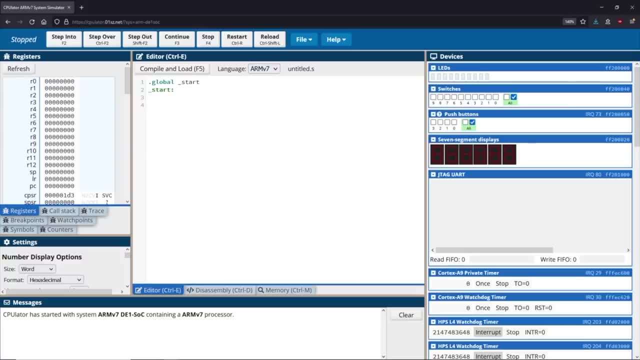 that we can manage this sort of idea. So in this video, we're just going to discuss some of the fundamentals of conditional instructions. Now, conditional instructions allow us to be able to complete a specific instruction based on a condition So similar to the comparisons that we 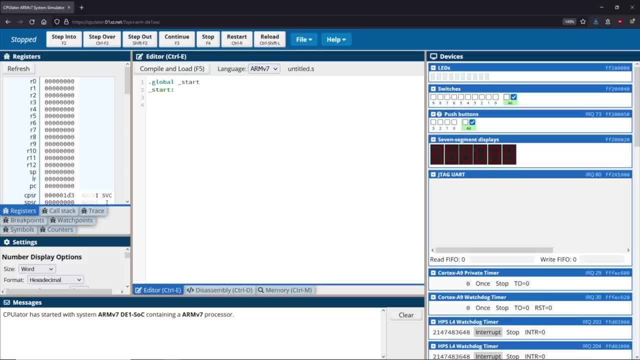 saw with branching, we're going to be able to do a bunch of different things, So we're going to do a bunch of different branches. what we're able to do is we're able to do a comparison and then specify to do another operation based on the result of that comparison, without the need to branch. 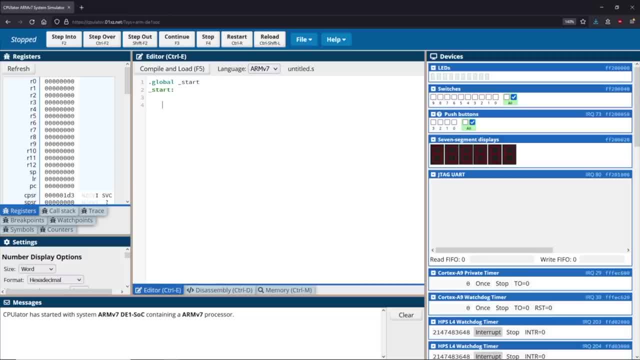 around the program or do anything complicated like that. So it allows us to create a more condensed form of our branching exercises that we were looking at in the previous few videos. So let's discuss a little bit about this with an example. So suppose that I were to move some values. 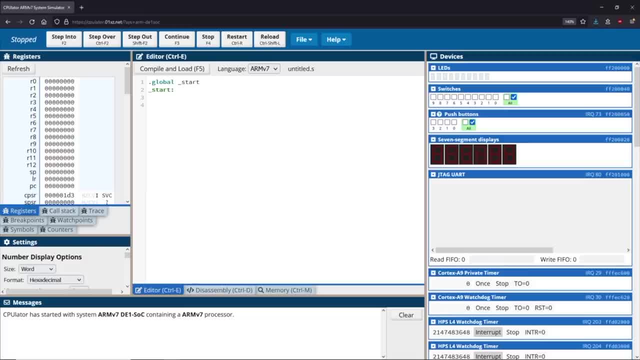 into registers. so we'll just move some random values- doesn't really matter what they are. So I'll move to into our zero and maybe we'll move forward to our one. No, we'll do is we'll compare our zero and our one. 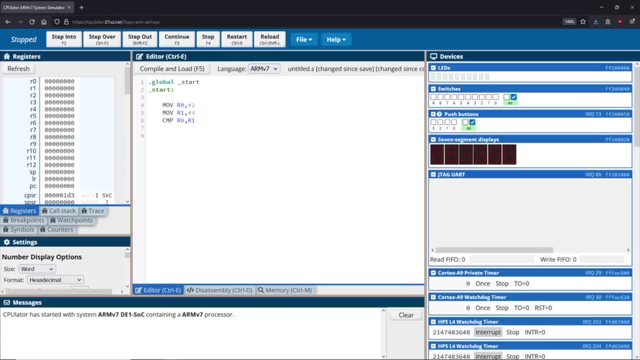 And of course, we know that the result of this comparison is that our zero is less than our one right, Because if we subtract two from four, we get a negative number. Now, in this case, maybe I want to add one to register two. 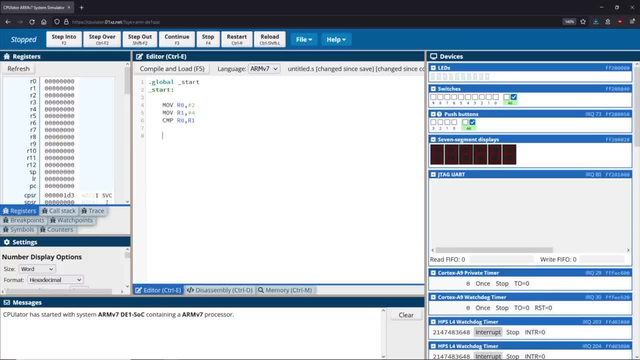 If the result of this was actually less than if we wanted to do this in the previous videos with the knowledge that we had, what we would do is we would do something like this. we would say, okay, we would branch less than. we could call it like add our two, and then we would have like an add our. 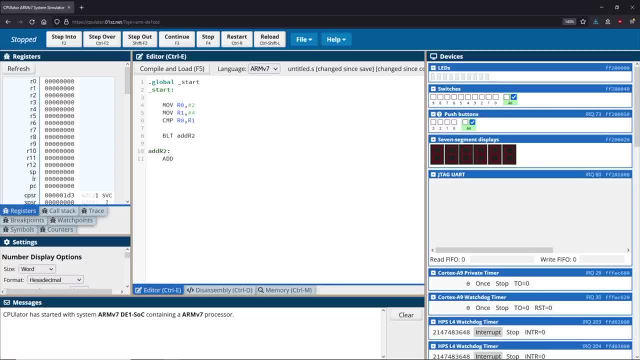 two, that would do exactly that. it would add to the register our to the value one right. So that would be the idea of what we could do in order to achieve that effect, And then we would have to have a branch over here to skip over it. just in case you know, we didn't actually want to do. 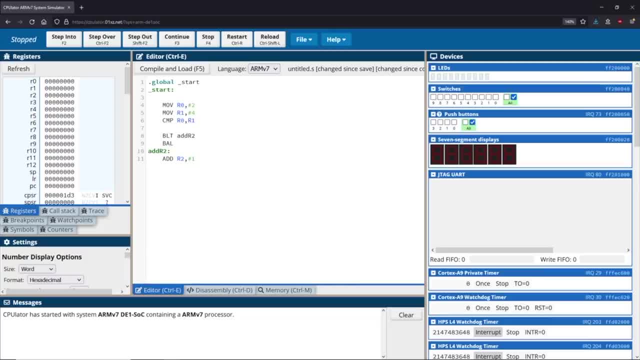 that right, just in case it wasn't less than then we could skip over it and say, like, maybe skip over to like an exit, And that would be, you know, over here. So this would be the way that we would. 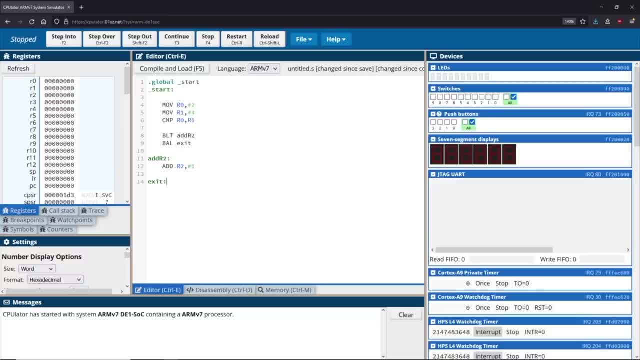 have done this before with just branches, right, And this is not bad. But there's a lot of lines of code for this specific instruction And really it doesn't require as much like of this code as what we really want, Right? So we can condense this a little bit more using these conditional instructions. 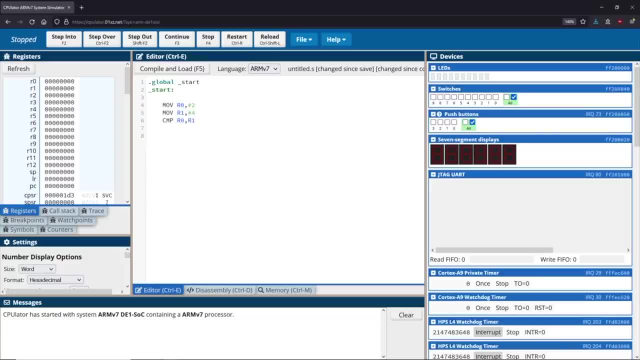 So the way that these conditional instructions work is that with things like add, you can add on a condition. So I can say, add LT. what that means is add less than. So what will happen is this instruction will only trigger if the comparison that came previous is less than. 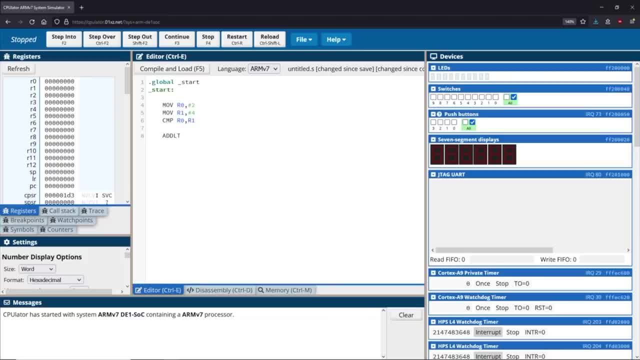 so if r zero is less than r one in this case, then we will do this addition instruction. So, like I was saying before, we'll try adding one to r two And let's just see what ends up happening. right, So we can compile and load. we see that we get two and four into those registers When. 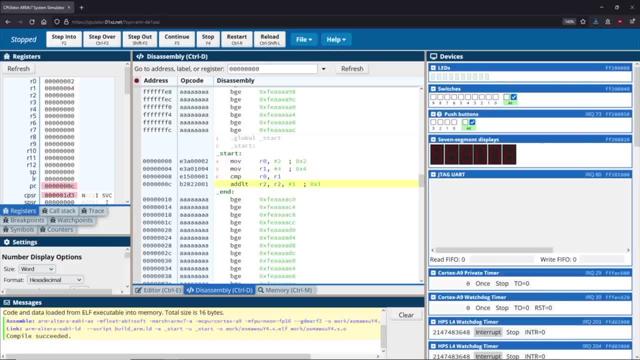 we do our comparison, you see that the negative flag gets set in the CPSR register. That tells us that the value was less than right. so two is less than four. And now we come up to this add instruction: and it should only add one to r two if the value of the previous comparison was. 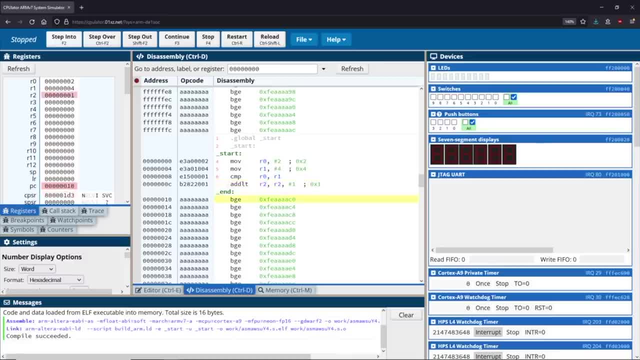 less than see that it does add one because the value was less than So. you can see that generally, this is how this instruction tends to work right, And there are other variations of this instruction. It's not just add that we can do this with. we could do this with a lot of the. 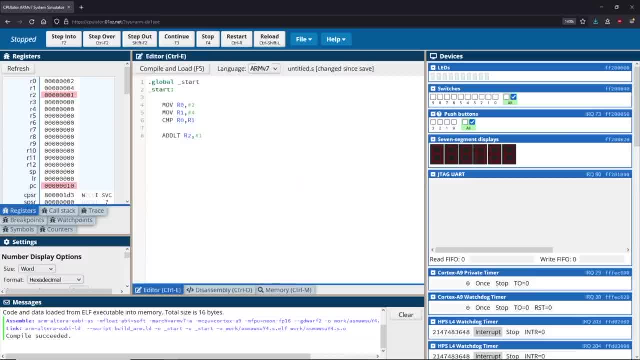 different instructions in arm. So there's things like like subtraction and multiplication. we could do with the move instruction as well. So just to give you like another example, we could do something like this: like move greater than or equal to the value five into r two. 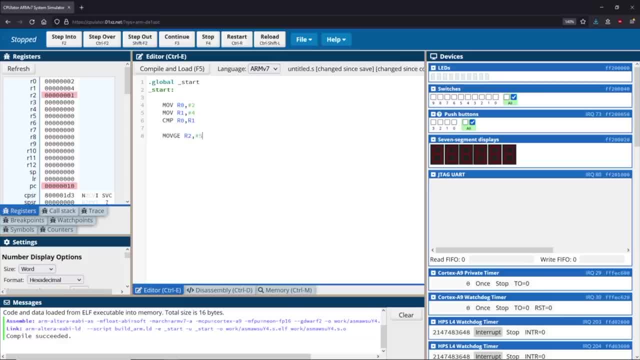 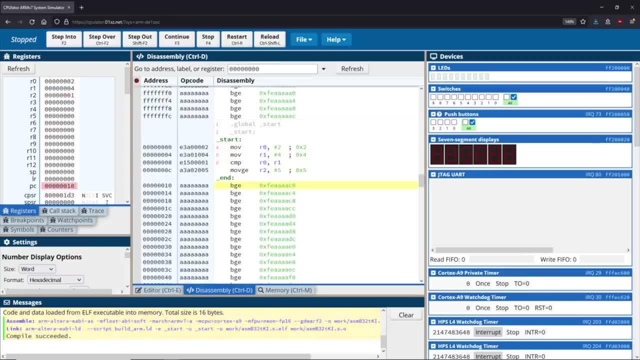 Right. This will only trigger if the value is greater than or equal. So you could see, when we run this and we go through our instructions, it doesn't actually do anything because the value was not greater than or equal. So the move instruction doesn't execute. So that'd be an. 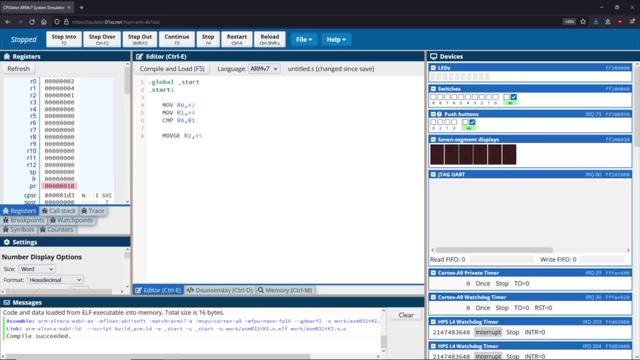 example of you know whether it will execute or not, And of course we can flip this around to be able to get it to execute. There's two different ways to do that. we can move a bigger number to r zero, or we can flip this comparison right? 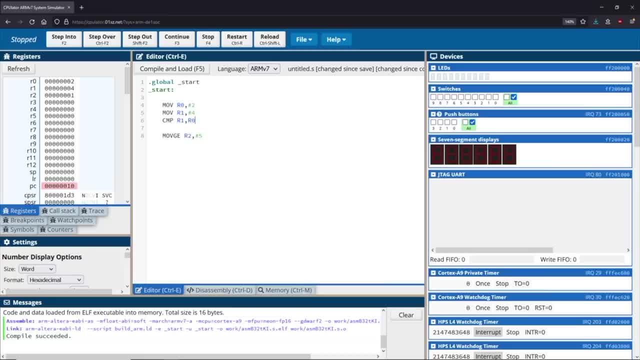 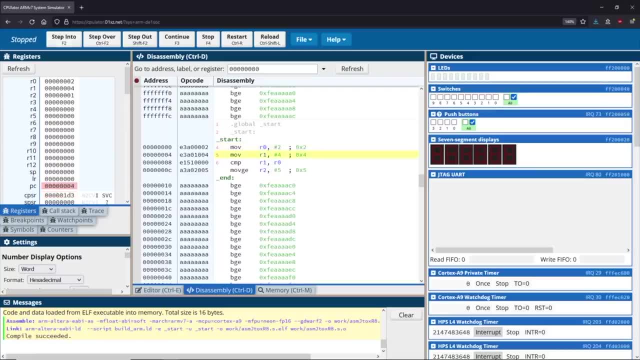 That flip this comparison. it now does r one minus r zero, So four minus two, that's a greater than or equal to value, And when we run this now, you'll see that we get to four. you know we do the comparison. 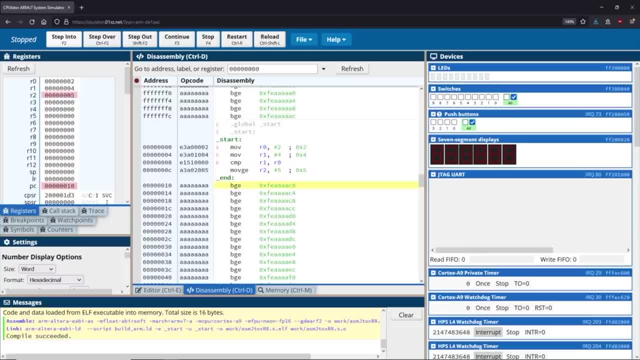 you can see the results in the CPSR register will result in it moving five in, because the result was greater than or equal to. So I just wanted to give you an idea of these sorts of instructions, just to show that they exist in assembly, just to be able to make your code a little bit more simple. 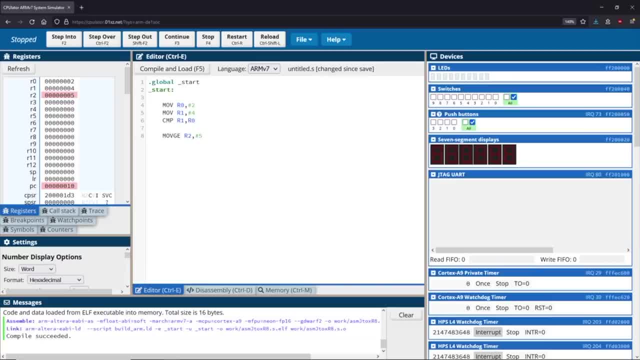 Because having to run branches all the time is very complex. we don't want to have to do that every single time, So this allows us to reduce the complexity of our applications overall. it just writes simpler code. So that's everything for this video. In the next video we're going to 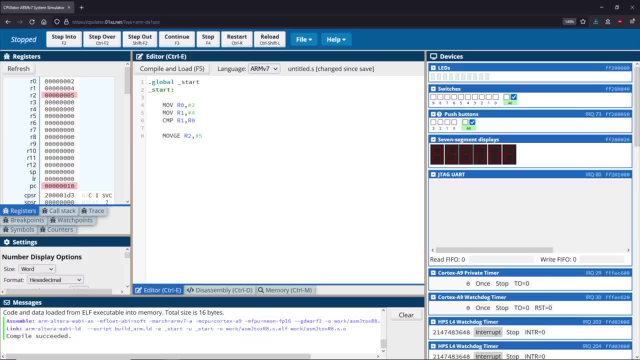 dive into the idea of functions, which are a bit more of a complicated way of doing branching. But, as you probably know, core to most higher level languages is the idea of a function, So we'll dive into more detail to get an understanding of how functions actually work at a 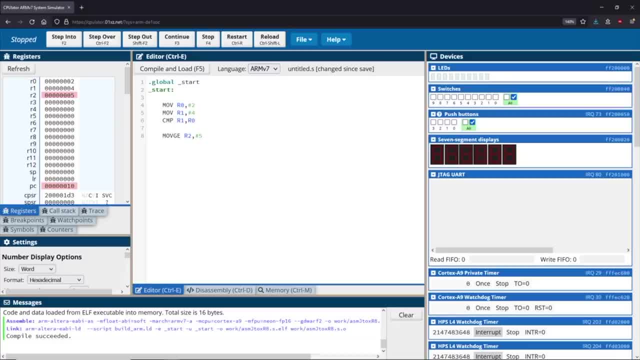 level perspective and get some familiarity with writing. functions with arm assembly. So in this video we're going to start to discuss the idea of functions in assembly And specifically we're just going to take a look at how we can call and return to a location using 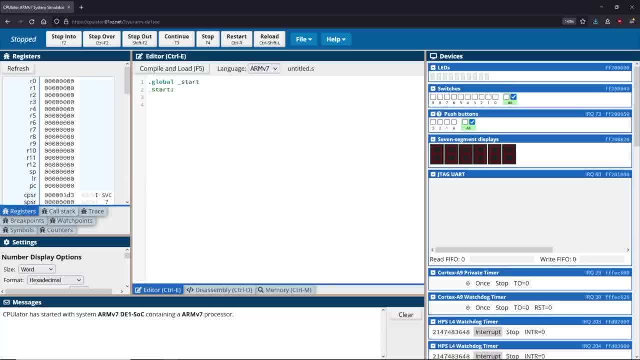 these functions, So we're not going to dive into a huge amount of detail. I want to give you sort of the higher level functional flow of things, And the purpose of doing this is that well, functions tend to be very complicated. A lot of people approach this by showing you the 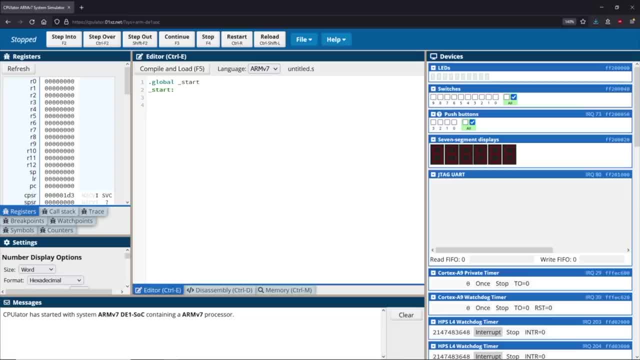 full picture immediately And we start getting into all these complicated register interactions and it's very hard to understand. So I want to break it down into smaller pieces that it's a lot easier for you to be able to grasp every single individual concept, And then we can put it all. 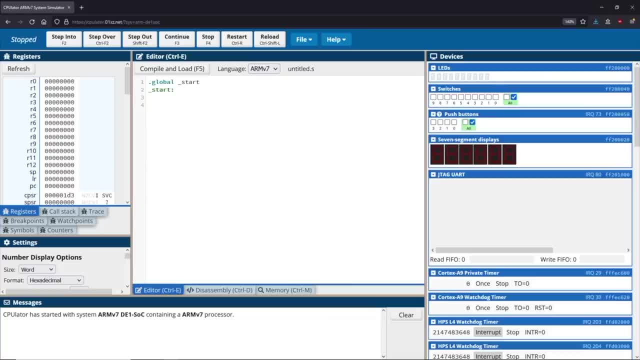 together and really run with it and see how things are working with a full example. So to start off with, we already know sort of the base fundamental ideas of calling different locations in our program right, moving around to different labels in our application. So let me give you a really simple example. suppose that we wanted to create a 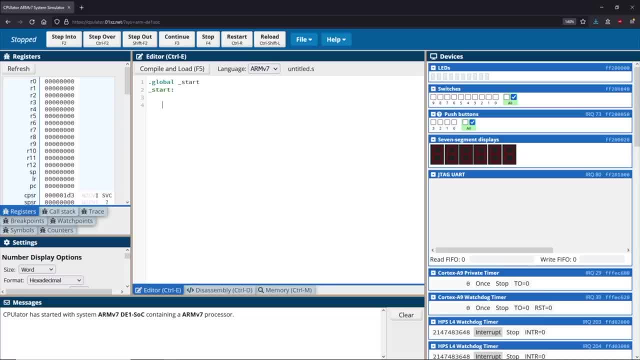 program that added two numbers together, And we wanted that to be a function, because maybe we might do it multiple times throughout our program. Well, in order to do this, we're going to go ahead and start by moving some values into some registers that we want to be. 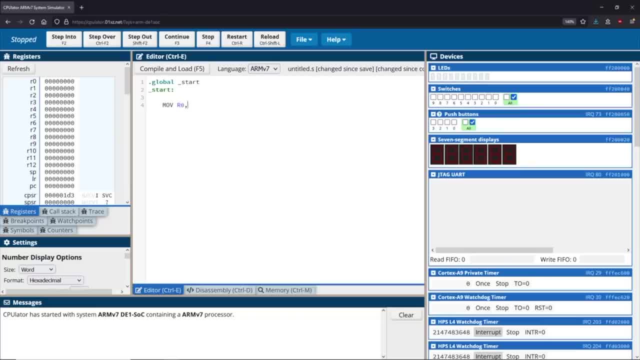 added And really you can make these values whatever you want. I'll just move into r0 and r1.. And then what I'm going to do is I'm going to branch off to a function that's going to add the numbers together and we're going to call that add to. 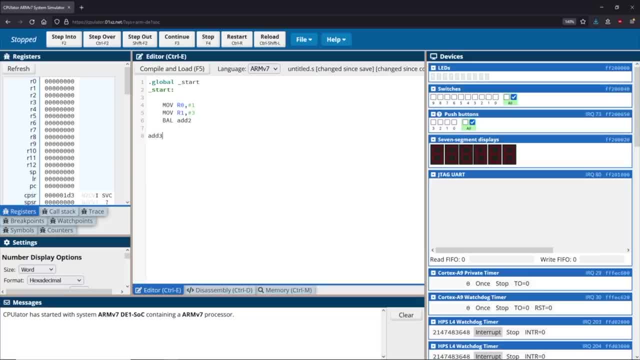 So we'll call it add to, And then I'll define it here, And all this is going to do is it's just going to add the numbers together and store the result in r2.. And there we have a very simple idea of a function. So when we run this, of course it. 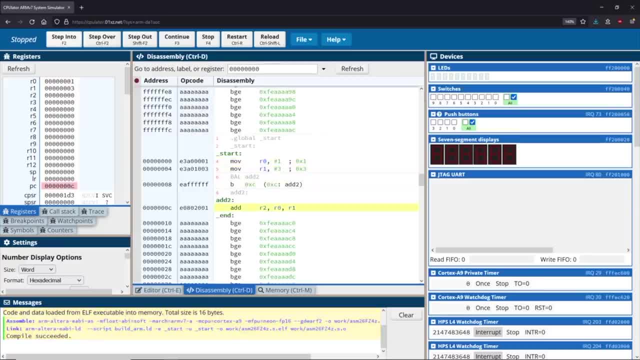 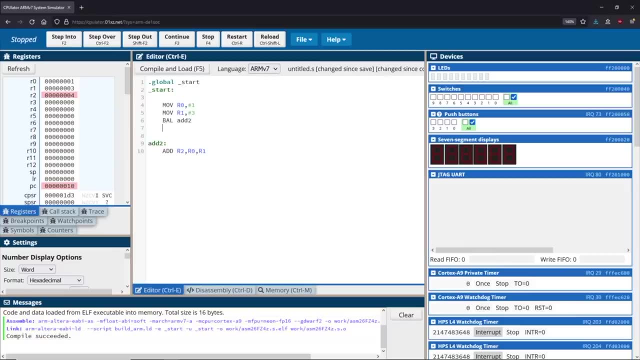 should work the way that we want it to. So we're going to call it add to, And then we're going to add the numbers together. we end up with four, and everyone is happy. Now my question to you is: what if I wanted to do something slightly different? What if I wanted to continue execution directly? 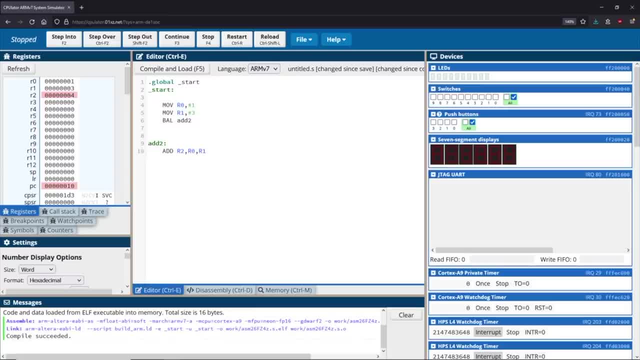 after this function call. So what I mean by that is that maybe after this function call, I want to do something different. right, I want to, you know, move some more numbers into registers. you know, maybe I want to like move into r3, the value for right. 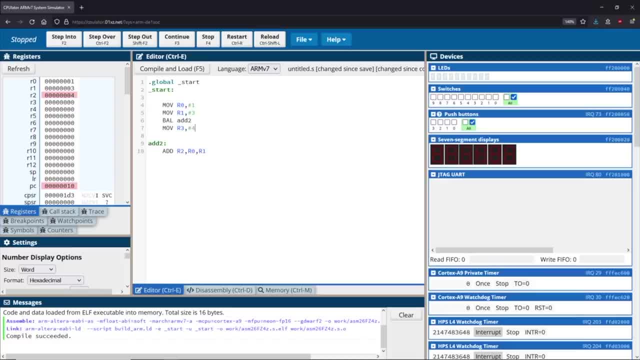 so if I want to do this, I have to have some way of coming back to this location after this function is called. Now, there are a few ways that we could achieve this sort of idea right. Like I showed in a previous video, what we could do is we could branch after this ad and we could branch to. 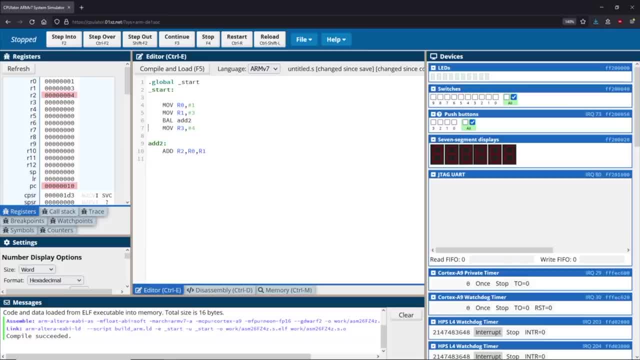 this location here And then after that location we can branch beyond the, the add to function, so we don't actually run back into it. This creates a little bit of complexity And we don't really like that complexity. it's a little bit weird to follow. So in these sorts of situations, 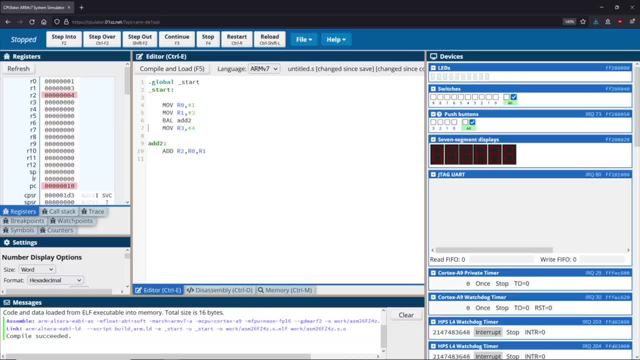 where we're just calling this as a function. what we can do is we can add in what is called a return address And with the return address, what we're able to do is we're able to return to the function where we started, So we're able to, at the end of this function, return back to the location. 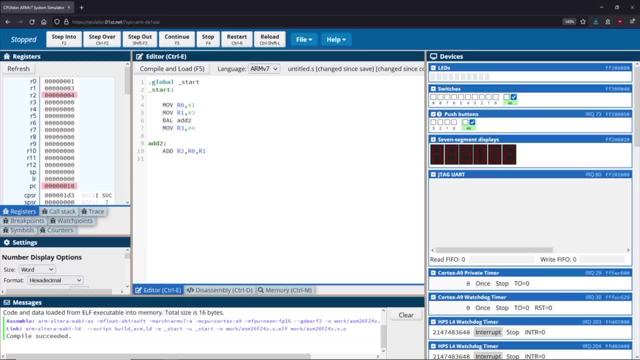 directly after we called that function. So this is the idea of a return. So that's what we're going to take a look at here. we're going to take a look at how we can do this, And the first thing that we're going to do is we're going to change this branch to a BL. 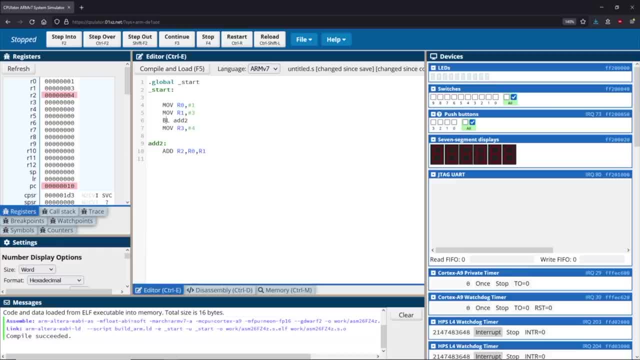 which means branch links, And what that's going to do is it's going to store the location that follows this branch inside of one of our registers, which is this one here, the LR register, or link register. So, without doing anything further, let me just show you what that looks like. 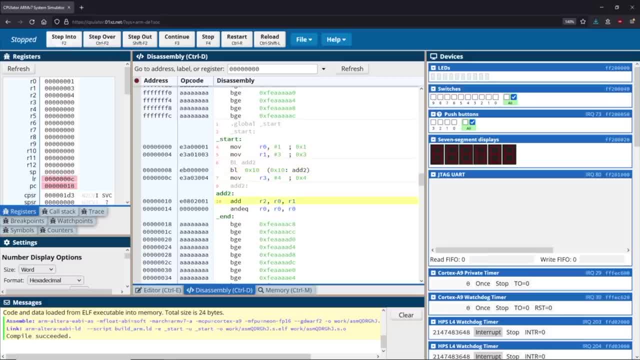 So when we go to this point here, bl, you'll see that LR gets 00000. And then see right, What that location corresponds to is the address of the instruction that follows the branch. So you can see, here at C there's this. 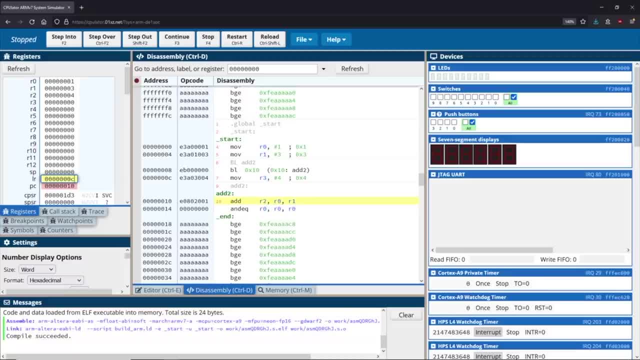 move instruction, which is right after our branch. So you can see that what this link register stores is it stores the location directly after the call or branch to the function. So, in order to make this work, I'm not going to be able to do anything further than say we're going to add this as a 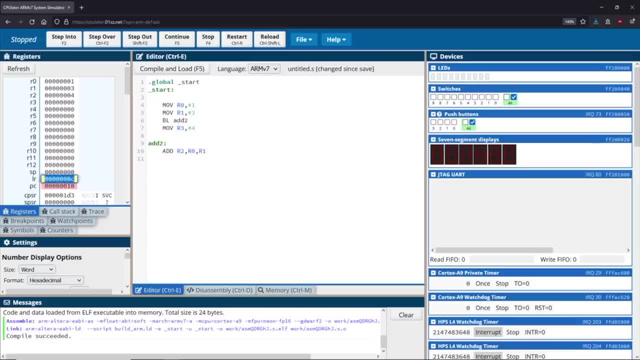 after we finish this here, we should go back to the location that's stored inside of the link register. So in order to do this, we can use another instruction known as a BX. this will branch back to the location stored in register. So in this case we can branch back to LR, which 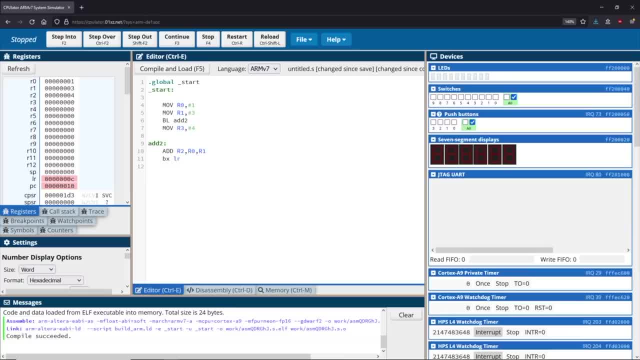 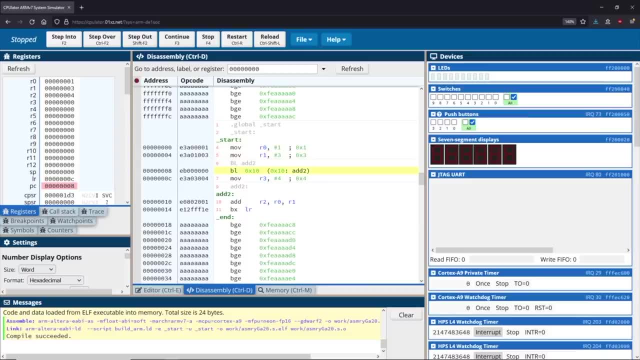 will branch us back to the link register. So let's pull that all together And let's see what that looks like. When we do this, we move the values into our registers, we branch into the add function. you can see that it's storing C as our return location, which is this move instruction. 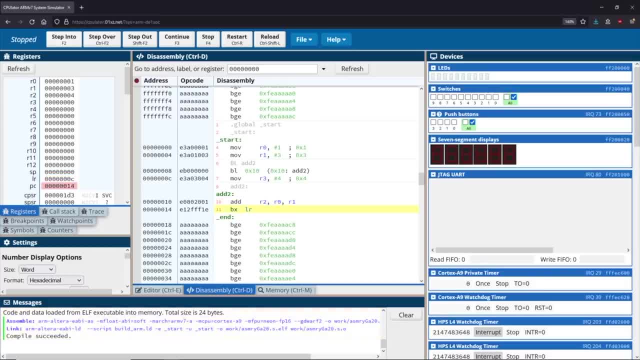 right after this branch, you'll see that we add the values together in our two and then we branch. it takes us back to this move instruction. So you can see that that actually worked. it brought us back to the location where we started. This mimics the sort of flow of a typical function, right? If? 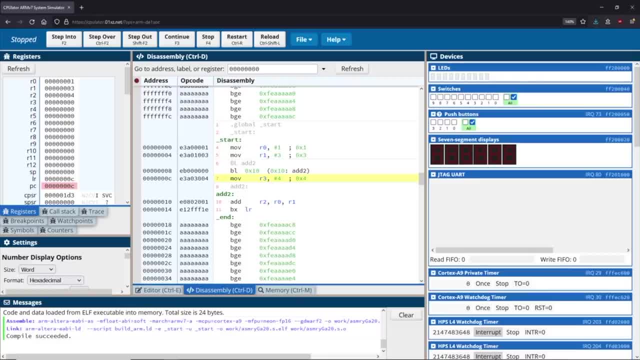 you are familiar with higher level languages. when you have a function, you have a return. the return takes you back to where you started. This is the exact same idea And this is what your higher level languages are doing in the background. when it translates into assembly, this would be the idea of what is 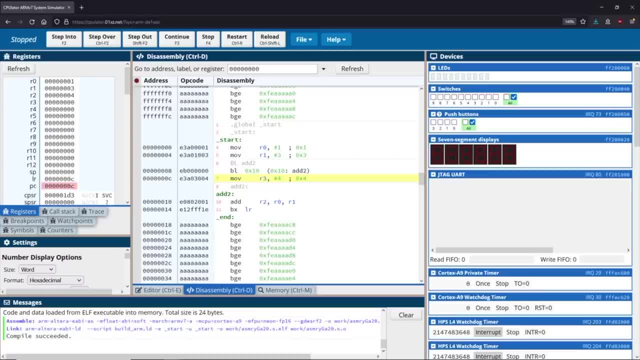 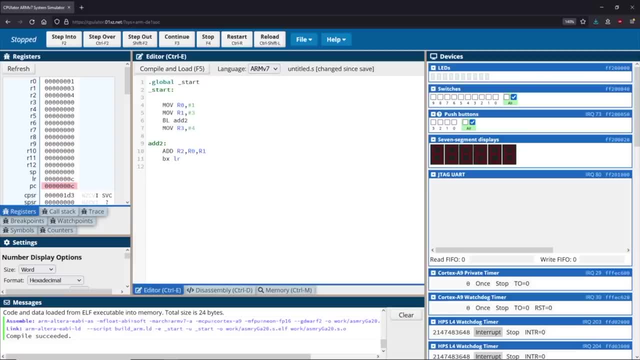 happening with that translation. So this gives you a bit of an intuition behind how we actually do these branches with returns. Now I'm excluding a little bit of detail here. there's more things that need to happen to make this work completely functionally right. 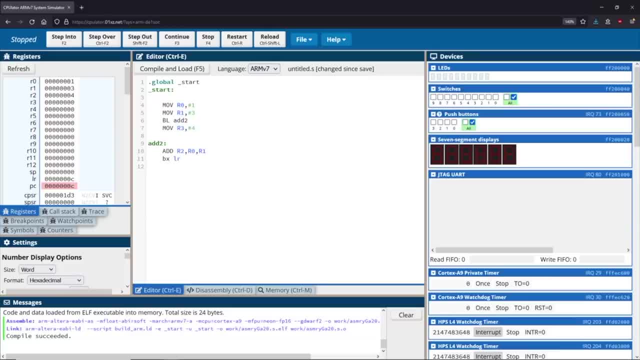 You know, if we have more complex programs, there's certain safeguards that we need to take in order to make this wake as as good as possible. However, for the time being, you have a good understanding of branching with the links, how that link register works and how to return back afterwards. So that's. 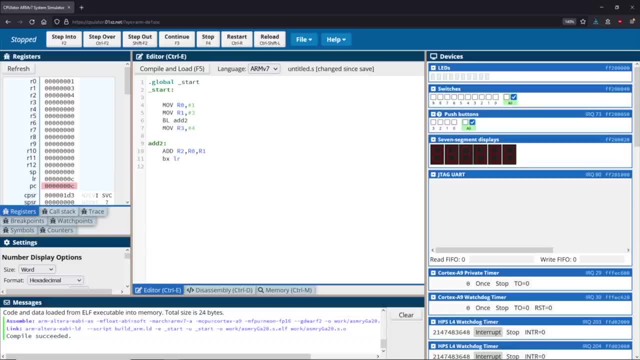 all we're going to talk about in this video. This gives you the fundamental ideas of functions and subroutines with returns, And now in the next video, I'm going to discuss a little bit more detail of how we can say: preserve things before we move into these functions. And then we're going to 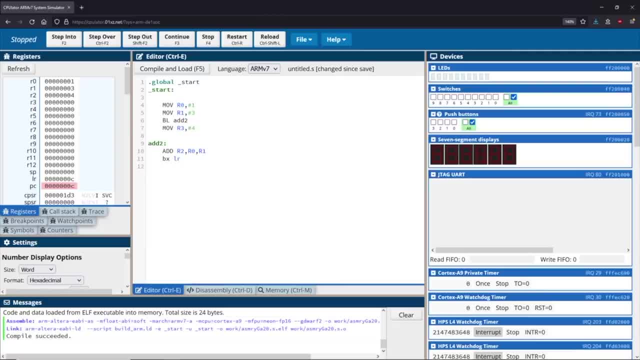 talk about how we can then be able to utilize that to our advantage. So that's what we'll sort of go into next after this video. So one notable idea about functions and subroutines is that they often have to do calculations inside of them in order to get the result that we're looking to get In order. 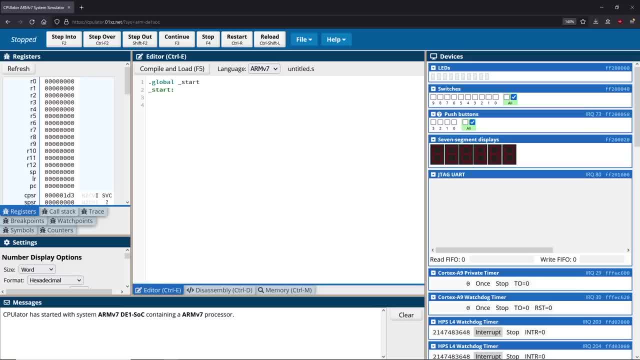 to do these various calculations, we may need to use different registers in our processor. Now, the number of registers that we have an arm are, of course, limited. we don't have an infinite number of registers to work with, So because of this, we may need to reuse a register inside of a function. 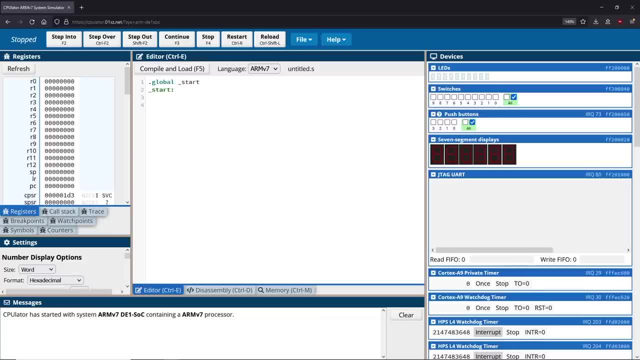 that's already being used outside of the function. In these sorts of situations, we need to be able to preserve what we had before we called the function and then be able to restore it once we're done with the function. You can think of this concept similar to local variables in the 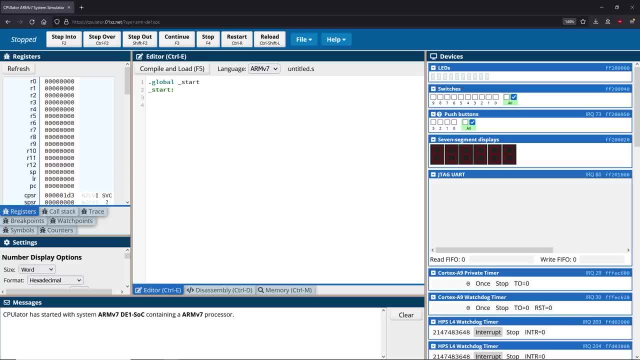 function. when we declare a local variable in the function, its scope is to live inside of the function. Once we read the function, we're going to have a variable. So the variable is just de allocated and a garbage collector will come and you know, remove the memory and all of that fun stuff. So what we're doing here is we're. 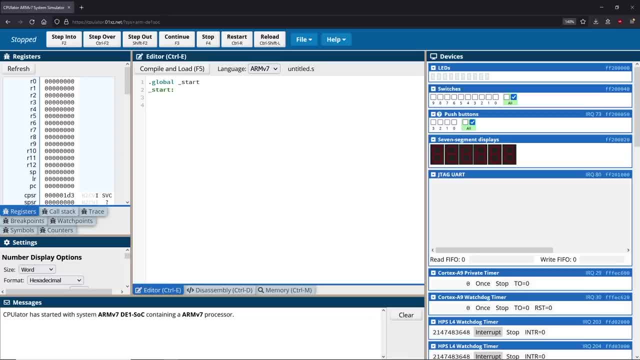 emulating that sort of idea. we're going to allocate some registers in our main sort of aspect of our program. we're going to call our function, we're going to use the same registers, then we're going to restore the values back to the main. This is done in the background in high level. 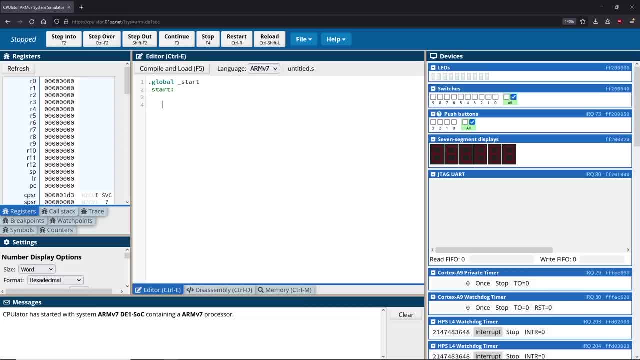 applications. Typically, the compiler is responsible for setting up these sort of register applications. This is something that we would see in sort of the low level assembly that comes out of compiling of programs, So it's something that is done by your high level languages without you really. 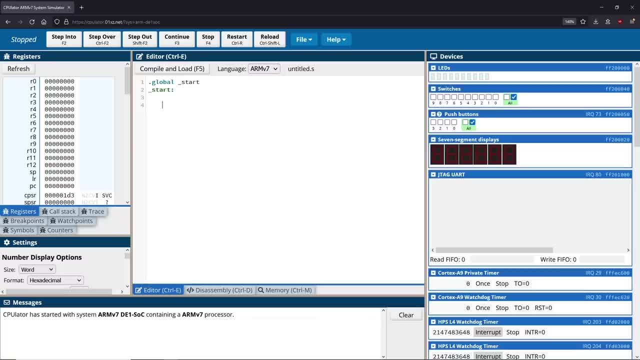 knowing about it. So let's take a look at the details of this. So suppose that we have a function where you know some stuff was happening beforehand and then we call function and then we continue on as normal afterwards. So maybe some of the stuff that was happening beforehand is using. 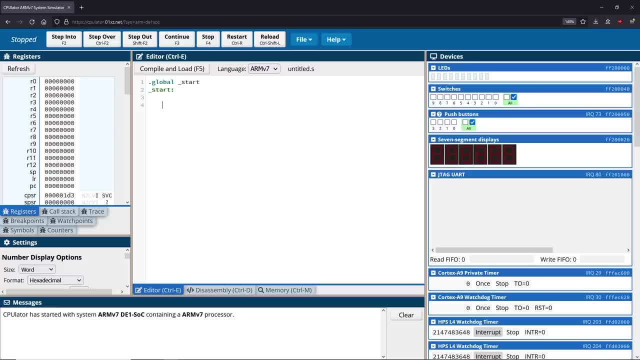 the registers are zero and are one. maybe they have some values inside of them. So let's say: you know, our zero has the value of one. Let's say, our one has the value of three. Now what's going to happen is we're going to do a branch for a function. I'm just going to call a function: get. 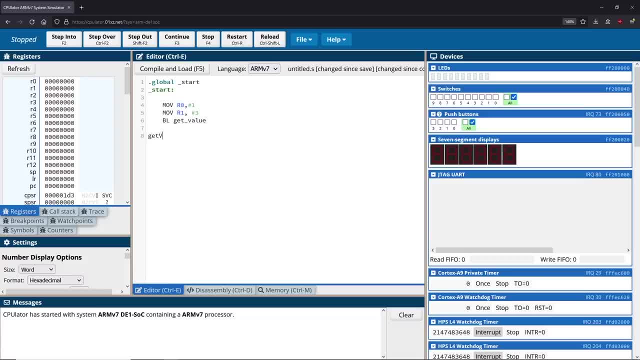 value And then we'll go ahead and create that function. So we'll say: get value, And what this function is going to do is it's going to need to use our zero and our one. we'll just pretend all the registers are full right now And our zero and our one are the only ones that we can really work. 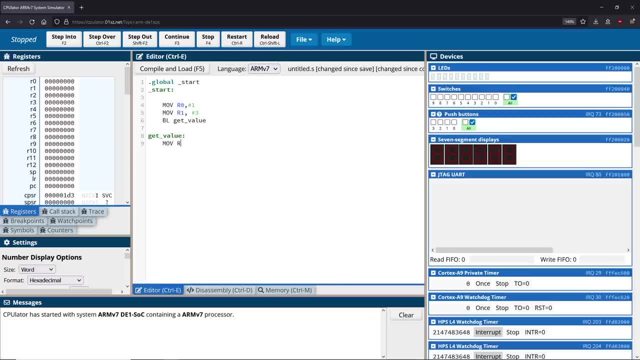 with. So we're going to say: I'm going to move some values into our zero, we're going to move some values into our one, And then we're going to do some sort of calculation. So I'll just add the two together. 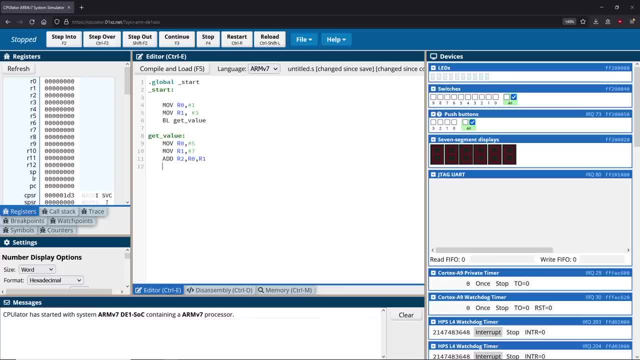 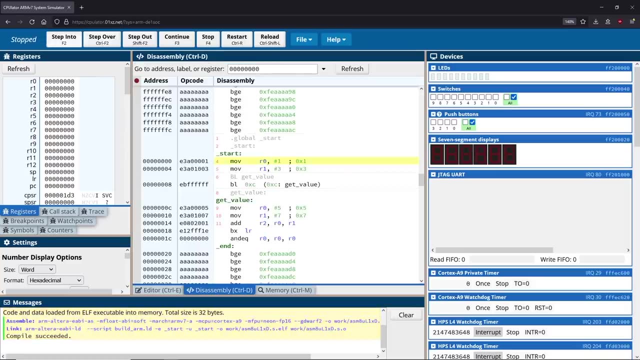 perhaps, and store the result in our two, And then we'll return back to the link register and we're done So. in this situation, you can see quite clearly that when we move into this function, our zero and our one are overwritten right. So we're to compile and load this right. 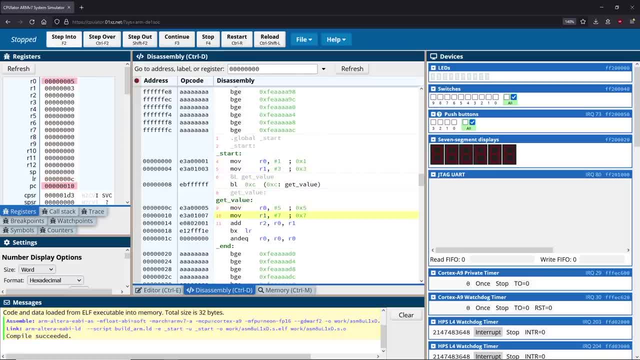 now, you know we would have one in three. then when we branch, we get five and seven. we do our calculation, But when we come back to the beginning of our function, we no longer have these results available to us, right? we no longer have. 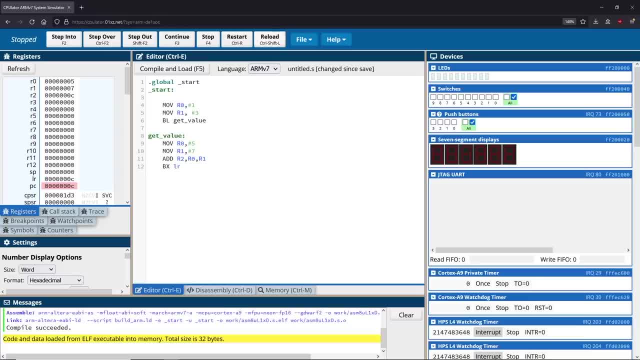 the R zero and R one values. So to be able to help resolve that, what we're going to do is something interesting here. what we're going to do is we're going to push the values of R zero and R one onto the stack memory. So we're going to do this. we're gonna say push. 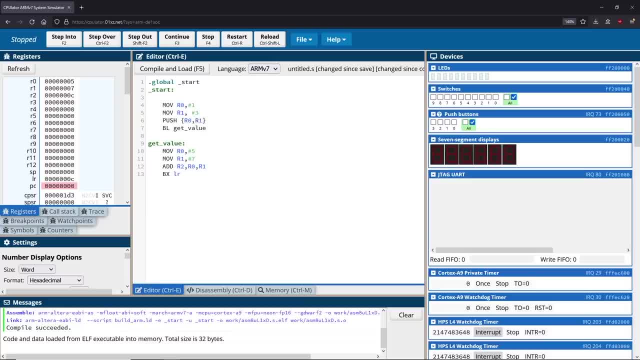 R zero, R one. what this is going to do is it's going to place the values of R zero and R one onto our stack, right, So it's going to place them onto the stack, And then what's going to happen is, once we're done doing everything related to this function, we're gonna go ahead and pop. 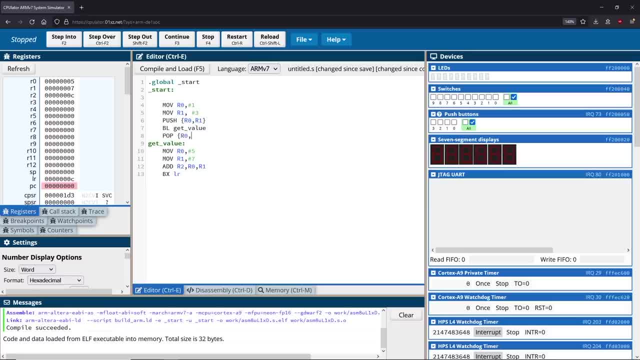 them off the stack like this. we're gonna say, pop our zero and R one. And then we're going to do is I'm just gonna, I'm just gonna branch to like an end label So we can just sort of like get somewhere that isn't going to have, you know. 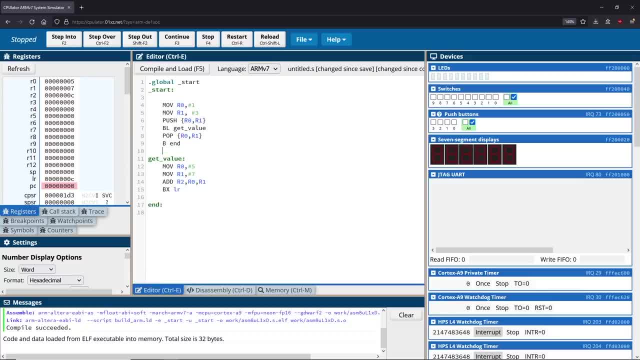 the function, interfering with it, Because otherwise we just move right into the function again, And that would be the end of this. So what's happening here is, when we move the values into R zero- our one- we then push them onto the stack of memory, So we'll get pushed over here. 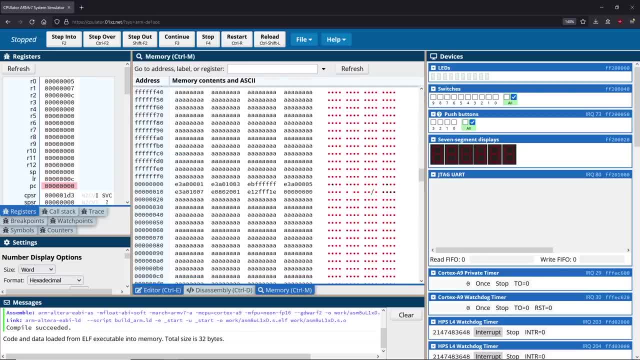 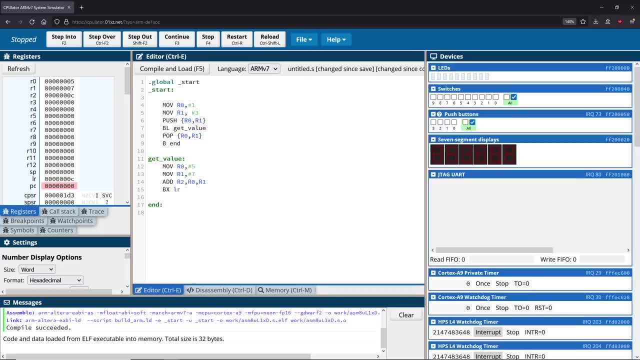 onto stack memory somewhere. And then what's gonna happen after that is: we're going to call this function, we overwrite R zero and R one, we do our calculation. when we return back to the link register, we come back here And then what we do is we pop the values off of the stack back into R zero, R one. R one and R one, And then what this does is we back the values off of the stack back into R zero and R one, And then what this does is we overwrite our x and r one, and then when we do that, it really wouldn't. 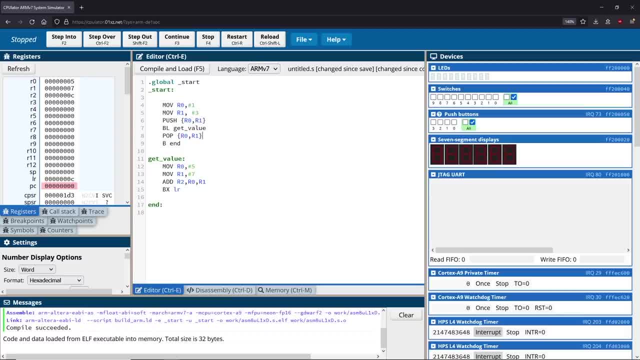 r0 and r1.. So it's going to pop those values and place them back where they started. This is preserving the values of r0 and r1 on the stack and then placing them back when they're needed again. So you can see that the result of this is that the values for r0 and r1 don't get overridden. 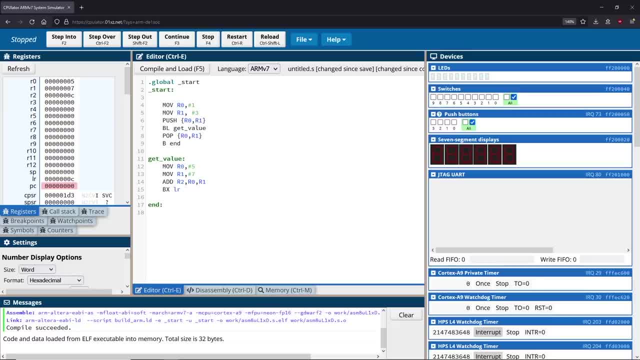 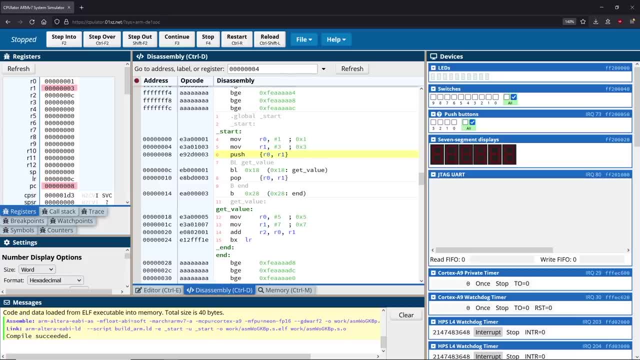 they get used locally in the function but we don't overwrite them permanently. So let's run this and see what happens. So you can see that we get one in three to r0 and r1. And then we push them onto the stack. If I come over to the stack memory here, you can see we have three and 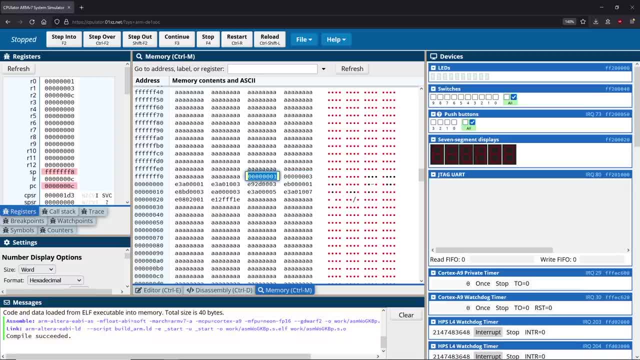 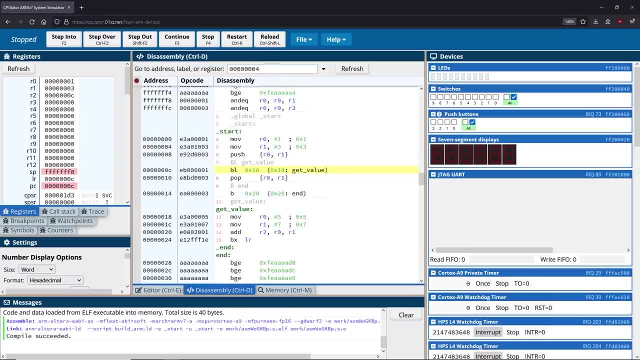 one. So when we're thinking about how popping works, just to just to sort of clarify why we're doing this pop, the way that we are- what's going to happen is we're going to pop the first thing into the first register and then the second thing into the second register, right Since the stack. 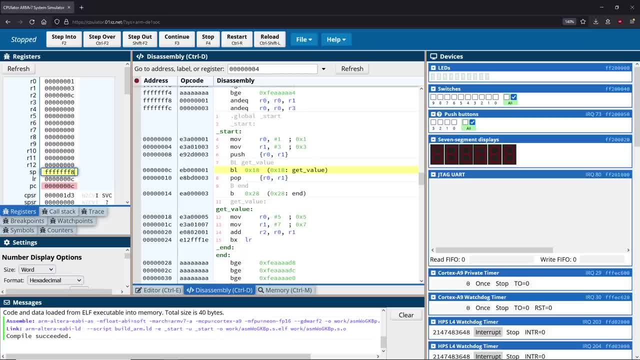 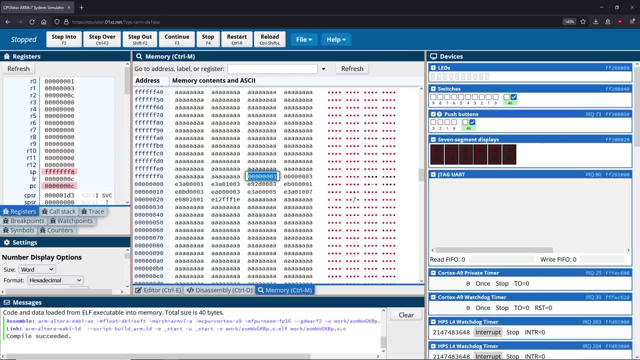 pointer currently points at this: you know F, F, F, F, F, eight address. what happens is it's going to take the value off of that address, which in this case is one. it's going to pop it on to the first register and then the second thing into the second register right Since the stack pointer. 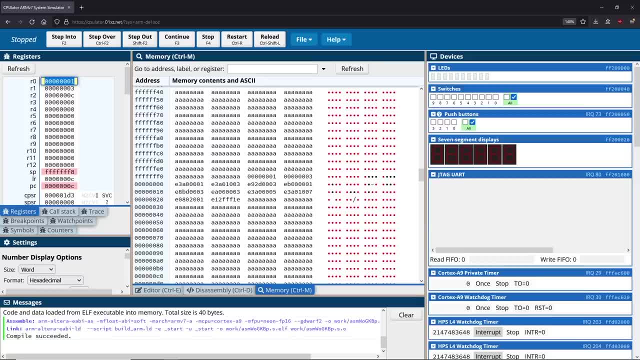 first register, which is r0, which is this one here, and then we're going to pop three onto our one, which is this one here, right? So you can see that it just pops one after the other like that, starting at the top and moving down to the bottom. So hopefully helps you understand a little bit. 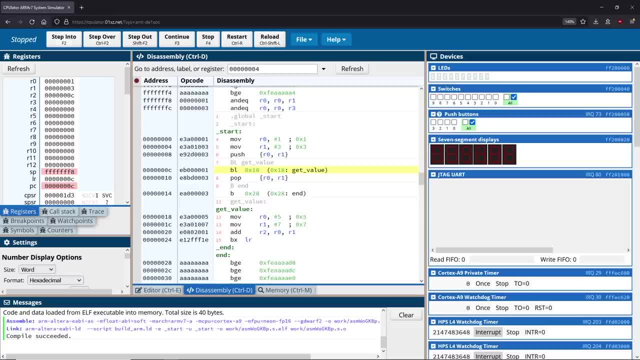 about the ordering of these two operations. Now, when we do our branch, you see that we come into here, we have five in our zero, we had seven in our one, that we do some calculations with them And then we branch back to the beginning. When we branch back to the beginning, you see that we hit. 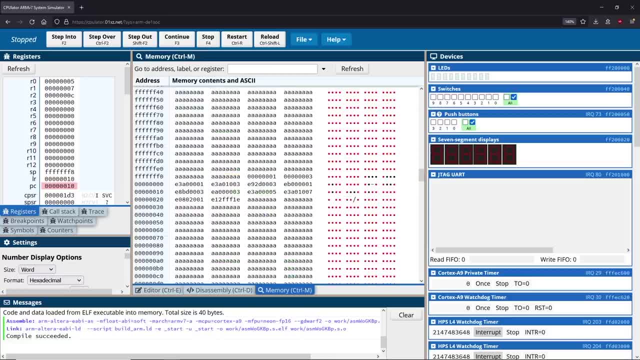 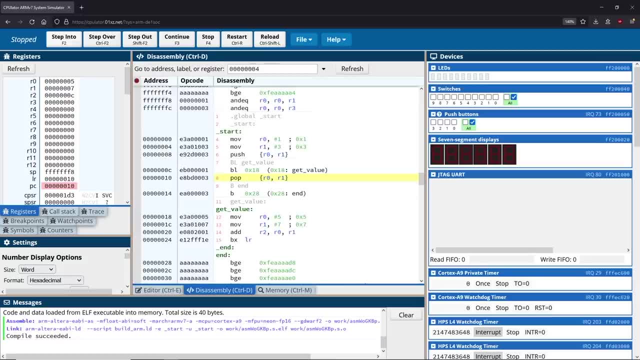 this pop instruction. Now watch what happens right. the stack pointer currently points at the location of one and three, right here And here. when we go ahead and run this operation, what you'll see is that r0 is now one and r1 is three. you can see that it actually did preserve those. 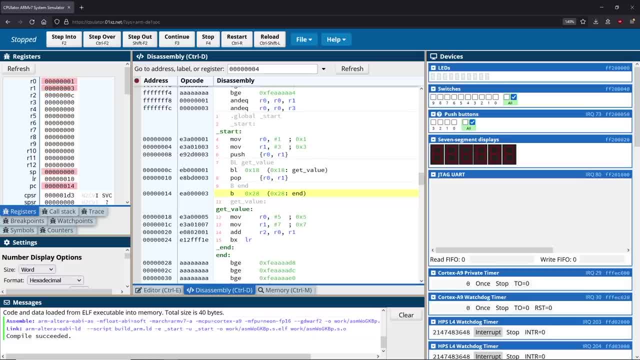 values right, So it actually did place them back into their respective locations. This shows that we can actually preserve these values So they can be used in the function and then sent back to their original values after the function- Right. And then, of course, we have our branch. that just takes us to the end. 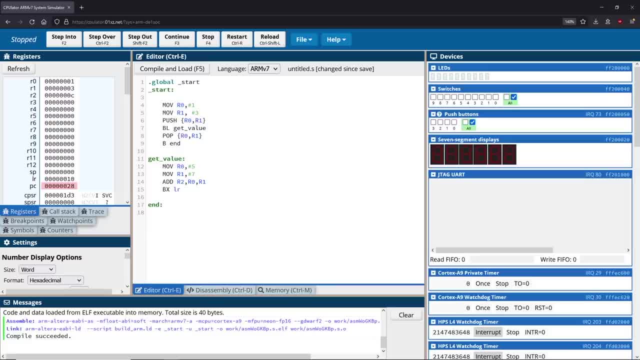 So hopefully this helps you understand the idea of how we can preserve values in our functions, And we can use these sorts of ideas in a lot of different ways, right? One other way that we can use this is actually with return values, right? Suppose that r2 was also being used. what we could 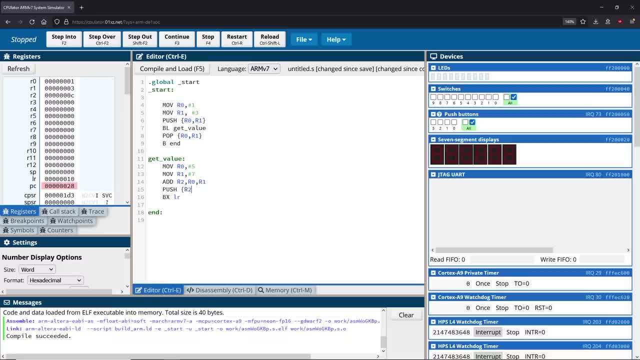 do is we could do something like this. we could say, okay, so push our two onto the stack, And then we come back here, we pop them. we'd currently be pointing at our two. So what we can do is we can. 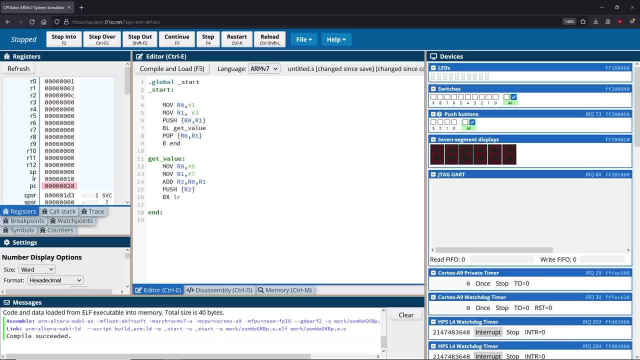 place it in some unused register, right? So if I want to get that return address value, I could say, okay, let's place it into an unused register. maybe you know our nine is unused, for instance, right, so that would be able to place us at our nine instead of having to be you know. 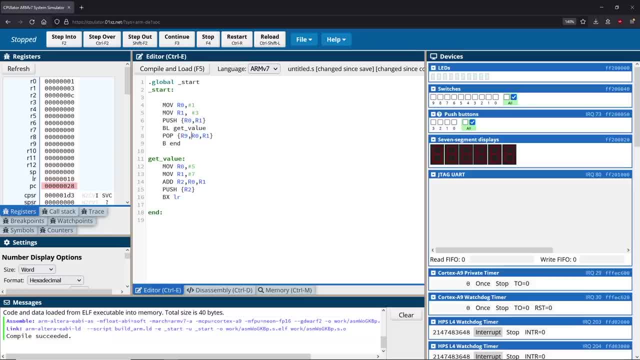 somewhere else, right? So instead of having to keep it in r2, we can place it on the stack And then we can retrieve it from the stack afterwards. This would be a more traditional way of returning values, Although I think often values are just returned on the in the register. 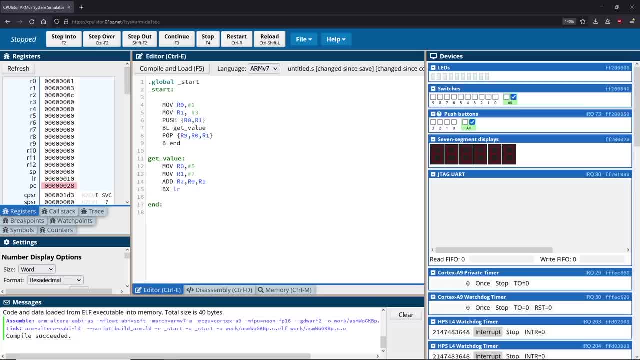 itself. So we don't really have to worry about this sort of idea, Because the thing is with values being returned. if you return a value, odds are you're going to be using it at some point in the code, right at some point soon in the code usually. So what happens is we place it into an 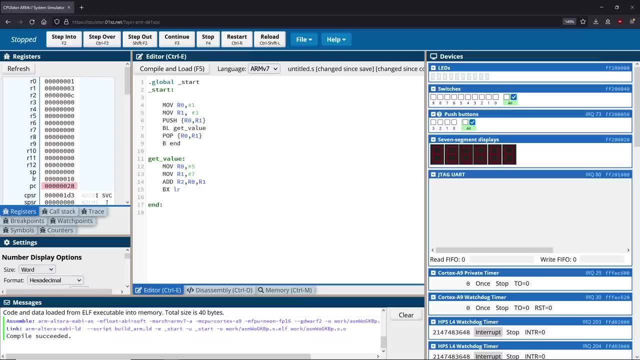 unused register and then we just use it right. So that's the typical case with these, with these returns. you know otherwise you'd have to pop it off and place it into its position immediately. So you need it in an empty register regardless. So that's why we don't usually do that. I just 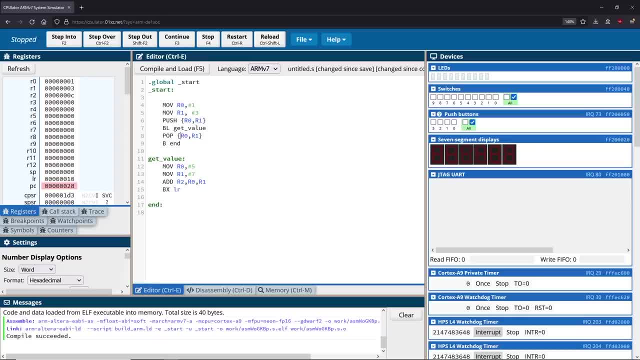 wanted to give you a little bit of context in case you ever see it. it is something that you can do. I think it's not usually the case that you would end up doing that. So with this you now have a full picture of subroutines and functions in arm. you understand more of how to preserve. 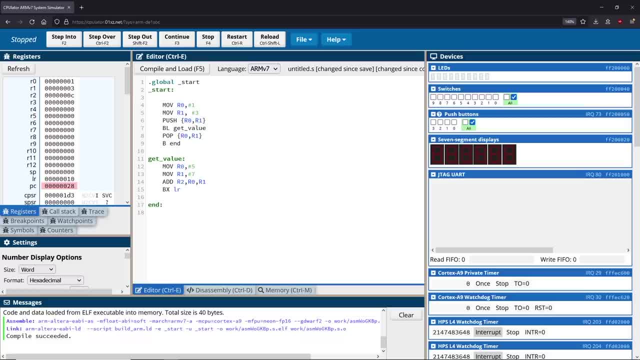 values, how to set values onto the stack and remove them from the stack, And this allows you to be able to write fully functional subroutines for your programs. So that sort of sums up a lot of the logical ideas of what we would typically talk about for sort of an introduction to arm. 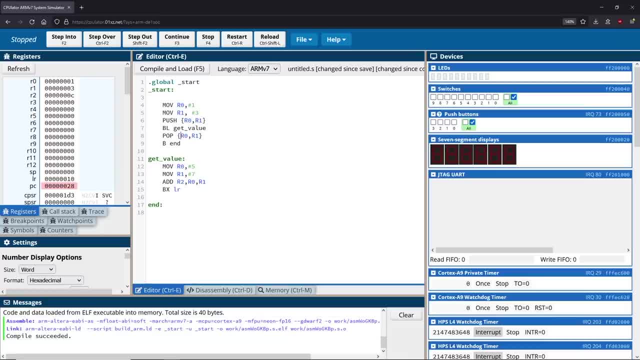 assembly type course. For the next few videos, we're going to be talking about some of the things that I put out. I'm going to be showing you the ideas of working with hardware, with the arm processor, which is actually going to be pretty straightforward because we actually have 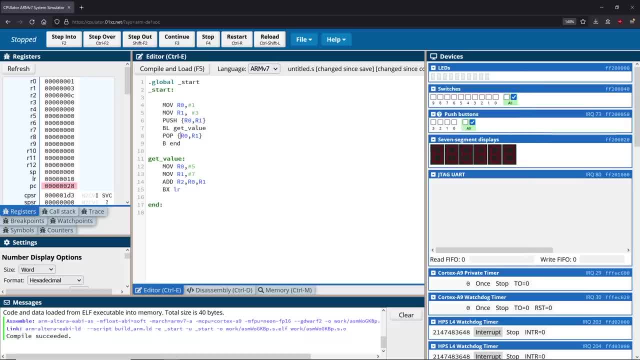 some hardware devices here on the right hand side. So I'm gonna show you how to interact with those hardware devices, get you familiar with hardware And then we can start to take a look at some other concepts, maybe at a little bit of a higher level, and see how we can interact with arm and other. 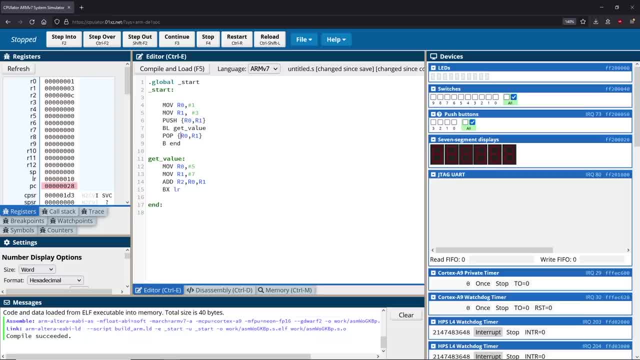 system related processes. So that's sort of where we'll take the next few videos. In this video we're going to take a look at how we can interact with a variety of different hardware devices using our arm processor On the right here. 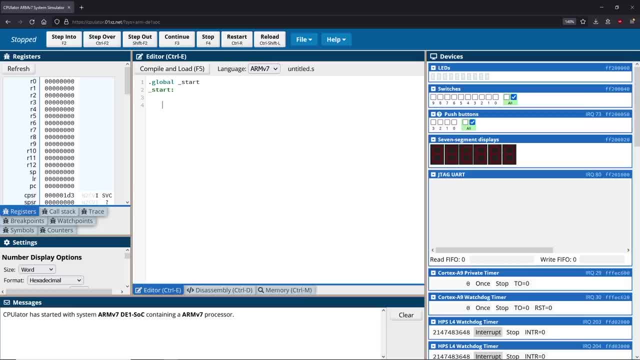 we have a variety of different devices. I'm just going to note right now you need to be using the arm de one SoC emulator to have these devices. for using just the arm one general emulator, you won't have these devices available to you, So you have to use the d e one sock emulator. 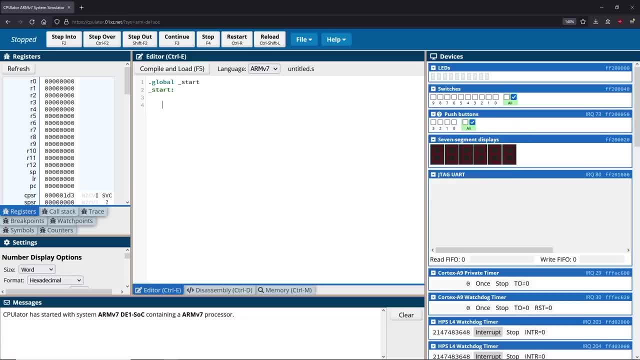 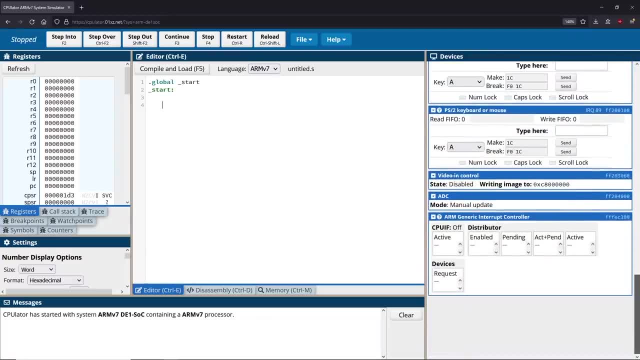 So, with this emulator, we have a number of different hardware devices that are available for us to be able to interact with. I'm going to show you how to interact with a few of these different pieces of hardware And, once you have an idea of some of the general devices that we're able to interact with, 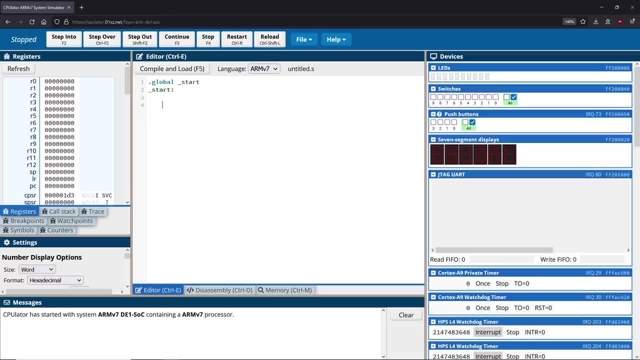 you'll have a better understanding of how to interact with the other devices that are available to you. So, primarily, I'm just going to show you how to work with the LEDs and the switches, And these are really just a rudimentary input and output. the switches are an input and the LEDs 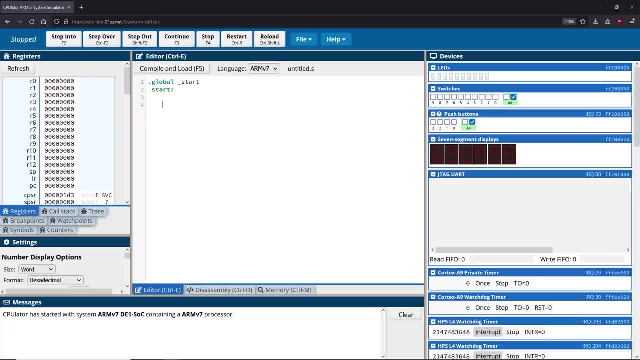 are an output, So let me show you how the input works first, which is the switches. The very first thing that we need to do is we actually need to declare a variable that's going to store the location of our switch and later our LED as well. The way that we do this, 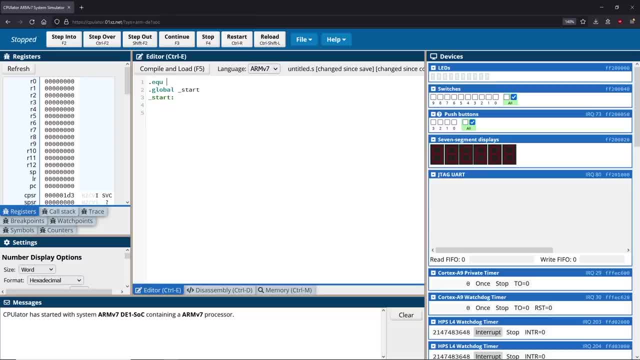 is. we say dot eq And then we put the name of the variables. So in this case I'm going to call mine switch And then we put the location of the variable. So in this case the location is right here, this ff2006.. 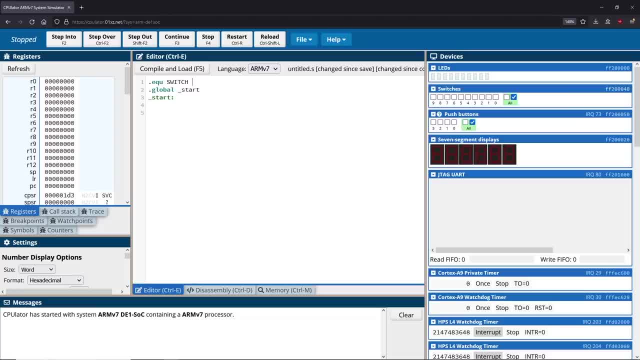 0040, right here. So we're going to put that in. So we'll put it in hex, right? So 0x ff 200040.. Now there's a good reason why we do this. the reasoning is because you can't directly load. 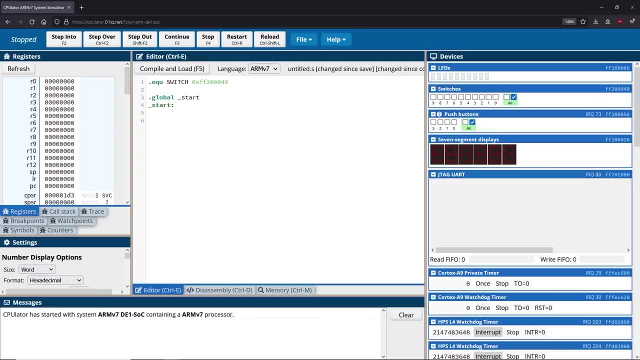 something this large into arm directly. So you can't use an LDR and just load in this value as a constant value. there's a limit to the size of the constant values that are allowed To be loaded in directly, So if your value is larger than that, you actually have to declare it. 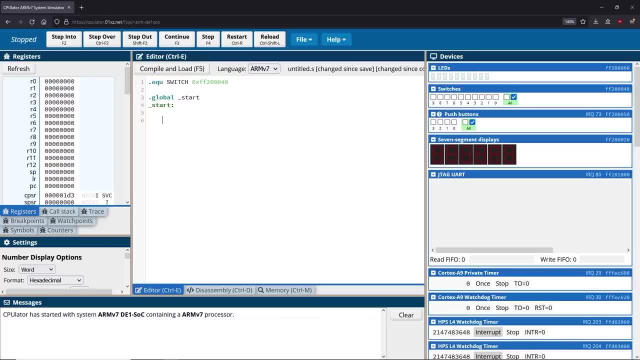 as a constant value, like I've done here, And then what you can do is you can load it in like this: you can say LDR, and then I can go into our zero, for instance the value of switch, And what you'll. 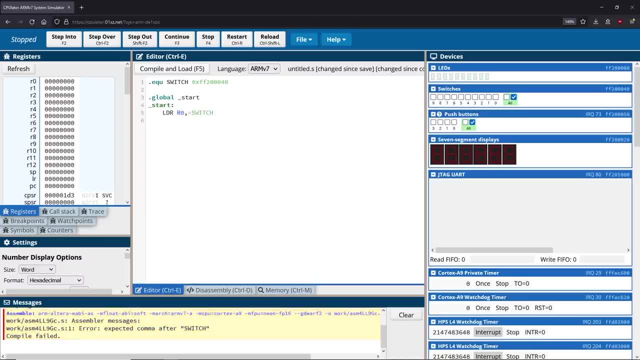 see is that when we do this, we can compile and load, And once we do that, we should be able to see the actual value. Oh, sorry, I forgot a comma here, So don't forget the comma here. So it'seq. 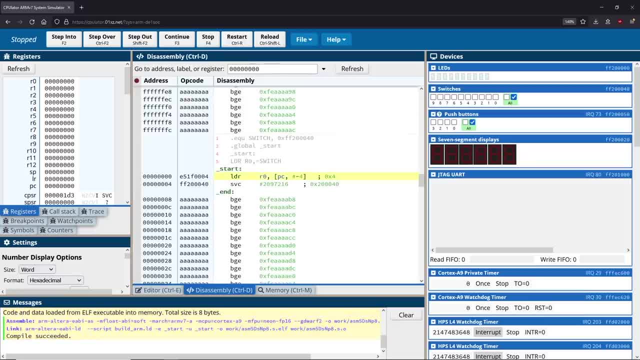 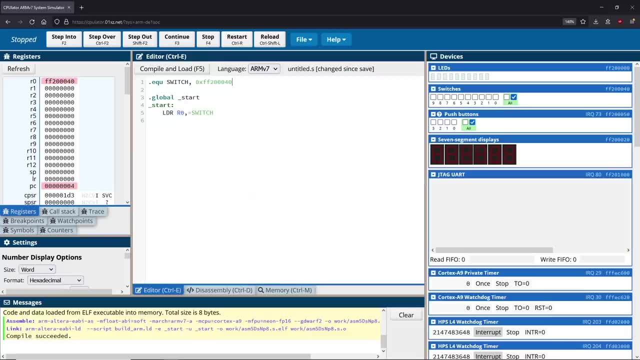 switch comma and then the address. Now everything will compile. And when we do that, you can see, we just get that exact value loaded into our zero. So all we've really done is we've declared it here as a constant and then we've loaded it into our zero register to be used later on. 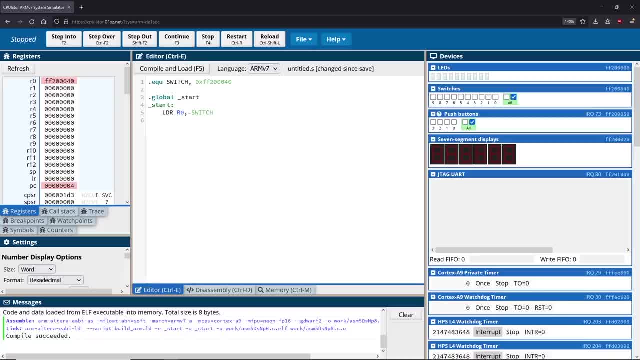 So if I want to be able to use this register, what I have to do is I have to be able to retrieve the value that is located at its memory address. So what's going to happen is each of these switches is going to correspond with a different number, And that different number is going. 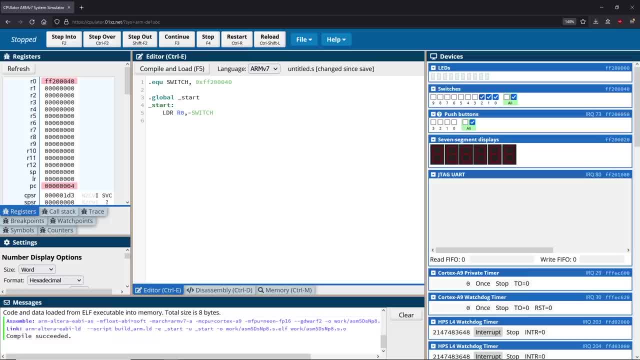 to be represented in binary based on the switches that are on. So this rightmost switch here is going to represent, like the two to the power of zero, portion of the binary: This one is two to the power of one, this one is two to the power of two, and so on, like that. So that's the way that this. 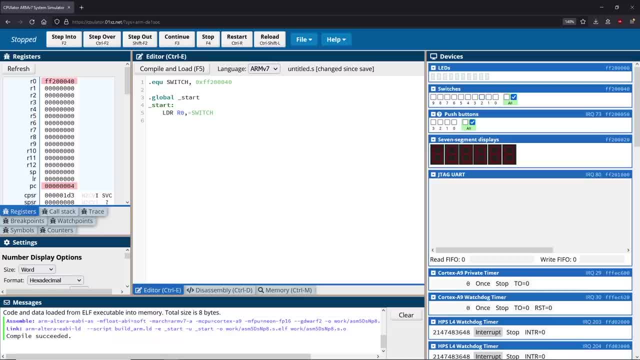 is working. If it's on, it's like a one in binary, And if it's off, it's like a zero in binary. So, for example, if I check this off, it would be the same as one zero in binary, which is two, of course. 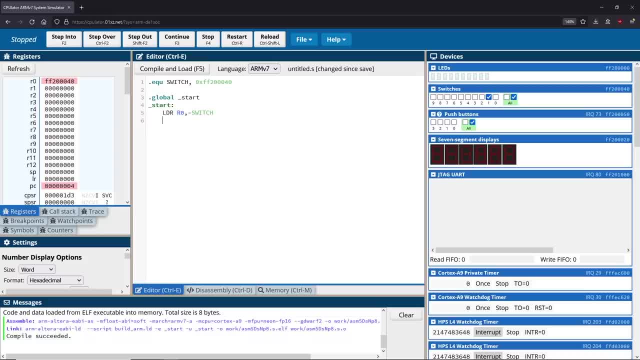 So let's take a look at how that works. What we do is we say LDR, I got to load into r1, the value that's stored in r0. So remember, this is the address of the switches. are zero is. 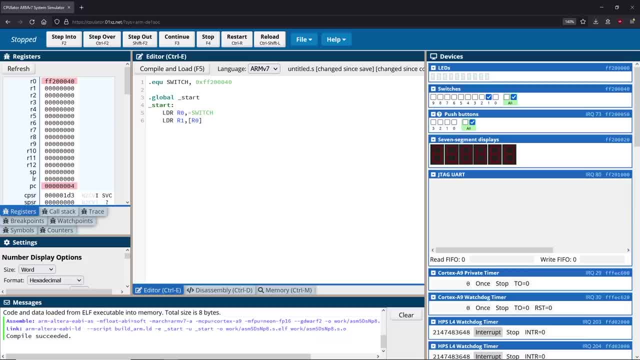 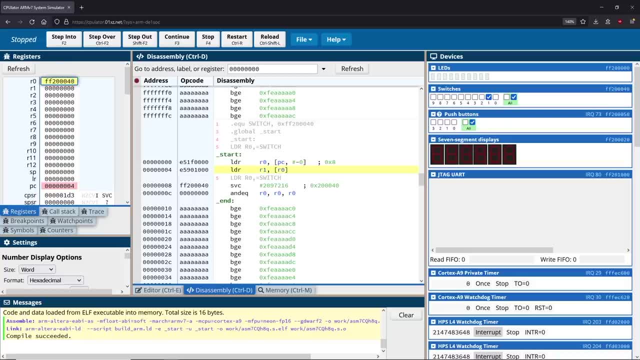 and we're loading from the location right r0 into r1. So let's compile and load and see what that does. You'll see that r0 is currently equal to this memory location. When I step into the next line of code, you see that we got the value two And that's because I have the one checked. 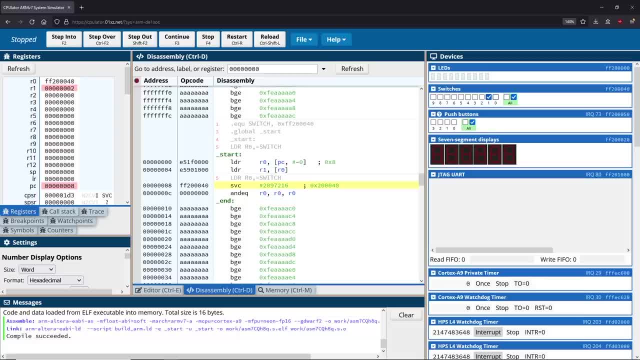 off, And that's because I have the one checked off, And that's because I have the one checked off. So, remember, it's one zero, which means that it's equal to two, And we can do this with all sorts of different numbers, right? So I could check off like all three of these, right we? 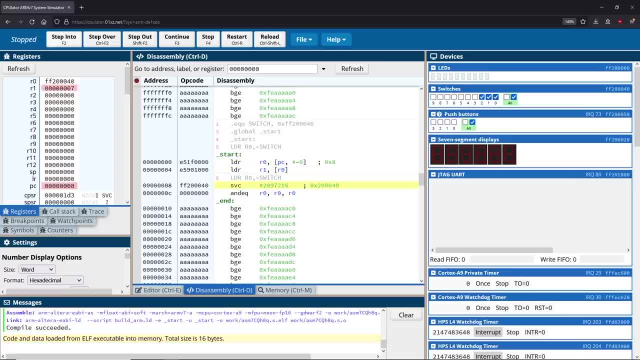 would get 111.. Let's just reload it and give that a try. You see that that gives us seven, right, Because it's four plus two plus one, which is seven, of course. So using this, we can actually get inputs from users, right? So I can actually do things based on the input from these switches. 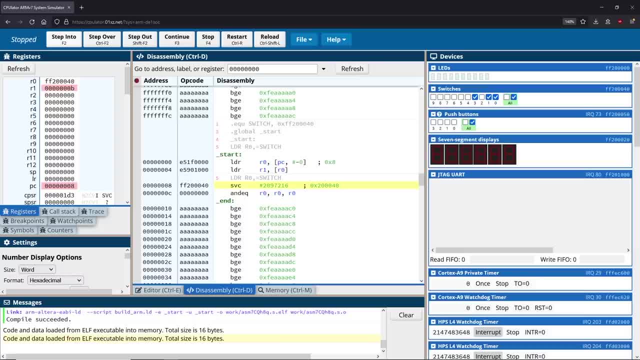 right? So I just put in whatever value I want in the switch when it loads that value. then we can manipulate it as we need. So this is a very simple way to gain input from a hardware device, right? So you may have been wondering throughout this course, like: how do we actually get input? 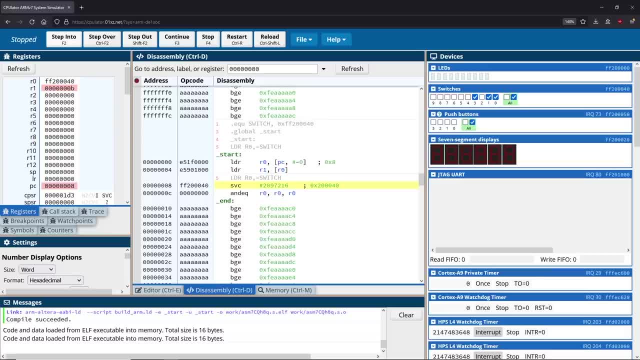 this is one way that we're able to do it. And then, similarly, how do we output values? we could do that using our LEDs, And the LEDs are going to work in a very similar way. When we take a look at the right hand side LED, the rightmost LED represents the first. 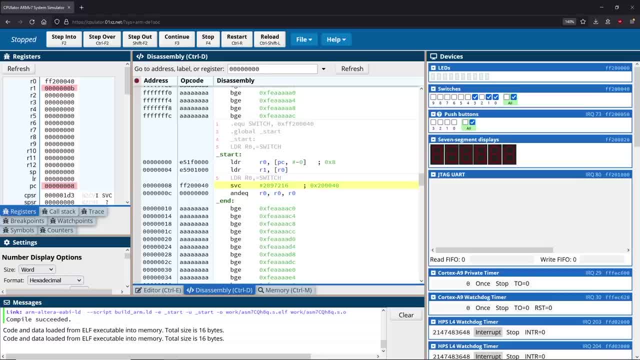 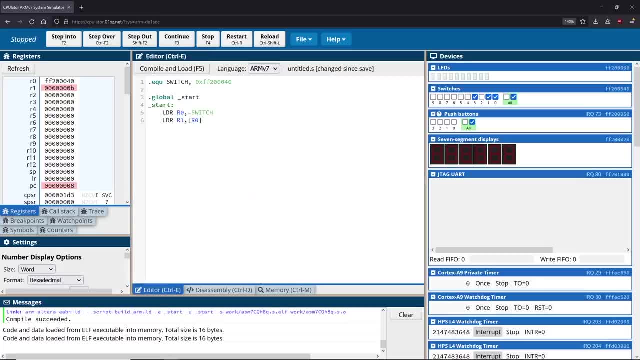 digit of binary, and then the second digit, the third digit, the fourth digit, so on and so forth, like that right. So it's the same sort of idea. So let me show you what happens with this. So let's say dot eq, because I have to declare the location of the LED right. 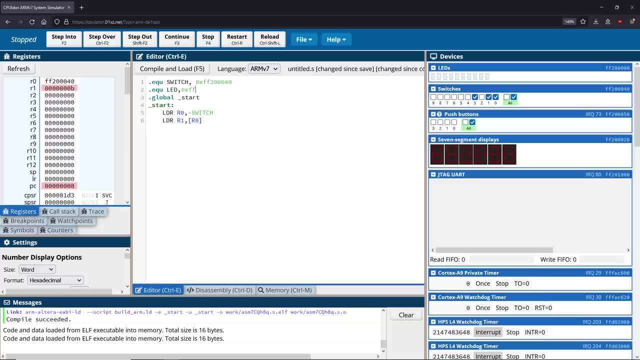 so it's gonna be led: comma zero x, ff 2000000, like that. So, once we have that located, what we're going to do is we're going to go ahead and load that value into memory, like we did before, But instead of loading data from that location. 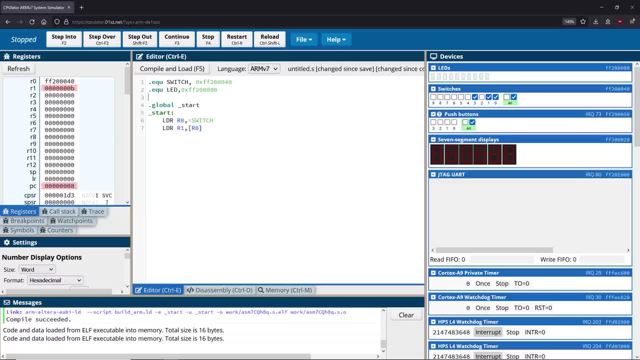 we're actually going to store data in that location, right? Because we're using it as an output rather than an input. we're going to put data into that memory location instead of taking data from that memory location. So to demonstrate this, let's go ahead and load the data that we got. 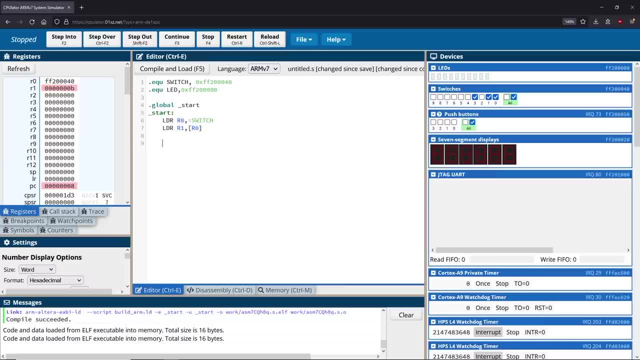 from the switches into the LEDs. So, in order to do that, what we're going to we're going to do is this: we're going to LDR And I'm just gonna go ahead and overwrite our zero, because I've already gotten the data from the switches so I don't need it anymore. So we'll say from our zero. 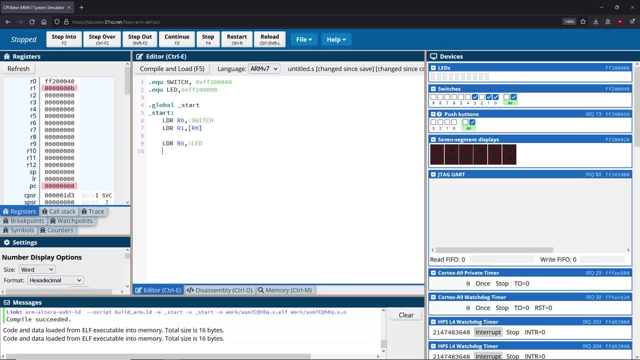 we're going to load in the LED address, And then what I'm going to do is I'm going to go ahead and store the data that's currently in our one into the location of our zero, And the way I do that, as I say, str our one into our zero. So what this is going to do is so well actually. 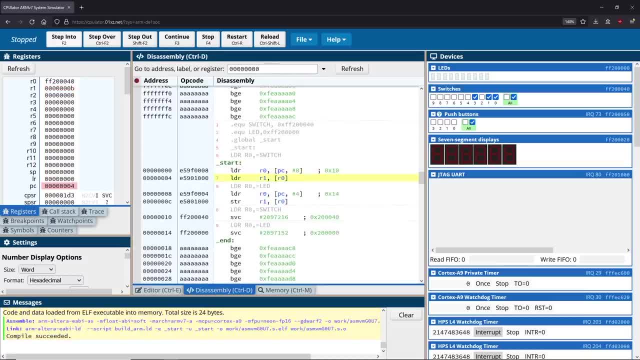 we can just run the program and see what it's going to do, right, So we can step in. you see that the first line loads the location of the switches And then the second line gets the value from the switches into register, our one right. So currently this value is B because 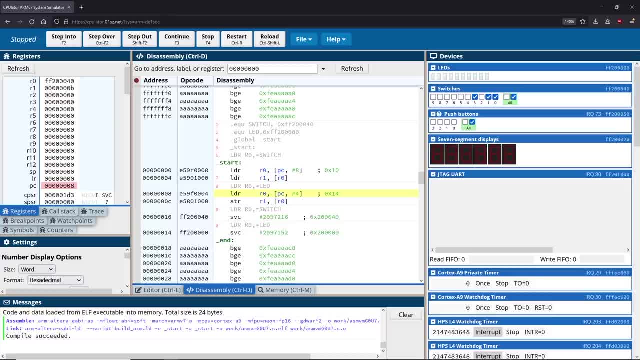 that's what's represented with this. it's 1011.. Right, So that's the value that's in here. that'd be 89, 1011, right, which corresponds to B in hex. Now, once we've done this, what we do next is we. 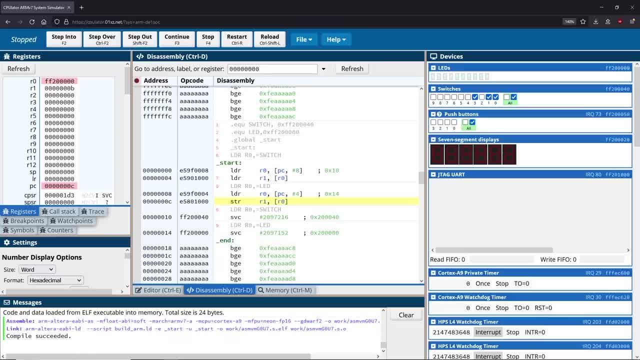 load in the location of the LEDs into memory, which is FF 2000, 00.. So you can see that those two match up with each other, are zero and the LED value here. And then what we do is we see store the value that's currently in our one into the location of our zero. So when I step into this, 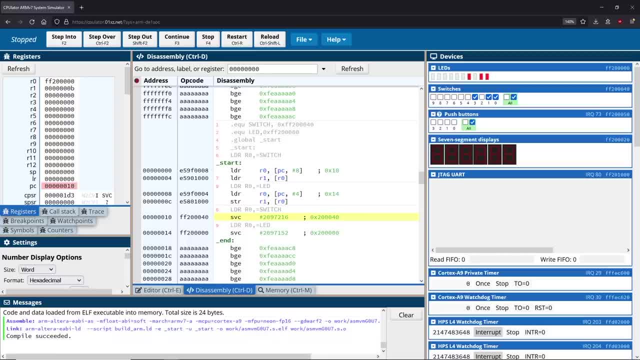 you see what happens is the LEDs light up. right, They light up based on the values that we placed inside of register: our zero or our one, rather. So you can see. what happened is these are matching up with each other. Now the switch matches up with the LEDs. The reason being is because we 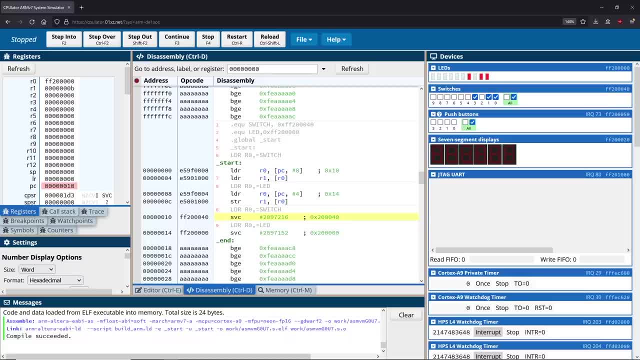 took the value from the switches and stored it into the LEDs, So you can see that that actually lights those values up. And then what you can see is that the value is now stored into the LEDs up, So we can actually represent a binary using these LEDs. So this gives you a very simple 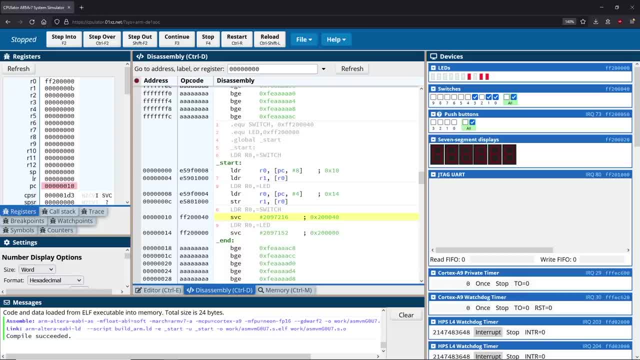 explanation towards how we can actually work with inputs and outputs using various different hardware devices. There's a lot of different hardware devices that exist here. right, There's push buttons, there's seven segment displays, there's J tags, there's- there's a lot of different. 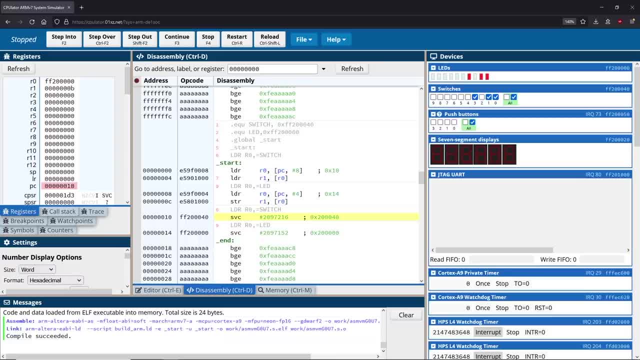 ones, And really the best way to learn these different hardware devices is just to play around with them, right? There's lots of documentation online that can tell you information about how these hardware devices typically work, And I encourage you to try each of these devices and 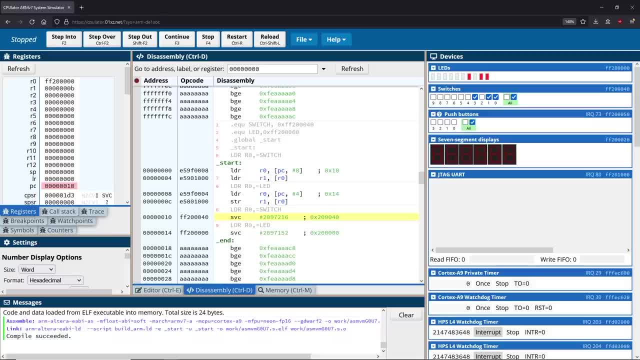 just see what they do, understand them and play around with them. That would be the best way for you to really learn those hardware devices. I've showed you the very basic ways that you can interact with them, And from here you should be able to interact with all of these hardware devices. 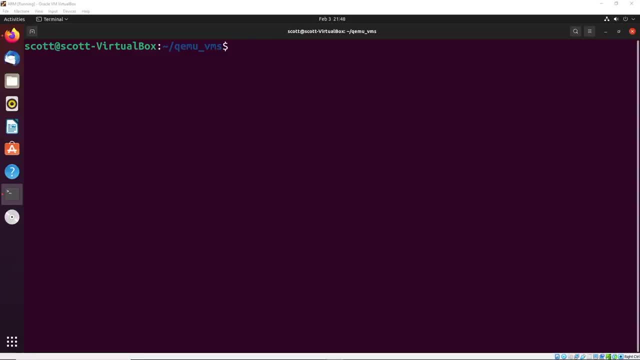 and see what each of them do. Hello and welcome back. I hope that you're all doing well. In this video we're going to start to take a look at the, the idea of programming arm through an actual operating system, in this case a Linux operating system. 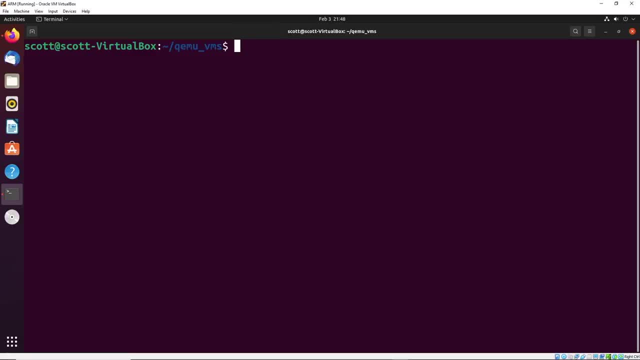 Now, the Linux operating system that I'm going to be using for these videos is called Raspbian. It's a Raspberry Pi based operating system, And the reason why I'm going to be using this operating system is because the Raspberry Pi computer runs an arm processor, And this: 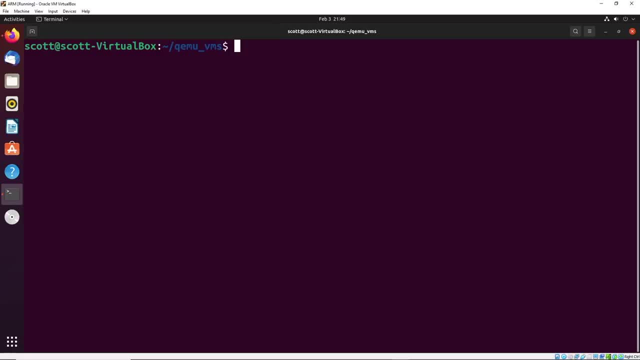 actual operating system is developed completely compatible with arm, which makes it a really good choice for us to actually program various different arm things on it. Now, of course, there's lots of different operating systems that use arm. However, this one is one that is lightweight, it's easy to emulate and it will support everything that. 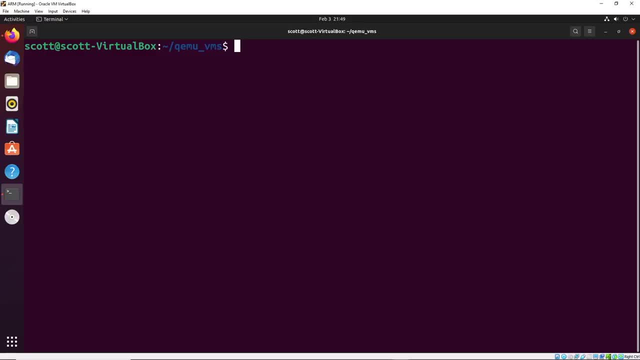 we need. So it's a pretty decent choice for our purposes. Now, the reason why we're choosing to emulate these operating systems is because I'm aware that most people probably don't have an arm device lying around. you know, a Raspberry Pi isn't too expensive, But of course it's a little. 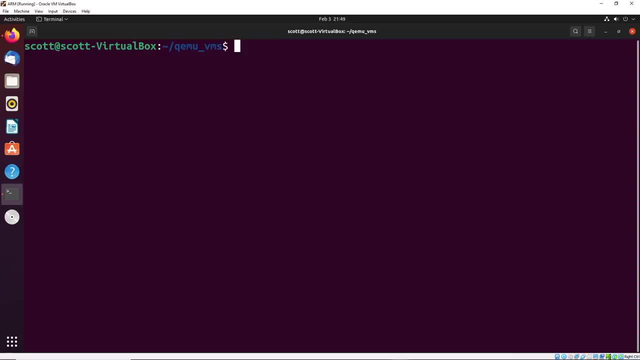 bit much to ask someone to go out and buy a device to learn arm assembly. And, of course, if you're going to use an arm, you're going to want to use an arm processor. So I'm going to show you how to emulate it, so that you can just write it on your computer And then at some point down the line. 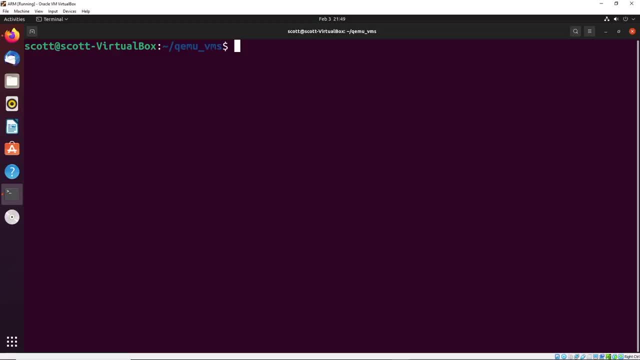 if you want a physical device, you can go out and get one of those, knowing all the arm stuff that you will know from these videos. So for the purposes of this video, I'm using VirtualBox. I have an Ubuntu machine. it's running Ubuntu 20.04,, I believe, and it is a 64 bit operating. 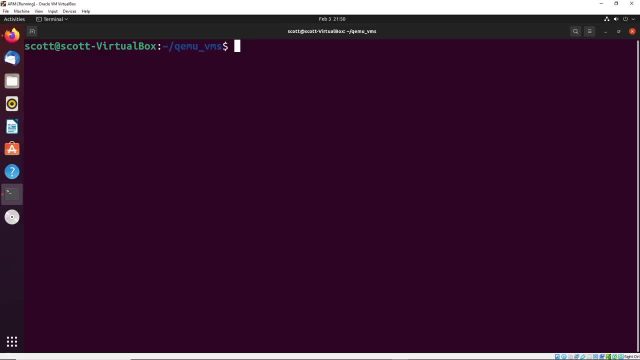 system. you should be able to follow along on any Linux system. the instructions are actually fairly straightforward. So let's go ahead and get started. So let's go ahead and get started And jump right into it. What you're going to want to do is you're going to want to download two 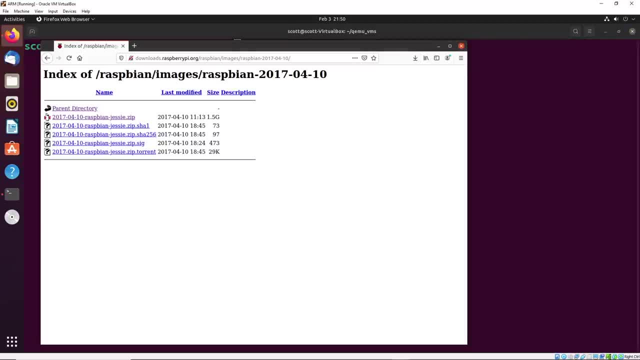 files onto your computer And I'll put links to them into the description. The first file is from this downloadsraspberrypiorg, And the file is this: 2017 0410 Raspbian Jessezip. This is the operating system image that we are going to use in order to work with emulating this operating. 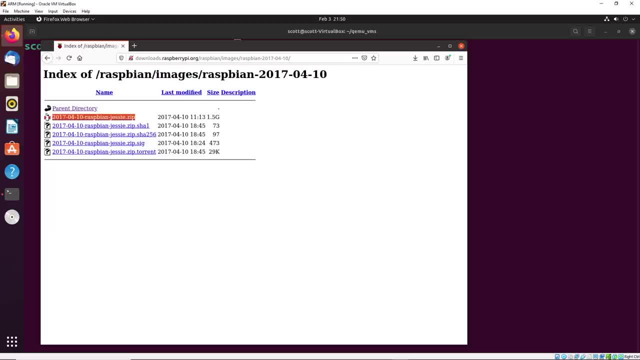 system. There are other versions of it. there's more recent versions. this one is the one that seems to work most stably with QEMU, So it's the one that I am going to be utilizing Now. in addition to this, we're also going to need a kernel that is working for this operating system. 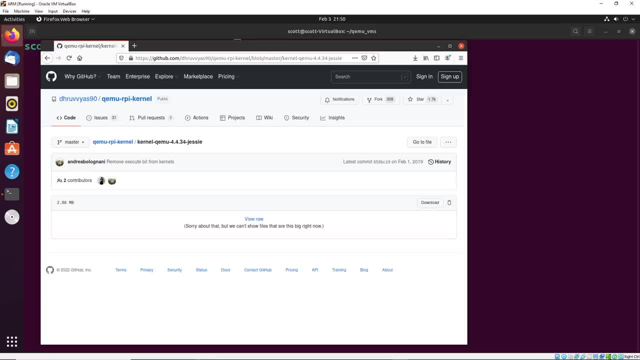 And we can get that from this GitHub link. Again, I'll put this into the description as well. This GitHub link is going to give you this QEMU 4.4.34 hyphen Jesse file, If you go to the root of this. 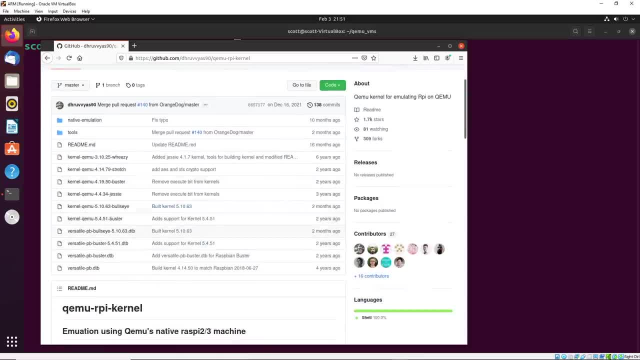 you can actually see all the different kernels that we have, So we have support for a variety of different types of kernels. This one is the one that corresponds with our operating system, though, So we're going to go ahead and download this one. 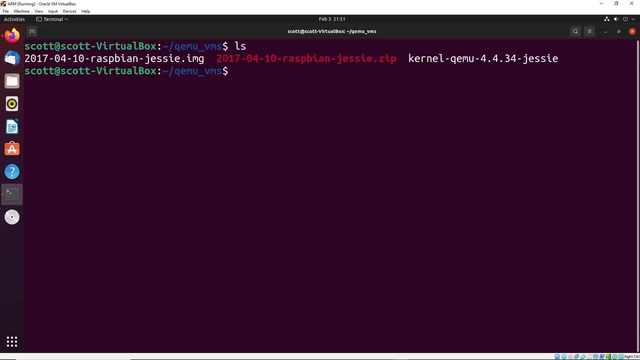 Once you have these files downloaded, I've placed them inside of this QEMU underscore VMs folder. you can put it anywhere on your computer, doesn't really matter, And you're going to want to unzip this 2017 0410 Raspbian Jessezip file to turn it into that IMG file that I have in a directory as. 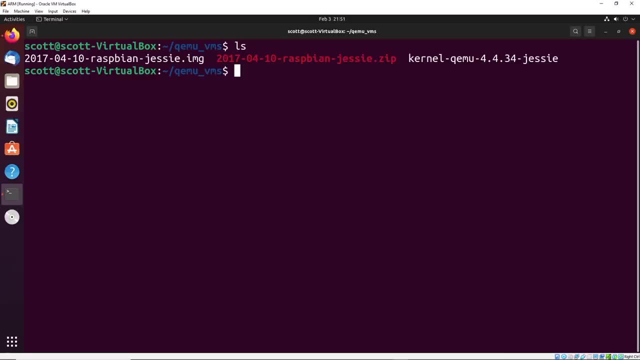 well, Once you have this available, I want you to install QEMU, And you can do that using sudo apt get install QEMU system. So I've already installed this. it will take a number of minutes on your computer, depending on how fast it is, And then, once it's completed, you will be good to go Once you have. 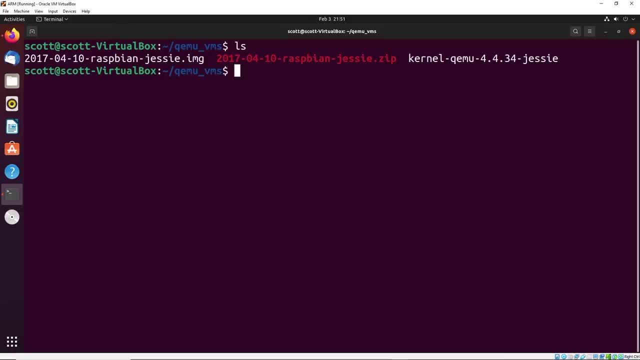 that all set, we're going to go ahead and just run our emulator, And the way that we do that is we say QEMU, hyphen system, hyphen arm and then hyphen kernel, And I'm going to direct it towards the kernel that we downloaded, which is in QEMU underscore VM slash kernel- this file here. 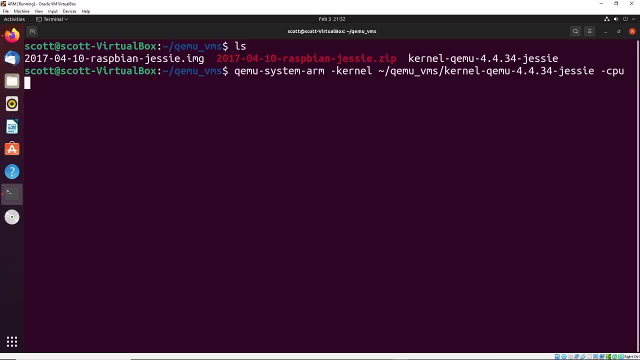 We then want to give it the CPU that we want to use for the emulation. I'm going to use arm 1176.. Again, this is the one that seems to work most reliably with this particular distribution, So it's the one that I will show. hyphen m is the amount of RAM or virtual RAM that we want to. 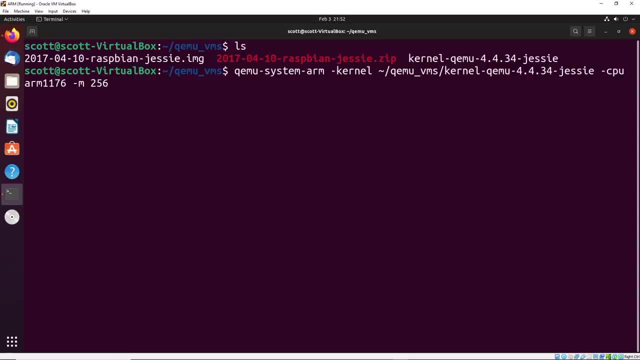 allocate, So I'll say 256.. That's a good size for this hyphen. capital M is the emulated machine type we are going to use: versatile PB. This one is just like one of the various types that's available with QEMU, Again one that works very well for this particular example. we're going to 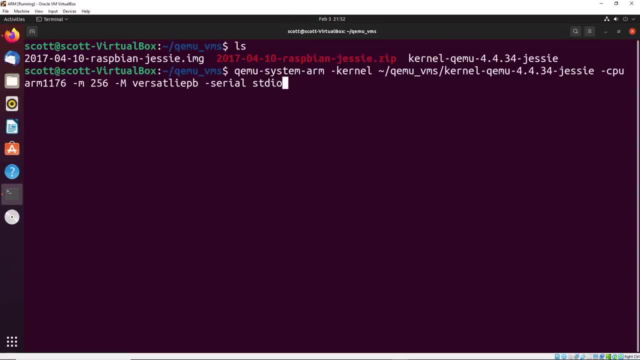 provide a serial as a CDIO just to allow everything to work through our standard input output. And then I'm going to use the append command to append the following: we're going to say root dev SDA to root fs. type equals ext for read writes. This just helps us set up the general file system. 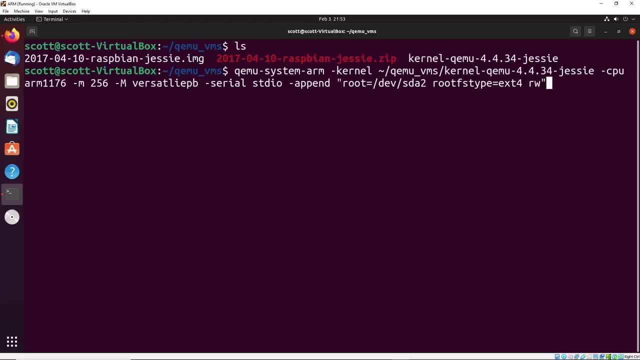 that we're emulating. So this gets everything set up the way that we need it, And I'm going to put hyphen HDA and I'm going to point towards the ISO that we have on our computer. So that is in QEMU underscore: VMs slash 2017.. This one here, dot img. 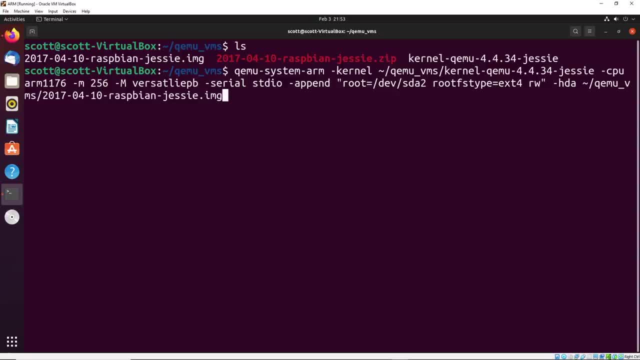 And then, finally, what I'm going to do is I'm going to forward a port from this computer to our SSH port, which is 22 on our machine. The reason I'm going to do this is because when you work through QEMU, it's a little bit hard to get things to full screen properly. 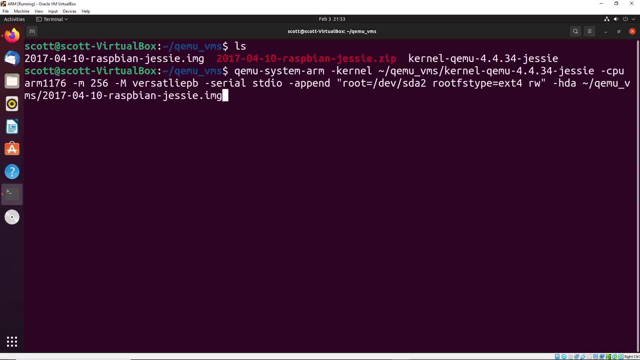 So rather than doing that, what I'm going to do is I'm going to SSH into the emulator through my virtual machine here. So to do that, we can just do the following: we do hyphen. Here's a user comma of hosts, forward equals TCP, and then two colon and 502 to 22.. So 22 is the port that 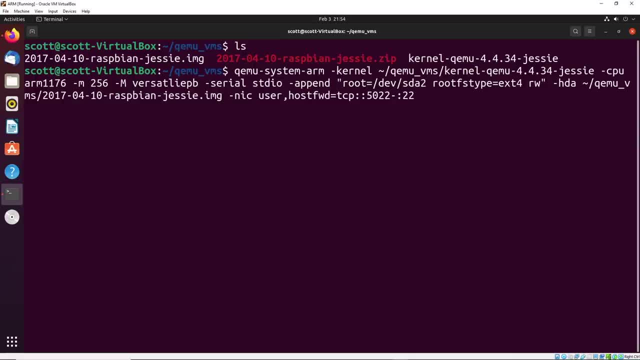 we're forwarding. So that's the SSH. port 5022 is the port that we're forwarding too. so when we want to connect to ssh on this computer, we're going to use the port 50 22.. so that'd be the idea of this. and then, when we launch this, we're going to say: no reboot, uh, just. 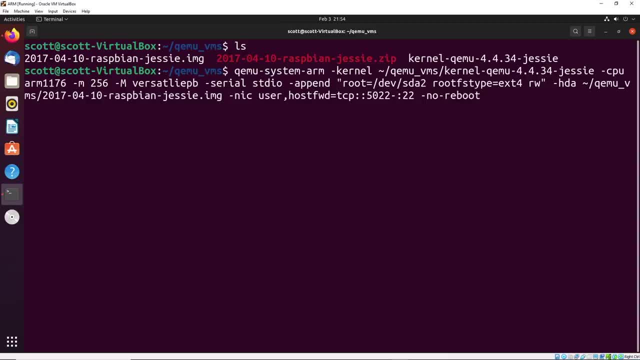 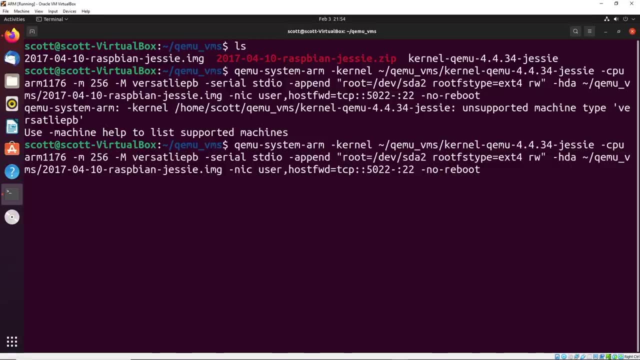 because i don't want the system to actually reboot, i just want it to boot as is. once we do this, um, it looks like maybe i just uh spelt this wrong. uh, the machine type, uh, let me just double check. it should be versi, uh, versatile. yes, it's about wrong. so you versatile pb like this. 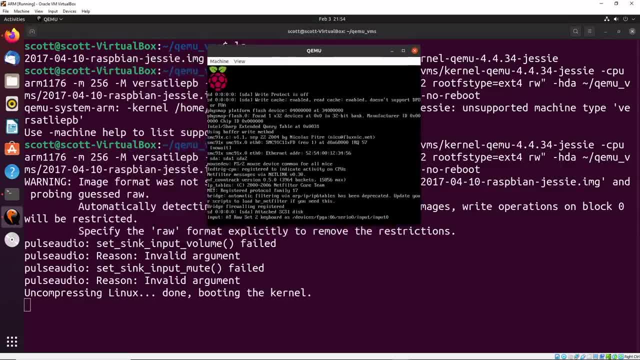 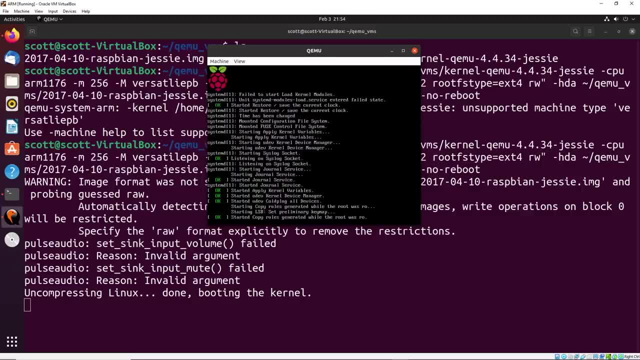 now, once we run this, you should see that your qmu starts to boot. so this is booting into the raspberry pi operating system. if you've gotten this far, congratulations. you now have a raspberry pi machine running on your computer. um, i will note that it's a little bit tricky to get this working reliably. i am able to get it working. 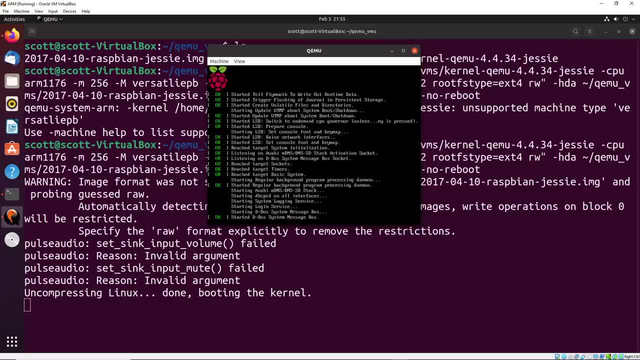 reliably every single time. so i'm going to go ahead and do that and i'm going to go ahead and start the main Gröner code and i'm going to just go ahead and run this thing and see what happens. time that i've tried it so far on my computer, which is why i'm showing this set of instructions. 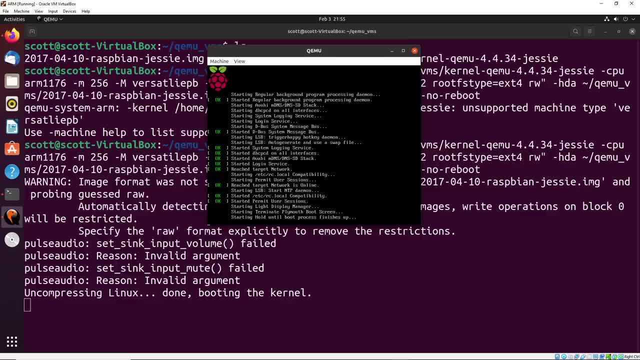 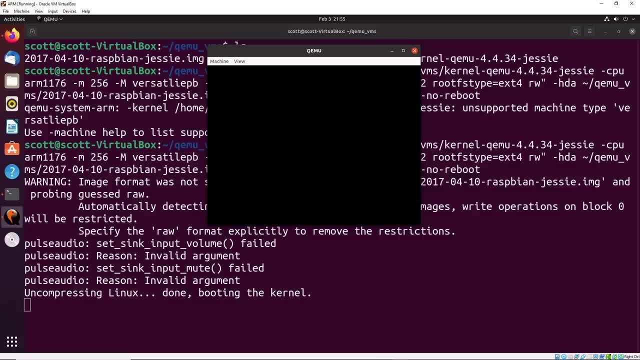 if you have any troubles with getting things set up. it should be relatively easy to troubleshoot the errors that you're getting, but feel free to comment them as well, and i will try to help you out as much as i can. i also plan to try to post this image, if possible, somewhere, so that 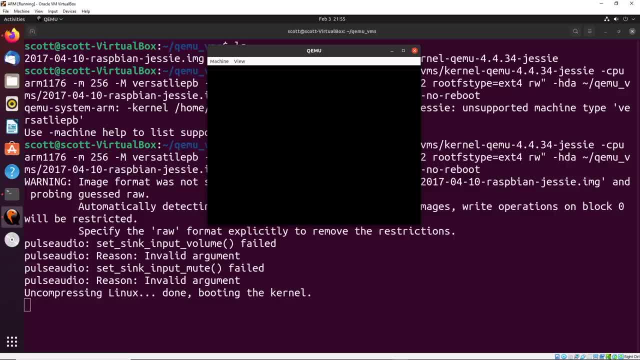 it's able to be downloaded, so keep an eye out on the description as well. i'm going to try to put a link to this virtual machine image so that you're able to access it and use it rather than having to do all these things later on, and keep that in mind if you are not familiar with this. 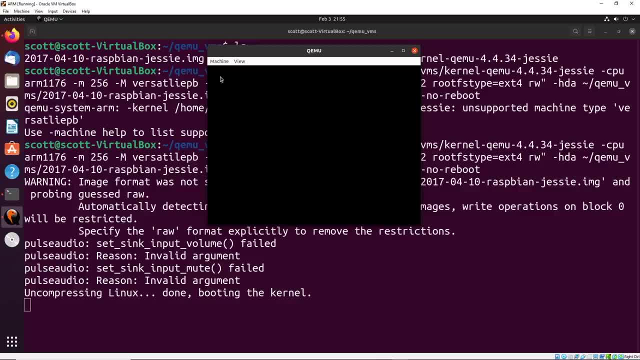 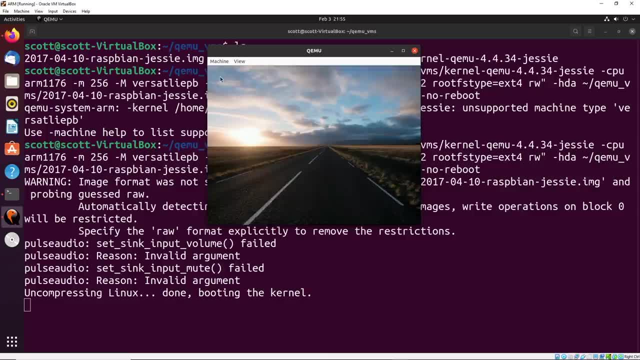 this setup yourself. That way you get one that is for certain working through VirtualBox, And then from there you can just sort of fiddle around and get it to work on your particular system. There's a few things like setting up emulation inside of emulation, like allowing 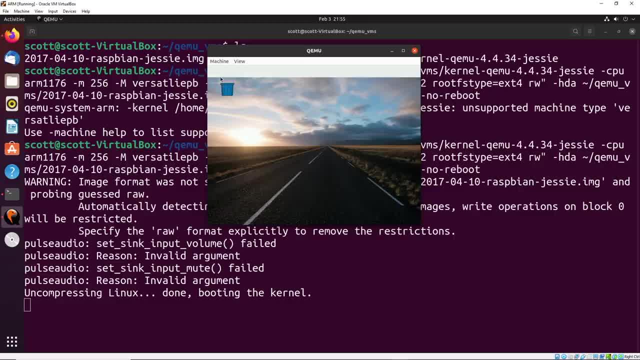 VirtualBox to run emulators like this. there may be some settings that you need to tweak in VirtualBox to get that to work, But regardless again, it should be relatively easy to get set up. If not, just feel free to leave some comments. I'll try to help you with troubleshooting some of 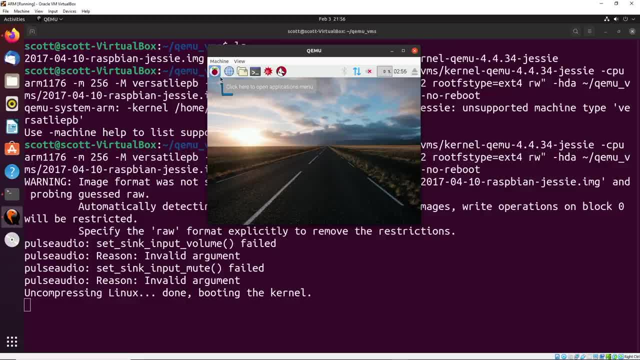 those errors, if possible. So once we have things set up here, what I'm going to do is I'm just going to run the following command: I'm going to open up the terminal on this emulated device And what I'm going to do is I'm going to forward SSH on it. So I'm going to say: pseudo service. 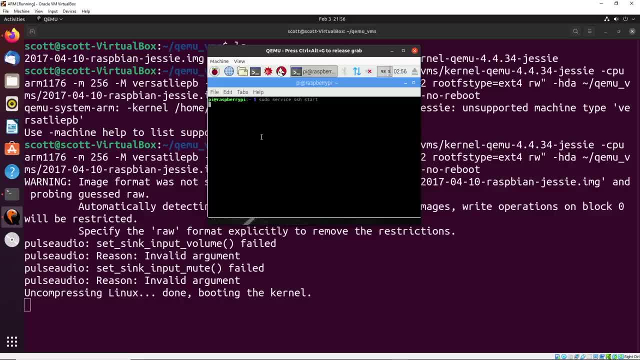 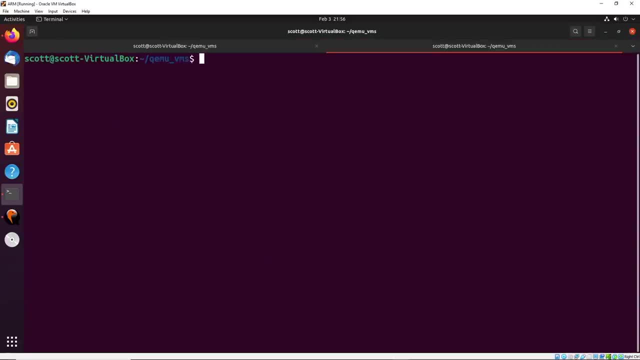 SSH start. Once that runs successfully, we're going to just try SSH into this machine through my computer and see what happens. So it looks like everything is good To go. I'll create a new tab here. Let's zoom it in a little bit. I'm going to SSH pi 127.0.0.1.. 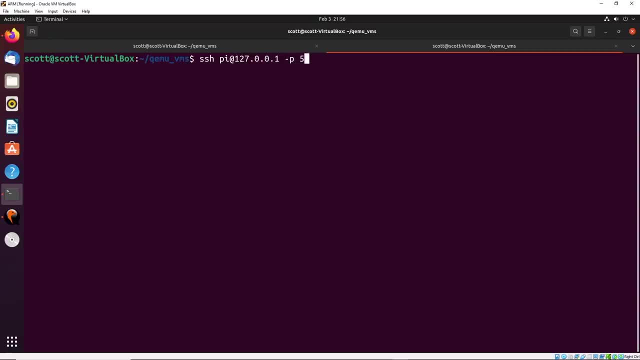 And then the port, like I said before, is going to be 5002 or 5022.. Rather, When that goes through, ask you if you want to continue. you can say yes. The password for this is Raspbian, RAS or sorry. 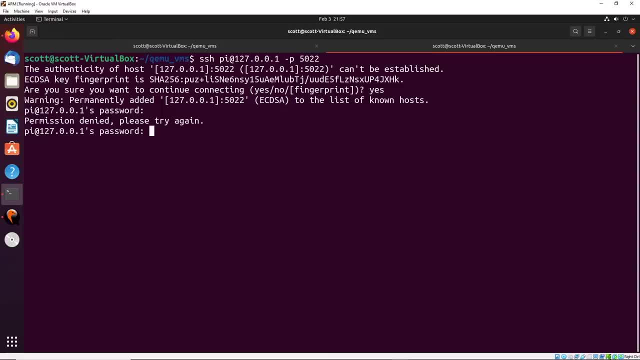 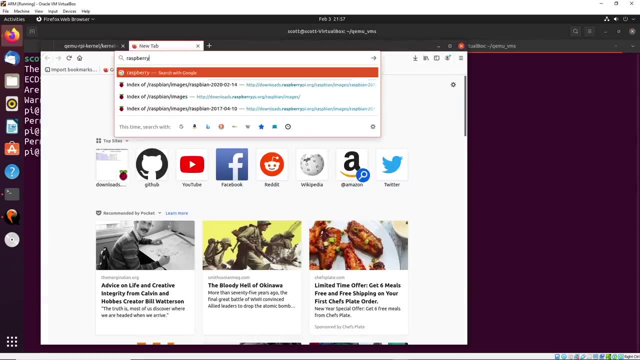 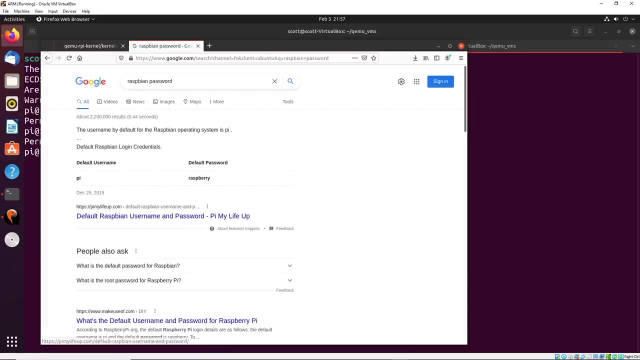 it's. I think it's Raspberry Pi. Okay, well, let's, let's double check and see what it is. You want to say Raspbian password? it should be raspberry, So raspberry should be the default password. Let's just try that. 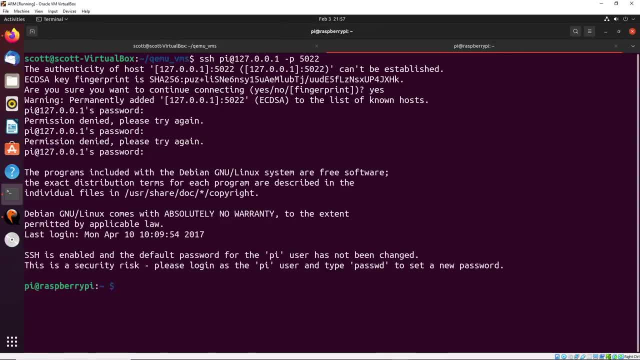 There we go. So now it has brought us into our device And we are now inside of our emulated device. So with this we now have an ARM device that is using the same application as the source, I guess. So let's go ahead and try this out. I don't think anything has changed At this point. 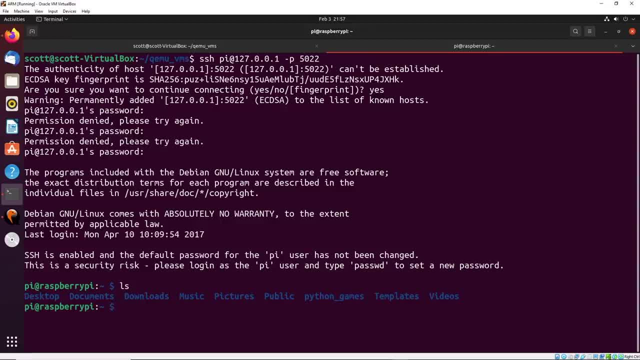 So with this, we now have an arm device that is running on a Linux system, And now we're going to be able to do a lot of really cool and interesting things with arm. we're going to learn about things like system and software interrupts, And we're going to really just 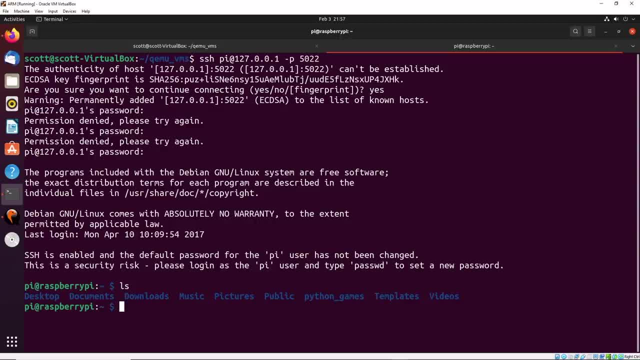 build up a lot of operating system understanding as well and really dig deeper into the sort of things that we can do with arm assembly. So thank you for watching this video. I hope that you enjoyed it Again. if you have any sort of trouble throughout this process, please do leave comments. 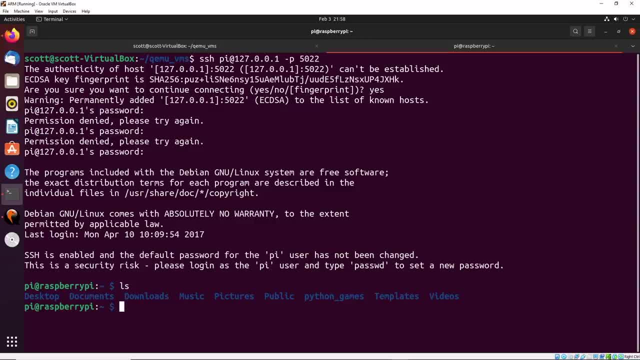 let me know. I'll try to help out as much as possible, And I'm sure some of the other viewers will be able to help out too, And then we'll be able to get things up and running like this, And then we'll be able to learn all these different operating system techniques. So again, thank you. 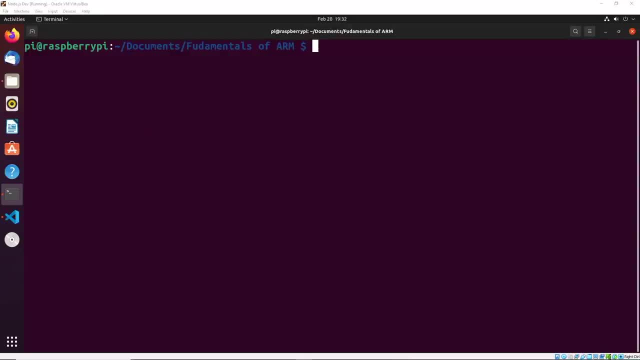 for watching and I'll see you in the next video. In this video we're going to start to take a look at operating system interactions by seeing how we can output data onto the screen. So we're finally going to do like an actual formal Hello World program where we 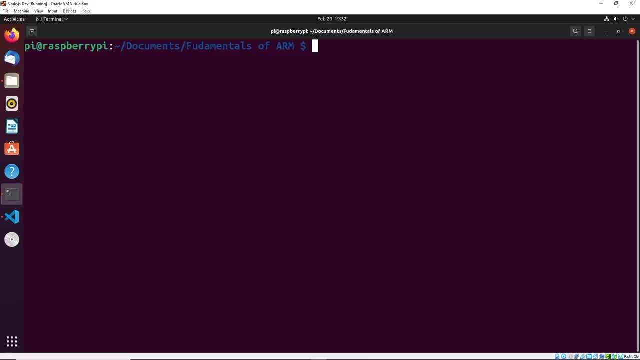 output Hello World onto the screen. And while we're doing this, we're going to explore the ideas of system calls and system interrupts done through our assembly. So let's go ahead and get started. For the purposes of these videos, I'm going to be working through our Raspberry Pi. 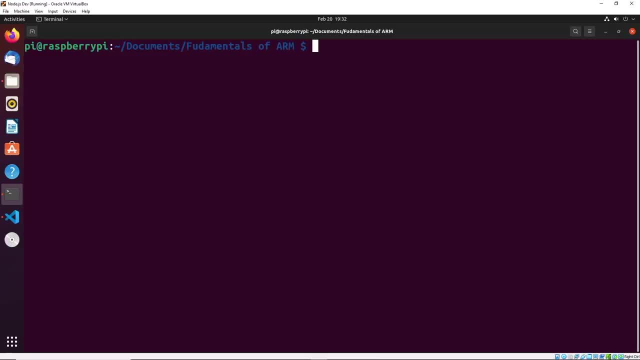 In this case I'm actually logged onto a physical machine, But you can use the emulator we set up in the previous video, Or you can use a physical machine of any kind that has an arm processor. If you want to follow along on something physical, the choice is really yours. it should work on. 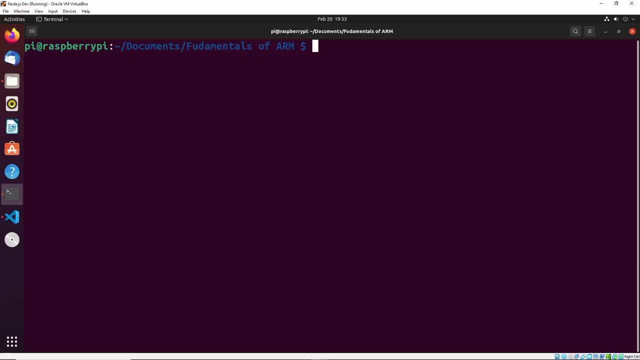 your device. So we're going to start off by creating a new file which I'm going to call Hello World. I'm going to do that through the nano text editor And it's just my text editor of preference. you can use whatever you prefer. The extension for this file is dot s. dot s is the typical file. 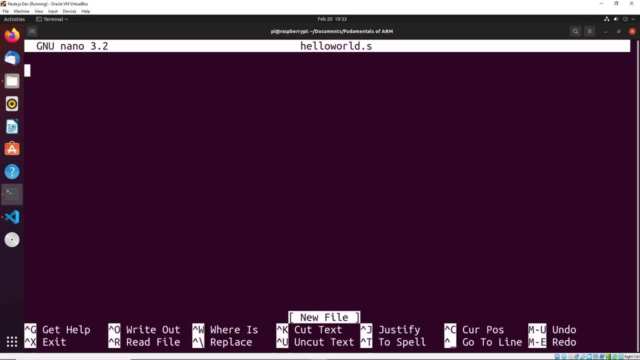 extension for assembly based programs, And what we're going to do here is we're going to set up our program in a very similar way to what we have done in the emulator past, right, So let's take a look at how we set that up. We say dot- global underscore- start. 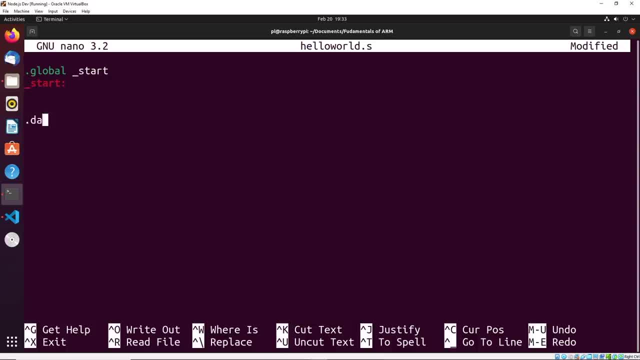 Start label And then for this we're going to need some data, And the data is going to be what we actually want to print onto the screen. I'm going to do that declared as a message. Now we want this message to be text. there's a lot of different ways that we can declare text in arm, And I want to 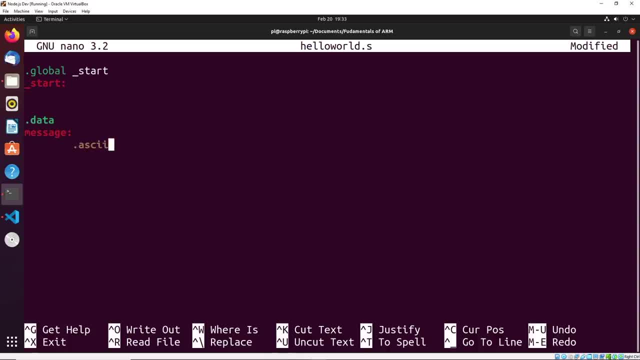 discuss each of them Now. the most basic type of text type is ASCII. ASCII is just general characters, And there's something about the ASCII format that doesn't really work well for a lot of text applications, And that is the fact that it is not null terminated, And what that means is basically in some lower 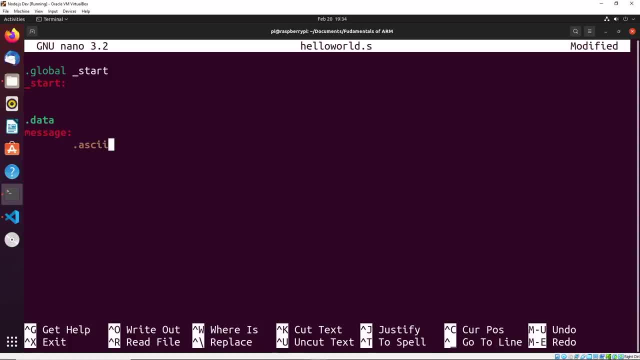 level programming languages. if you've programmed in C, you'll be familiar with this idea. When we create a string- since it's really just like an array of characters- we have something that indicates the end of the array of characters Because, of course, as we're going into memory in 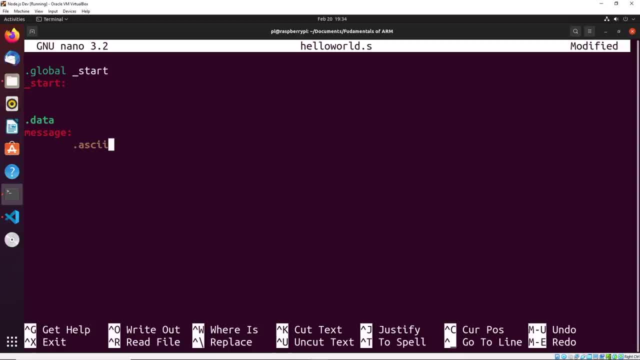 memory. it's not always predictable what an empty slot of memory will contain. So what we do is we pick a special character that indicates the end of a string and we call that the null terminator. So it's a special character set aside that always indicates the end of a string. 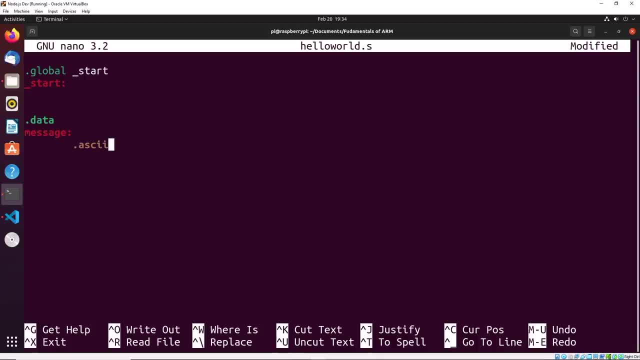 the ASCII format does not have that, So this sort of format works best for things like individual characters or situations where we don't need the null terminator. In almost every single case, though, you're going to want to have a null terminator for your string, So instead we're. 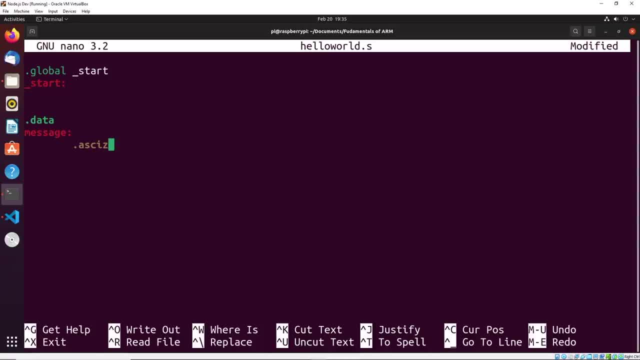 going to use this here- ASCII zed, I'll call it- And what this does is it declares a string, but it adds on a null terminator at the end, Which allows us to know where the end of the string actually is. Now, one other note that I want to make. 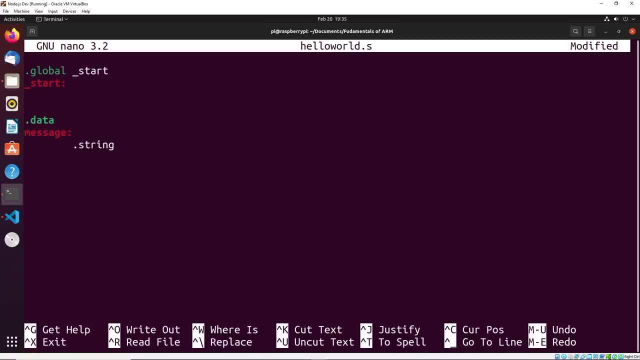 here is. sometimes you might see dot string. dot string is actually an alias for dot ASCII zed, So dot string is the same as this declaration here. So I just want to note that, just in case you ever see dot string. it's the same as this dot ASCII zed, So those are the same as each other. It's a. 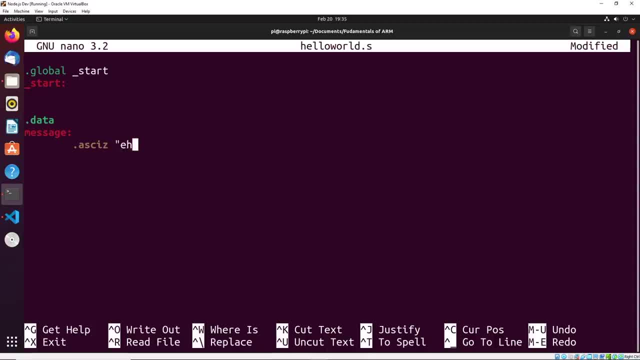 null, terminated string, And then from here we could just type in the name or what, what text we want. right, world, I can put backslash and we can put this new line character, And so all that does is it indicates a new line. backslash n, And essentially we can add that in because it will get interpreted. 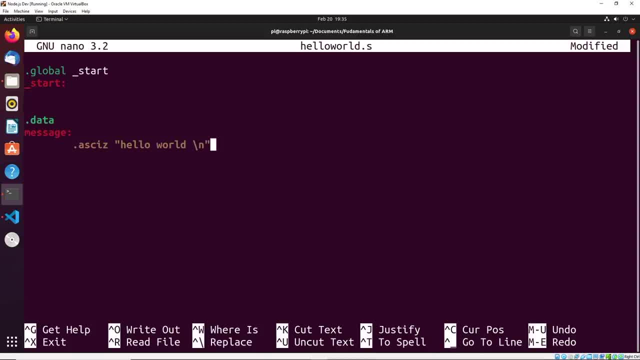 through the operating system to write a new line character, So that's something that we're able to put in as well. Now. I will eventually show you what this looks like in memory, But for now we're just going to sort of take this for granted and say, Okay, this will work And we will continue on. 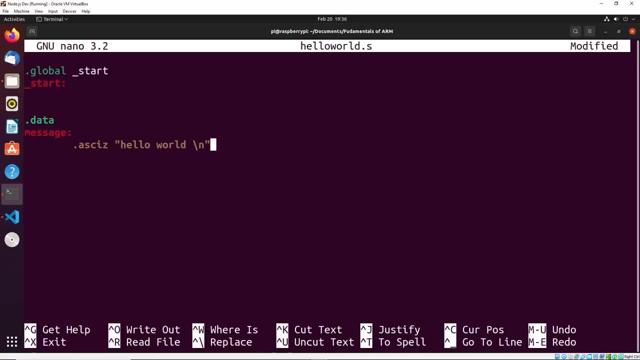 with this. Now, one other thing that I wanted to show you is that, if you want to add a new line note, is that when you, when you make the call to write data to the screen, in this case- which is what we're going to be doing- we're actually using components of the Linux operating system, which is 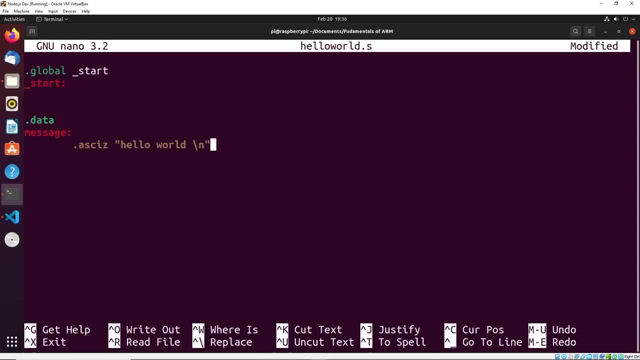 really interesting sort of idea. So you'll see that from this point on, when we start using the system interrupts and system calls, there's gonna be a lot of parallels between assembly and C. So if you're familiar with C, it will be very helpful for you, If you're not familiar with C, not to 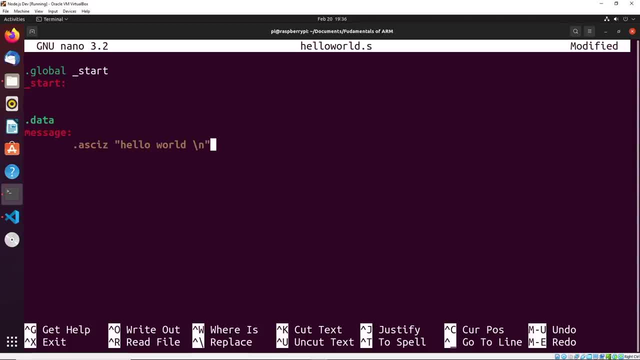 worry, we will eventually discuss C and its consequences In future videos as well. So once you've declared the text here, what we could do is we could declare the length of the text So I could say: le n equals dot minus message, What this is going to. 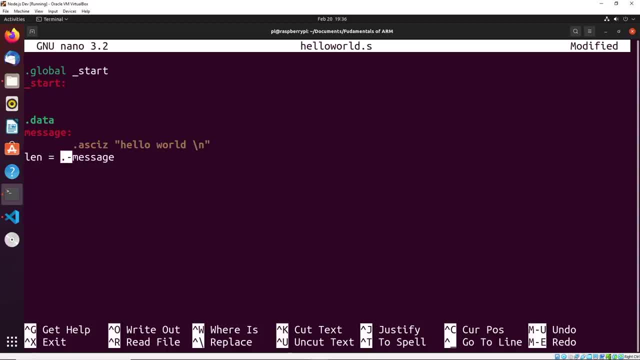 do is it's going to declare a variable called le. n is going to be equal to the length of message. this is the way that we declare that. the way that this works is it starts at the beginning of the text, So it starts at this H character here And it continues moving through it until 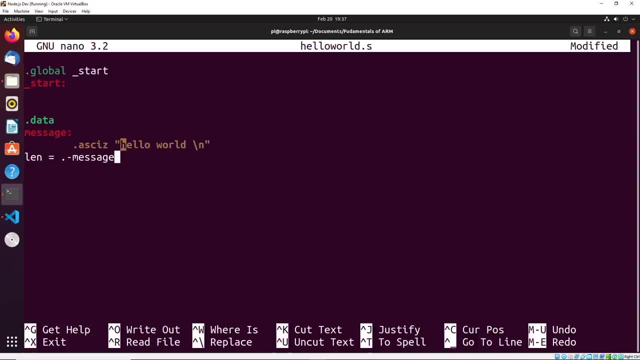 it reaches that null terminator that I mentioned previously. Once it reaches that null terminator, it knows it's reached the end of the string. that is the length, and it stores the length in this le n variable for us to use. So that is all the data that we're going to need to create our Hello World program. 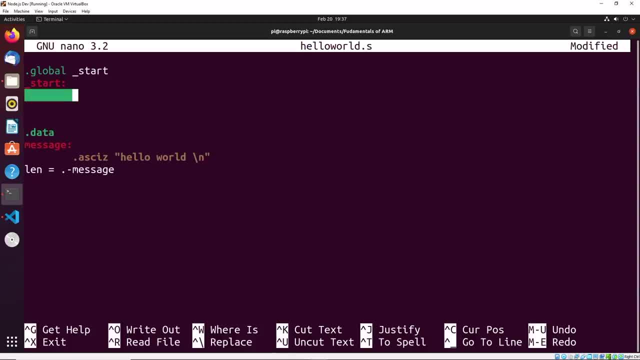 Now, in order for Hello World to work, in order for us to write data to the screen, we're going to need to declare and have ready three different pieces of information. The first piece of information is: where do we want to write the message or text or data to? 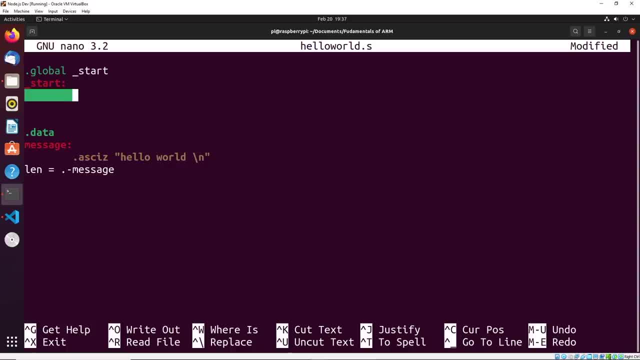 The second thing that we need is a reference to tell us what one, what we want to actually output. And the third thing we want is the length: how long is the thing that we want to output? And those are going to be stored in very specific locations, So we're going to move. 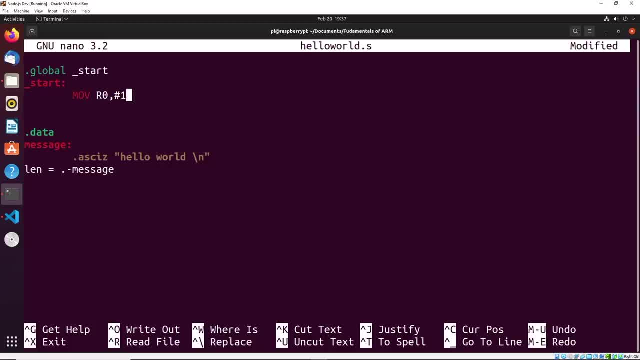 into our zero, the value one. this one indicates that we want to place, that we want to place the output in the standard output for our computer. So this would be the standard output, which is where all things output by default, in the case of me being SSH into my actual computer. 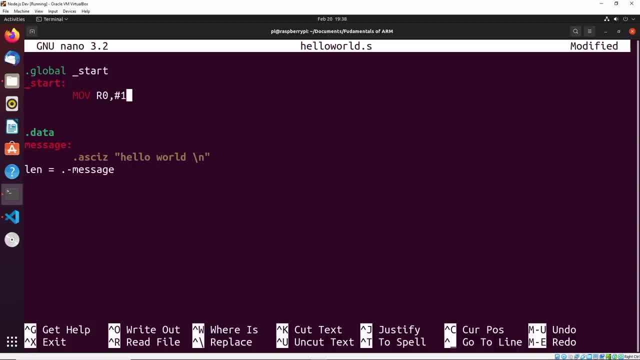 the standard output would typically be the command line interface, So I'd be without an output. So this is generally the way that we output things into the standard output. we can output to standard in by using zero as our argument. we can output to standard error. 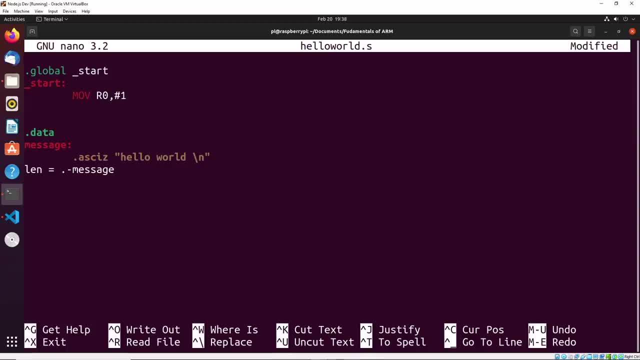 using two as our inputs. Now, in general, we can also add in different values other than zero, one and two. this will actually take in any valid file descriptor as a an argument, So we can actually write the files as well. For those of you who are not as familiar with the Linux operating system, 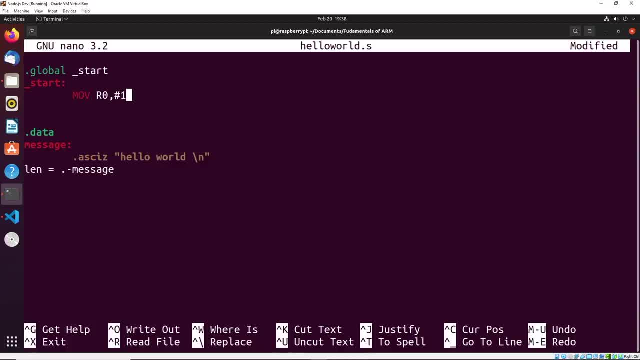 in the background. what Linux does is it assigns things called file descriptors to the files on the system. What happens is, when you open up a file, we are given a unique identifier for that file, which is typically represented, I believe, as an integer, And that allows us to know where. 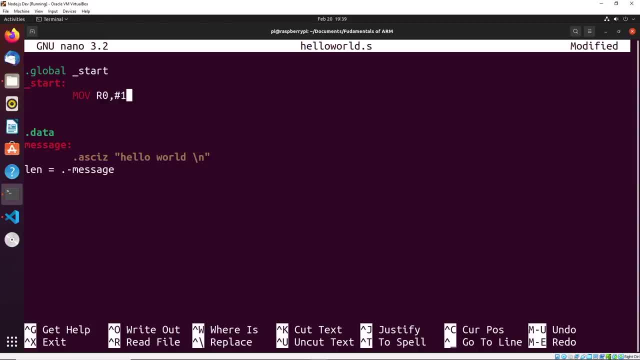 we're reading and writing from. So whenever we make calls to read and write, we're going to get in right to files. we use this file descriptor, which is an integer which uniquely identifies the file. Because this R zero is taking in some integer value we can actually provide it with. 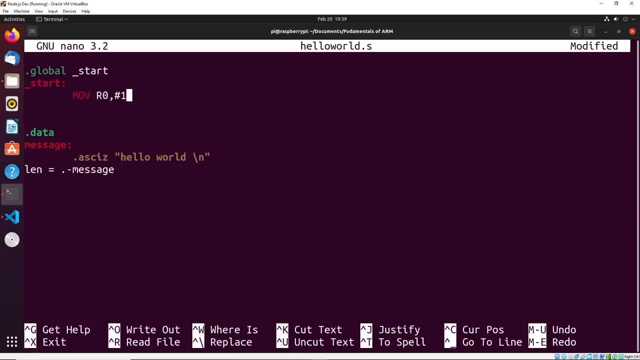 any file descriptor of a file on our system and it will actually write to that file. So that's something that's interesting about this. Now, like I said before, we also have to give it the value that we want to print as well as the length. So we can do that using LDR. So I can LDR into our 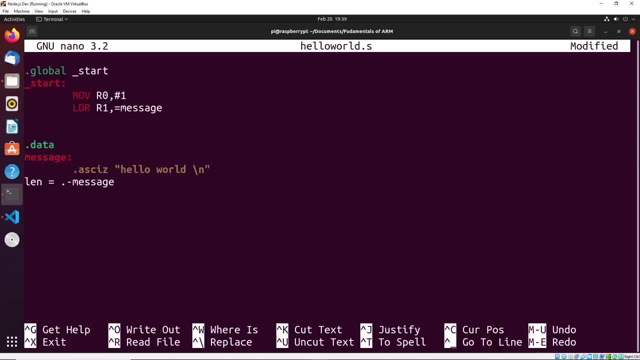 one, the message. So it's going to load the address of message, like we've discussed previously, into our one. So I'll tell it where message is currently located in memory. So it's kind of like a buffer right. It tells it the buffer location of the message And then what? 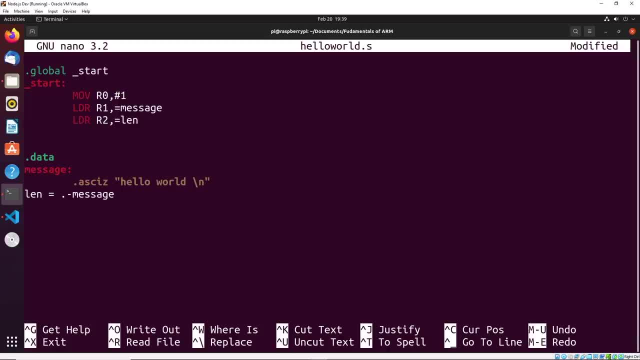 we could do is we can LDR into our to the value of length. this places the length into register two. So now we know the length of the actual string itself, we know the actual string that we want to print and we know where we want to print it. The last thing we need to do is tell the 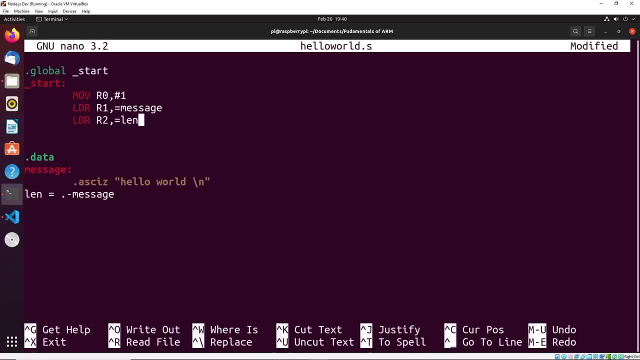 computer to print the thing to the screen. Now, the way that we do this is actually quite interesting. What I'm going to do is I'm going to move into our seven the value. for now that might seem a little bit random. what's happening here is when we communicate with 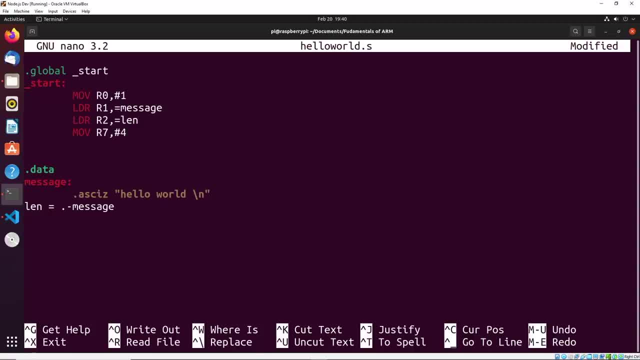 the operating system. our seven is a special register that actually keeps track of what we want the operating system to do. So when we do an interrupt which will allow the operating system to take over the processing, what the operating system is going to do is it's first going to look. 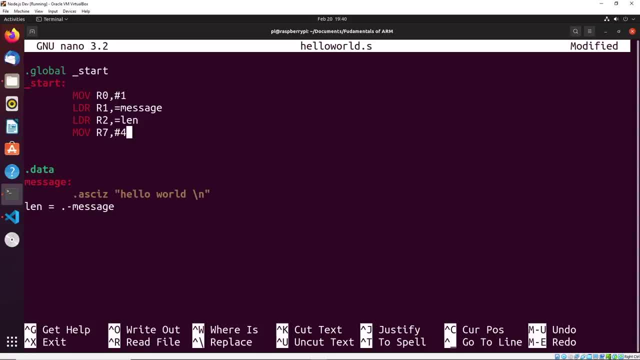 at register, our seven- and it's going to check what number is the number of. the number of the data is written there. that's going to tell the operating system what it needs to do next when I give it the value for what the operating system sees, as it sees that I want to write. 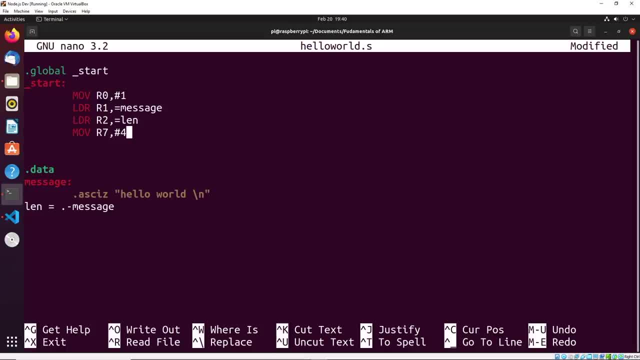 something to the screen. it's then going to take a look at our zero, our one and our two- to answer the questions of where to write the data, what data needs to be written and what the length of that data is. it will then write out the data and then it will return back to the program to allow. 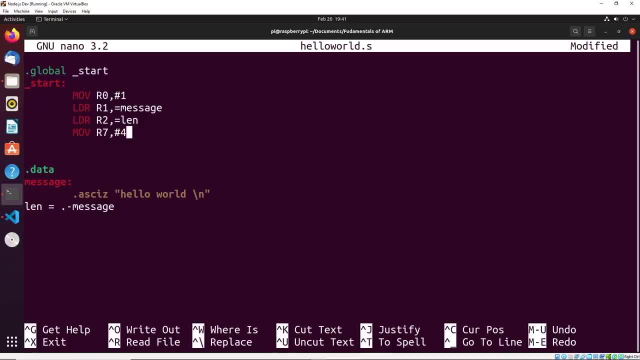 it to continue executing. That's the general flow of what happens when we do this sort of interrupt. If we want to go into a little bit more detail, we're going to go into a little bit more detail. what's actually happening here is: in Linux, there's a system call called right. What this? 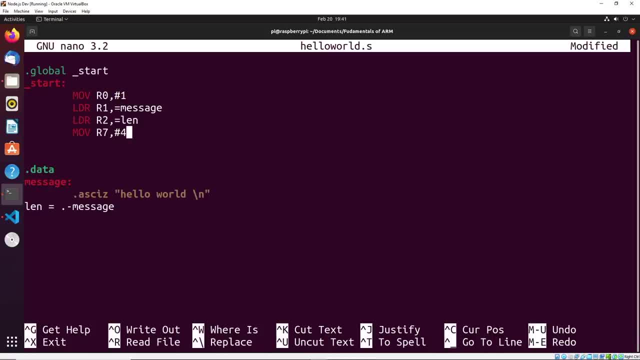 is doing is it's actually calling that right function? And again, if you have familiarity with C programming and specifically like system level C programming, you are likely familiar with the right function. you use that actually to write files on a Linux system. That's the same function. 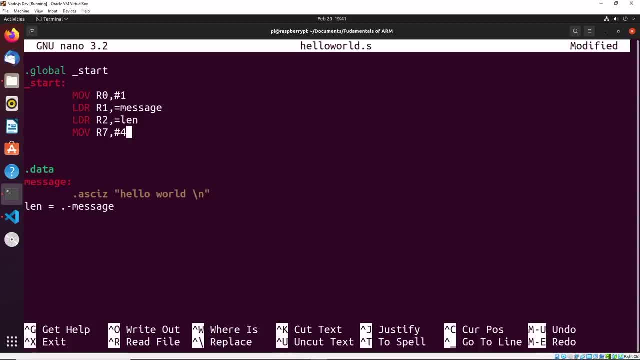 that's being called here. we're just calling it through a system call in a little bit more of an abstract way. So I just want to bring out that parallel, Just in case you're familiar with C programming, because it's a really valuable one to keep in mind. 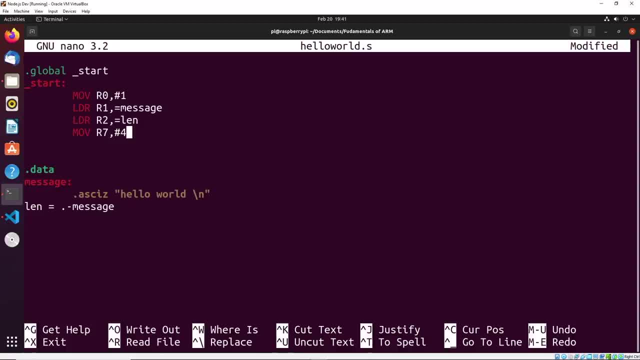 that we are actually able to communicate with the system calls in this way. So we've set up the value that is needed in order to know which system call to make. Now we have to make the system call, which we do using SWI zero. SWI means software interrupt, So what it does is it interrupts and it tells the. 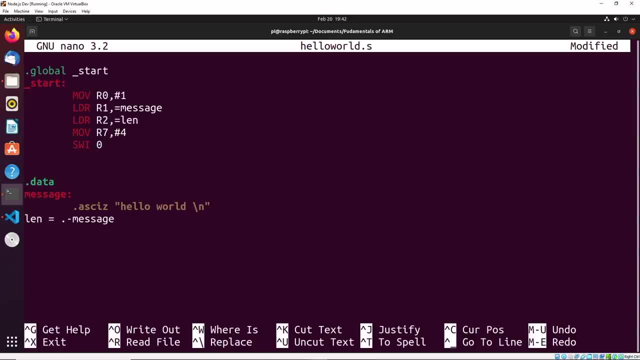 operating system. hey, we need you to do something. The operating system helps us handle hardware things like input and output, To do the output for us. Again, it takes a look at our seven. it sees the value for it says that's an. 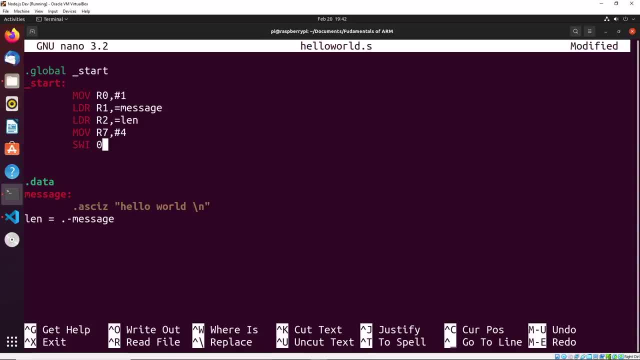 output. it then outputs based on our what, our zero, our one and our two values. Once that is done, it returns back to our program and lets our program continue to execute. At this point, what's going to happen is we're going to flow into the data and weird things are going to happen In order to 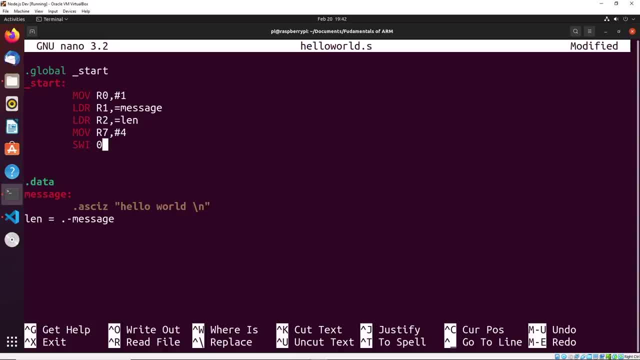 prevent that, we have to properly tell our program to exit, which hasn't been something that we've really had to do throughout the emulation type videos. To do that we do is we say: move into our seven, the value one, and then we do an SWI. So what's happening here? 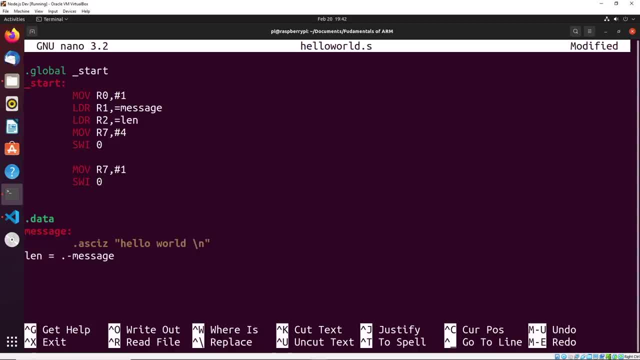 is again, we're telling the operating system what we need it to do. The argument of one is telling the operating system to terminate our program. So this time when we do our software interrupt, the operating system will interrupt. it will take a look at our seven. it sees one and it says: Oh that. 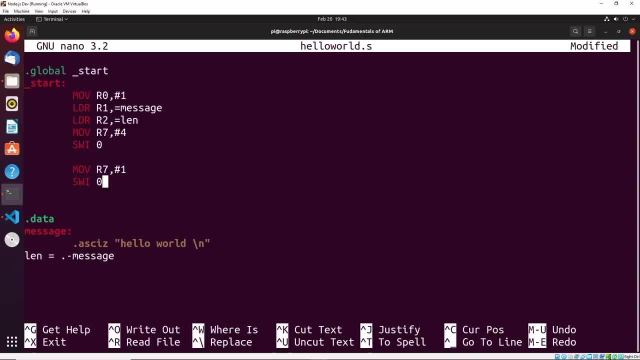 means I should terminate the program and it will terminate it and we will be done. So this is everything that's involved in creating our simple hollow world program. You can see it's not necessarily all that simple, But now that you have a familiarity with a lot of the general concepts of assembly, hopefully this does. 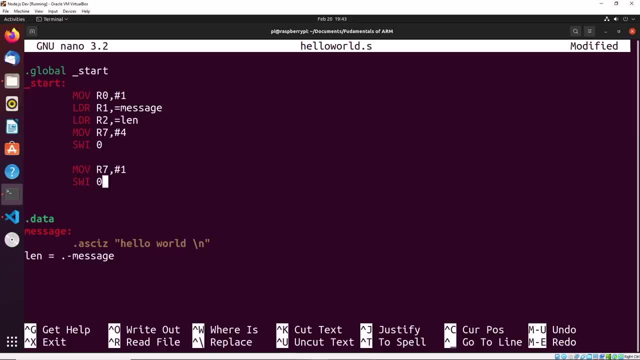 actually seem a little bit easy to actually do right. So a lot of these instructions are already familiar. There's a few new ones, a few new concepts, but this should be relatively straightforward, hopefully. Now, last thing that I need to show you here is how to actually run your program. We're 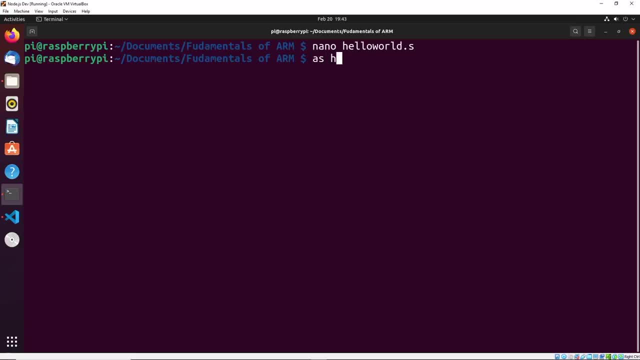 going to do two steps. we're going to first assemble the program, So we're going to do as usual. we're going to create a binary code, So we're going to write an object file. we're going to say Hello World dot s hyphen: O, hello world dot O. This is creating an intermediate for it file. 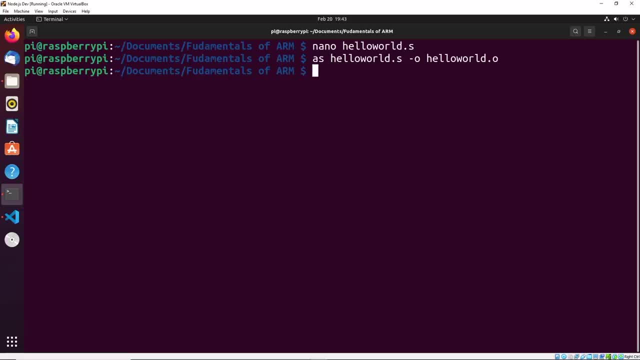 known as an object file. The object file can then be combined with other object files if required, and compiled into what is called a binary. The binary is what is actually run on the system to execute the code. So to create the binary, we do LD. 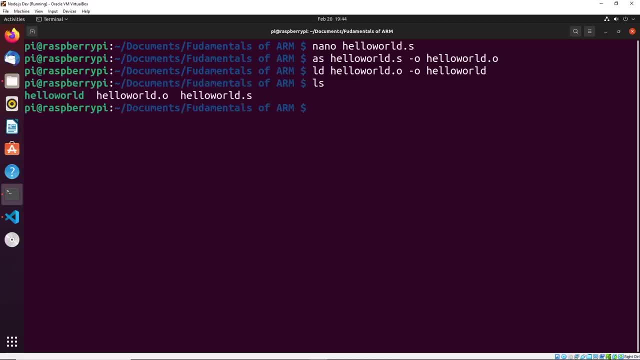 So you can see, right now we have three files. we have hello world, which is the binary I just created, hello worldo, which is the object file, And then hello worlds, which is our assembly code. Now we want to execute hello world. we do dot slash hello world And, as you can see, 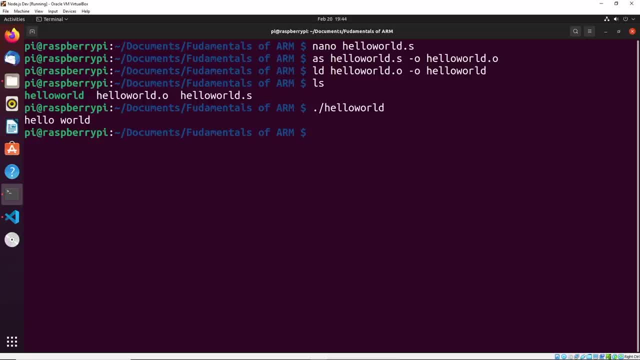 hello world is printed to the screen, So it looks like everything is working as expected. So from this video, you should now have a better understanding of how system calls work and how we're actually able to output data onto the screen. So thank you for watching this video. 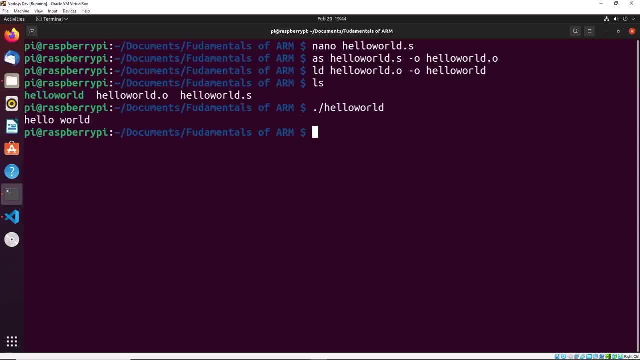 In the next video I'm actually going to walk through GDB to show you how you can get a better understanding of the actual layout of memory on this Linux system, Because you can't really see a lot of the details just running it. I want to show you how to debug and understand the code. 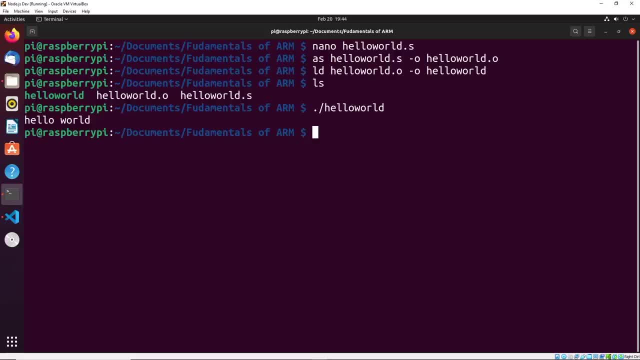 that you're running with a little bit better than what we have now. So thanks for watching and I'll see you in the next video. In this video we're going to take a look at how we can execute hello worldo, actually debug our assembly programs through the Linux command line. And what I want to do is I: 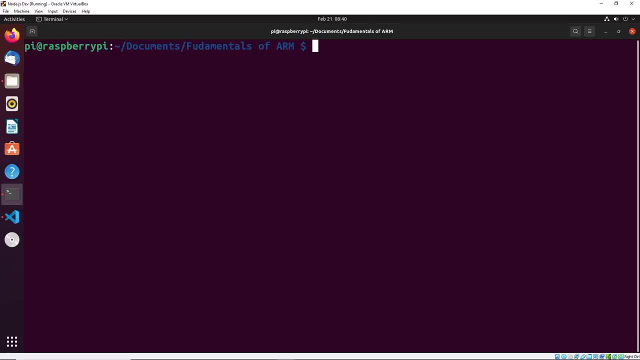 want to show you that a lot of the things that we saw in our online emulator can also be replicated through the actual Linux command line using programs like GDB, And that's primarily what we're going to focus on. we're going to take a look at the same program that we had before. 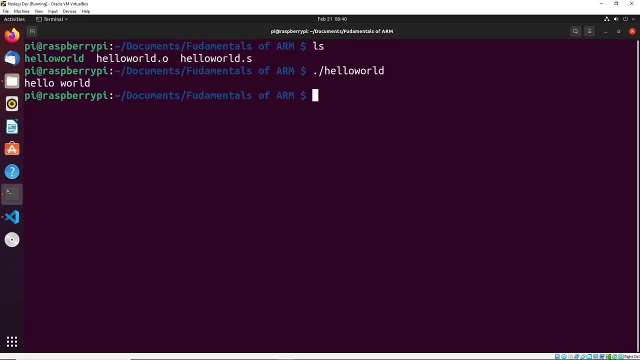 that was this, this hello world program that was able to print out hello world to the screen. I'm going to show you how we can step through it and see all of the different pieces that are required in order to make this work. So, first off, we're going to launch this program into debug mode using GDB. 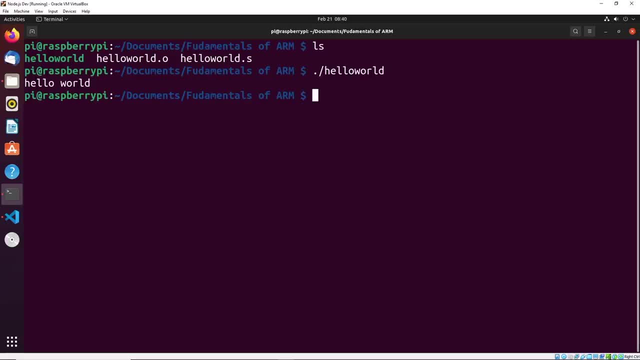 which is a debugger that comes typically default on most Linux distributions And it's a really valuable debugger for assembly, as well as other programs like C you'd often see it used with. So to do this, we just do GDB And then we type in the name of our program, which is hello world. 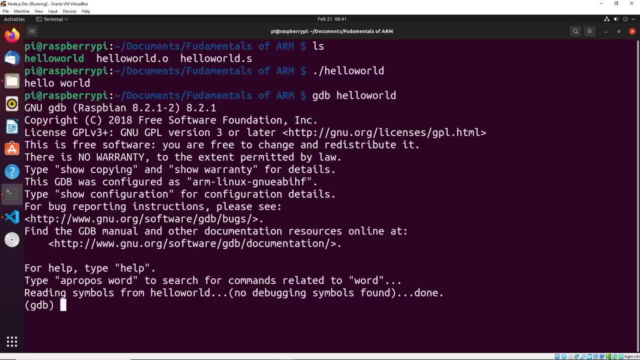 And you'll see that we'll get this screen that will say all this information about GDB and that it's been launched successfully. So, in order to get this running, what we have to do is we have to add in a breakpoint. What a breakpoint. 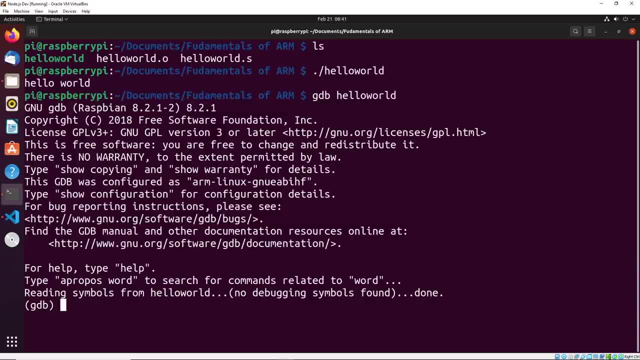 is going to do is it's going to stop the execution of our program at a point specified by us, allowing us to be able to see what the current state of the memory is at that point, and step through to the next instruction and continue stepping one by one, The typical thing that we 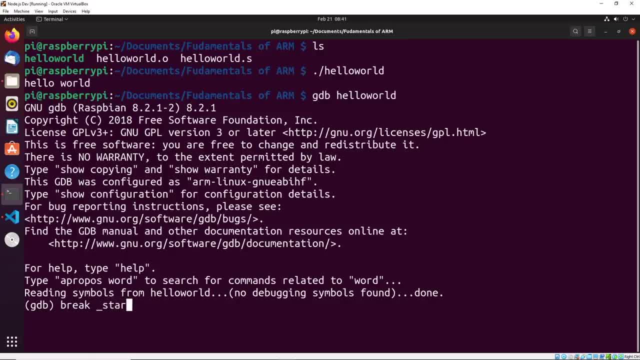 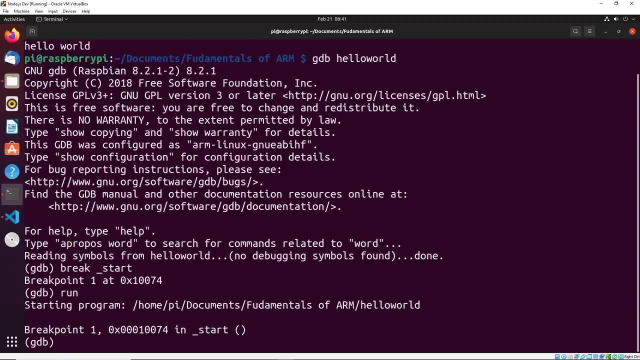 break on is we break on the start label So we break underscore start. So what this will do is, when we run our program, stop at that start label and allow us to start executing step by step from there. So once we have our breakpoint set, we could just type in run And you'll see that it started the program and it's hit. 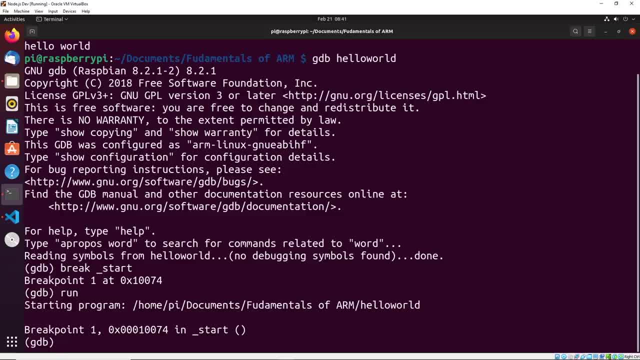 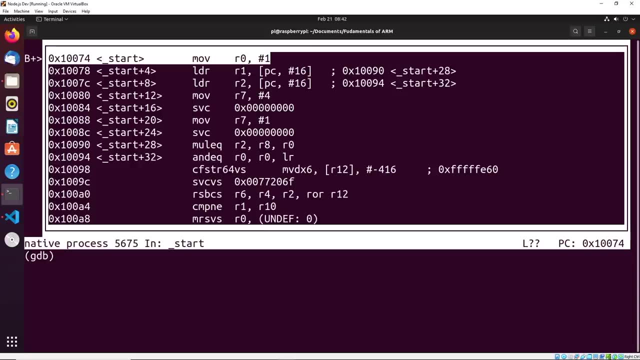 the breakpoint at start. Now you can't really see any of this information right now. So what we have to do is we have to change the layout of GDB So we could say layout ASM And you could see that this gives us a layout that shows all of the instructions in our application. So you can see the 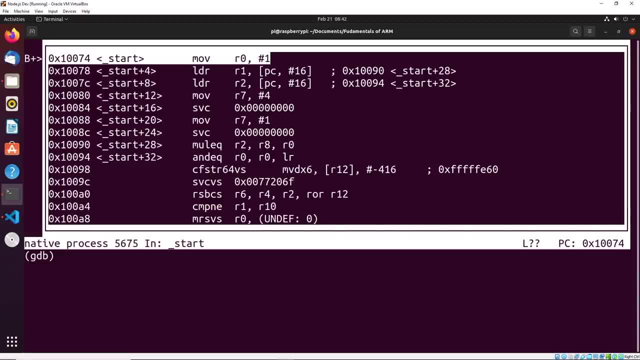 first instruction which is moving one into R0.. And then we have the loading of our strings and our length, And then we have our system call And then we have our end of our program with the system call for that. So this is giving us an idea of how we can actually look at the instructions that. 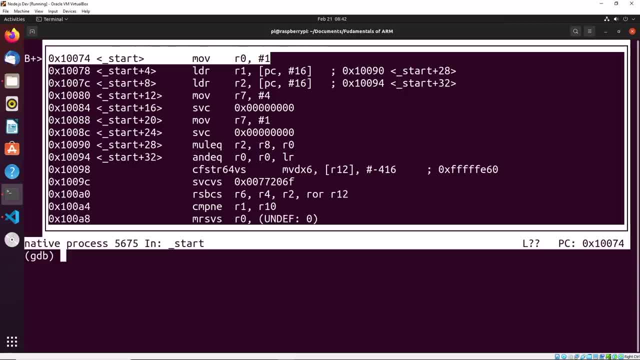 are associated with our program. Now the next question is: how do we see the registers? there's two different ways that you could typically see the registers. The first is you could say info register and then type in the register that you want. 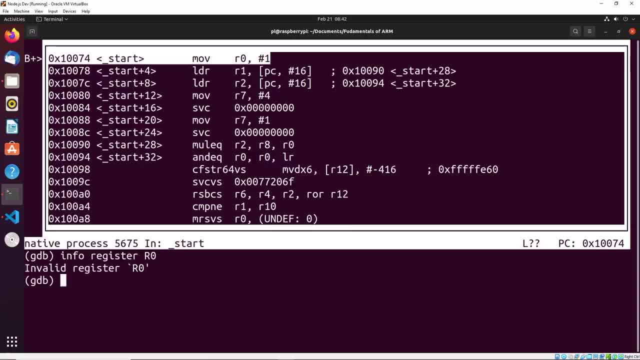 on, So I could type in, for instance, our zero. Oh, sorry, I have to do it as a lowercase r. So the info register, our zero, And you can see that it has a value of zero. So there's, there's nothing. 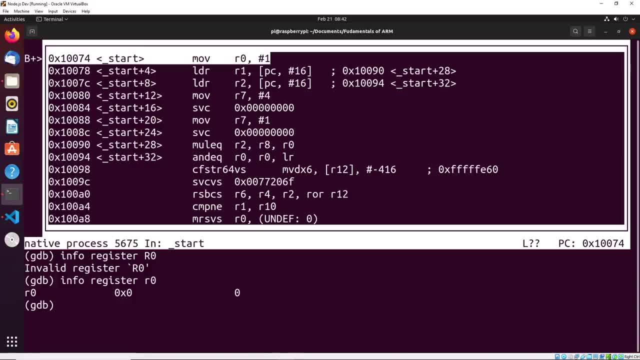 currently in it. it's set to zero currently, So that's one way that we could see the register. Another way that we could see the register is we can actually type in layouts, re GS, And you can see that. that will show all the registers above our instructions. 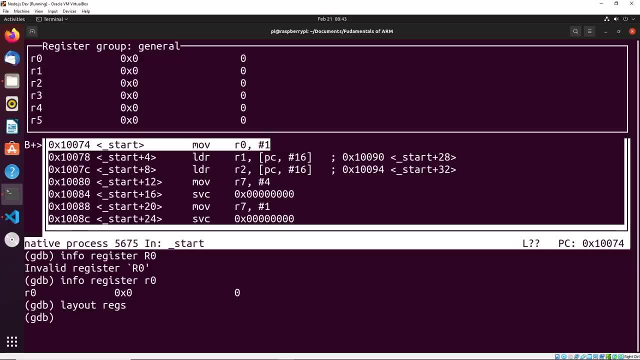 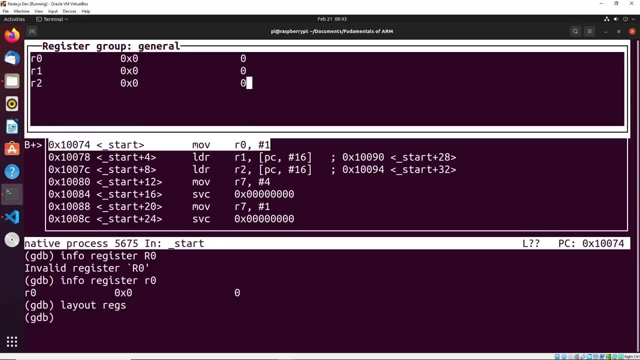 What you could do is you could type in Ctrl x and then oh, and that will allow you to switch between the instructions and the registers. So you could see. now I can scroll with the arrow keys And I could see each of the different registers that exists. So you could see like the stack. 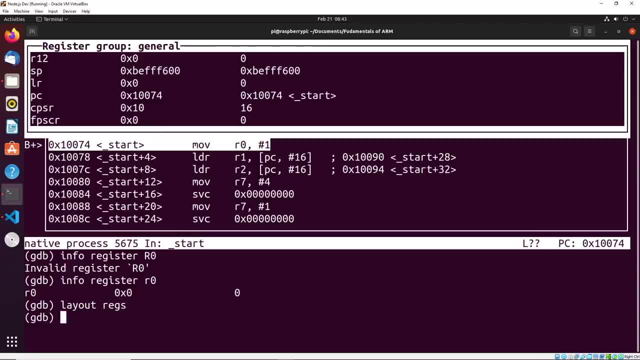 pointer, the link register, the program counter, the CPSR registers, you could see all that information that we would typically have when we were running through the emulator. Again, that's Ctrl x and then type O. after doing that, And that will let you. 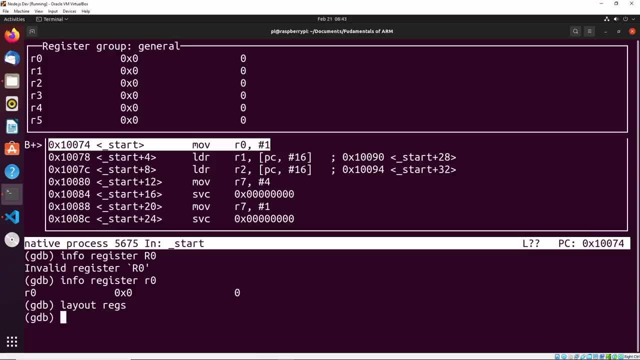 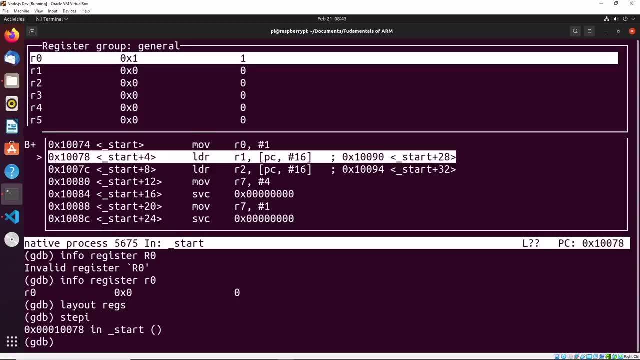 switch your interface between the layout ASM and the layout of registers So you can have both of them going and switch between them with Ctrl x o. Now from here we can step to the next instruction using step i. So I type in step i And you could see that it highlights the next line. So it 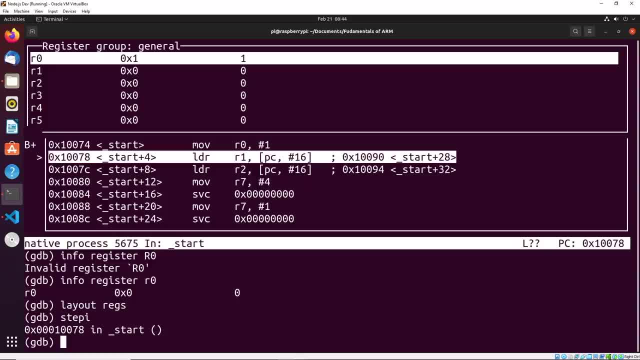 executed the first line and moves on to the next one, And we can confirm that, because if I look up at my register view, I see that our zero has been set to one, which is what happens when we do this right: we move our one into our zero, And we could see that that actually did happen. 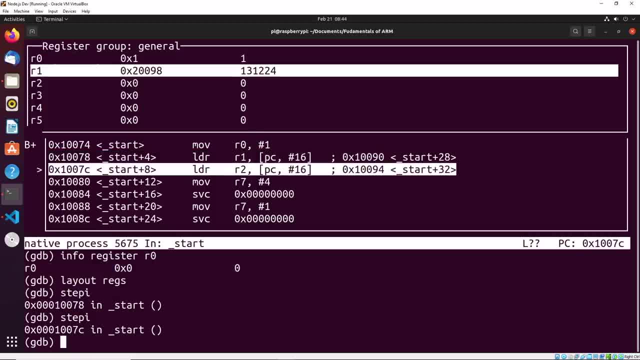 Let's step by again And you could see what's happened now is it's loaded our string into our one And you could see that it has the address of the string now stored in our one. Now the next thing I'm going to talk about here is: well, how do we actually see the string in memory? So how do? 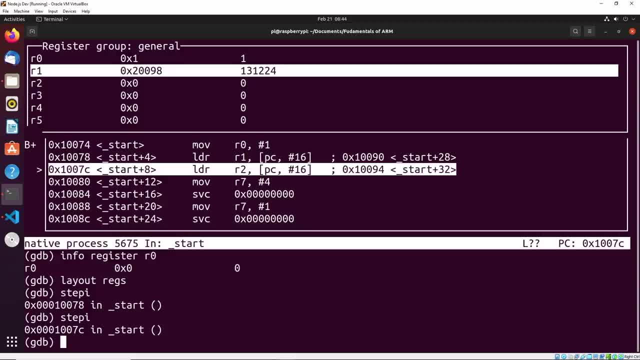 we actually see the stack memory. The way that we do this is we do the following: we do x slash x. So basically, what x is doing is it saying examine. so we're going to examine a part of memory, And then what we have to do is we have to tell GDB: how many pieces of memory do we want to? 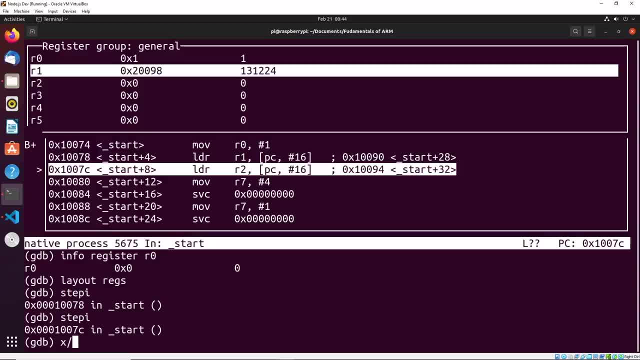 analyze And what format do we want to see it in? So for example, you could say 10x with that would do is it would show us 10 hexadecimal memory slots. So what's going to happen is we specify a starting point. So I would say address, So say I want to see the address of our one. I put dollar. 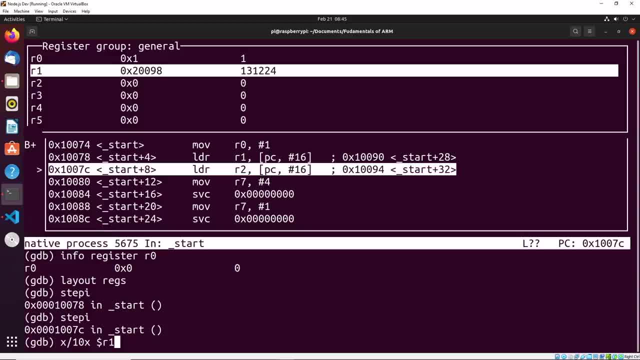 one. what's going to happen is it's going to start at the address of our one, which is 20098.. And it's going to show me 10 hexadecimal starting at that point. So it starts at 20098.. And then it 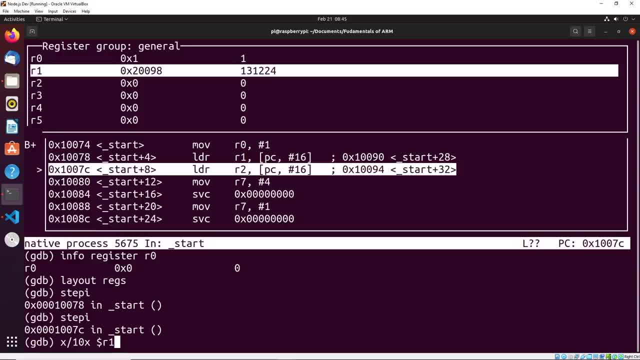 goes to the next memory slot and then the next one, until it showed me 10 hexadecimal values. You can see. when I press Enter, that's exactly what happens, right? So we see the 20098.. Right, this is the first slot, and then the second slot, and then the third, fourth, fifth, all the way up. 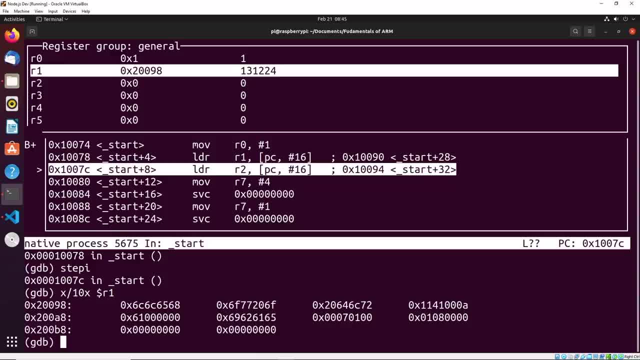 to 10.. Right, So you can see that. that generally shows us the hexadecimal values. Now, looking at these values here, it's not necessarily clear what each of these represents. right, We could see that each of these is a single piece of our stack memory. you know, this really parallels the same. 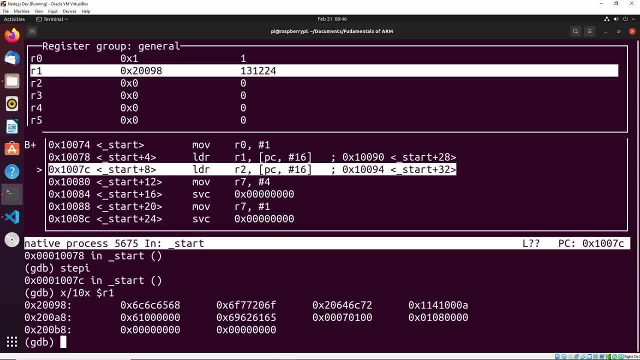 ideas as our emulator right. Nothing's really changed. there's still the same number of- like hexadecimal values per slot of memory. we're still working with 32 bits for every single piece of memory here, right? So you can see we have 10 32 bit slots. that's what's really happened here. Now, of course, looking at the 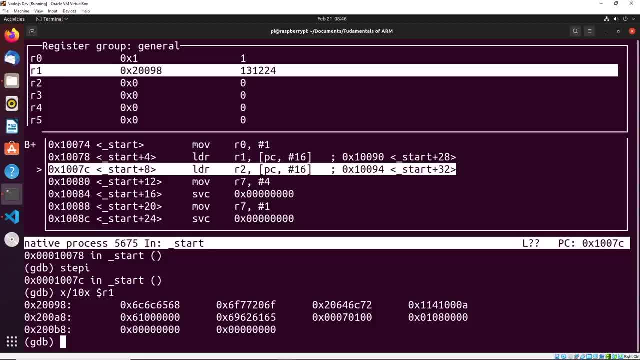 hexadecimal numbers is a little bit confusing. So what you can actually do is you could specify different formats. I can view these in decimal. by changing the x to a D like this, You can see that it gives us decimal values. again, still not entirely clear. So let's do something different. 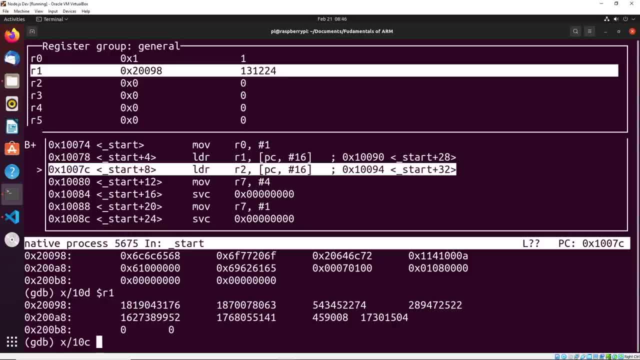 we can actually specify character using 10 C. So C is character, D is decimal. Just to give you a few more here: U is unsigned decimal, So that sort of gives you all the same ones that you would have had in the emulator right: x for hexadecimal, D for decimal, U for unsigned decimal. But then we 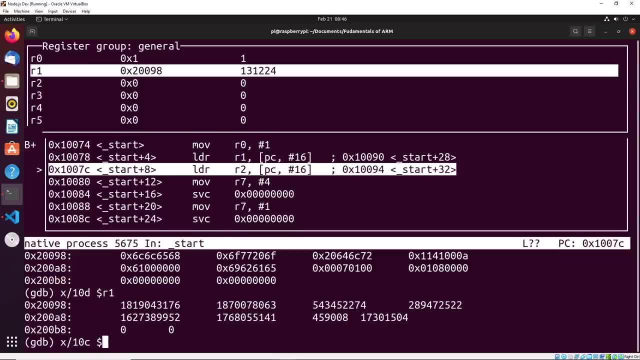 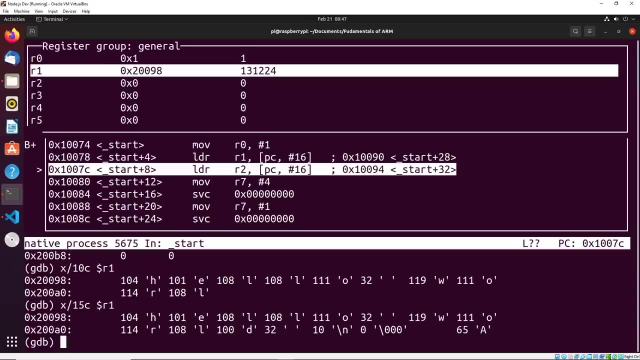 also have to see for character, which is nice. When I do this one, what you'll see is our string right, Hello world. I don't quite have enough numbers here. Let me put in 15 should be enough. Yeah, you see, there we go. We have Hello world, backslash n, And then you see that, backslash zero. 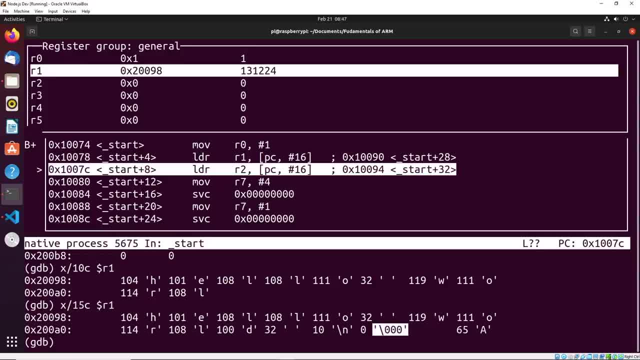 zero, zero here. let me highlight it here. This right here is the null terminator that I was talking about. It's the special character that indicates the end of the string. So that's something interesting to sort of point out here. that's the null terminator for our string. So you could see. 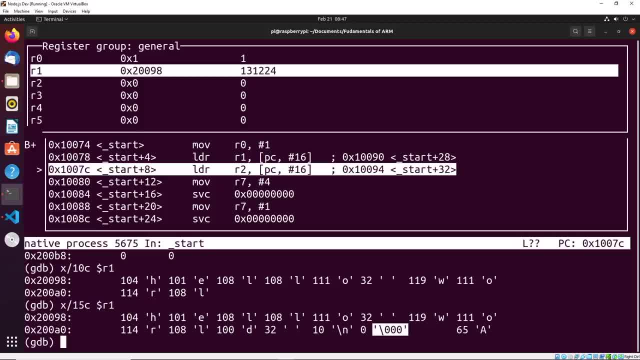 that this is each of the different values that exists inside of our memory. right, you can actually see that each of these does represent the characters that we were expecting. right, we have the Hello world string with the null terminator and the backslash n for the new line. 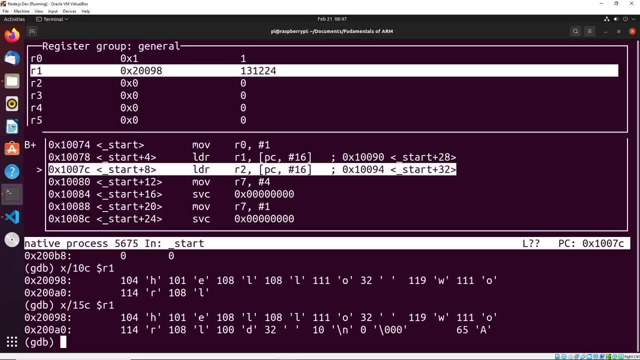 all stored in stack memory. So this allows you to actually see what's being stored in that memory, So you could see that you have a lot of the same troubleshooting techniques as we had when we are working in the actual emulator itself. And again, we can continue through this, we can continue. 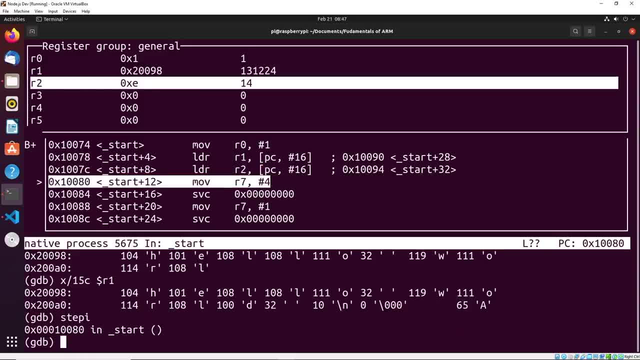 stepping through as much as we'd like, you could see that we have generally the length of the string being stored and then we do our system calls And you know we move on as as is right. if you want to just like complete the execution, you can just type in run again And what will? 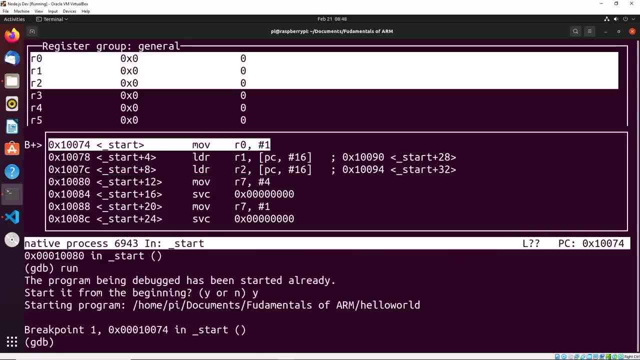 happen is we'll actually run will take us back to the beginning. we can remove the breakpoint, for instance, and then run it again. But generally the way they interact with the application through GDB would be stepping through, step by step to sort of debug problems And then 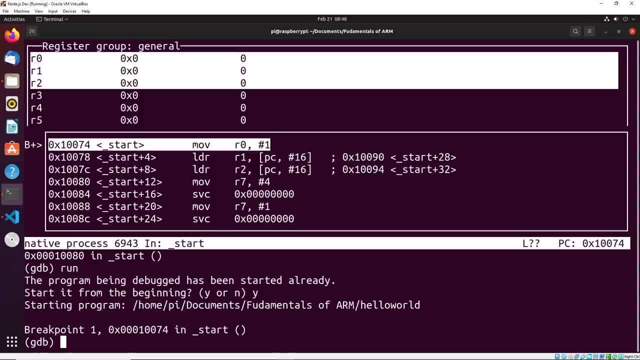 the way that you would run. it is what we saw in the previous video where we did the dot slash, you know, and then running the program as is. So this should hopefully give you a bit of a better understanding of how we can actually debug our applications, And you're going to see this a fair 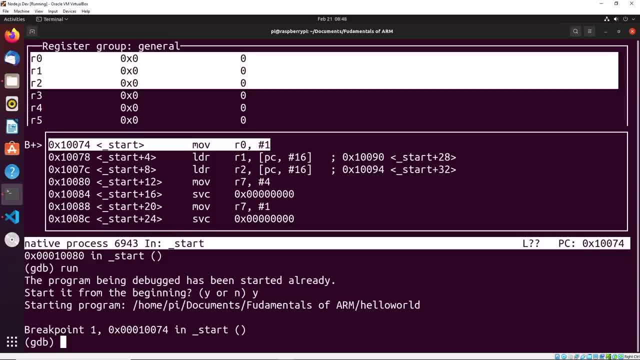 bit whenever we're working in assembly. you're going to see this a fair bit. whenever we're working in assembly, I'm going to be using this debugger to sort of show you the general idea of what is happening when we're going through each of these different memory locations. So not to worry.